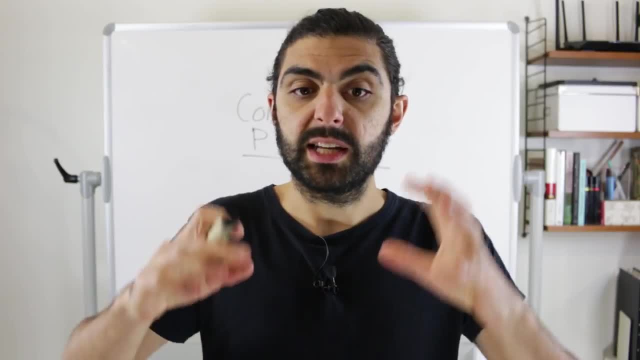 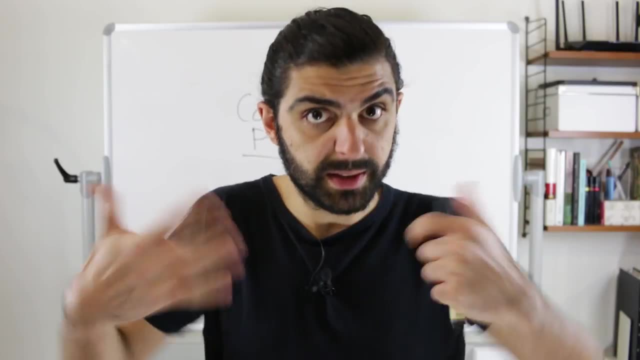 whenever you have a problem of that sort. But when you have a problem of that sort, it might be super helpful for you to actually be able to treat them uniformly, to be able to apply the same operation, to run the same function on a single object or a collection of objects. But let's start to think. 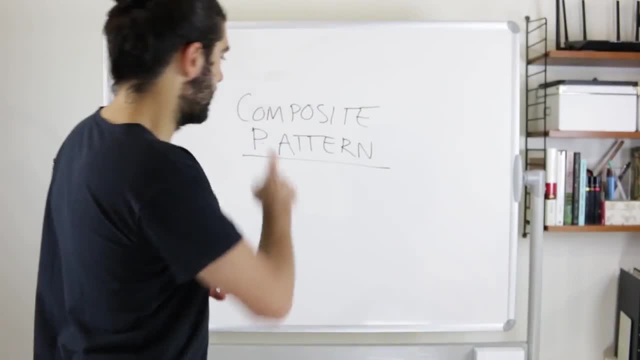 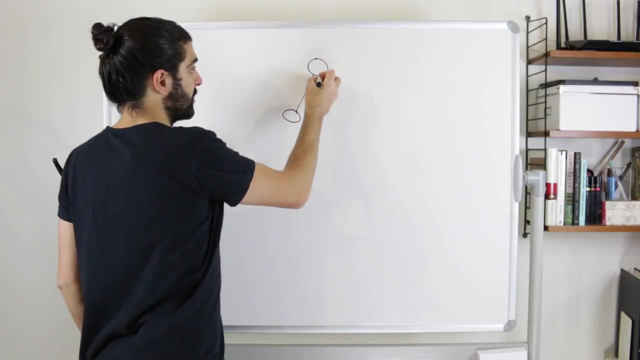 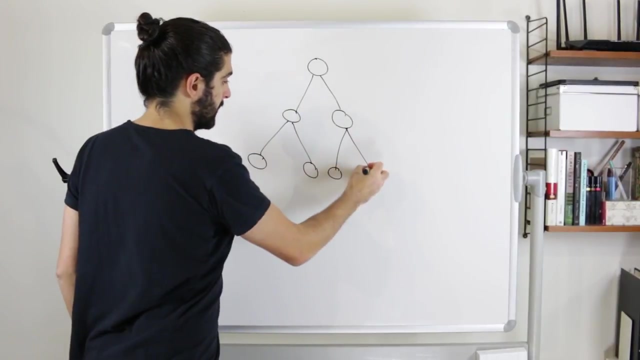 about family trees. So what if? let me just remove this first. So if this is me and I have two parents, let's say these are my two parents, but my two parents both have two parents, So these are their two parents- Then we have a tree structure. And if we think about this tree structure there, 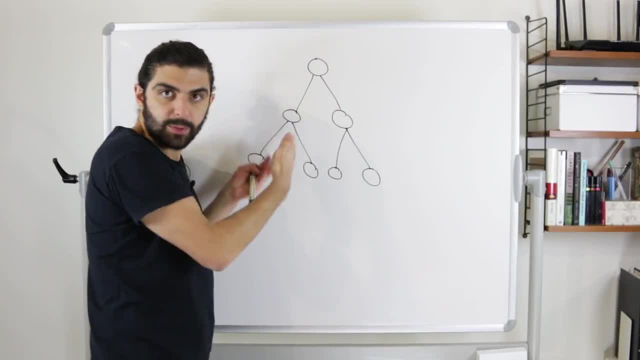 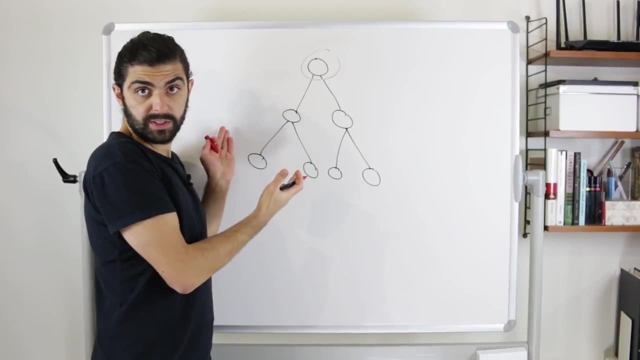 are some particular properties or phenomena or things that we can name or talk about in relation to this tree structure. One is that we have a tree structure And if we think about this tree structure, we can say that I am the root. right, I am the root of this tree structure, But also 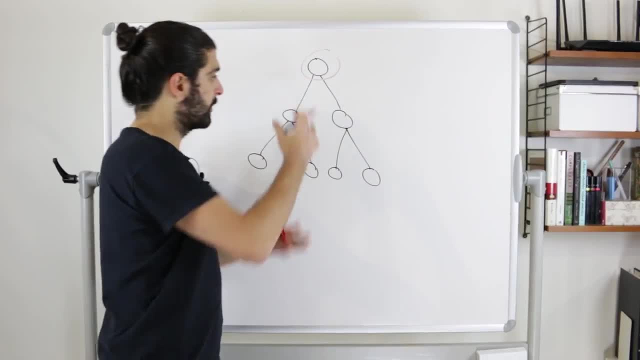 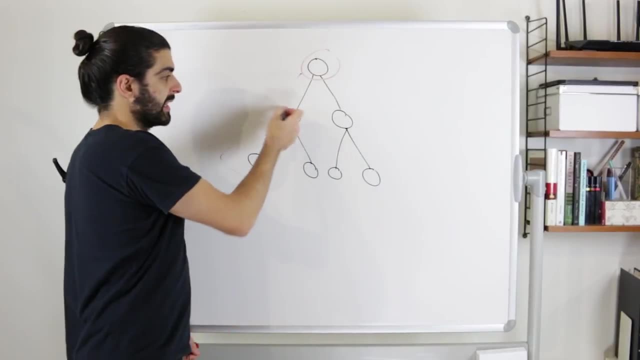 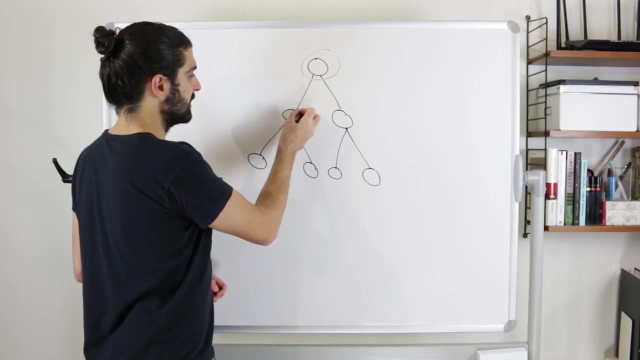 if you take dependencies downwards from any point, from my point you have the whole tree right. I encompass the whole tree, Whereas if you would take this particular node, for example, that doesn't encompass this whole tree And I guess that's a consequence of being the root. But if you look at 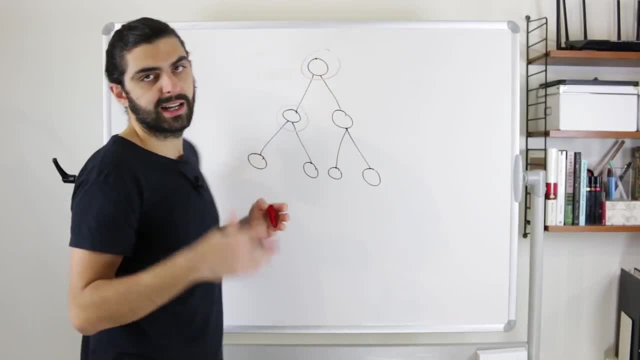 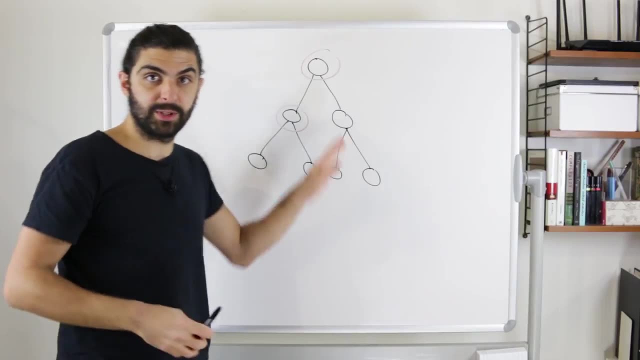 only this node. it has, let's say, children. So it's a bit funny because I flipped the order of this example. Oftentimes it's a bit funny because it's a bit funny. because it's a bit funny because we talk about parents and children when we draw trees And then we say that this node has two. 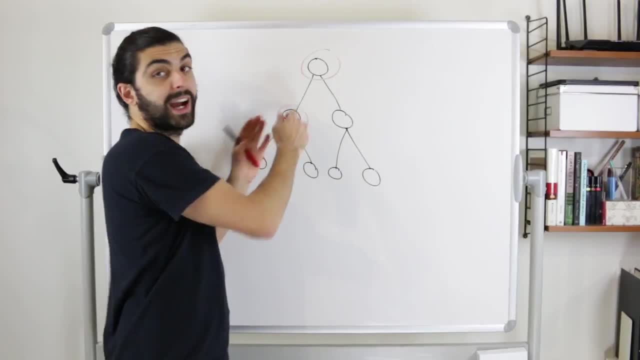 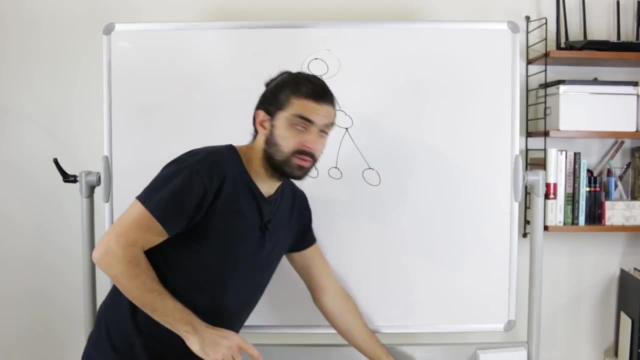 children. But now, since I'm using a family example, the child is upward, So sorry about that potential confusion. So let me instead say that this node references two other nodes. Let me do this also. Let me make this directional right, Because I haven't specified directions. 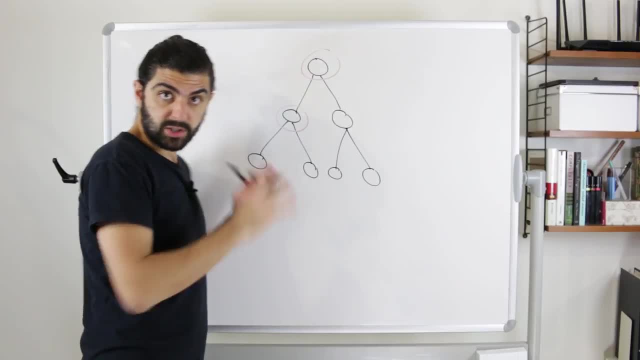 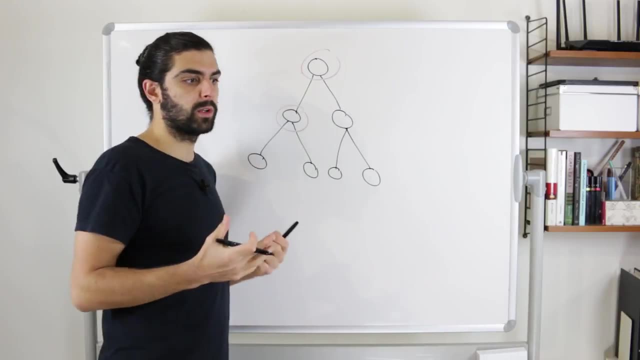 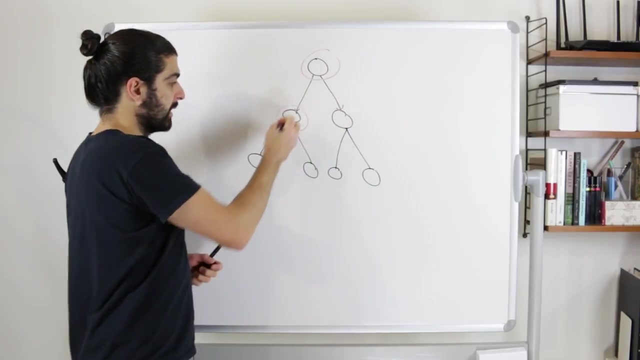 of the arrows, So we are not sure who references who. But just within this example, let's talk about the notion of having a parent, right? So we're not modeling the two-way relationship, we're modeling nodes that have parents. So again, I have one parent and another parent, And the 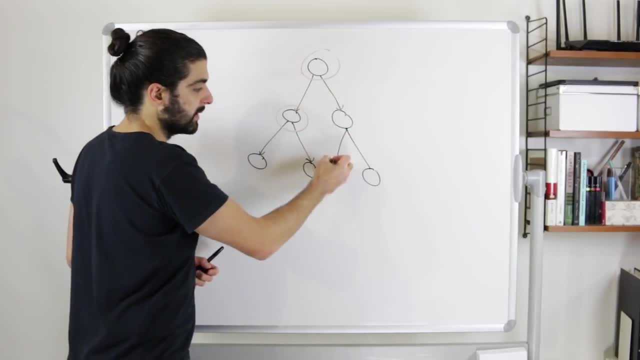 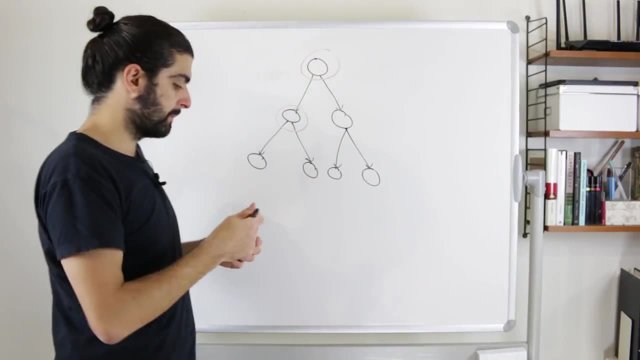 first parent has one parent and another parent, And the second parent has a first parent and a second parent, And then we could go on right, Like we could go on indefinitely. clearly, But back to this scenario. If you think about this node, if you would look at the subset of this tree, 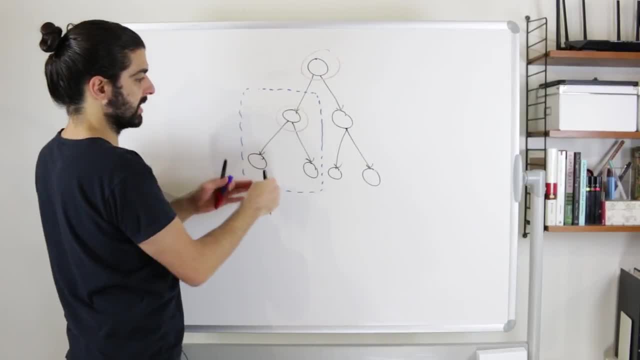 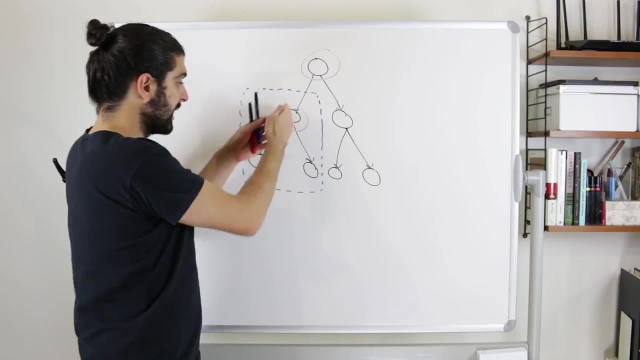 like this right. So let me do this dashed right And let me just think about this dashed square here. If you only think about this portion, then this node is the root. This node is the root and it has it references two other nodes. 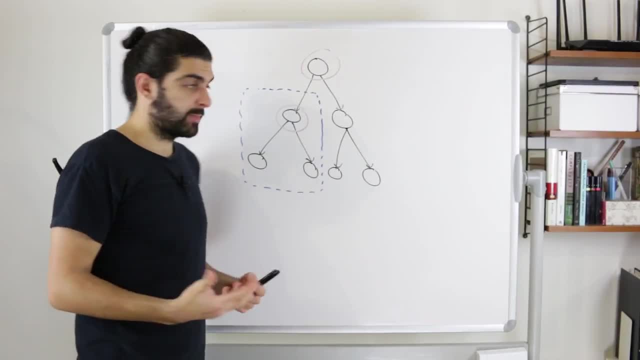 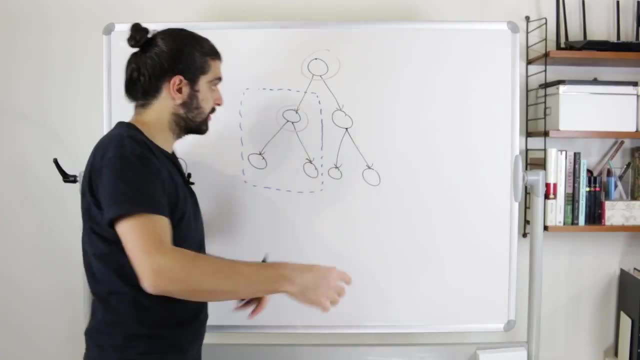 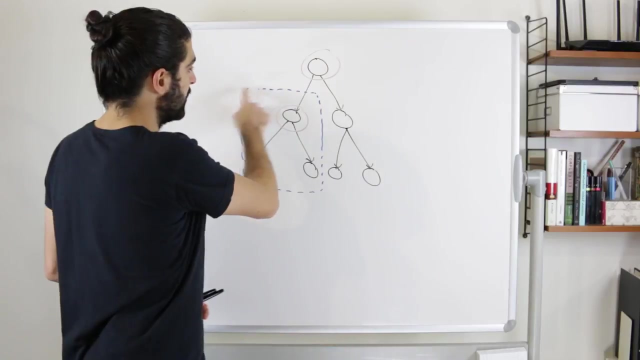 It has two subnodes. So in the context of composite pattern, this is a composite. So the root is a composite because it has, it contains, multiple nodes. This node, in other words one of my parents, is also a composite because it contains multiple nodes downwards. I only drew 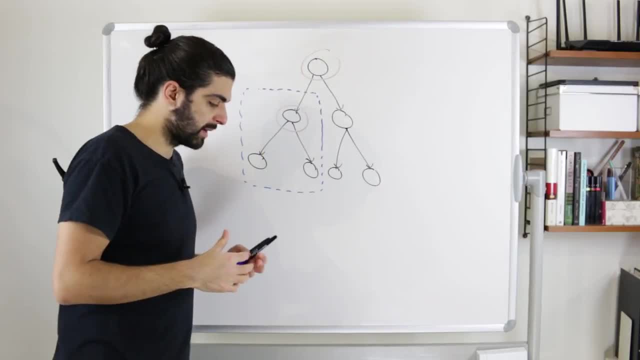 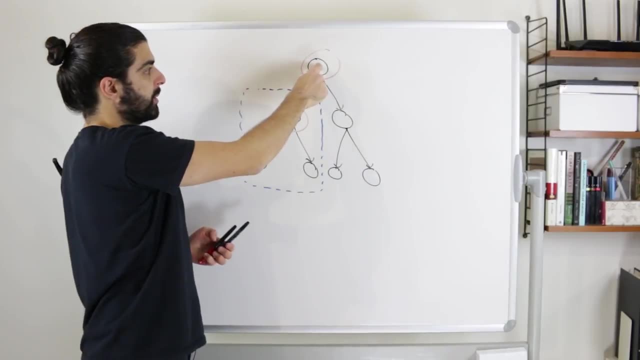 this just so that we could think about the fact that if you only think about it in steps of one level right, Or in relation to one node, you can think of it like this: So from the perspective of this node, from the perspective of me, what we have is that we have one node that references 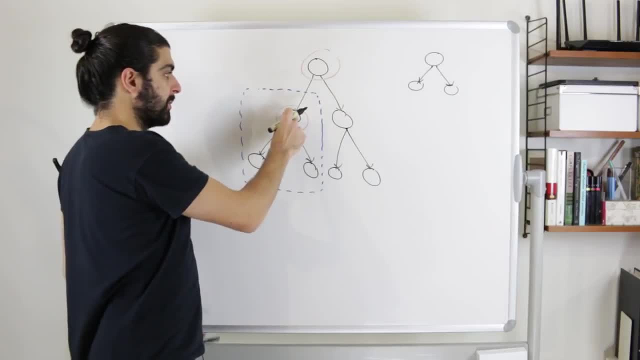 two nodes. But if you change your perspective and you think from the perspective of this node, from the perspective of one of these nodes that happens to be somewhere in a hierarchy, from this node's perspective, we have exactly the same scenario. right, We have one node that. 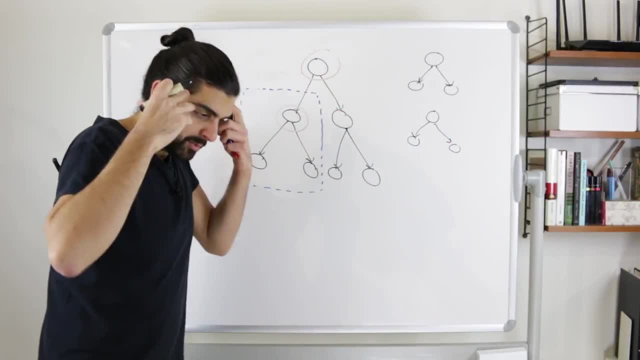 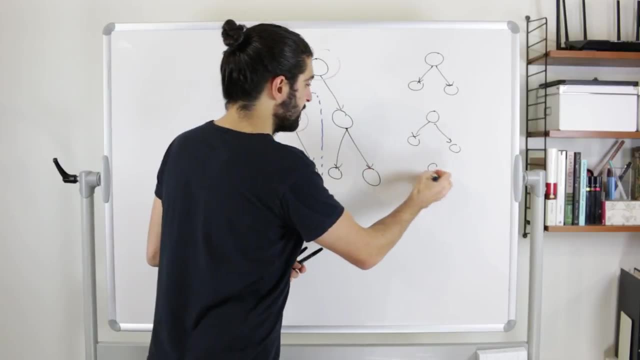 references two nodes, And if you take this node as your sort of point of departure or as your venture point for thinking, or if you look at the tree from that node's perspective, then you have the same thing again. Then you also have one node referencing two nodes. So in some 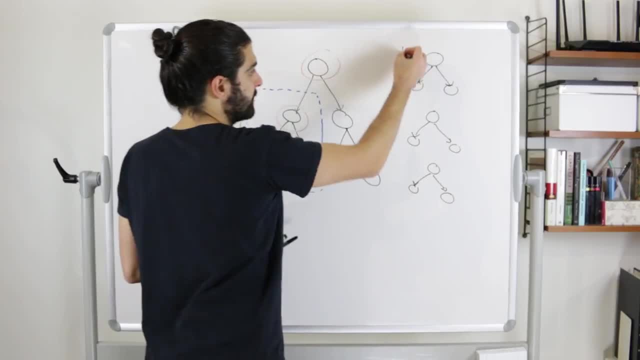 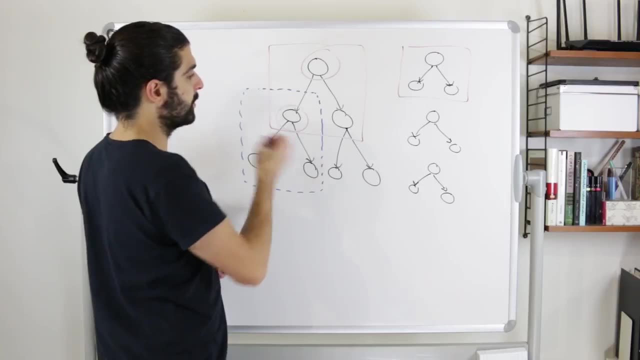 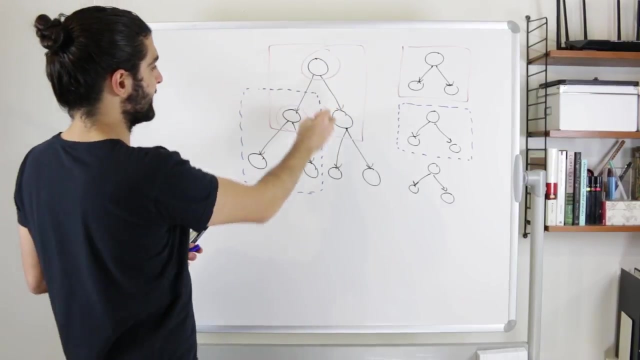 sense. now we can actually just redraw this. Let's say that this, this first triple, corresponds to these first three, to that view. This, ah, and I've already drawn the blue one, The blue one dashed corresponds to this. So this one corresponds to this slice. And then, lastly, 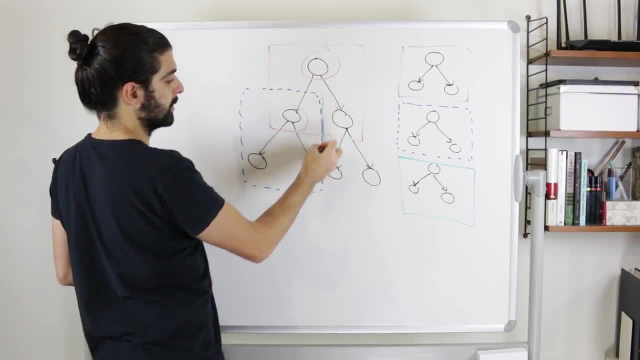 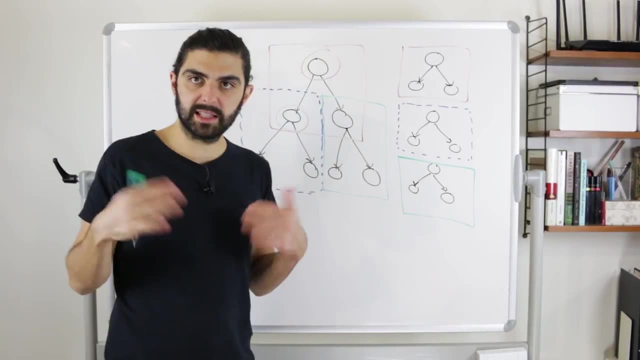 this last triple corresponds to this triple within the whole tree, And this might seem a bit stupid, but the reason I'm saying this is that this puts us in the mindset of reflecting about the notion of recursion. I don't want to talk in depth about recursion if you are not familiar. 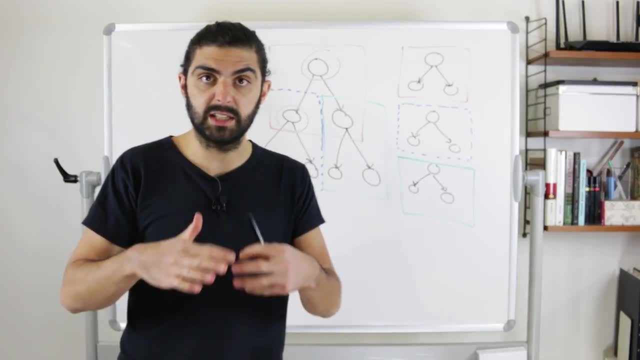 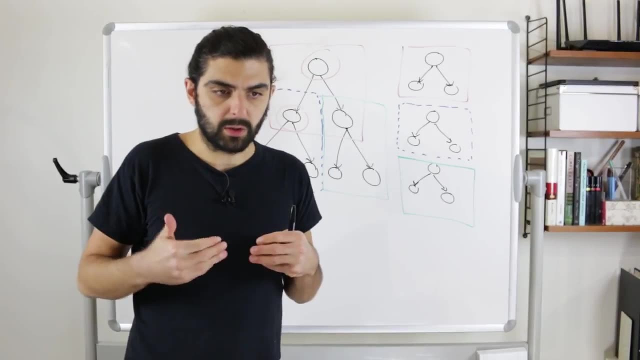 with recursion from before. If you would like me to talk about recursion in a specific video, do shoot something in the comments so we can dig into that. But recursion is essentially self-reflection or is essentially a method calling itself, But in object-oriented. 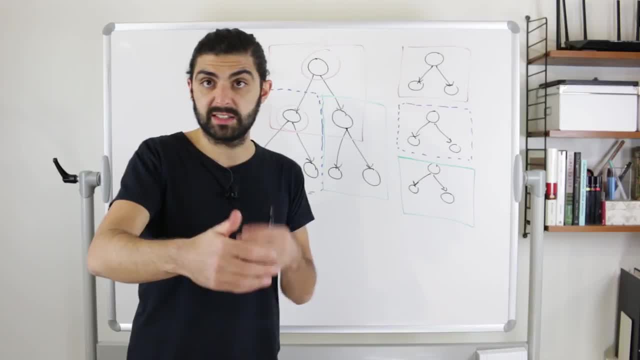 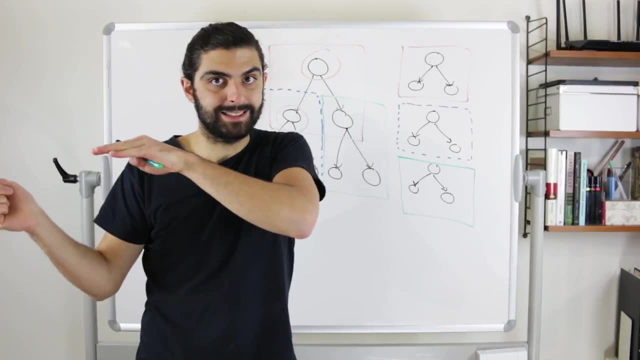 programming an object of a type calling another object of the same type. who calls another object of the same type? which essentially means that you execute the same function but on different instances. So it's the same function defined in a class but in different instances, But again. 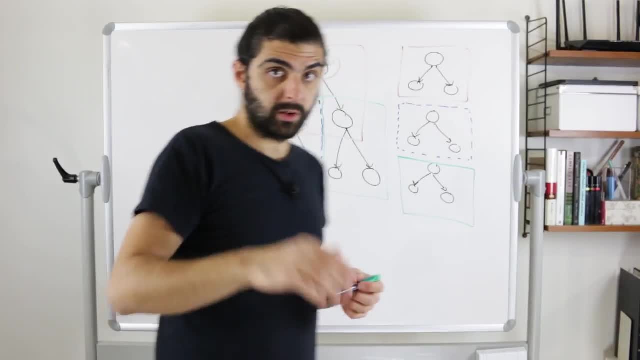 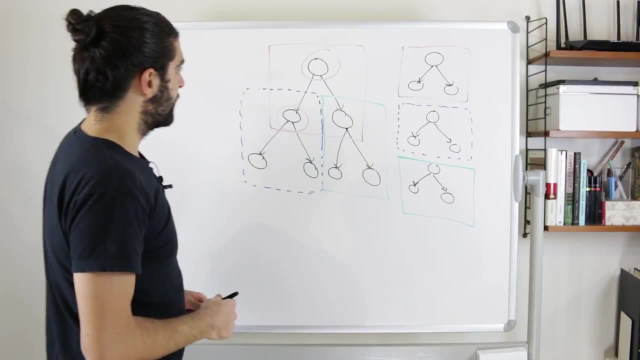 let's not think about recursion in general, unless you want to but then ping something in the comments. So again, if we look at these slices, we have these sort of cuts of three. But if we think about it in a different way, let's think about every node at a time, right? So if you 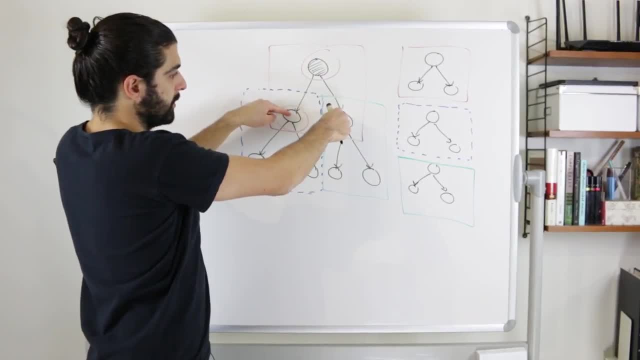 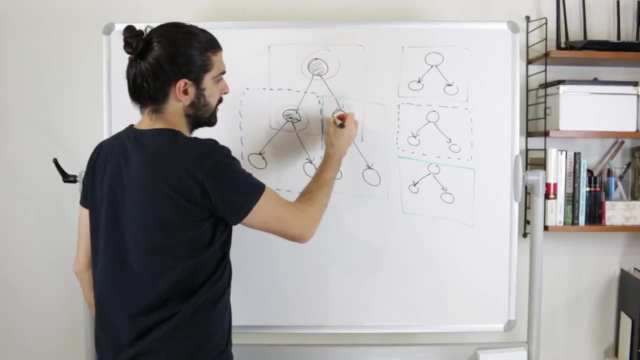 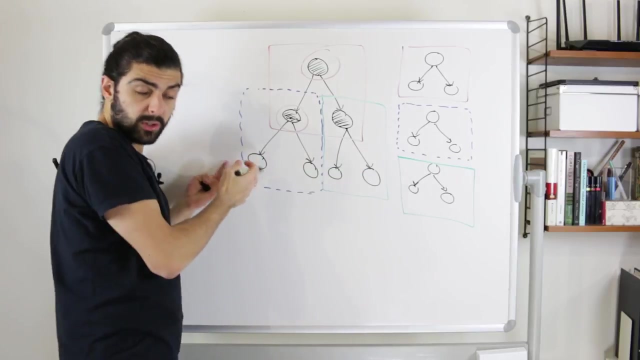 this node is a composite node because it references two nodes. This node is also a composite node because it references two nodes Further. this node is also a composite node because it too, references two nodes. However, these four nodes at the bottom, these are not composite nodes. 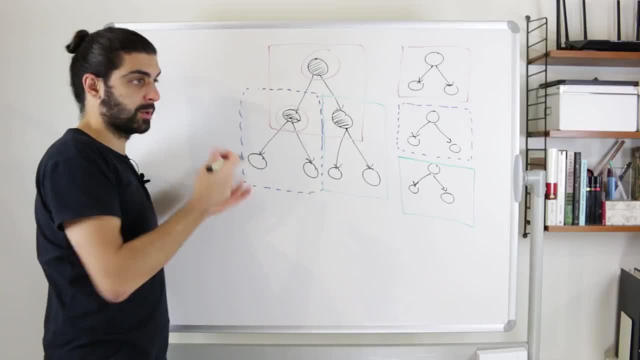 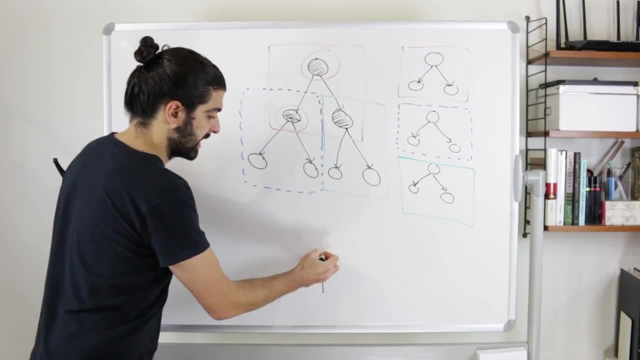 These are simply nodes, or whatever you want to call them, within the context of your composite pattern And in tree structures we tend to call them leaves. So if you think about a tree right, You have a tree which has a stem. 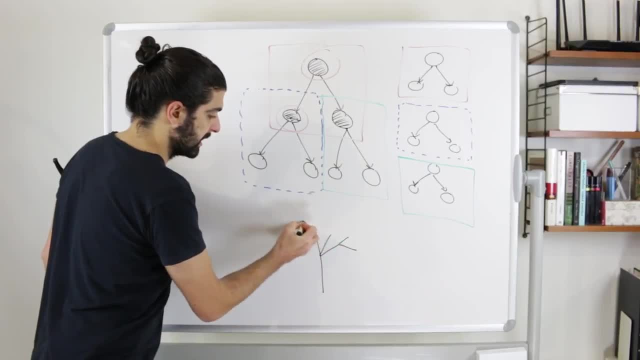 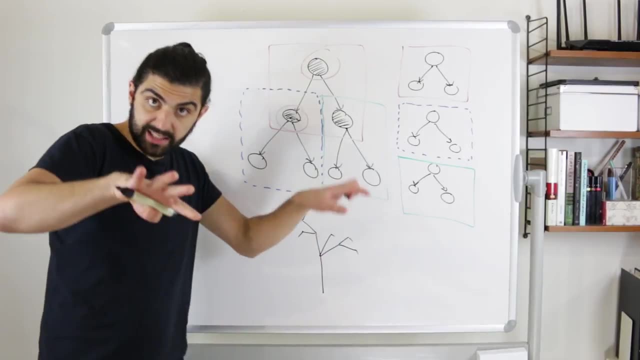 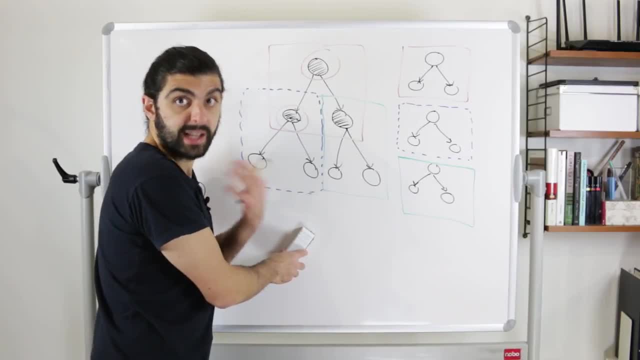 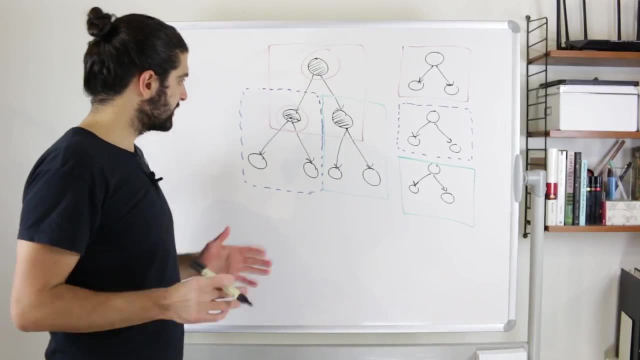 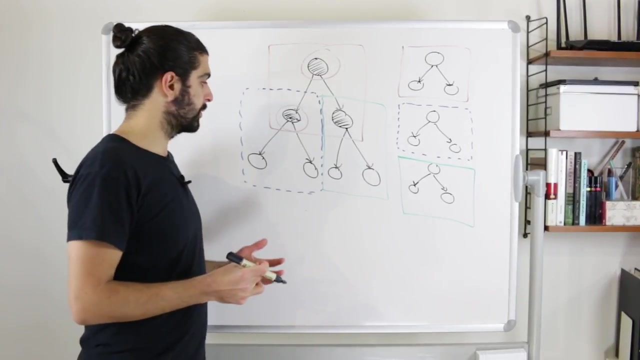 of the branch, Like branches that don't have sub-branches. So these are all leaves And essentially the point with composite pattern is that sometimes you may want to be able to perform some computation and you don't want to have to think about whether you are in a leaf. 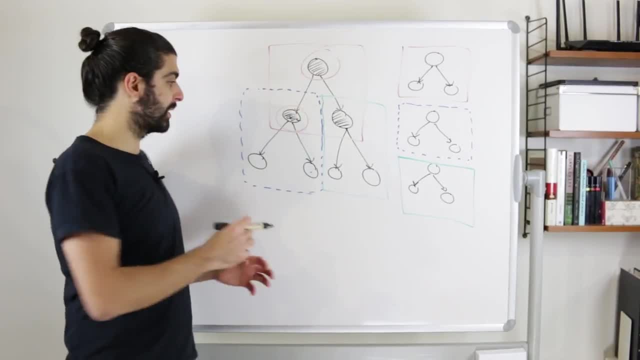 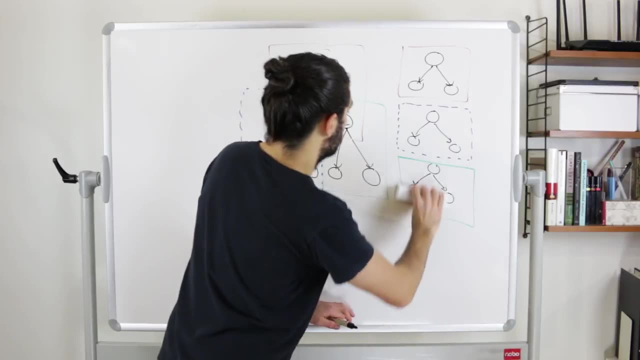 or whether you are dealing with a composite. So whether you are dealing with someone who has sub-nodes or simply someone who is a node- Let me remove this stuff on the side here. So what might one ask oneself? Let's think about it this way. Let's go back to the example of 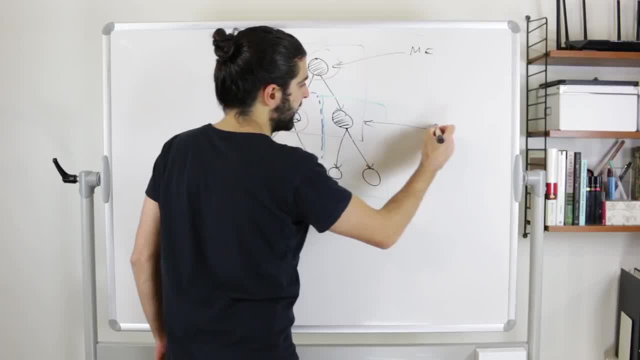 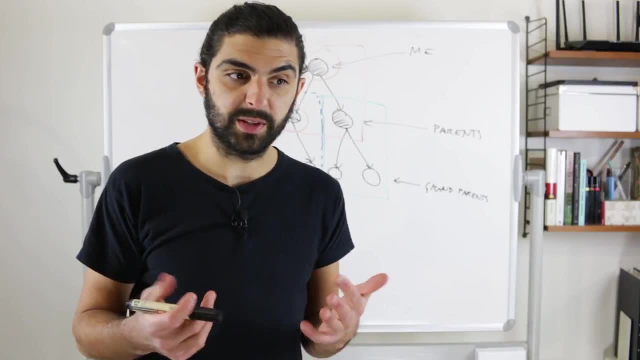 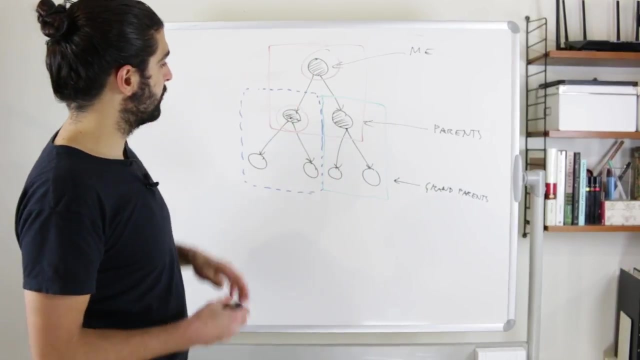 this being me right, These are my parents and these are my grandparents. So what if, for example, we wanted to write an algorithm that collects last names within this family hierarchy? So, hypothetically right, We could say: I have one last name. 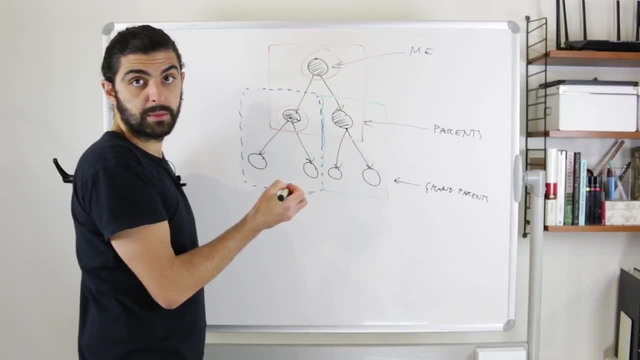 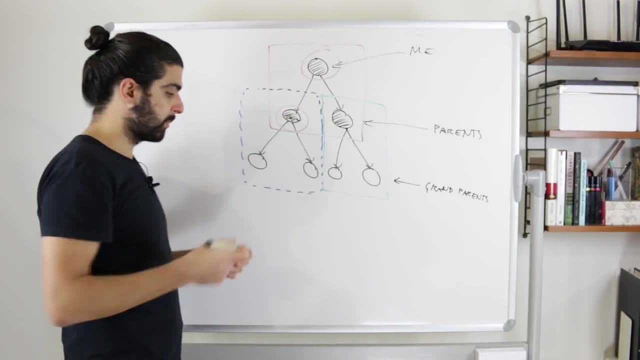 my father has one last name and my mother has another last name, And then my father's father has one last name, but my father's mother has another last name, And so forth. So let's just assume that I have the last name- A- my father, B- my mother, C- my grandfather. 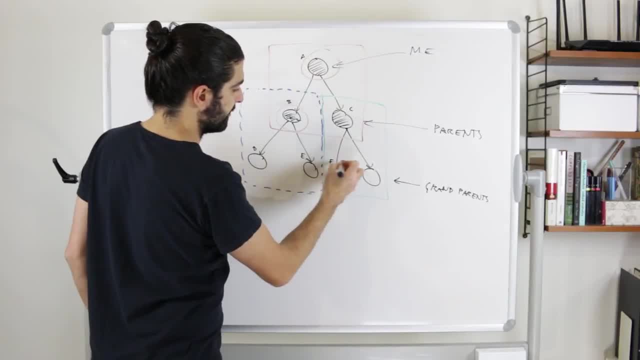 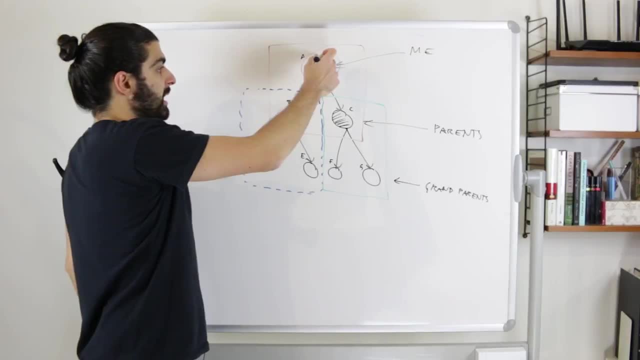 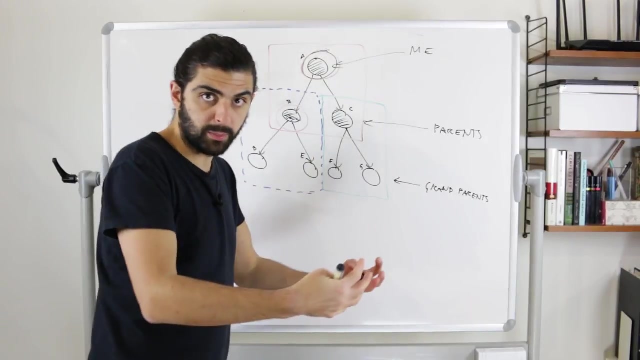 on my father's side, D, and then E, F, G, just some random names. The point is, then, that we can traverse this tree and collect the names. so if I have in my program, if I have a reference to myself, I can say: I can ask my, I can ask the composite. I can ask the composite to say get. 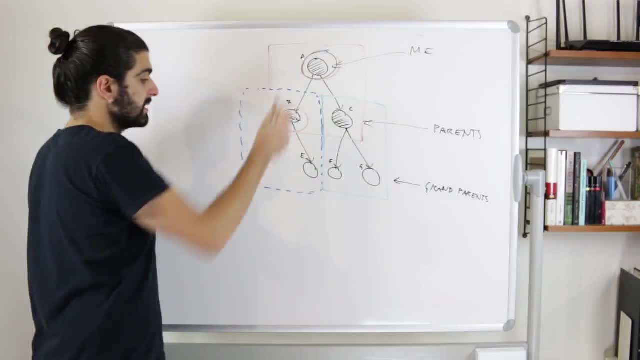 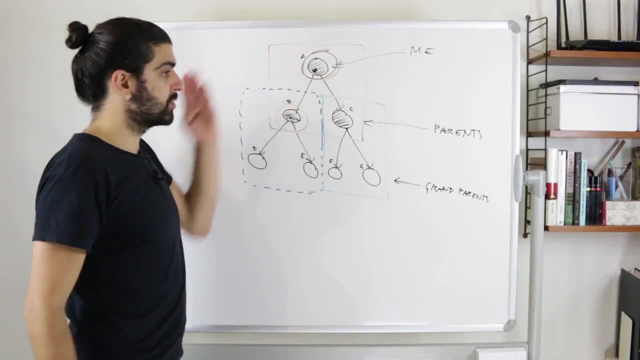 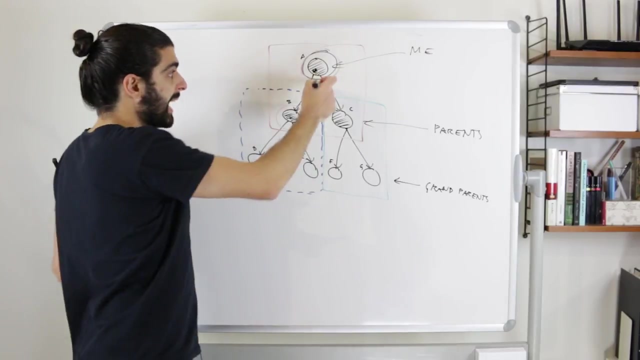 last names, for example, and what the composite would do is that it would extract the name that it has itself and then it would say: but actually, because I'm a composite, I cannot just report my own last name. I need to ask the reference I have to this object for its last name and I need to ask: 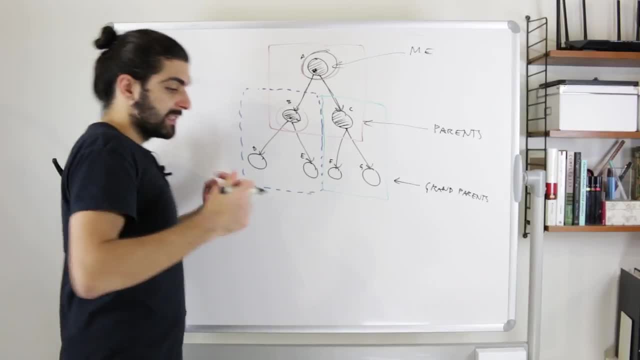 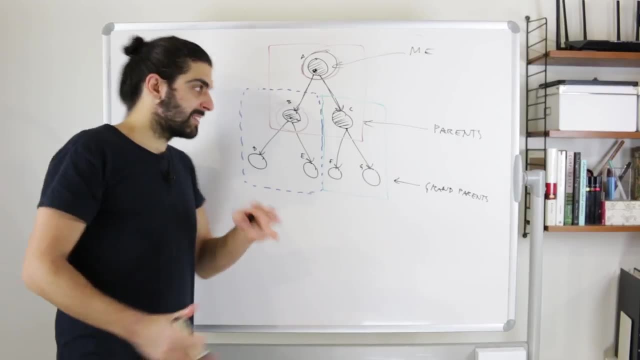 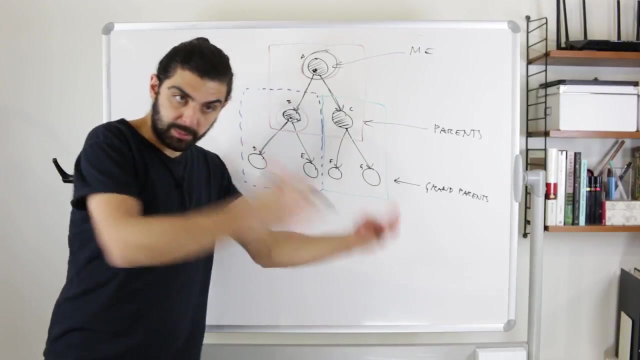 the reference I have to this object for its last name. so I, as a composite, need to ask the objects that I'm composing. I need to ask them for their last names, but because they too are composites, they will ask their children, or or their subcomponents, or the objects that they are. 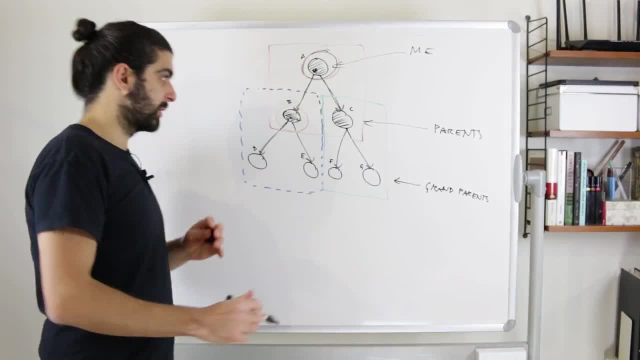 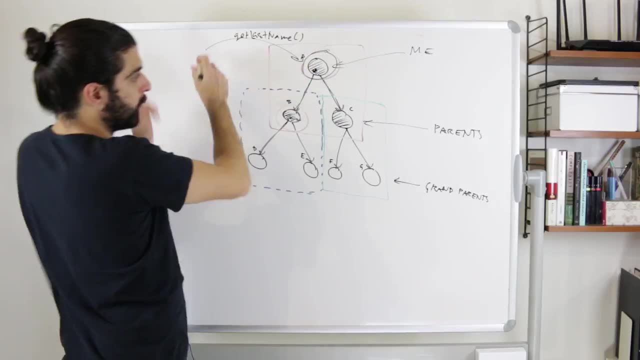 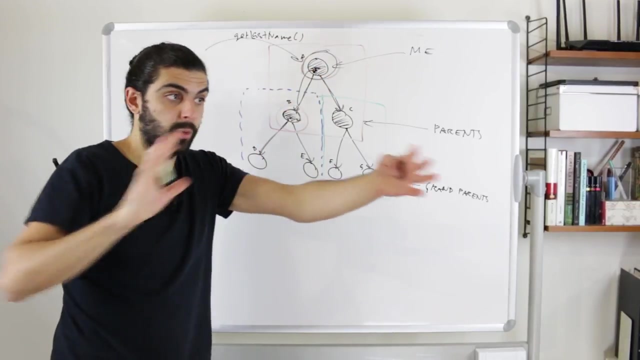 composing for their last names. and this is the way that I'm composing my own last names, the recursion. so when the program asks me for last name, say, get last name, what happens is that because i'm a composite, the method will report my name, but it will also merge that with or or. 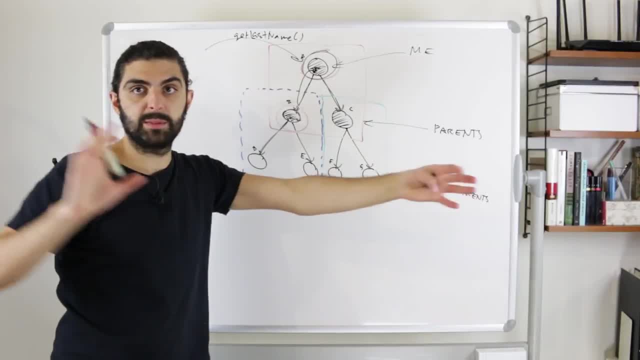 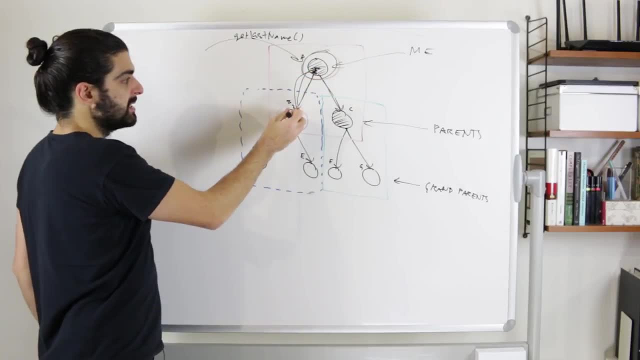 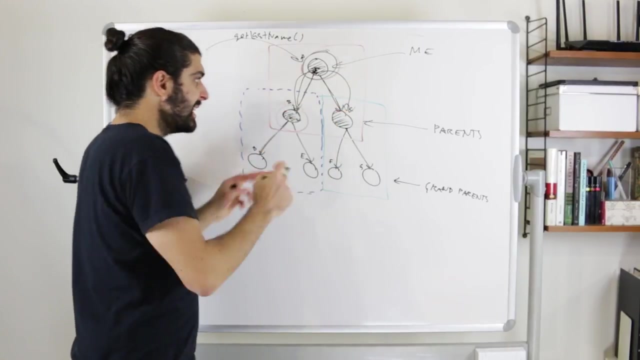 concatenate that with, let's say, we're we're constructing a comma delimited string or whatever. so it will take my name, but it will also concatenate it with whatever this node reports as its last name and whatever this node reports as its last name. but again, since these are 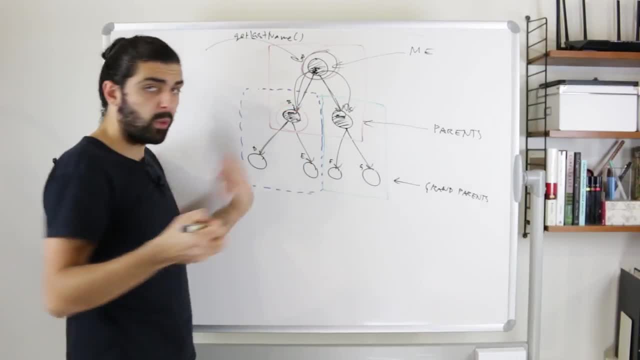 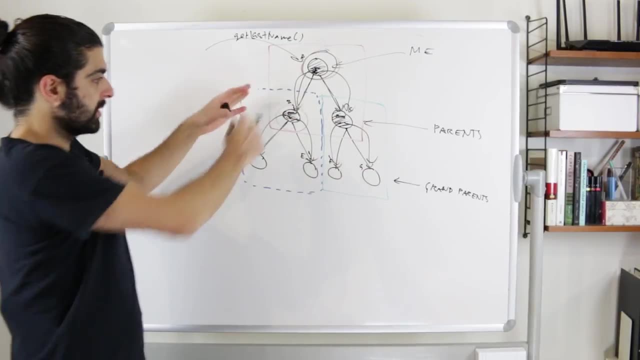 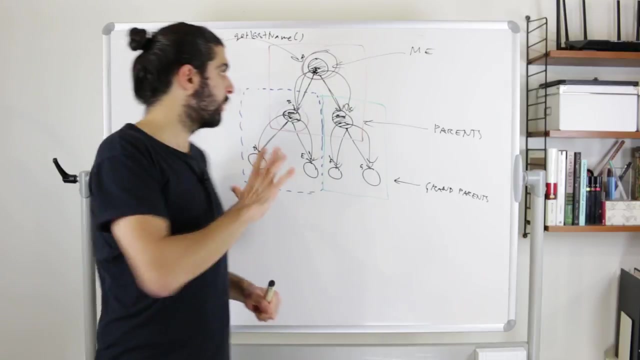 composite nodes. they will report their last names, but also the last names of their children or their sub nodes downwards. sorry, now i use the same colors for these arrows so it turned out quite messy, but i but i think you see the point right. the point of composite pattern is that when you 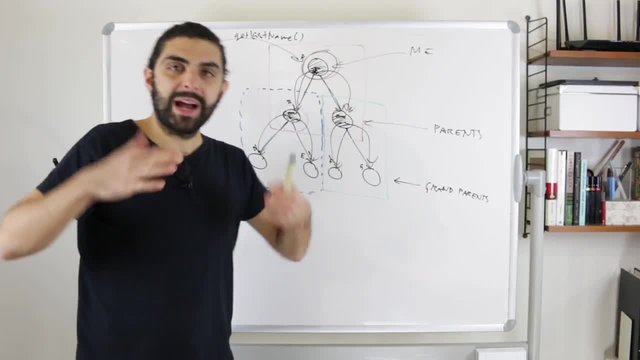 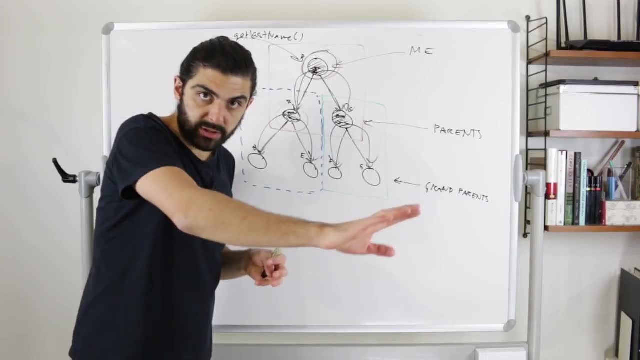 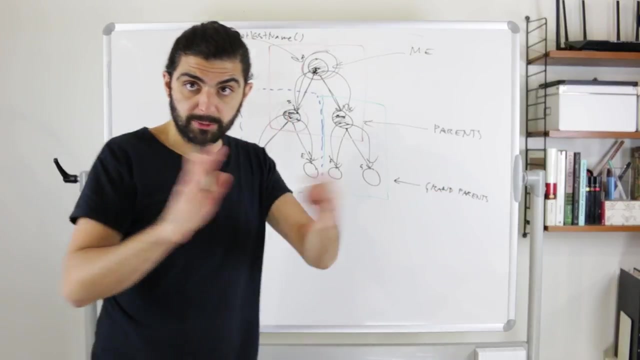 have a hierarchical structure, or let's let me put it this way- you have some data that you can usefully model as a hierarchy. then performing computation over that hierarchy becomes trivial because you can treat leaf nodes and nodes uniformly, which means that you don't have to 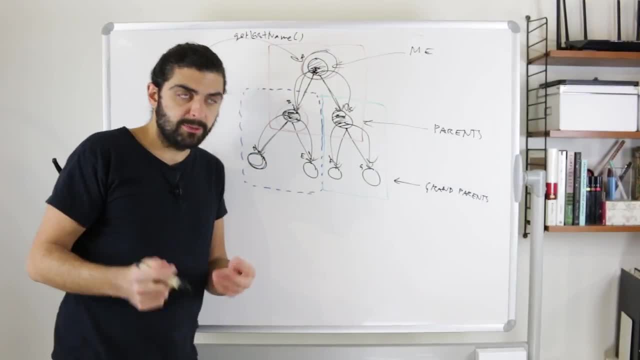 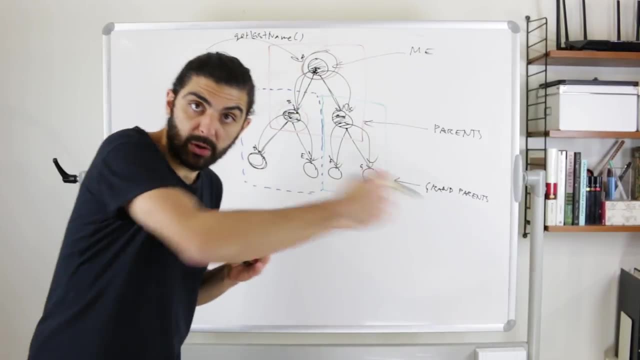 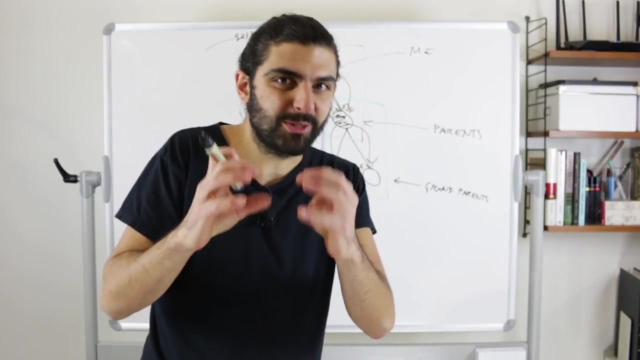 if statements to say if i am a leaf, or if the length of my children or, sorry, in this case, the length of my parents, right, the length of my sub nodes. if i have no sub nodes, then do this else? do that in some sense? in some sense, that's the only piece of logic that we're trying to get rid of, right, we are trying to 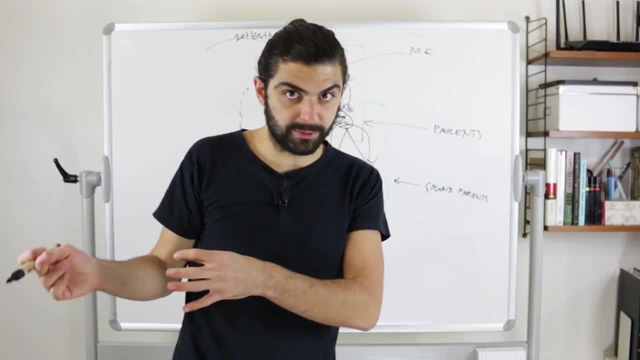 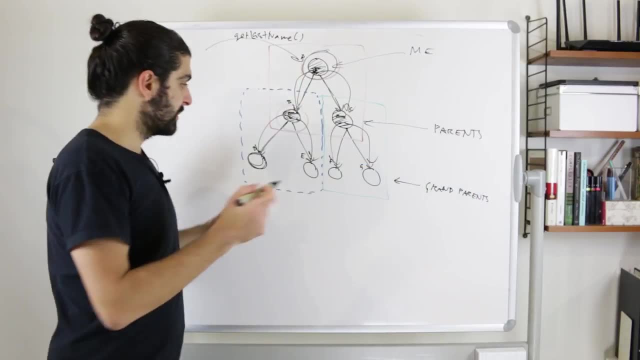 if you think about refactoring, replace a conditional with polymorphism. so instead of saying that we have a branch where in one case you do this and in one case you do that, we simply use polymorphism to specify that there are two types. maybe this i didn't say clearly enough before. 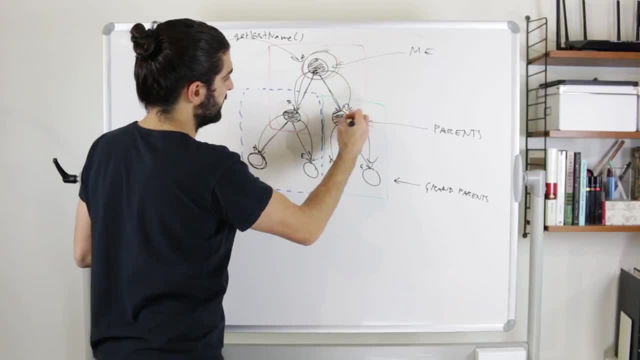 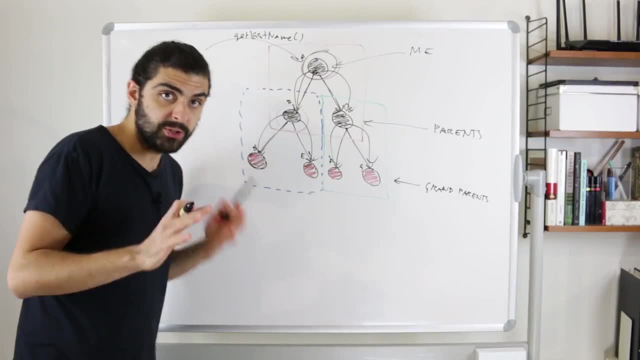 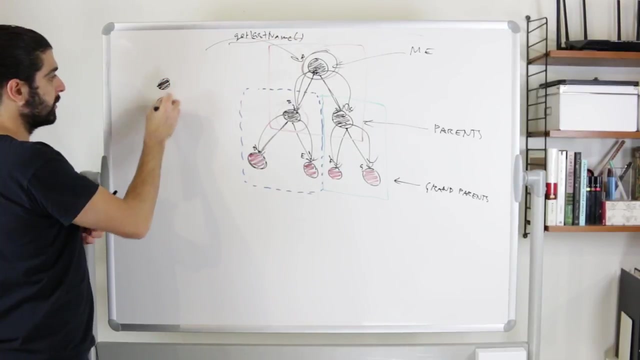 but i mark these, these three nodes, as sort of solid because they are one type and let's mark these in red instead. so these leaf nodes are of a different type, so the implementation for get last name will be one thing. so there will be one implementation for these nodes and there 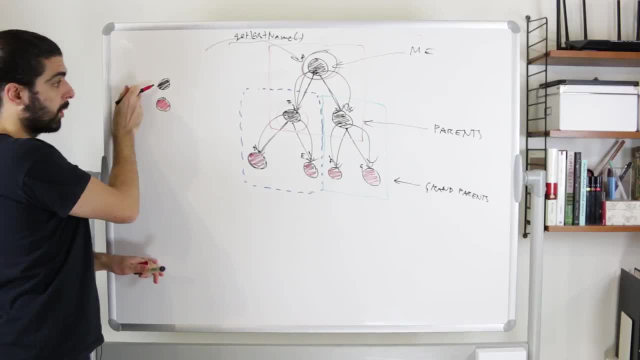 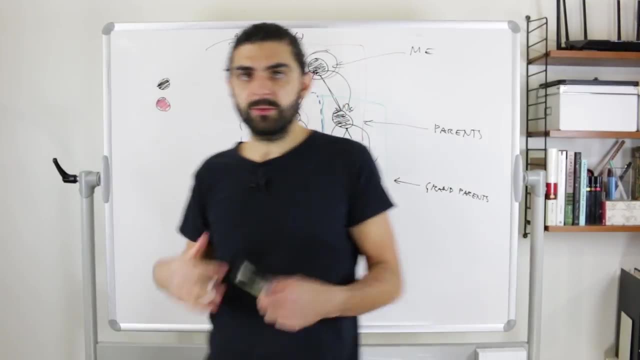 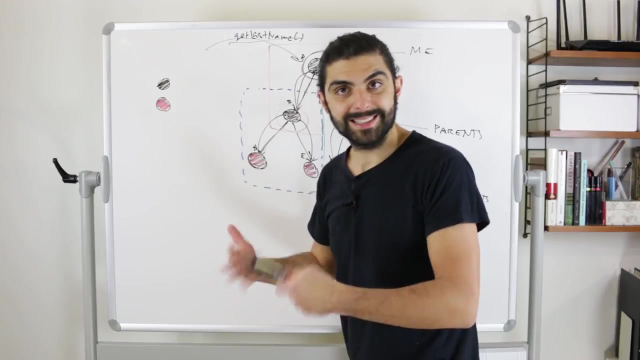 will be another implementation for these nodes. so composite nodes have one implementation and leaf nodes have another implementation. and now that we're saying replace conditionals with polymorphism, the point is that by doing that and then making them both inherit from the same superclass or implement the same interface or be part of the same inheritance hierarchy, right be of the same. 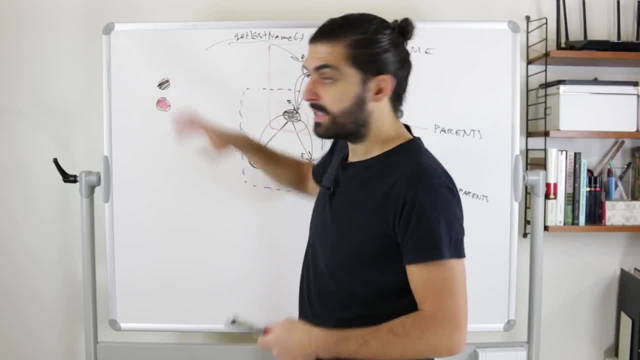 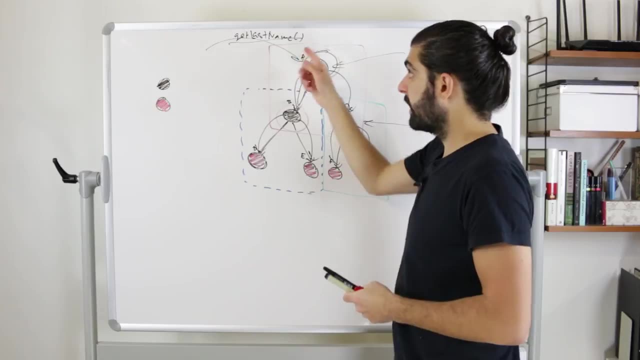 interface right be able to be treated uniformly. since they are able to be treated as the same thing, we can put them in a data structure and then simply traverse that data structure and ask the nodes to run the method, get last name and we don't ever have to think about whether any particular 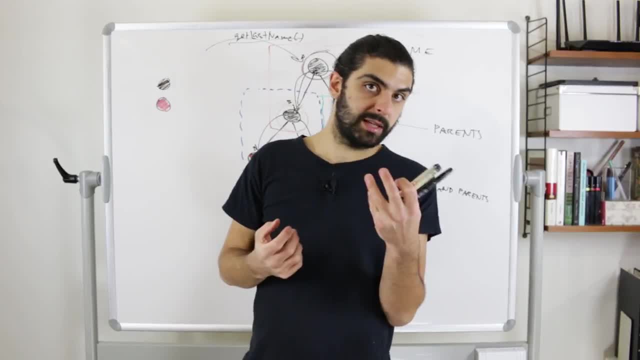 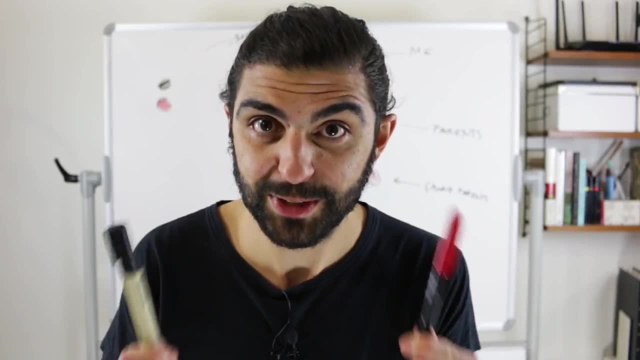 component happens to be a composite or happens to be a leaf, or happens to be a leaf, and thus we eliminate that if statement. but i've been talking for way too long without actually giving a definition for the composite pattern, so let's look at a definition. so i want to read you the 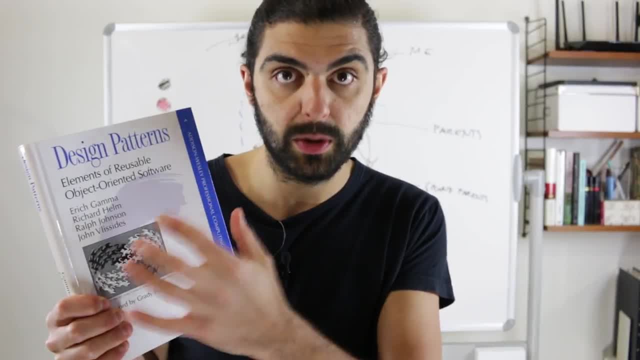 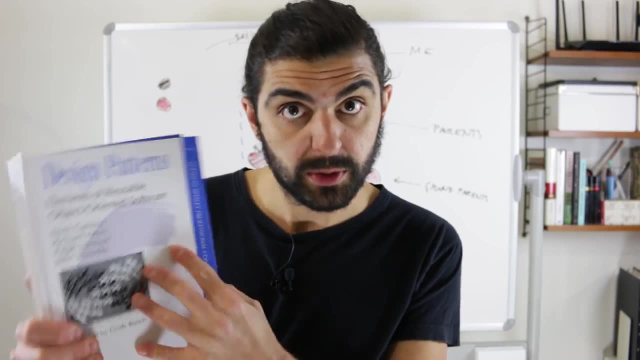 definition from this book: design patterns- elements of reusable object-oriented software. it's written by gang of four and this is like the classic design patterns book that sort of tried to put names on things that i assume other people were also doing and, by the way, i highly recommend that. 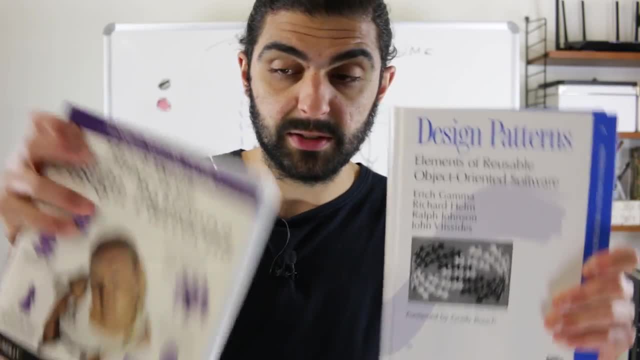 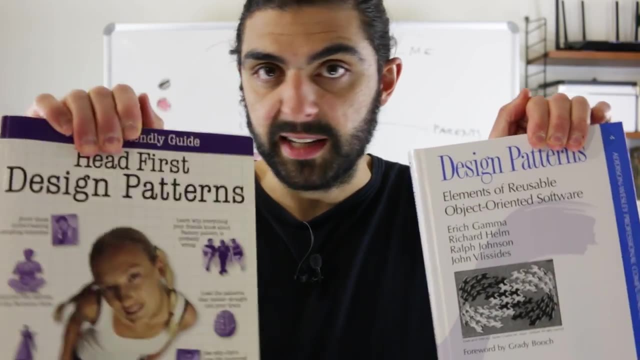 you get this book or this book headfirst design patterns. so this book headfirst design patterns i would say is better if you want something very pedagogical. it has more images, more fun examples and all of that stuff. but if you want something that's more like a reference book, get this. 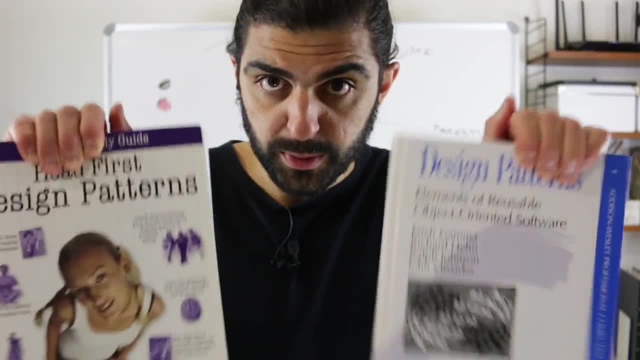 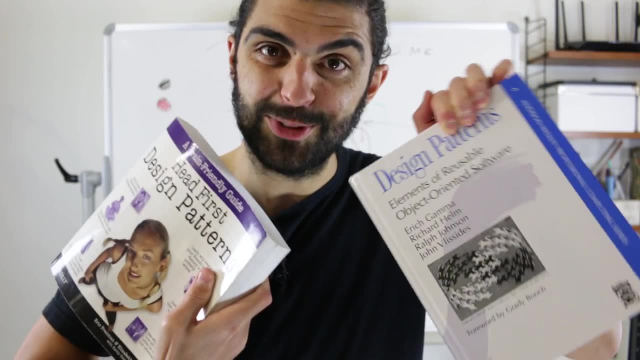 four design patterns book and, when in doubt, just get both super good books. even if i cover a lot of stuff in these design pattern videos, there's a lot of stuff left to be discussed, and this stuff you can find in these books. links are in the description. let's move on now to the definition. 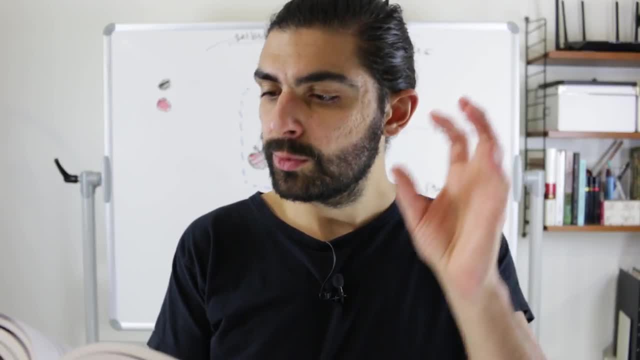 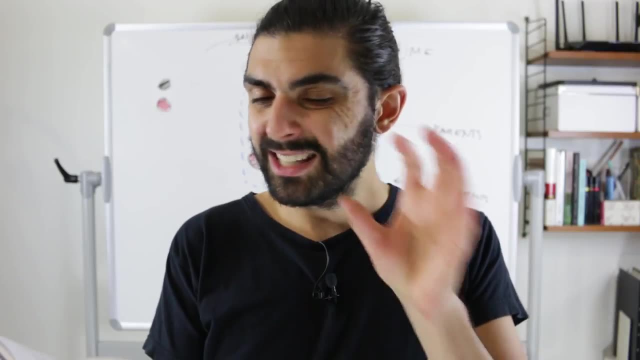 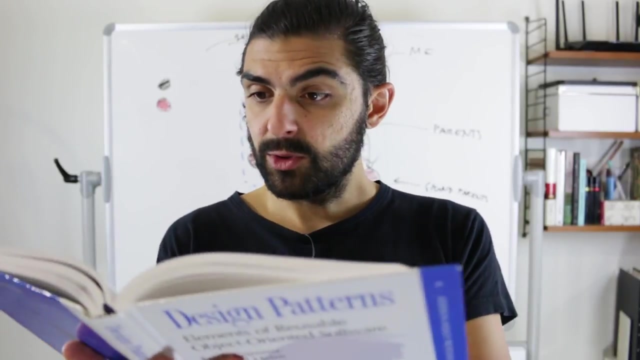 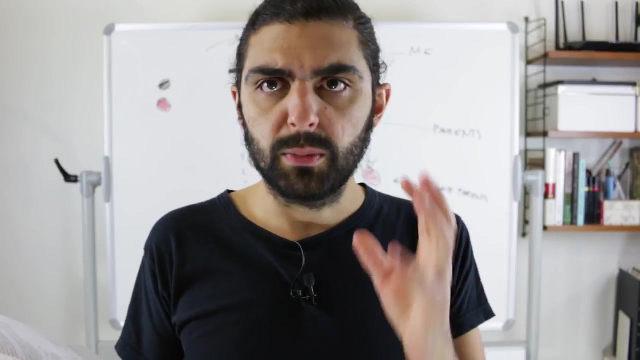 the composite pattern composes objects into tree structures to represent part-hole hierarchies. composite lets clients treat individual objects and compositions of objects uniformly, and this is kind of what we were saying, right? so composite pattern composes objects into tree structures and this is what we looked at here, right, anything that is suitable to model as 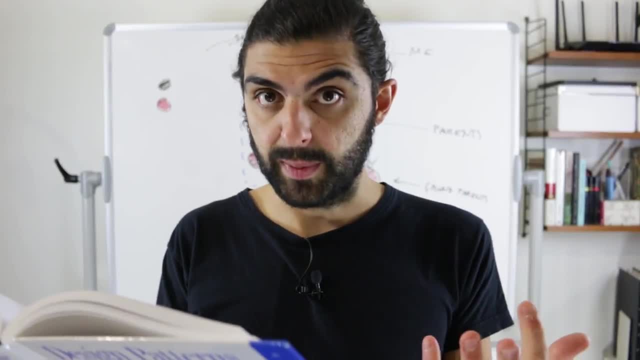 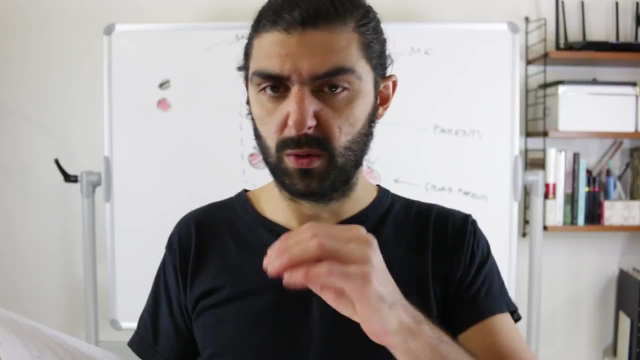 a tree structure is a potential candidate for a composite pattern, and we do this to represent part-hole hierarchies and honestly, i am super confused by this wording- part-hole- apparently. this is well, i guess, an idiom. yeah, i guess this is a common saying and maybe it's super natural. 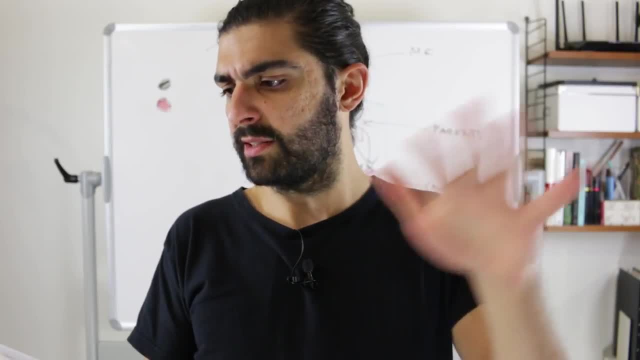 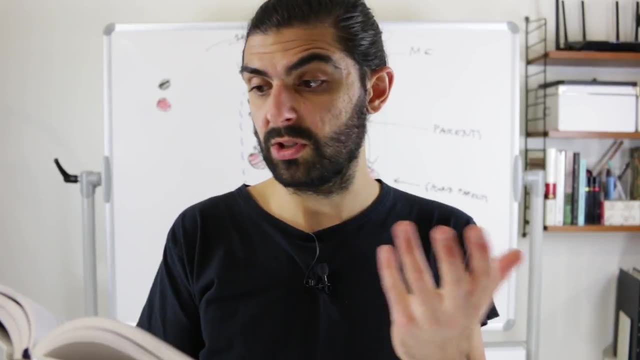 to some people, but i just find it fairly confusing. so like i just googled it and it seems the part-hole point is that any object is a part of the whole and the whole is a collection of parts, and i guess this is what they were trying to suggest by saying part-hole hierarchies. anyways, 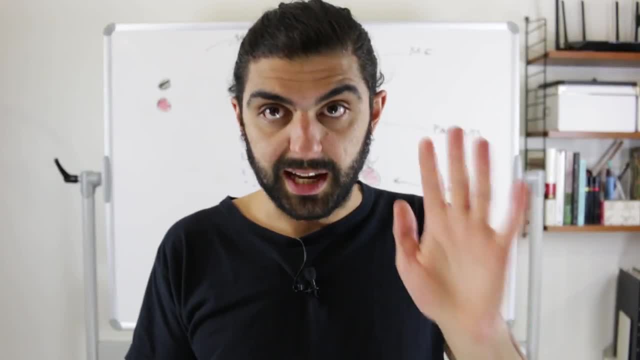 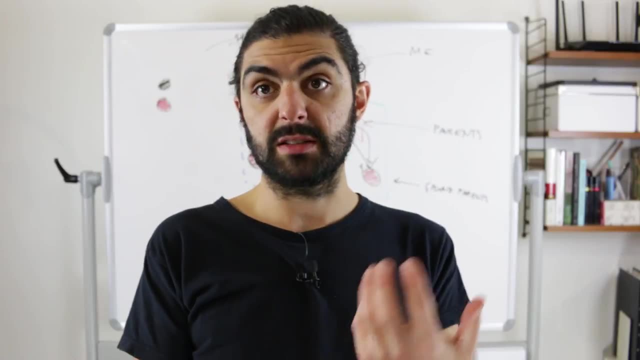 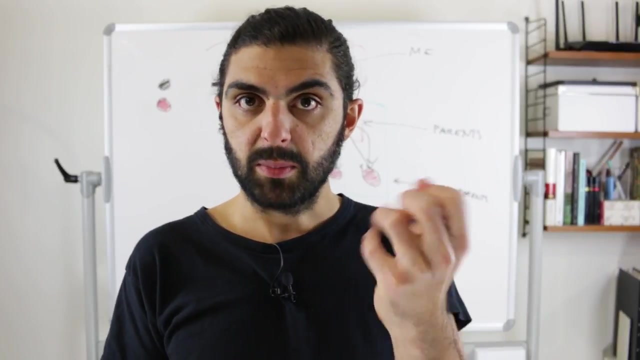 i mean, you know, you understand what a hierarchy is, anything that can be modeled hierarchically. next sentence: composite lets clients treat individual objects and compositions of objects uniformly. and this is exactly what we talked about. right like, if you think about a hierarchy, the leaves are single objects, but anything before the leaves are collections. 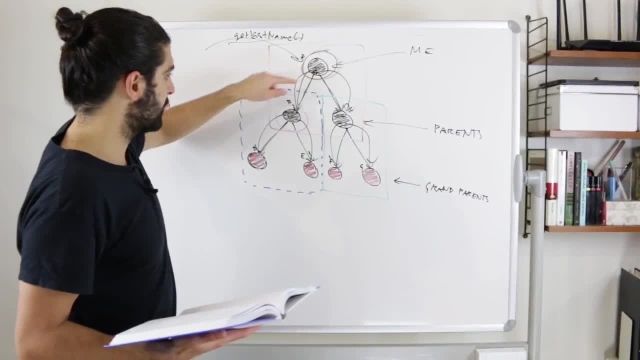 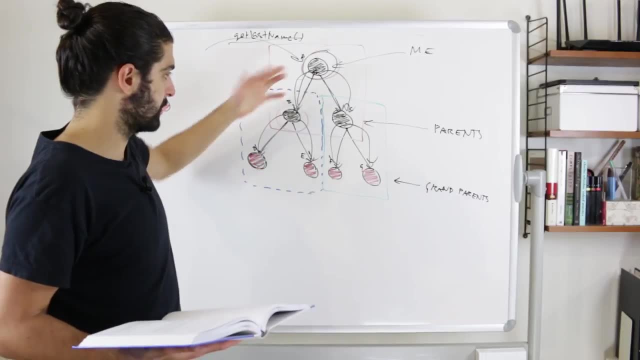 of objects and- and clearly let me just mention this before i forget it- here we looked at- uh, i guess, binary tree. right, because this node has two sub nodes and this node has two sub nodes and so forth, so all nodes have two sub nodes, but of course, with composite pattern, it could be that. 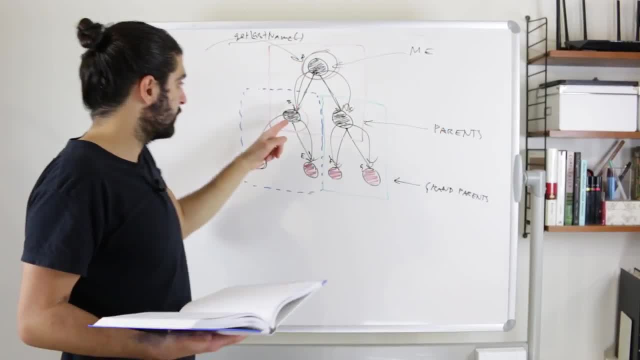 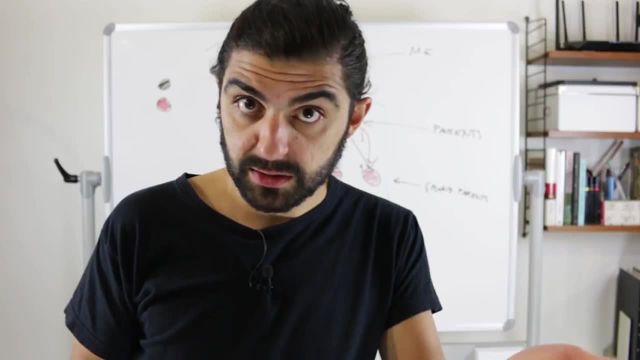 this node has 20 sub nodes right and, and one of these nodes have two sub nodes and another one has 10, and so forth. i mean two made sense in this scenario because i was modeling parents, but but the composite pattern makes no restrictions on what it means to have a. 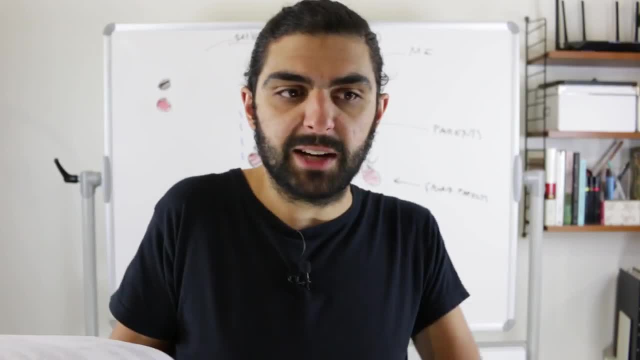 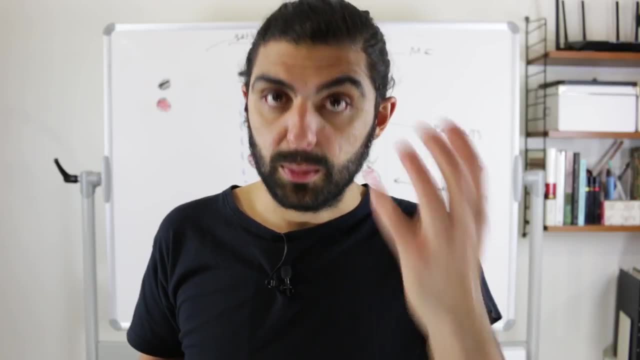 a composition of objects. if you have a composition of objects, it might mean that you have 10 or 2 or 200 objects. the point is that it's a composition of objects and it's not a single object, and you could also, of course, have a composition of a single object. i mean semantically. this is a bit. 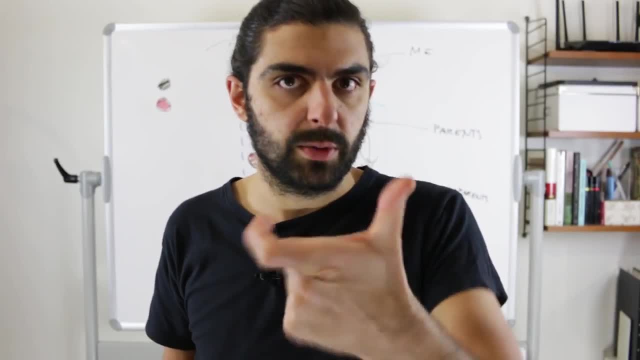 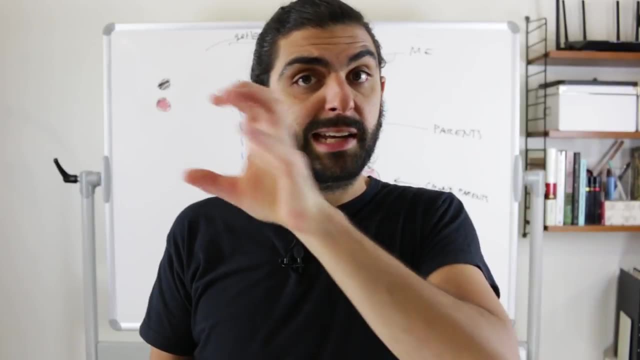 interesting. but but clearly you, since i mean just think about a list. you can have a list of one element. so i mean that's a composition with one element in it. but the point is again that collections and individual objects, compositions of objects and objects are able to be treated. 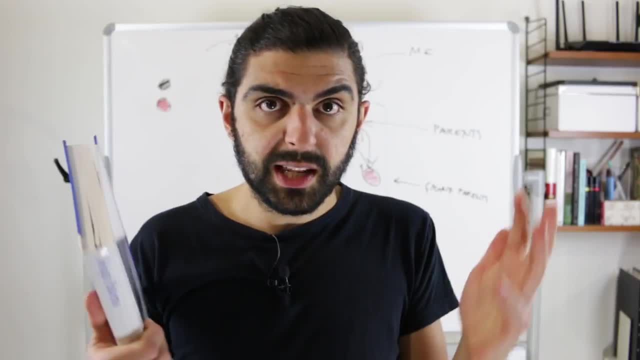 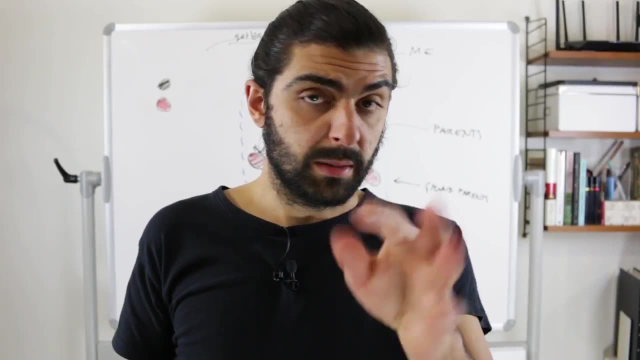 uniformly, and that's the definition. so i think on a general level this is sort of pretty straightforward and at some point, if you haven't felt this already, you will probably feel a bit angry because you maybe you're thinking: well, this sounds 100 like the decorator pattern. 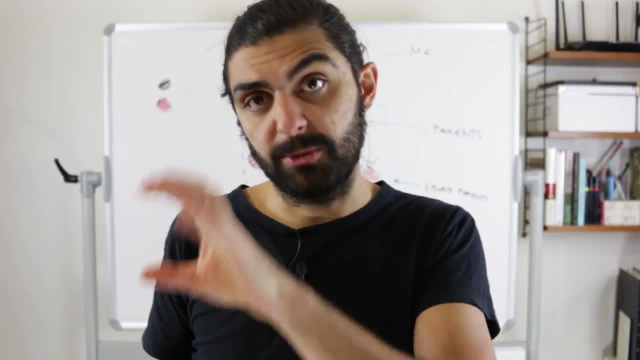 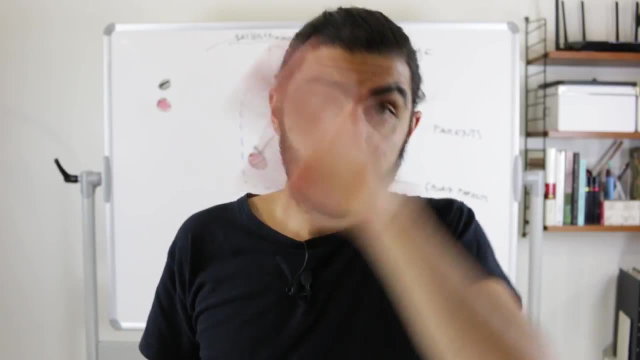 i want to touch a slight bit on why and how composite pattern is different from decorator pattern. but i will make a separate video on composite pattern versus decorator pattern, versus chain of responsibility pattern. but because i haven't made a video on the chain of responsibility pattern yet, that will be. 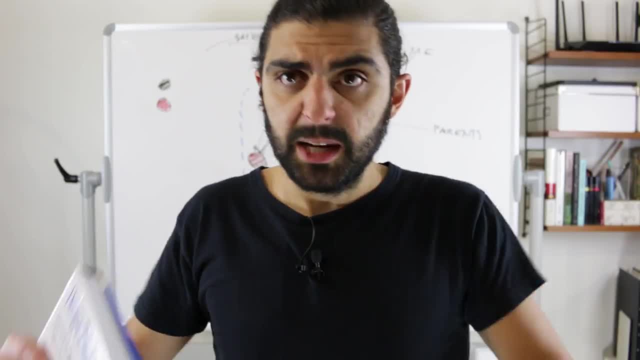 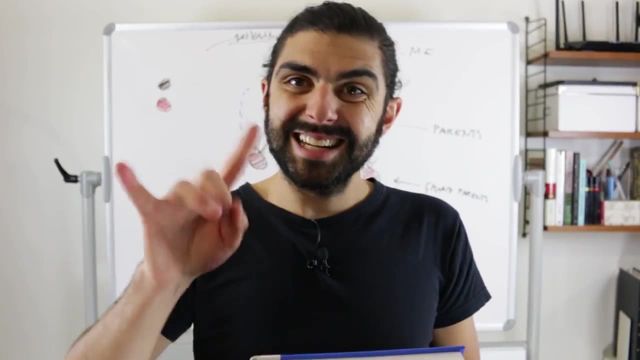 video will have to wait, but again, this is why we'll touch only briefly on it now anyways. so again, i think on a high level this is sort of straightforward, but now we need to get into the details. let's first look at the uml diagram, then let's translate that into an example which 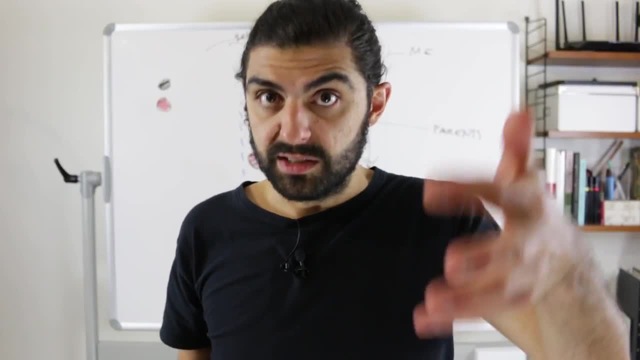 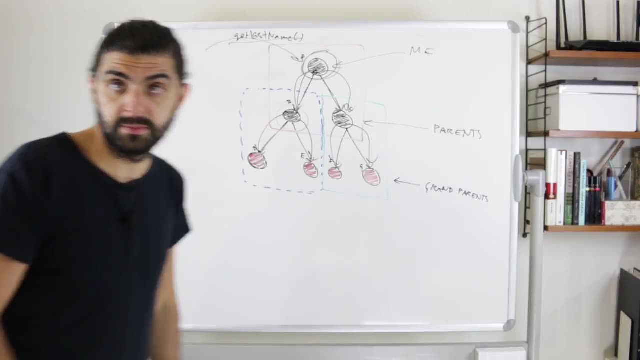 i think makes a bit more real world sense. we'll talk about a to-do list manager, if you're building an application that manages to do's. and then, finally, let's look at some code. let's get started. let me start by removing this stuff. so here's the deal. you've got something called a component and 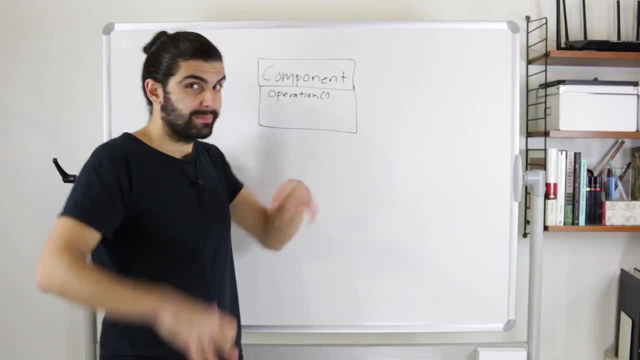 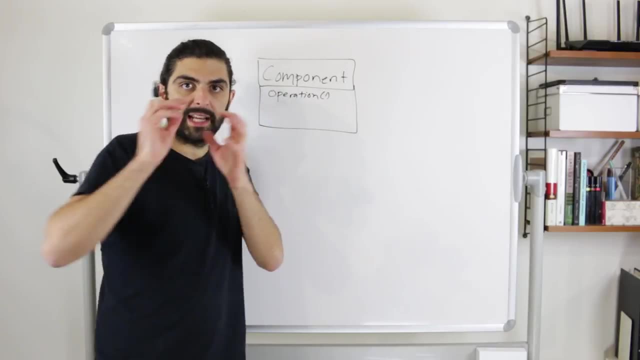 the component has some kind of operation, it has some function that does something and this is the function that you want: to be uniform across composites of objects and individual objects. so hypothetically we call this operation. i can't, i'm not specifying a return type, because i mean 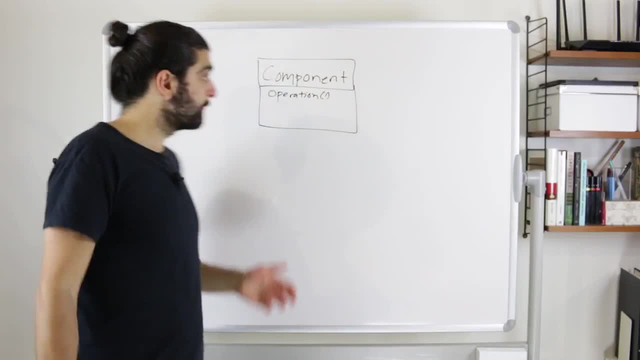 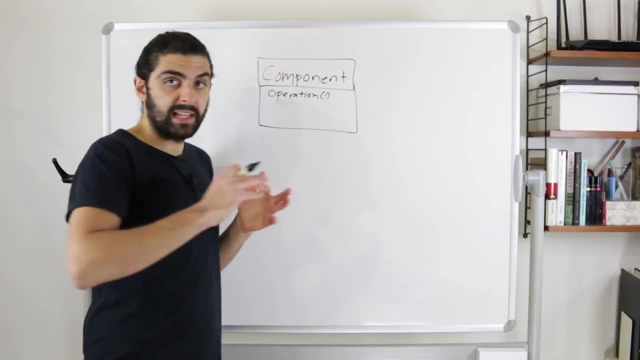 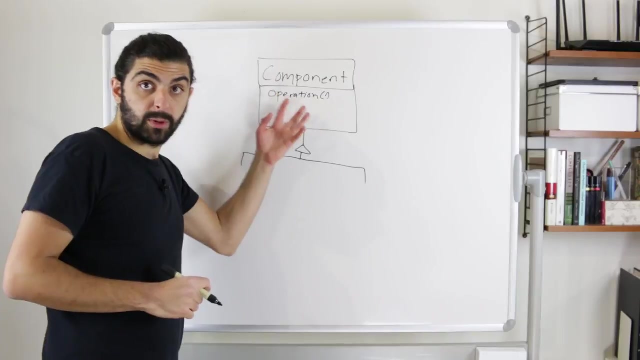 generally, we don't know what this operation does in your particular scenario. so this is the interface that we will use to refer uniformly to collections and to individual objects, which means two other classes that implement this interface or inherit from this class or abstract class, if it's a class or abstract class, but in this case i think the both two books that i mentioned model. 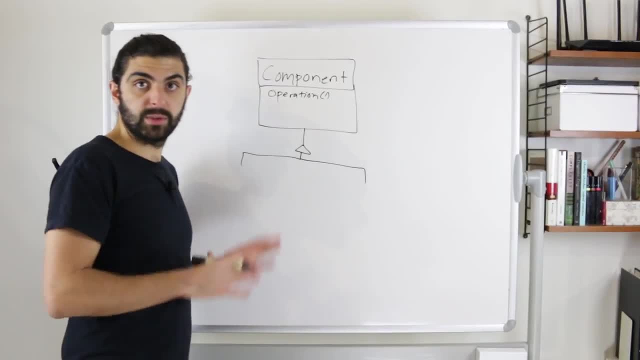 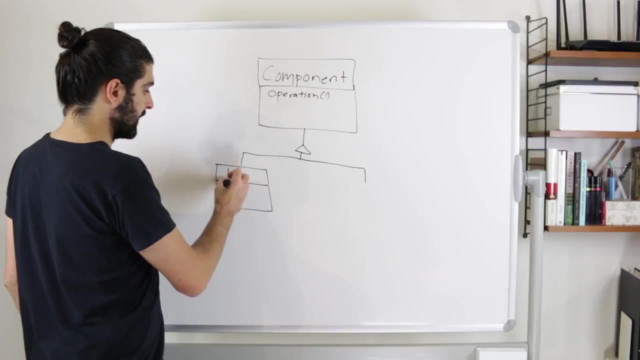 this as an abstract class, but we will model this as an interface. i will show you and tell you why in just a moment. and then these two subclasses, or rather these two classes that implement the interface we call leaf, which again is the, the single object and not the composition of objects. 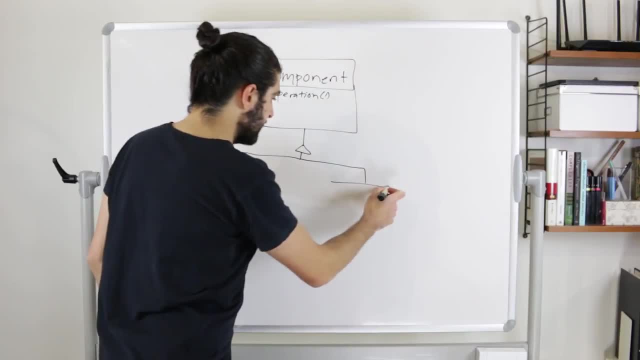 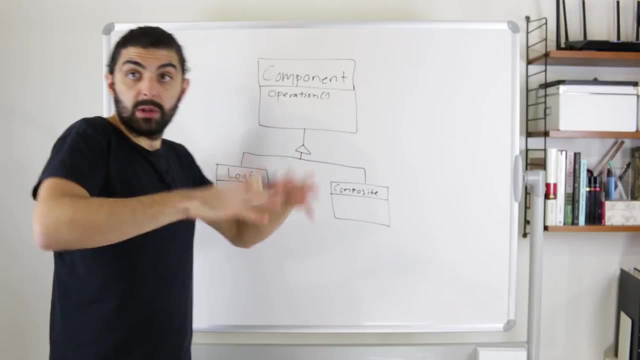 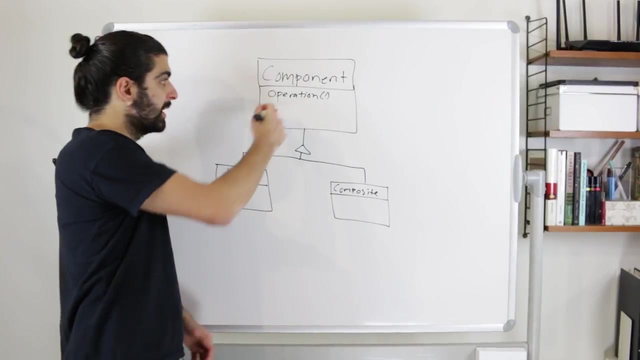 so the leaf nodes and not the branches. and then class is a composite. so just think about the terminology here. component is the all-encompassing concept. everything is a component. a leaf is a component and a composite is a component. however, the implementation of the function operation may be different in leaf than from. 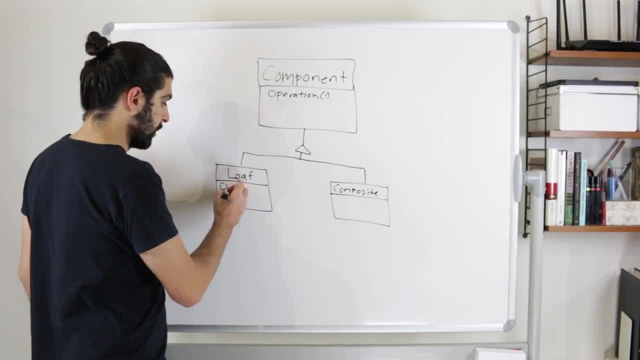 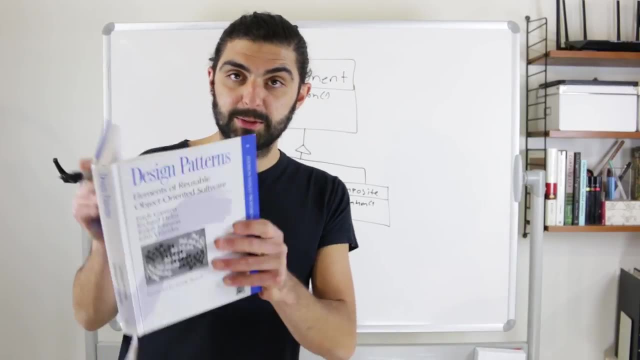 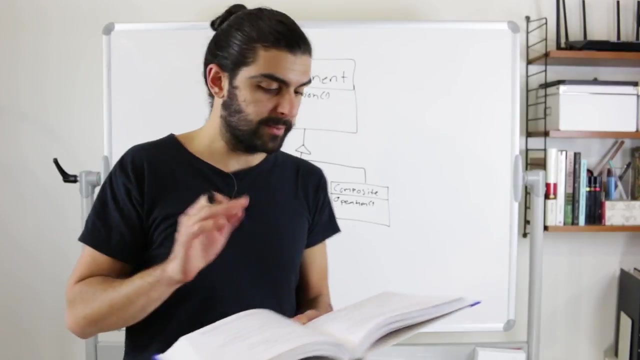 composite. so let's now specify that leaf has the operation operation and then of course the composite has the operation operation. now, usually i don't diverge from, uh, what's in these books or the common literature generally this quickly, so i apologize for doing that, but here's the thing in. 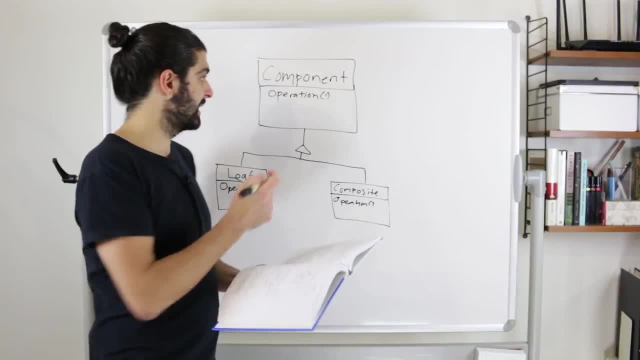 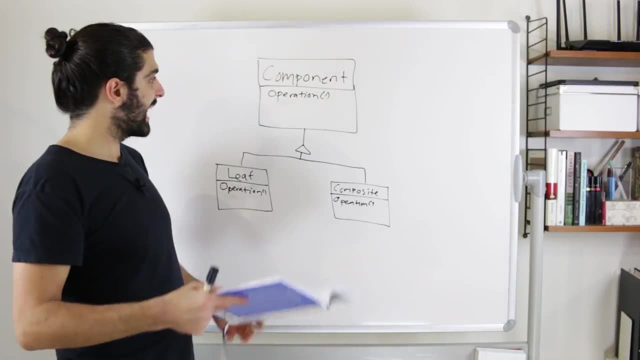 this book and also in the head first book, they add methods along these lines. they say that the component has an add method, a remove method and a get child method. so the ad method. if you think about what we're modeling, we're saying that a component is either a leaf or is a composite by 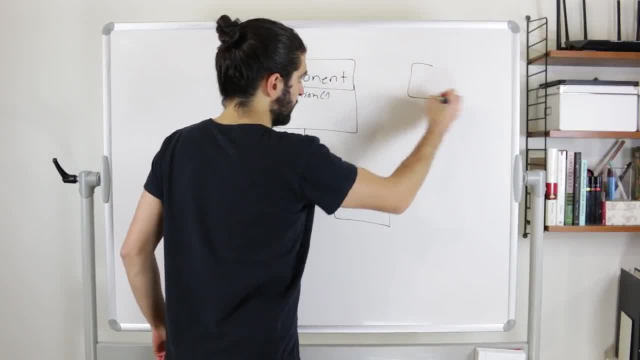 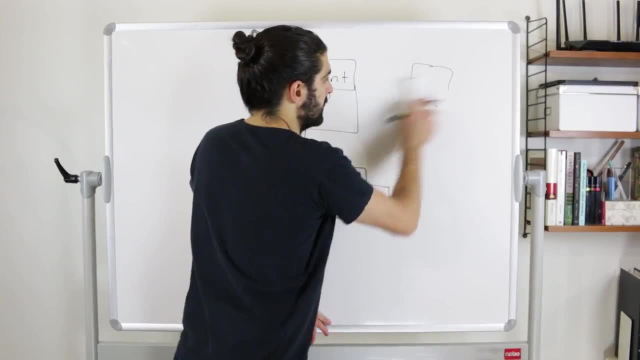 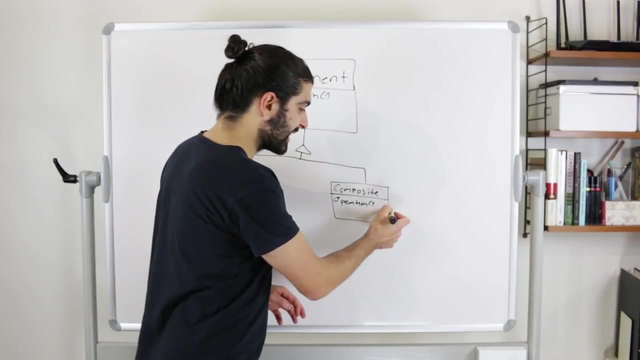 the way this notation is just because we have two things. i mean it's equivalent to to drawing to arrows. right like this is just shorthand. so a leaf is a component and a composite is a component. ah, sorry, before we go any further, i i was missing one arrow. the composite clearly has components and 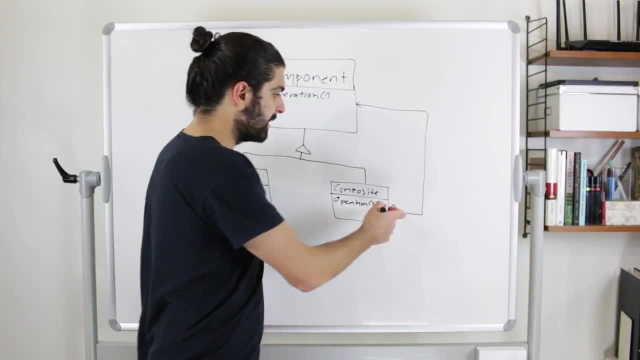 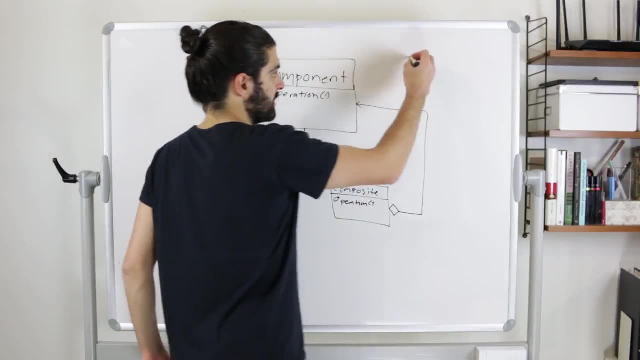 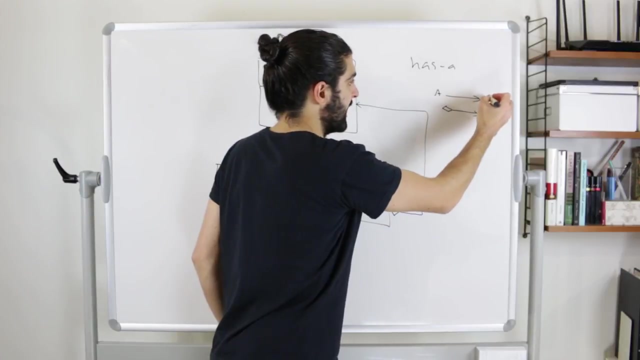 this is the recursion portion. sorry, i was going too quickly. by the way, this funky arrow in uml with like the diamond here at the start is essentially the same as association, essentially the same as has ah. so both this and this denote hazard relationships. so if we put a in one end, 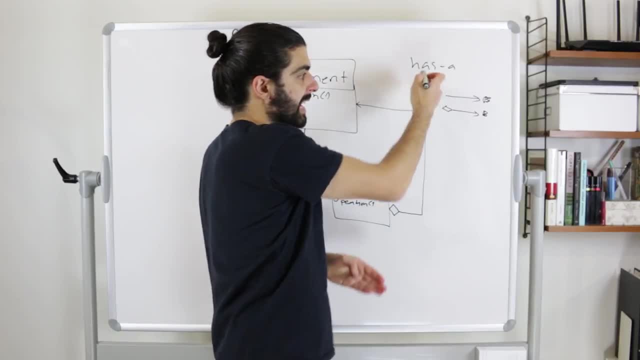 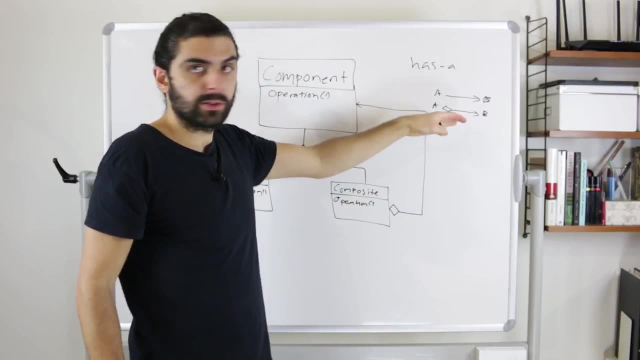 and b and the other end. so the first one is a hazard relationship where a's have b's, and the second one is also a hazard relationship where a's have b's. the first one we call association and the second one we call aggregation in uml. in all honesty, i find this a little bit vague and kind. 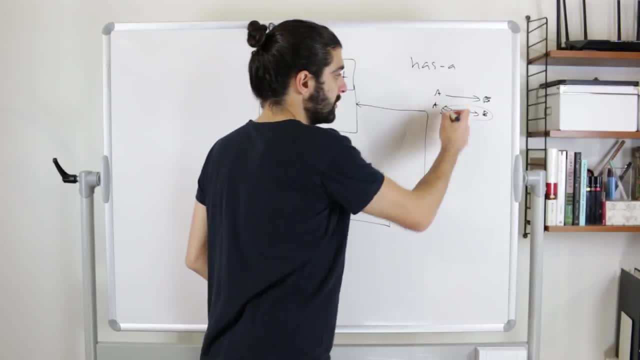 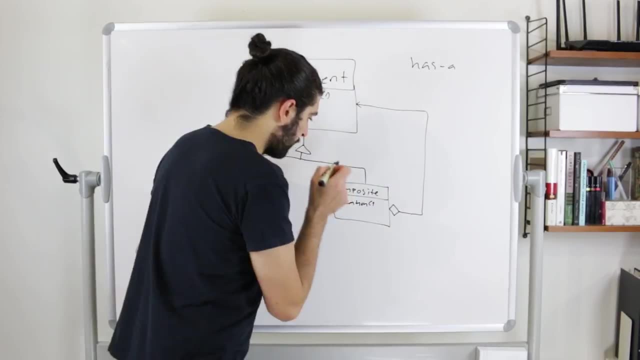 of completely unnecessary, because we don't necessarily have to use this. we could just say that it's an association and then be done with it. so because here we can specify even explicitly if we want to. i mean, a composite has a component, yes, but it can actually also have multiple components. so depending on what we're, 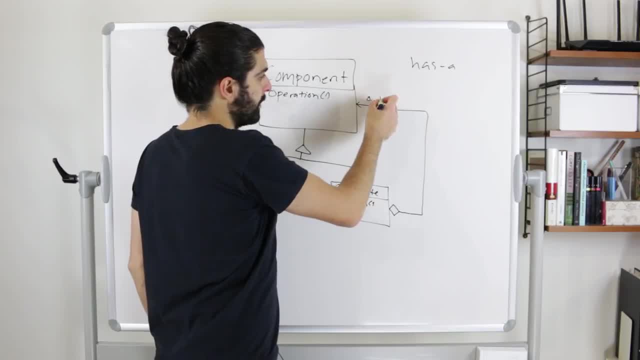 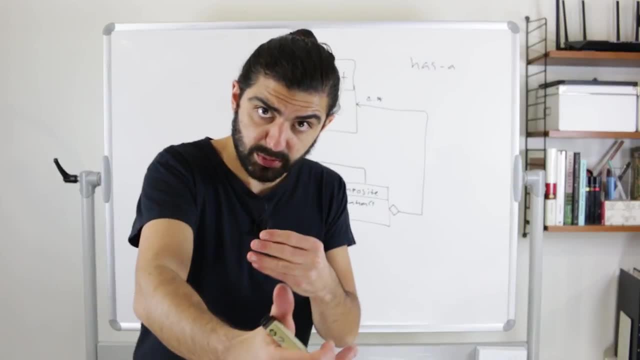 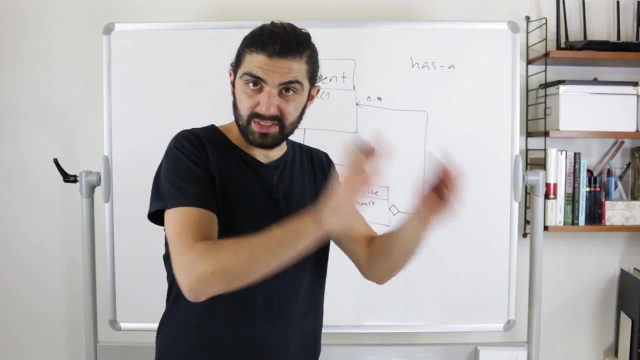 modeling. we could even say you can have zero too many components. so a composition is a composition of objects. the question is: do you mean of at least a single object, or do you mean of at least two objects? but here we're actually saying: a composite is a composition of anything from zero to many. 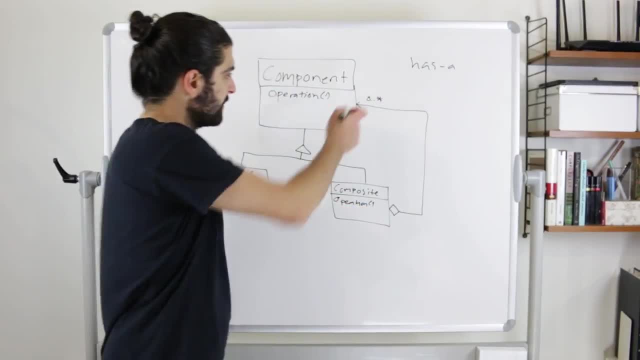 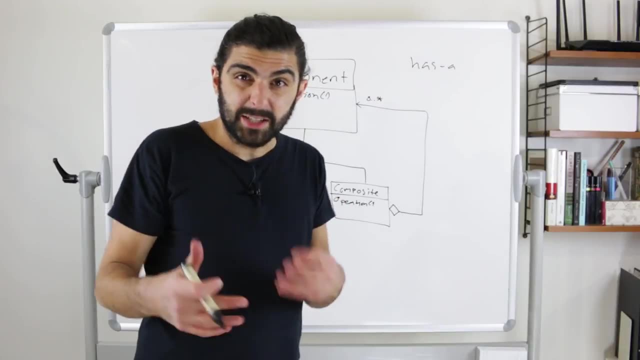 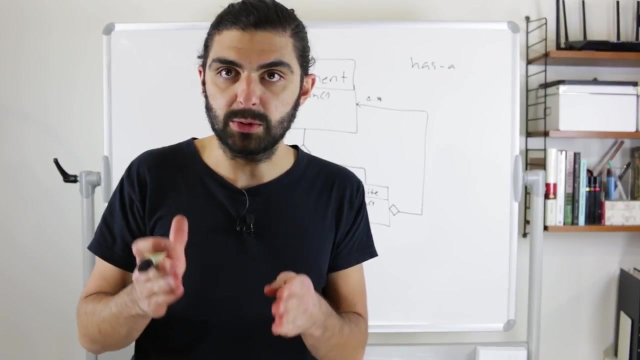 objects, which kind of maybe doesn't make a whole lot of sense, because if we say zero here, then it's essentially a leaf right. so i mean, it's a bit shady, but this kind of also shows you that, which is a super tangential point. but but it also kind of shows you how it's powerful to to write algorithms that work. 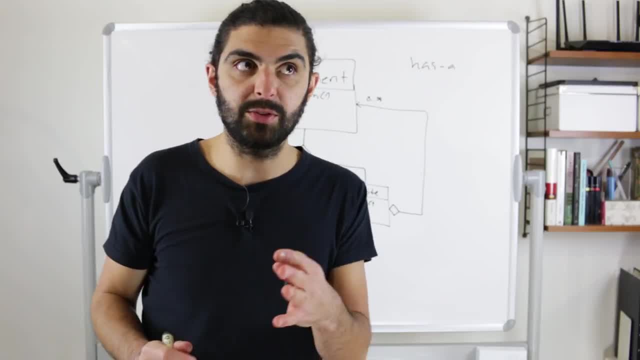 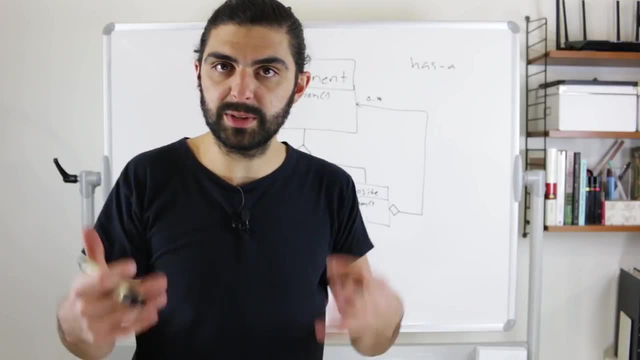 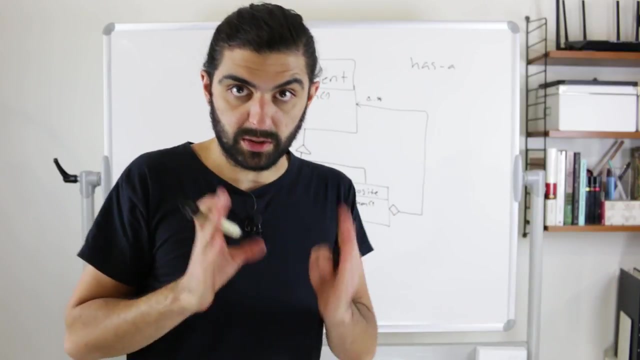 on collections of things rather than on individual things. so if you think about the library j query, for example- i guess hardly even used anymore, but they treated so when you retrieve dom elements, when you retrieved instances of things from a web page. so if you searched for something and you only had a single match, you still got the list of a single. 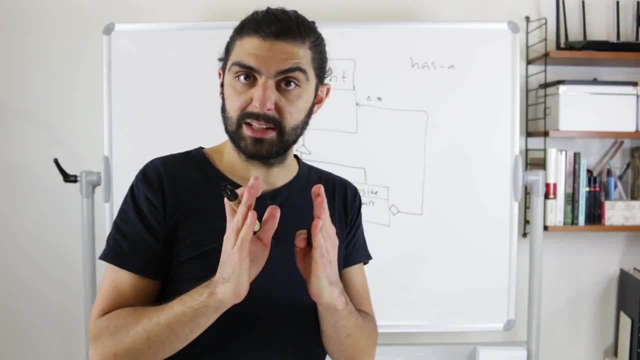 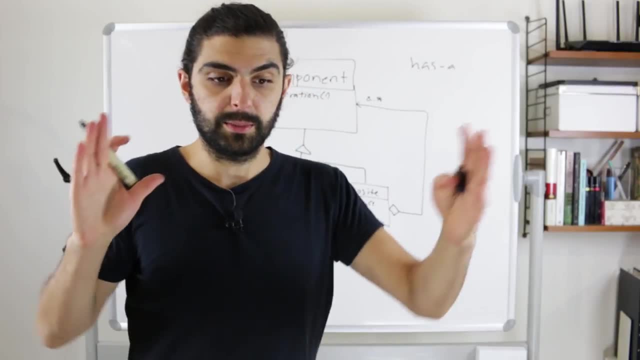 match right, and if you got no matches, you still got a list of no matches, or an empty list essentially. and if you had multiple matches, you got a list of multiple things and then you could apply your algorithm to to that list. so you always had to write the algorithm for a list of things. 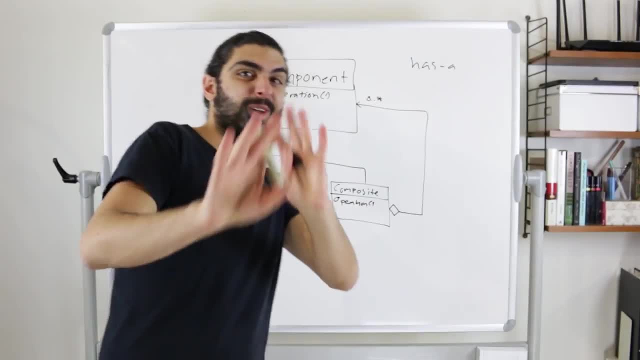 so that's very powerful, but it's also completely not related to what we're talking about. sorry about that. so back to this point. let me also remove this hasa back here. we're essentially then saying that composites can have components, so this is a more comprehensive way of looking at it. 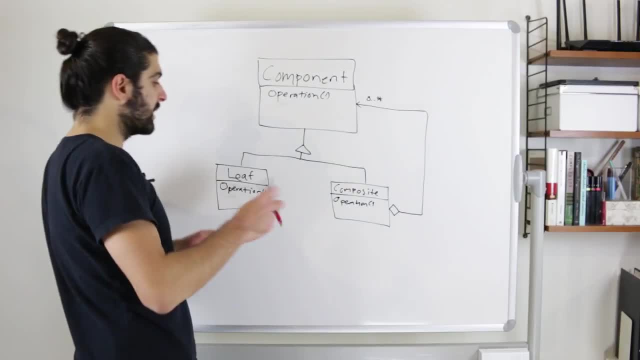 but it's also just more efficient in terms of usage. that we're talking about, because when we're talking So what are we saying? then? I mean, we are again building up the data types that we need to construct the trees that we drew before. 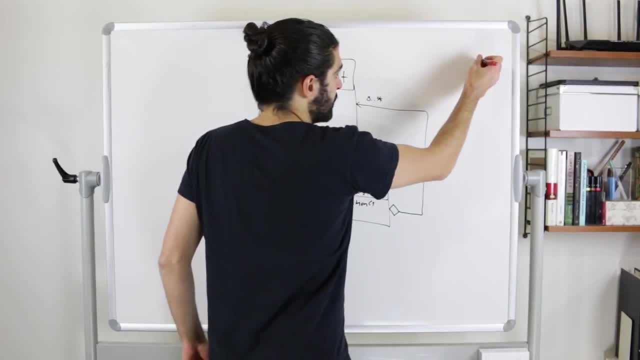 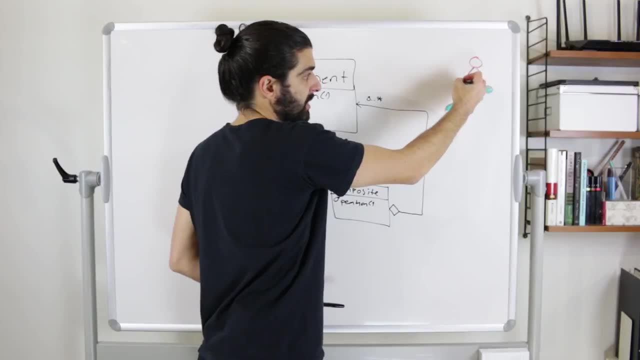 So everything is a component, right, But if we draw just a random tree like this, then this is a leaf and this is a leaf, but everything else is a composite. So this is a composite and this is a composite, but all of them are components. 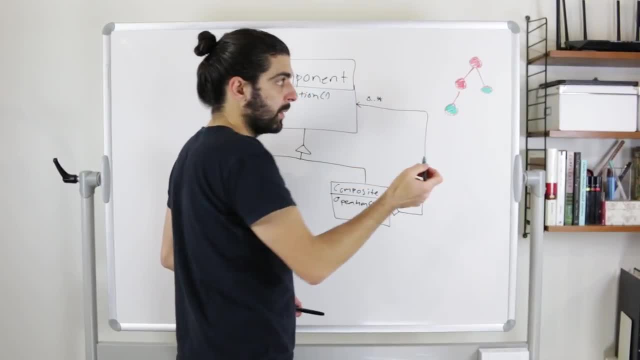 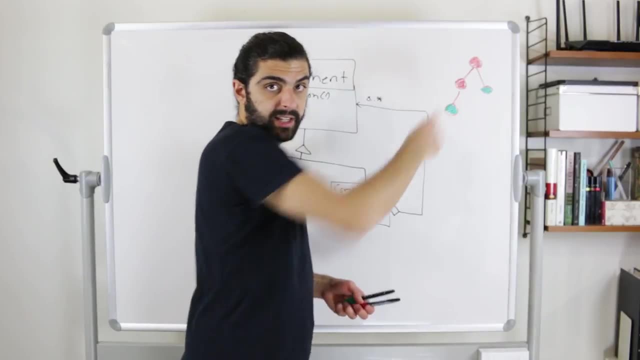 So this is a component, this is a component, this is a component and this is a component, but that's on the general level, on the abstract level. So that means that if we happen to have an instance of any of these things, 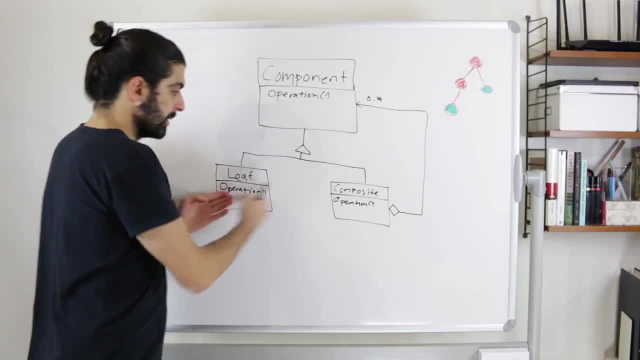 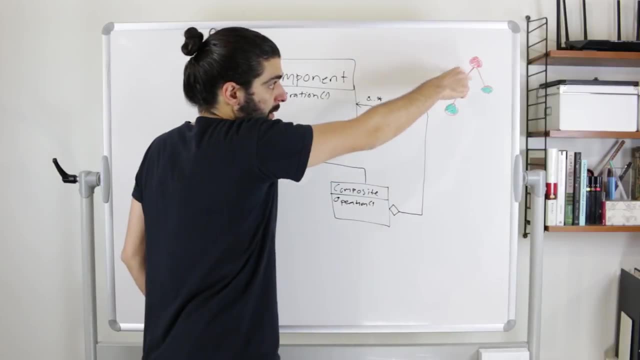 then, when we call the method operation, when we call the method with the function operation, which implementation of the operation method we will perform depends on whether we have a green or a red node here, depends on whether we have a leaf or a composite. 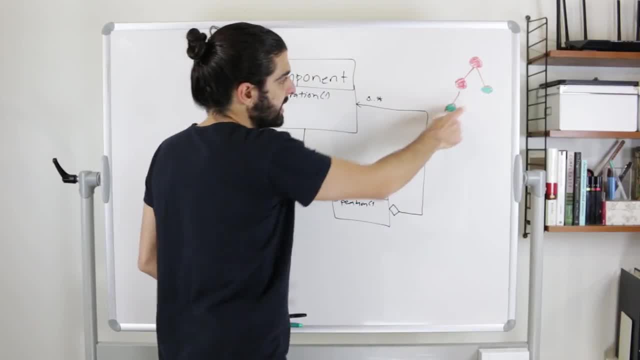 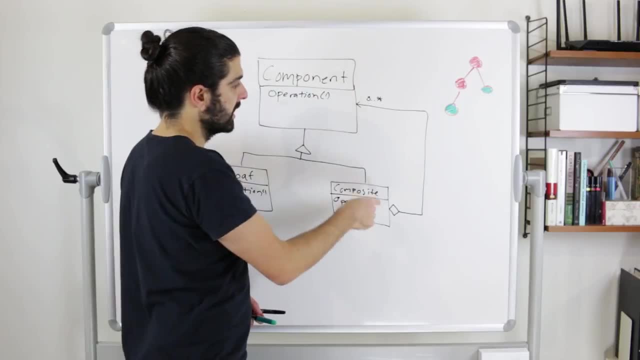 Polymorphism, right. So actually I mean, in this case I said that these are necessarily. these two green ones are necessarily leaves. They aren't necessarily leaves if we had modeled it so that composites could have zero components. So let me just change that to at least one right. 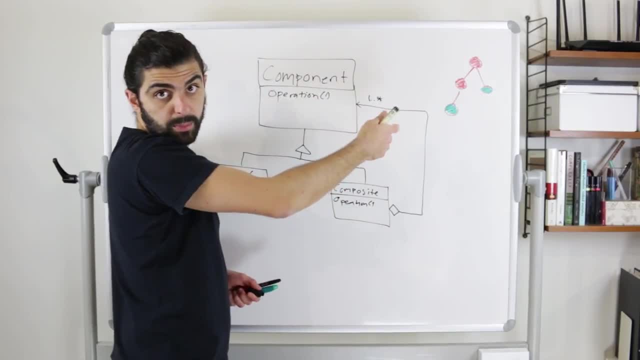 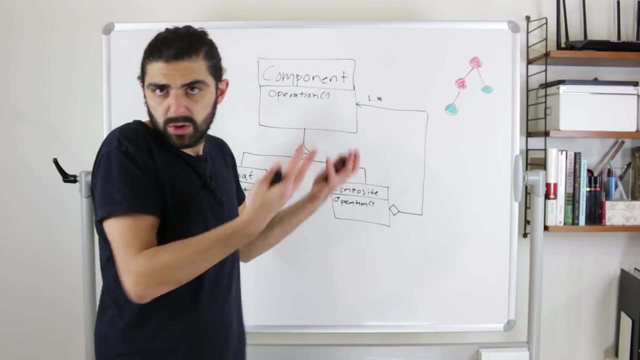 So composites have at least one component, but can I have multiple components? Because I mean otherwise it doesn't really make any sense. Let me also say that we're not going to enforce that in code here in these examples, but you could if you would want to. 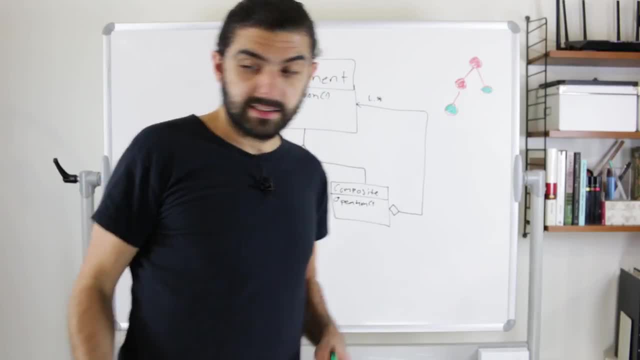 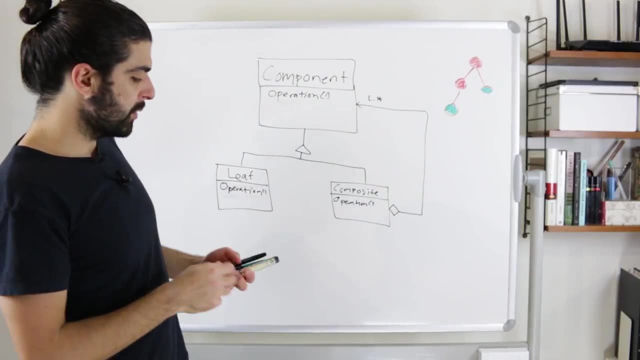 Anyways, back to the point that I raised in regards to this book. I said that they also want to add an add method and a remove method, The point with that being that let's say that in your program you have a reference to this object. 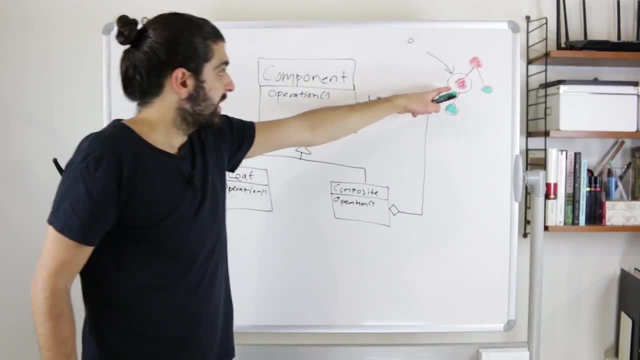 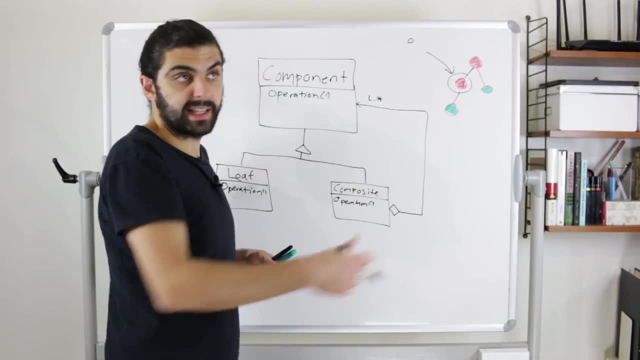 Let's call this O, right, Like in your program, you have a reference to O And this is of type composite. Yes, it is a component, but we can see here that it has a sub component, It has a child component, which is this component. 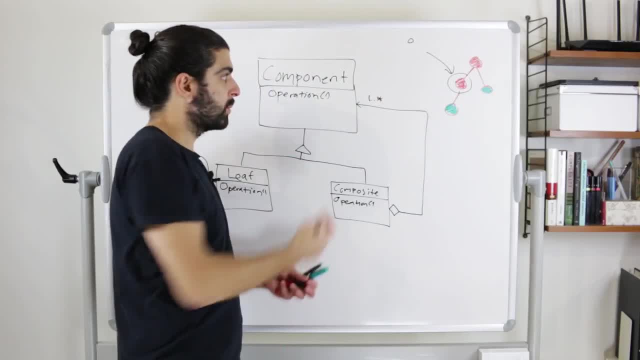 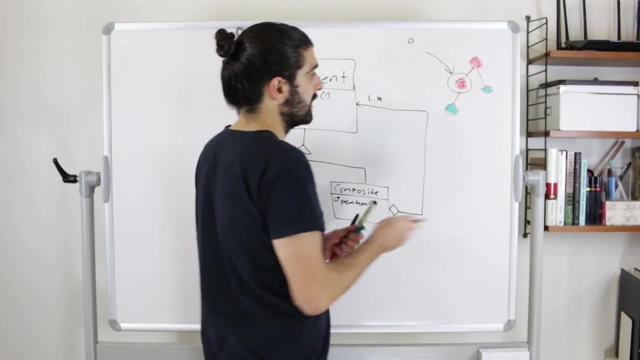 And because it is a composite. the idea is then that, well, we could extend this tree. If it's a composite, then it happens to have one leaf at the current time. Well, I mean, in the future, we could add another leaf, just add another one. 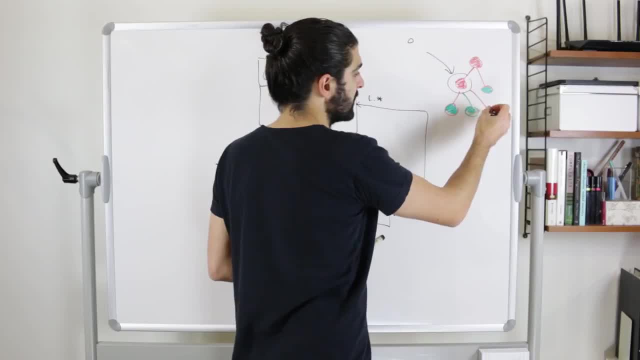 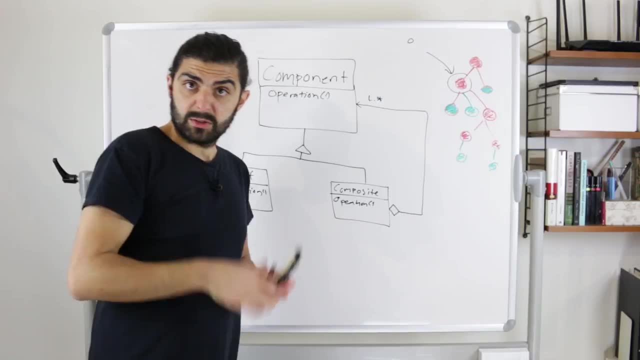 And actually I mean, we could of course add another composite that in turn will have another composite and another composite that in turn maybe have leaves. So the point is that as long as you have a composite in your hierarchy, you could hypothetically 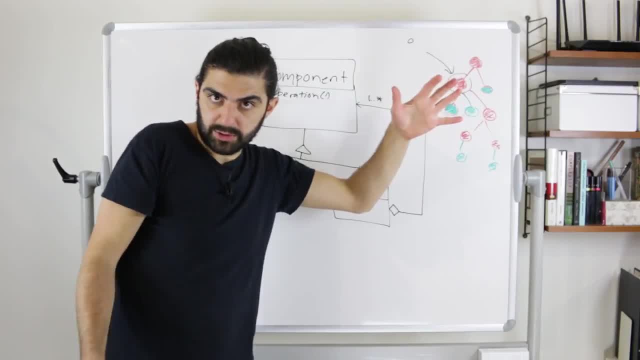 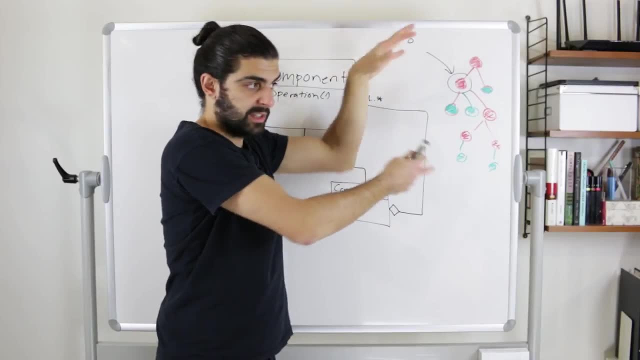 keep adding further composites or leaves and build out the tree structure, And the reason, then, that they add the add and remove methods is that they want to allow you to mutate, to change this tree, to change this tree, to change this tree. 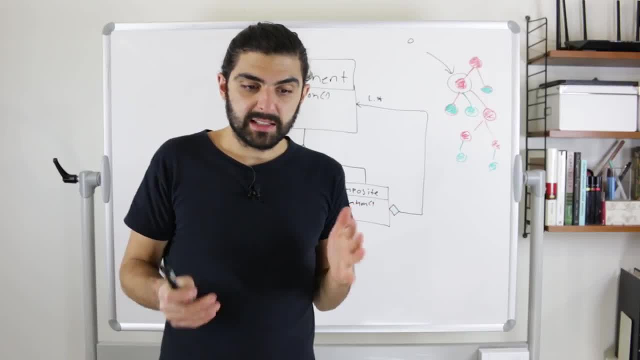 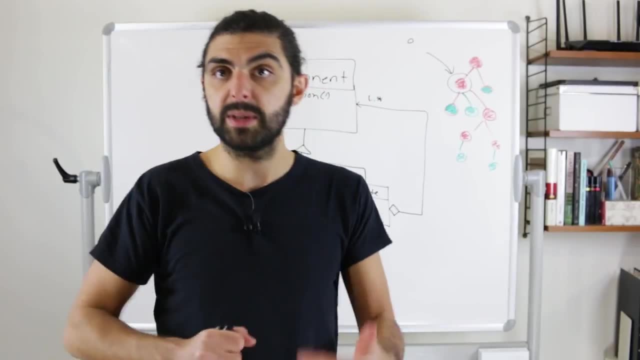 as you have it in memory. The reason I'm not bringing that up here is that I think this is a sensible time to talk about mutation. So be aware that this is kind of subjective and opinionated, But as far as I understand, it seems that we're sort of collectively agreeing. 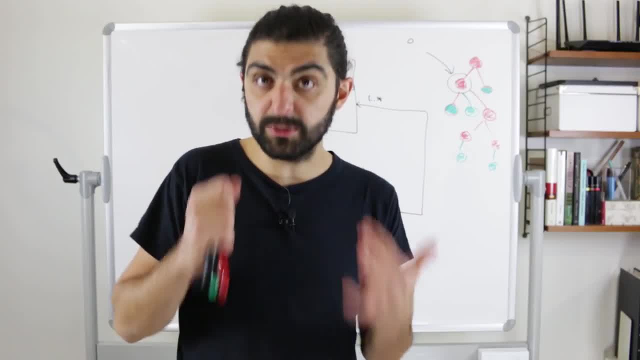 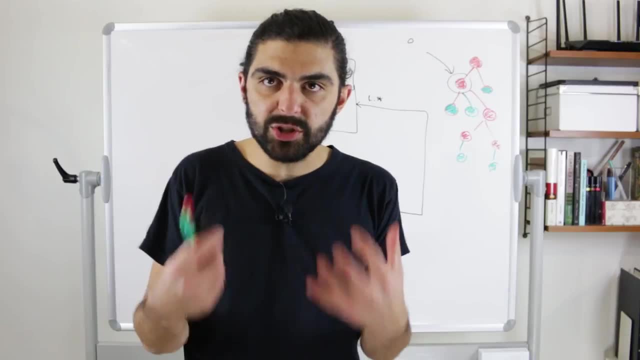 that mutation should whenever possible be avoided, And mutation means to change. We won't dig into that in super detail, but just think about it this way: Can you change the contents of something without making it a new thing? So if you have a string, 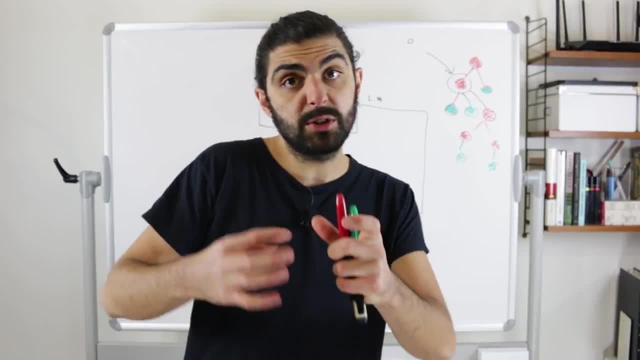 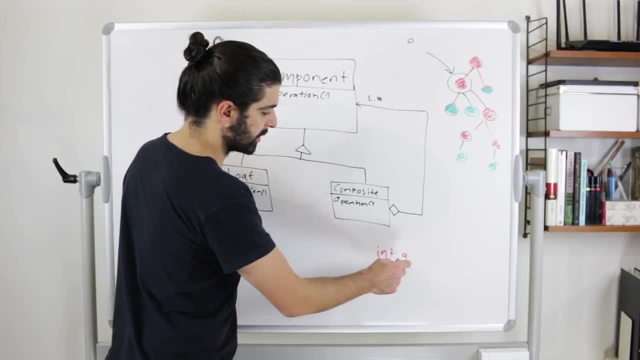 and you alter that string, does that create a new string or does it actually alter the original string? So if you have- or let me put it this way, If you have, an integer called a and you put five into it and then you say a++. 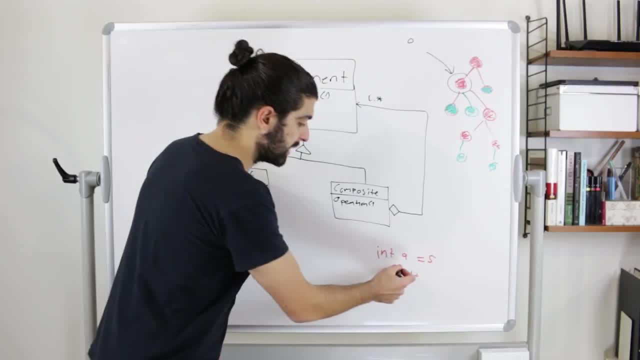 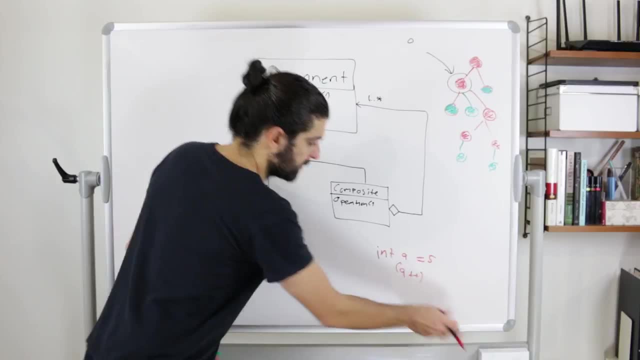 does that mean that a now is six, Or does that mean that you've created the number six here but you haven't assigned it to anything, so it just disappears, The difference being? let me show you What if we do this. If you add int. a equals a. 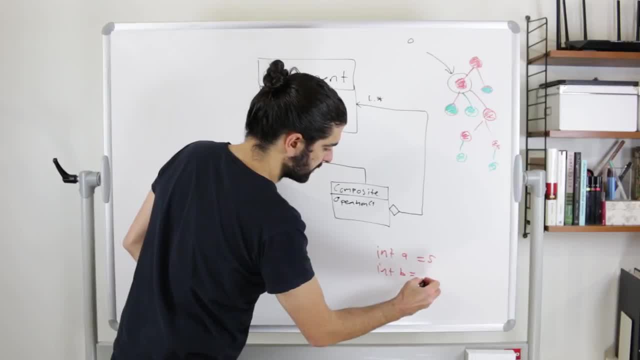 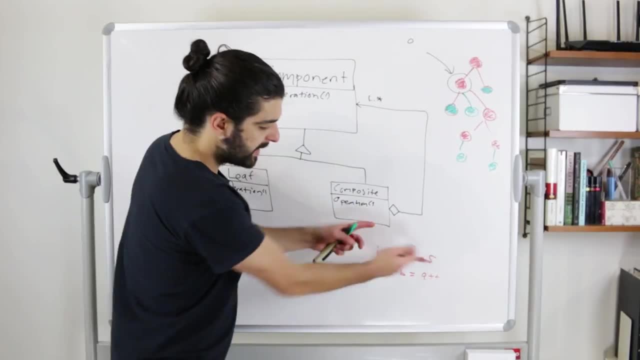 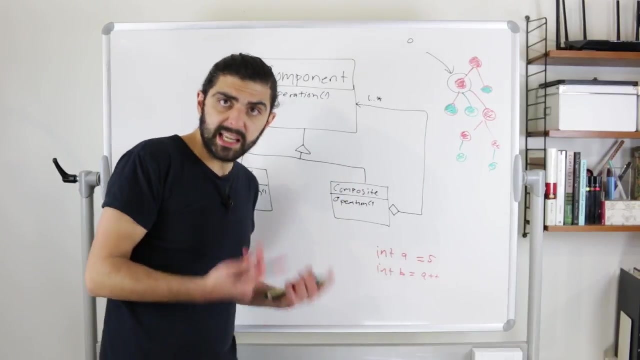 equals five, and then you have int b equals a plus plus. i mean, i'm using making use of the plus plus notation because plus plus presumably then mutates the value. so in the second case now, b should definitely be equal to six, but the question is whether a is equal to six, because if a is equal, 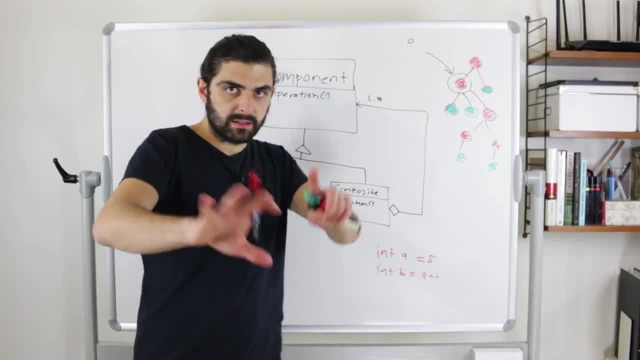 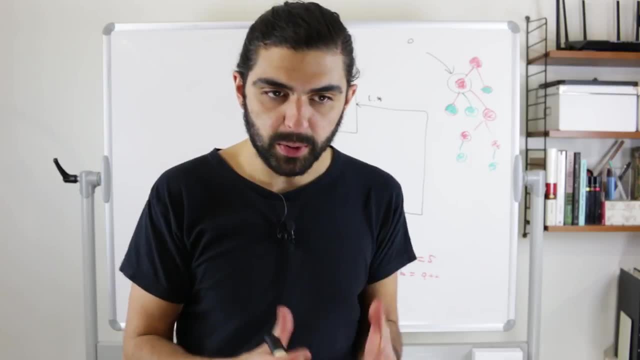 to six, you've suddenly changed the value of something, and again i- i don't want to dig down into this, but i mean without making it complicated. the point is, if i have a data structure, is it possible to change the data structure? or if i want to change the data structure, do i have to? 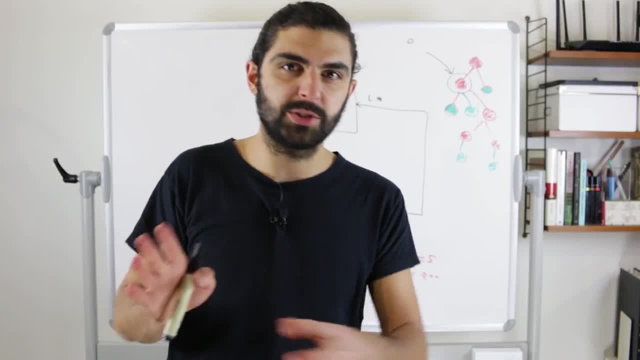 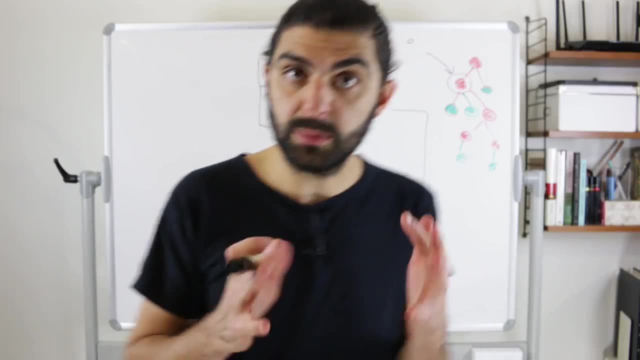 create a new data structure that is similar to the old data structure but now, but has the new change. and again, i think we're sort of collectively agreeing that whenever possible, we should use immutability, we should avoid mutation, we should avoid allowing things to change, and this is one. 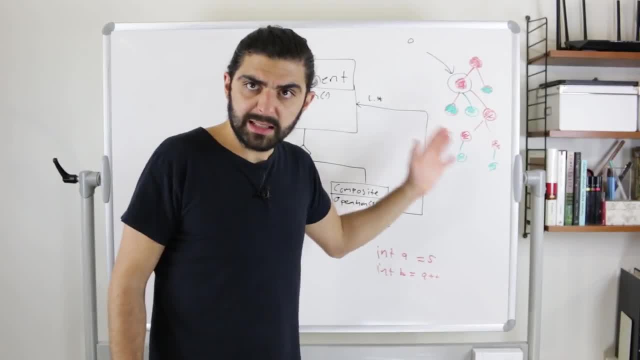 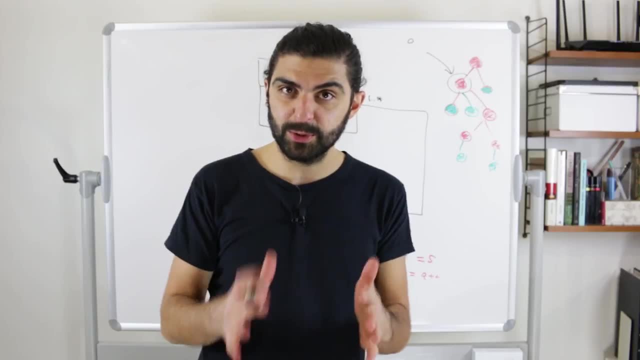 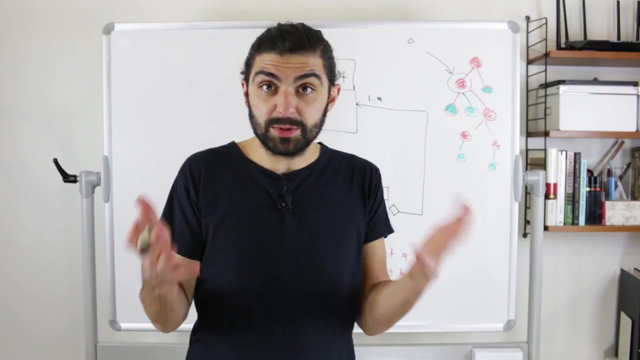 these scenarios, right like building hierarchies. i think it's completely unnecessary to build hierarchies that are mutable, unless, of course, i mean, you could argue that it's very, very suitable for your scenario. but even then i would guess that it's a pragmatic solution. i mean, i would assume that there are immutable solutions for almost. 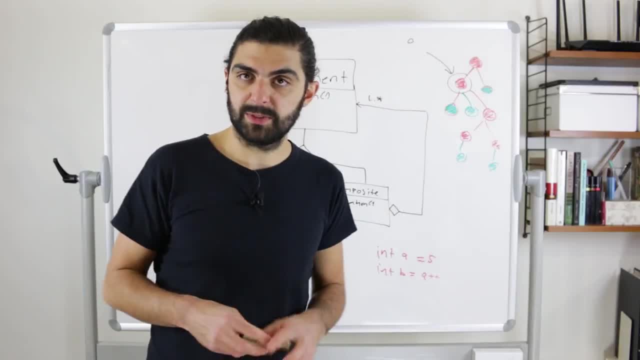 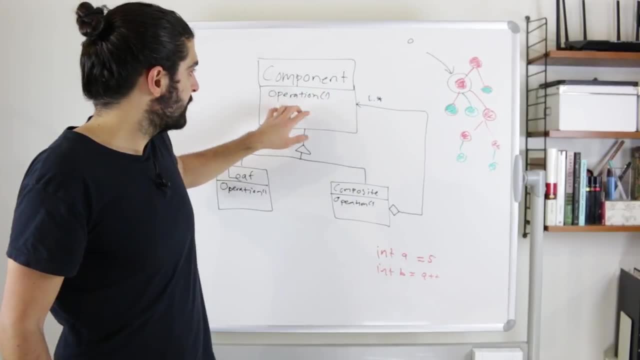 every mutable solution. so i don't really know if, like some specific scenarios really require it, unless, of course, mutation is an inherent part of the requirement of the application. but anyways, so this is sort of the reason that i'm skipping the add and the remove methods. but now you know. 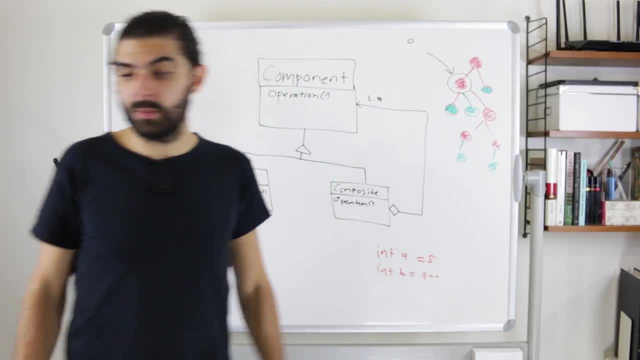 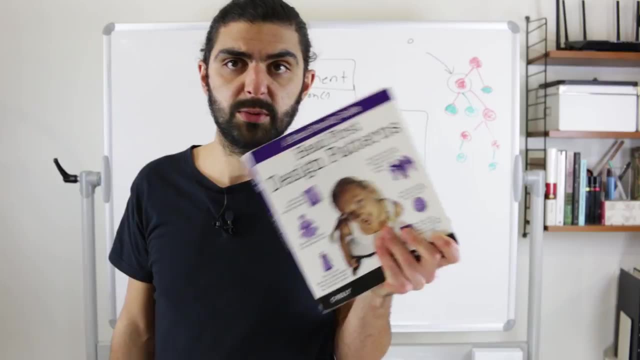 kind of what the intent of those were, and if you want to know more about that, you can check out these books for some information. if you have the headfirst book, i'd caution you that for this particular chapter i don't think they're nuancing this discussion enough, so maybe read that with a grain of salt if you have the gang of four. 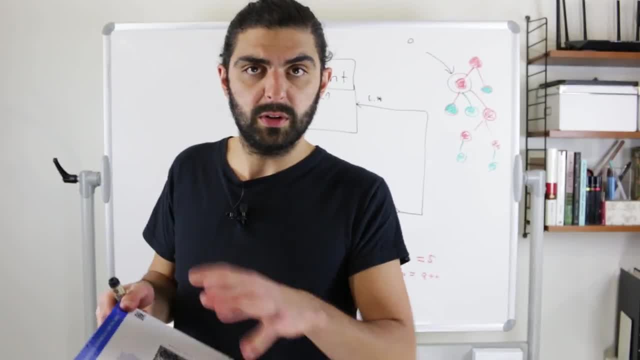 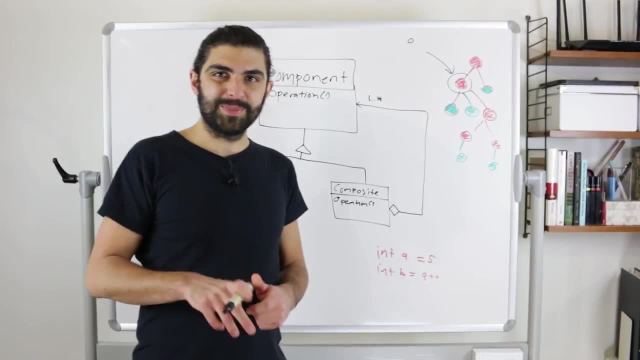 design patterns book. i think they do a little bit of a better job of nuancing that discussion, but again, i think there's there's more that could be said. let me make this super explicit why it's also kind of becomes a problem because when they add the method add here and the method remove, 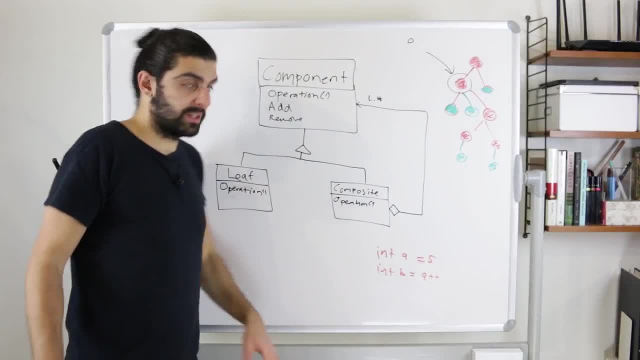 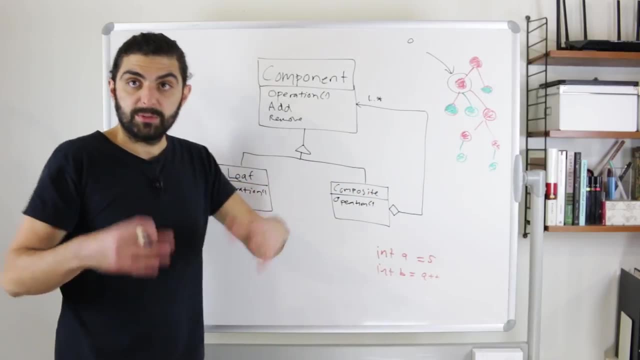 they add it to the base class and then they focus their discussion around whether these two methods should be in the component, or whether they should be in the component or whether they should be in the composite, because if they are in the composite, suddenly we've lost this transparency. 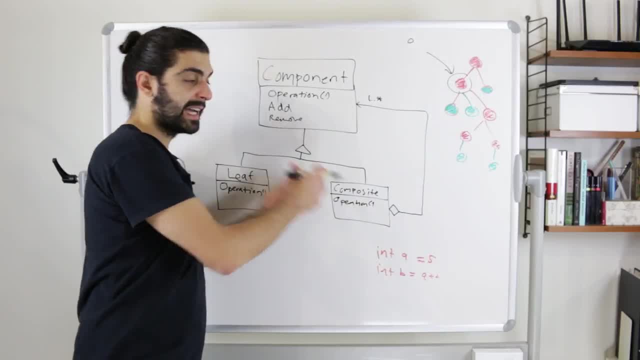 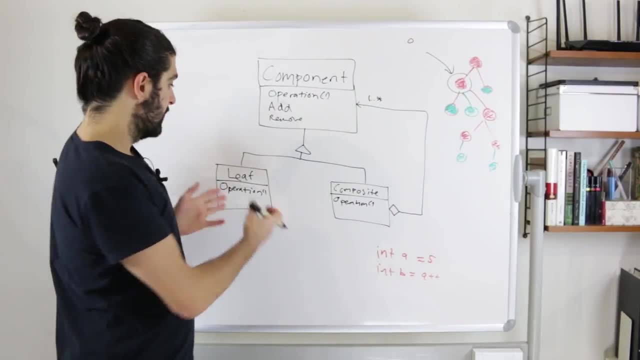 we've lost this uniformity where leaves can be treated exactly as composites, because then we can't just pick out any node when we're traversing this tree and say: add on it, because if it's a leaf it doesn't have the add method. we can't make the program compile if we're in a compiled language. 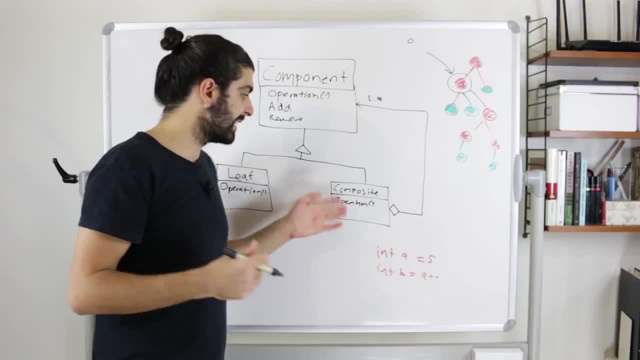 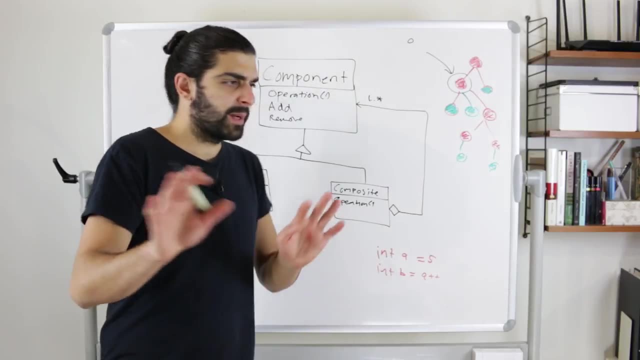 so then we would have to typecast them and we would introspect, we would check the type and see if it's a composite, typecast it to a composite and then call the method add or remove, because then we know that it's it exists. if you've seen my other videos on typecasting, you know that i'm just fundamentally opposed to. 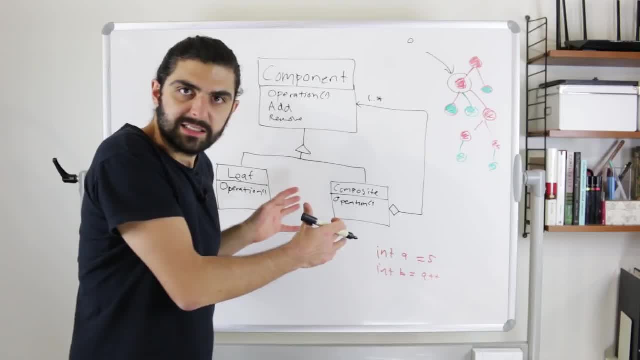 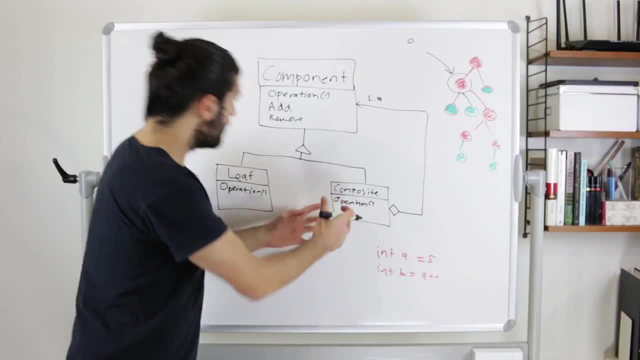 it so. so that's not even an option, at least for something like this. i mean, if you have some esoteric scenario, for sure, but but this seems too trivial to have to force us into a position of typecasting. so the other alternative is to put add and remove here in the component. 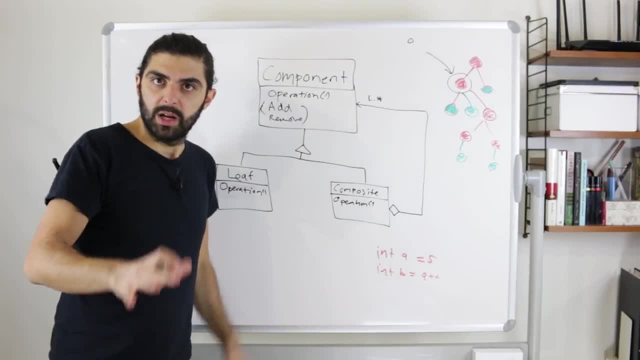 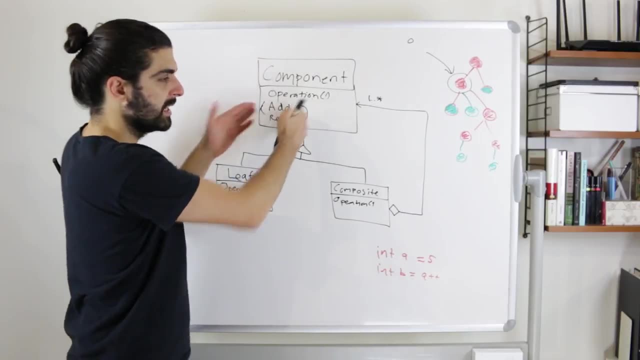 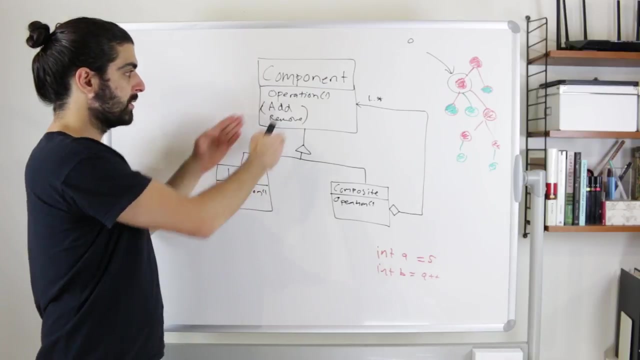 but the problem with that is the interface segregation principle, which states that clients, implementers of an interface, should not be forced to depend on methods that they do not use. literally, literally. this is what the interface segregation principle states: clients should not be forced to depend on methods that they do not use. and that's exact, 100, 100, exactly what happens. 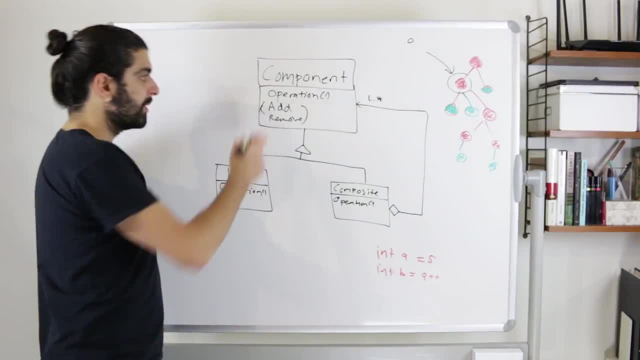 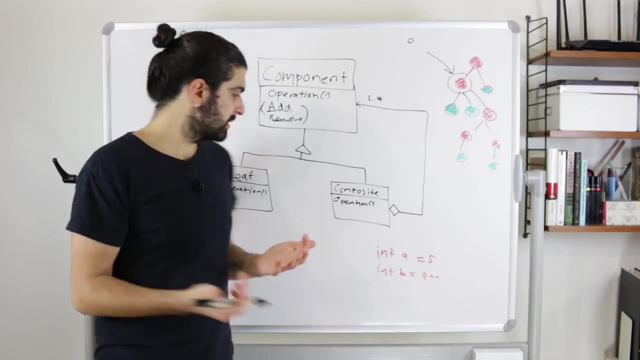 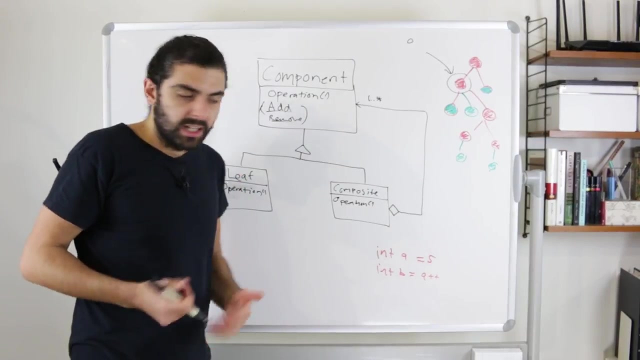 here we are saying leaves need to have the methods add and remove because we want to be able to treat them as components. but it fundamentally makes no sense for a leaf to have an add and remove method unless a leaf can actually add and actually remove. so they go through all these things and they're 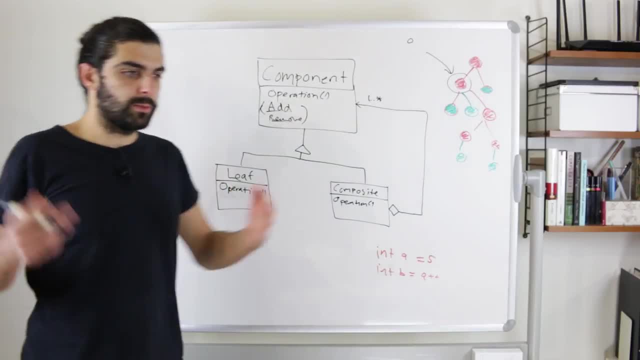 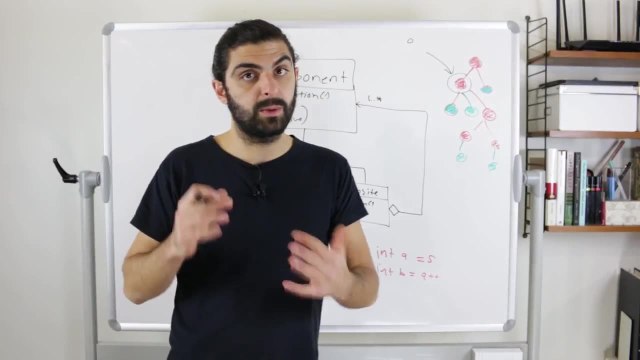 all these hoops of like, okay, should we throw an exception here, or should we return null, or should we silently do nothing? and i mean, okay, these are all semantics. so it might be that you're in a case where one of these cases is valid, might be right, and then that's super fine, then it's not actually. 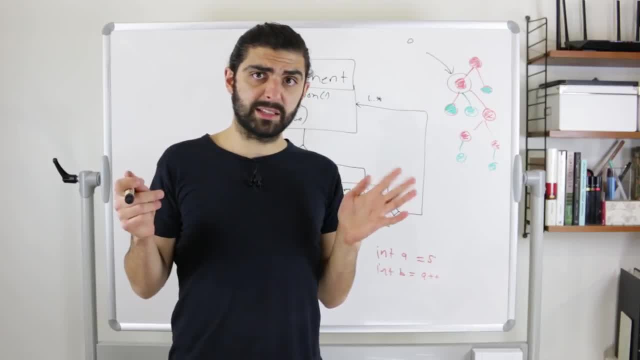 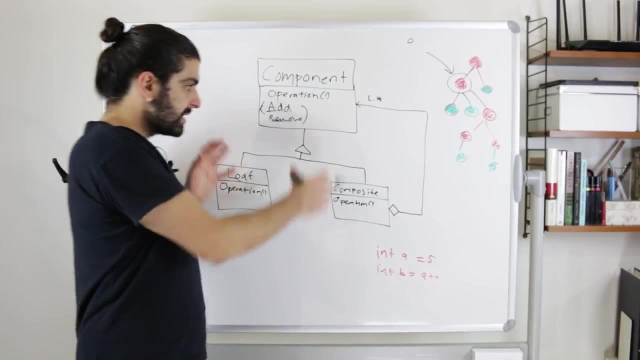 a violation of the interface segregation principle. remember that all of these things are semantic. right like it's difficult to say whether something is objectively incorrect. you have to argue for your particular case, but this just seems to me like we would never find a solution for a good. 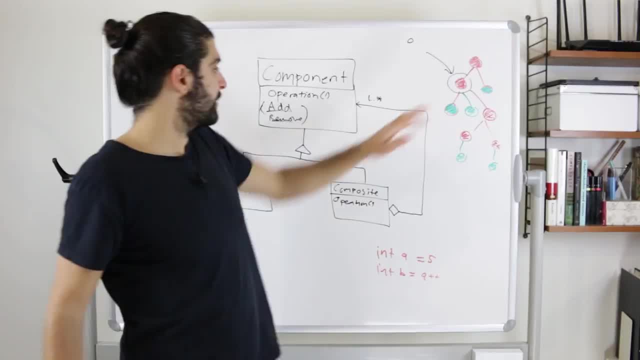 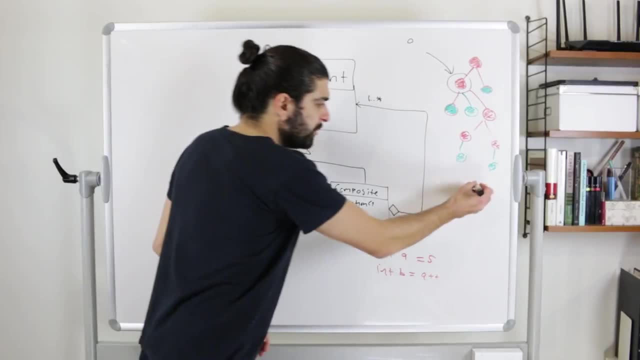 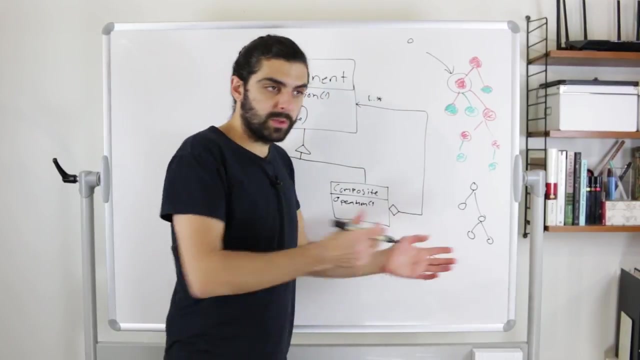 if we would look at immutability, what we could do is that, if we said that these hierarchies that we're building up using the composite pattern are immutable, meaning whenever you've built a hierarchy, you cannot change this hierarchy. you've built it, that's it. what you can do is you can create a new. 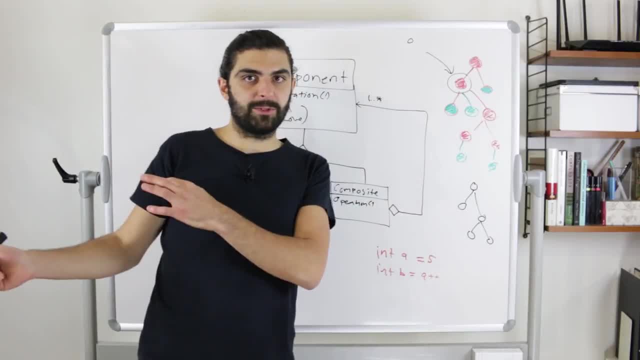 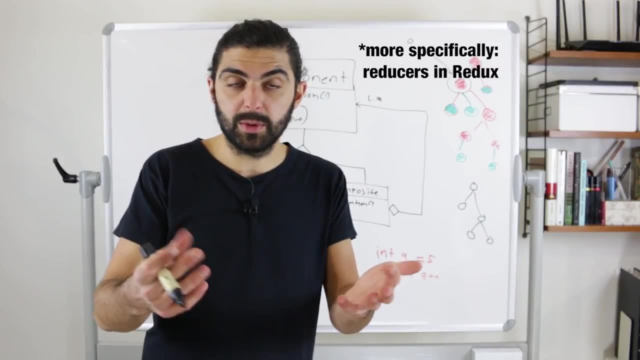 hierarchy that looks like the old hierarchy but it's slightly different, and that's the way of changing it. and this is i mean if you are, if you are familiar with javascript frameworks like react, for example, that's kind of the way it works. but if you are familiar with the javascript, 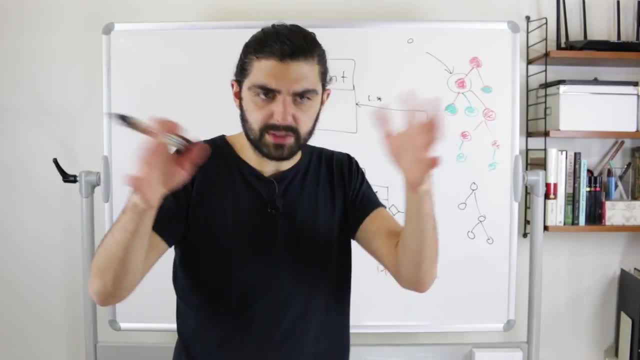 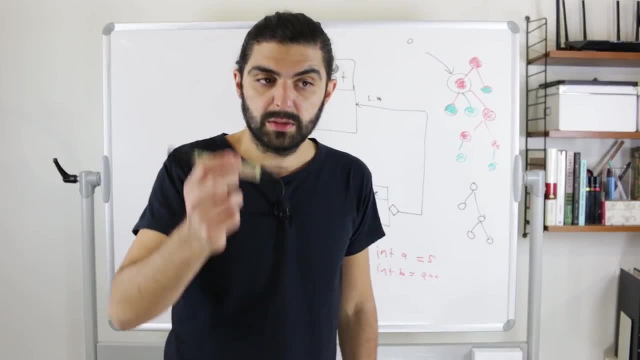 way that works. So I'm saying that also to emphasize that this is not sort of some esoteric academic idea. It actually like it's highly useful And again, that I maybe wasn't clear about before, but because programs with a high level of mutability are difficult to reason about. 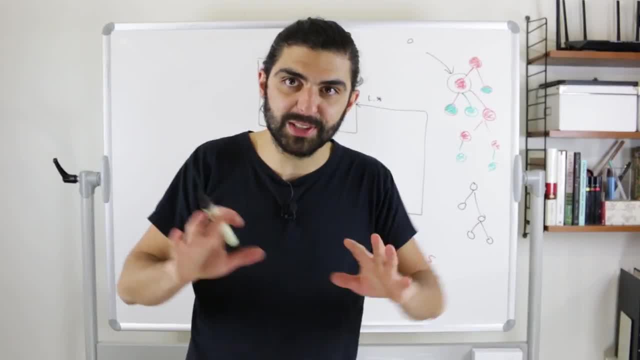 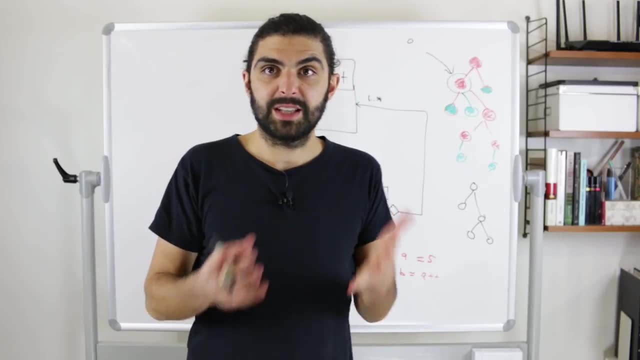 So when things start to change underneath you, and especially if you're doing asynchronous programming, it's very difficult to reason about what state things currently are in. But if you can make the assumption that things always are in the state that they were when they were originally, 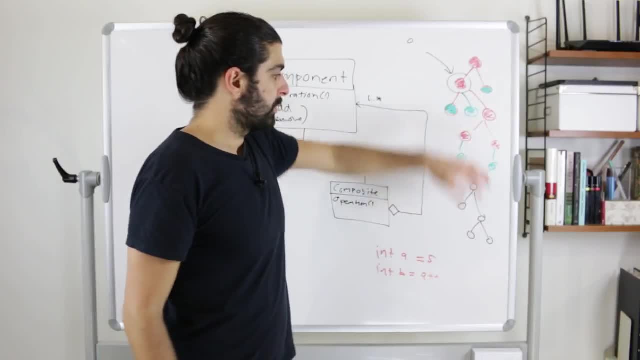 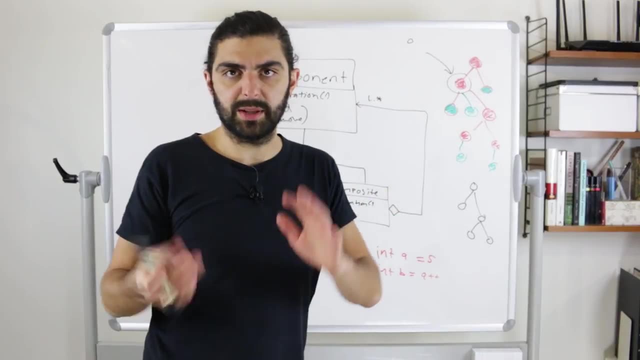 instantiated. it's much easier to reason about And, again, it's not super difficult to implement things such as copying the whole tree and then making that particular change. We won't talk about that now, but do ping if you want to talk about that. Maybe we can talk about that in a 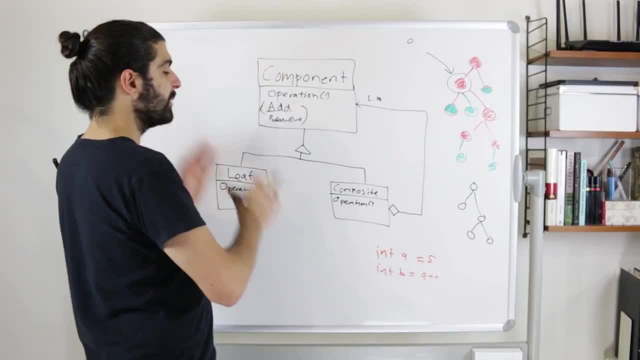 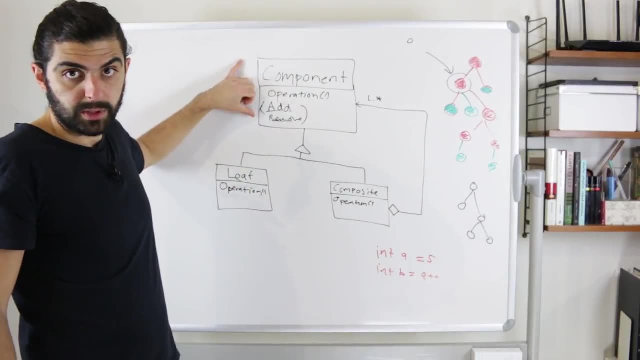 future video, Anyways. so that's why I was saying that if we instead construct these types such that we can build immutable hierarchies, then add and remove can suddenly be part of the component, because they suddenly now make sense in the leaf, Because the leaf, if you call add on the leaf. 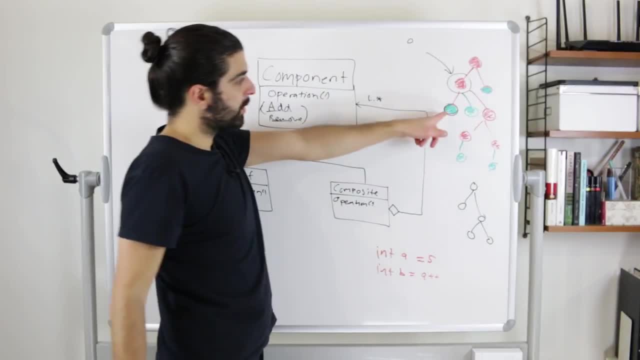 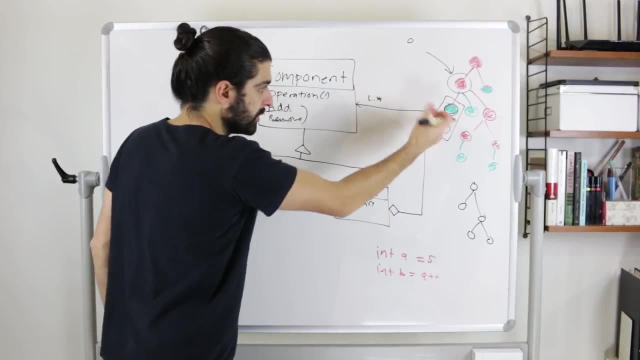 what it could do is that if you are here- right, this is a leaf- If you call, add on that leaf and pass it another leaf. what it could do is that it could return you a new construction of this relationship. It could. 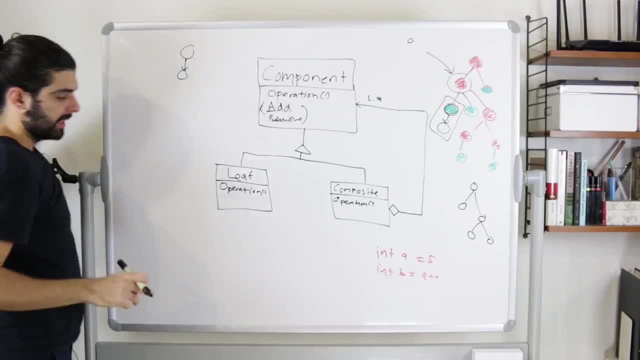 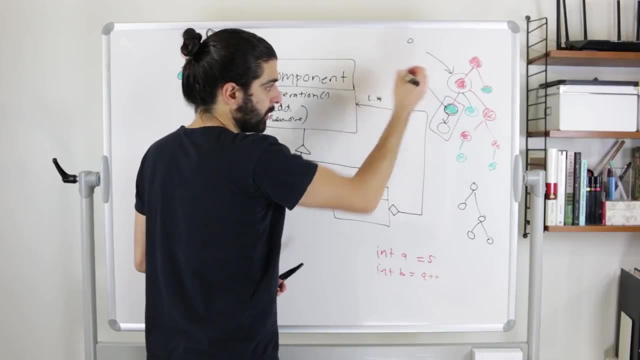 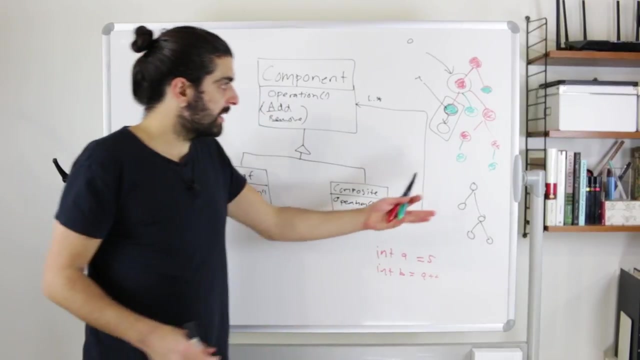 return you a composite that has a relationship with a leaf, So a composite object here and the leaf here, And clearly, maybe this node here that we were copying, maybe this contained X and now this composite contains X Because, again, you can't add in the old 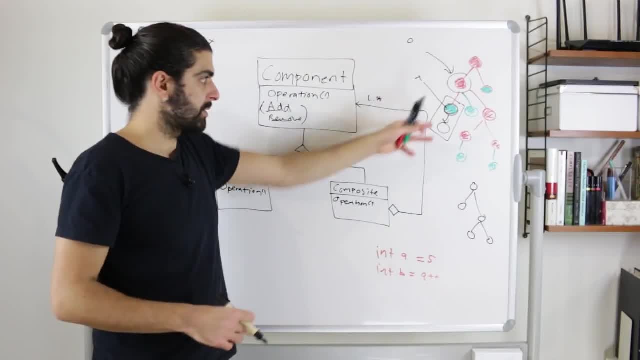 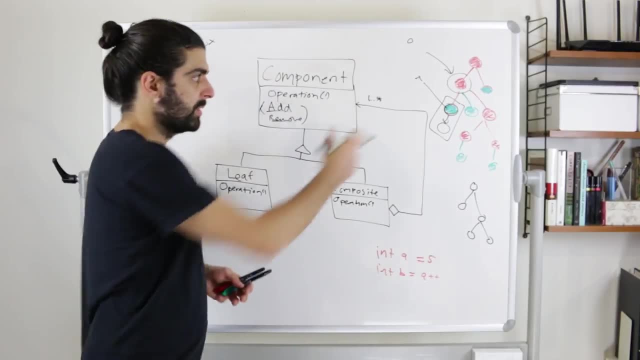 scenario: you can't add to a leaf because leaves can't have children, So you need to transform the leaf into a composite and then add. But when we are doing it in an immutable fashion, you can return the new value for this subset and then you can simply reconstruct So you can take out the 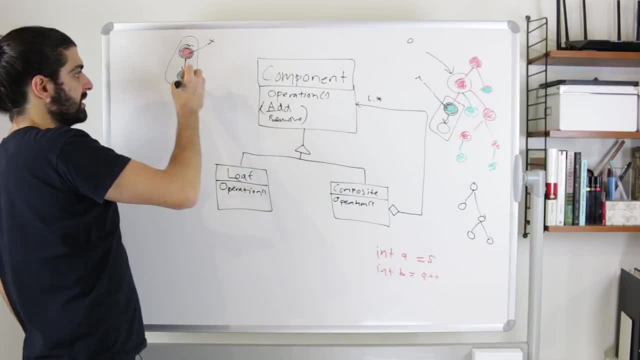 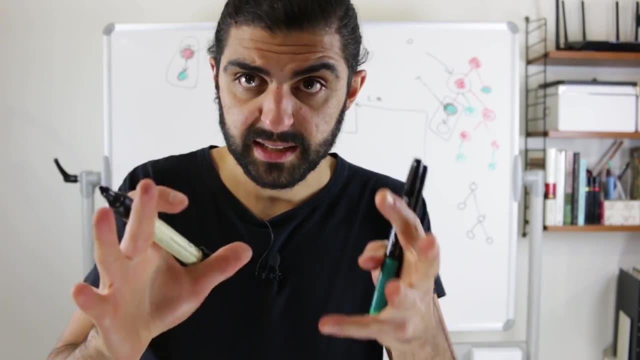 value from this old leaf, put it into a composite and then add a new leaf to that composite. But I mean, I'm sorry, this is total overkill for this pattern. If this doesn't make sense to you, don't worry about it, Ping me if you think this sounds interesting. 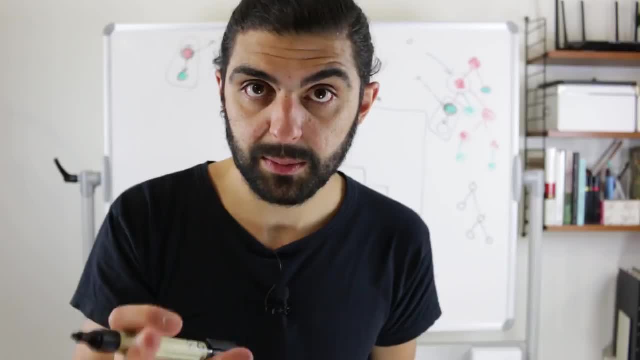 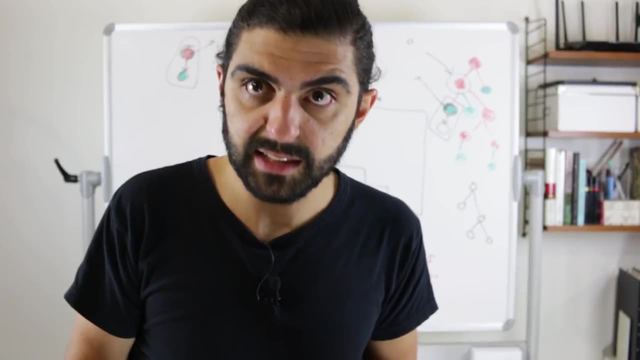 And we can talk about it some other time- And generally, whenever you can make something immutable, make it immutable. Whenever you can avoid having a data structure that changes, that changes its state, avoid allowing it to change its state. So this is why we are not. 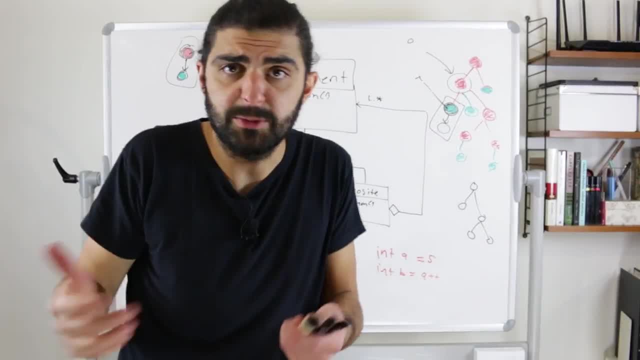 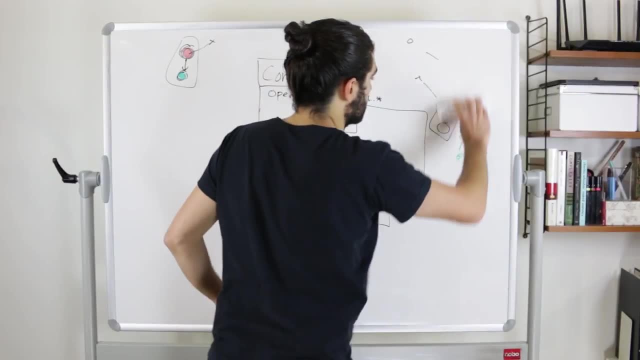 talking about the add and the remove methods, But again, if you really want to read more about that, check out the books. Anyways, okay, let me remove some of this stuff from the sides. Let's now move into the example. So the example I want to give is a 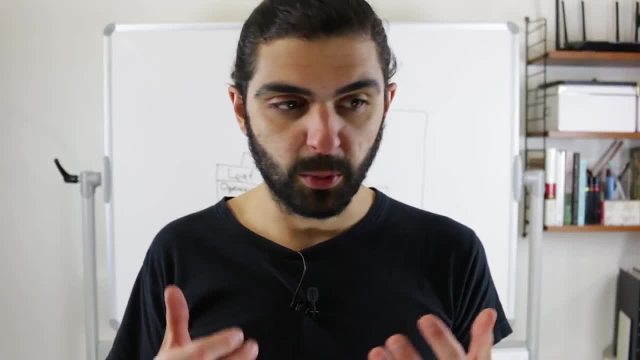 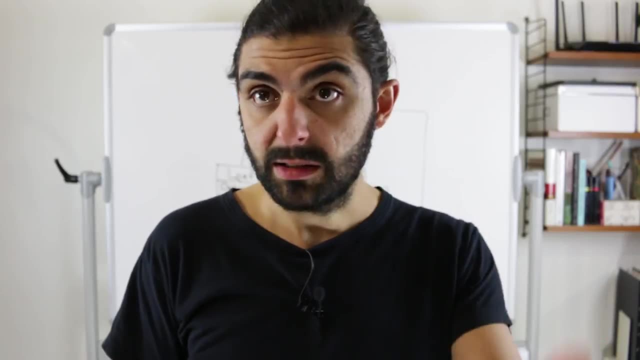 related to user interfaces. If you've read anything about the pattern before, you probably can cause some user interface related example, And actually I think these are as relevant today as they were in, for example, the 90s. But today we find these examples in frameworks such as: 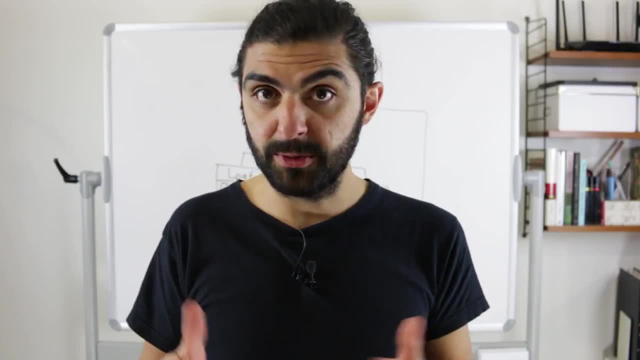 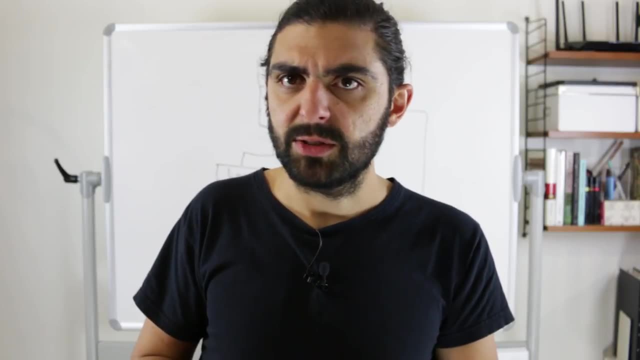 for example, React. So we're not going to talk about specific frameworks, but if you are familiar with anything like Emberjs or Angularjs or React, maybe even Vuejs- I don't actually know because I haven't tried Vue, but it might be, it might not be, But either way, the point. 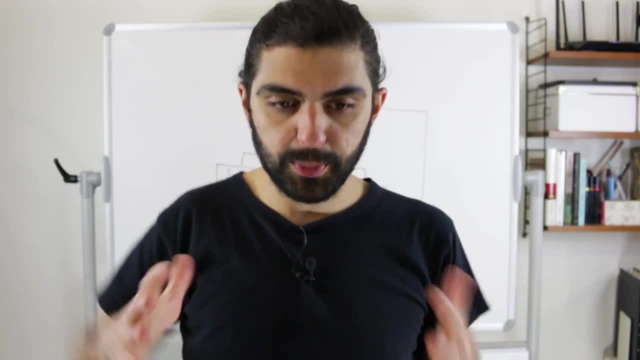 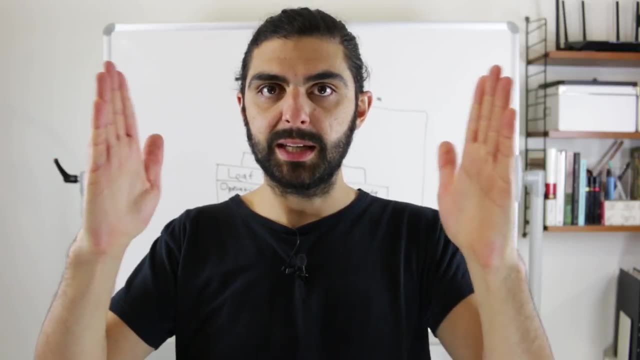 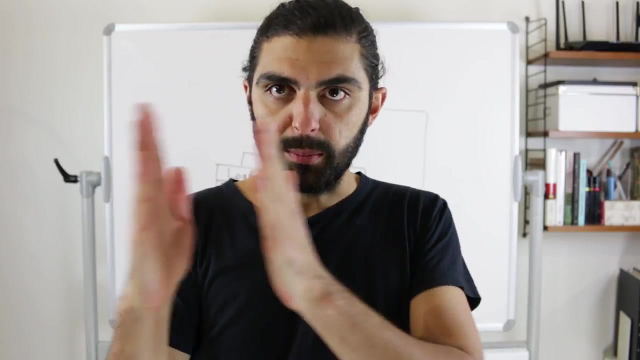 the point is that frameworks that are component based, that are built around the notion that a view is built from a main component that can be destructured or decomposed into smaller subcomponents, and every smaller sub component can be structured into smaller sub components. So the big, huge main 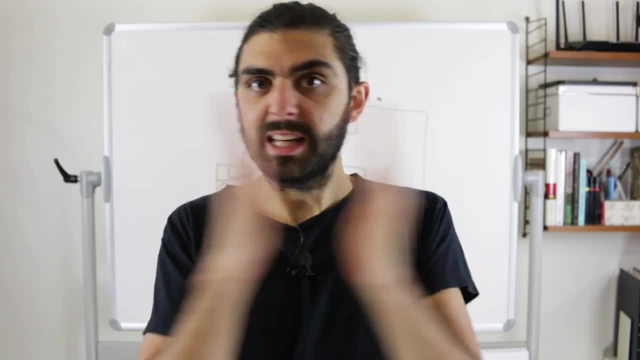 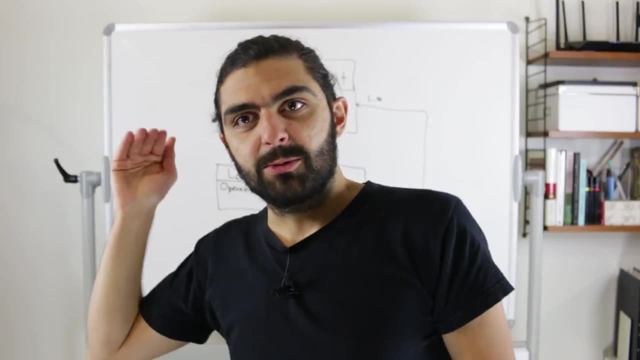 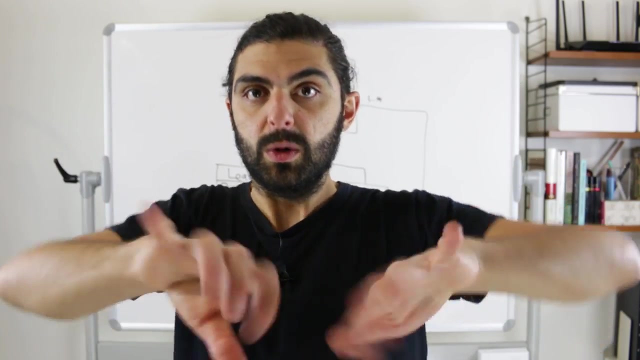 component has maybe two sub components, and each of these sub components have multiple other sub components. And that's the way you structure a page usefully, because then you can, for example say refresh to the outermost component and then that refresh command can trickle down into all of the small. 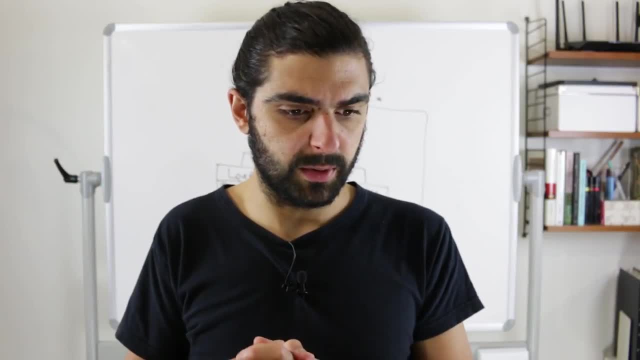 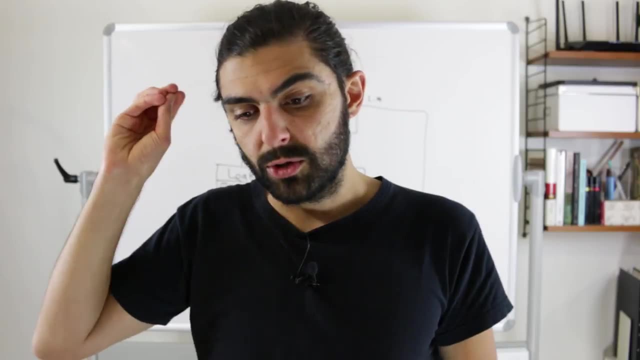 pieces of all of the components And that's not the way it's used in, for example, Redux. But I mean I'm not a heavy Redux user but I mean, but that library and other frameworks I guess sort of use the approach that you should send the data downwards and then propagate. 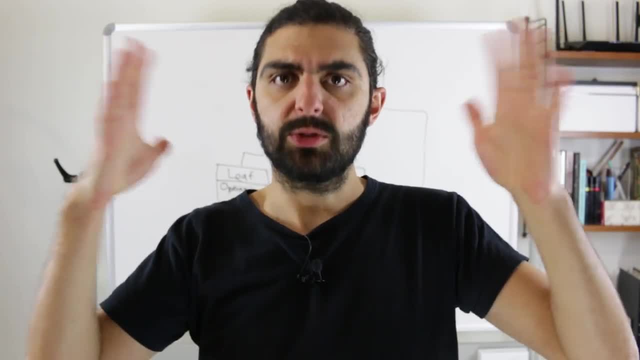 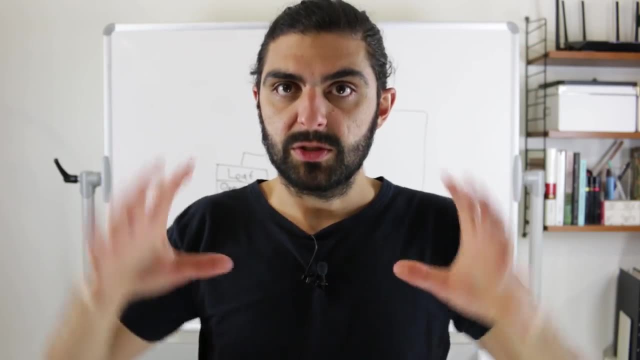 events up so that, for example, if you have this massive state tree that describes the state of your application, you give it to the main component and then sub portions of the state tree, sub portions of the information that should that should currently be displayed. 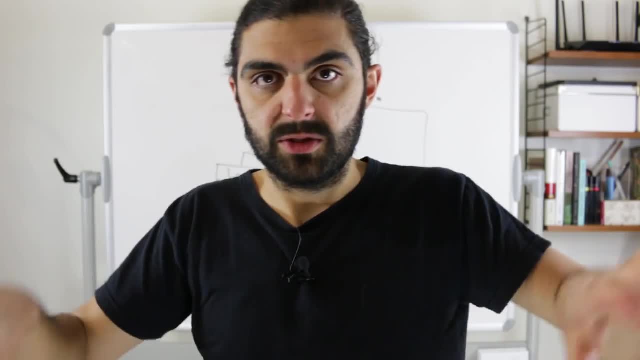 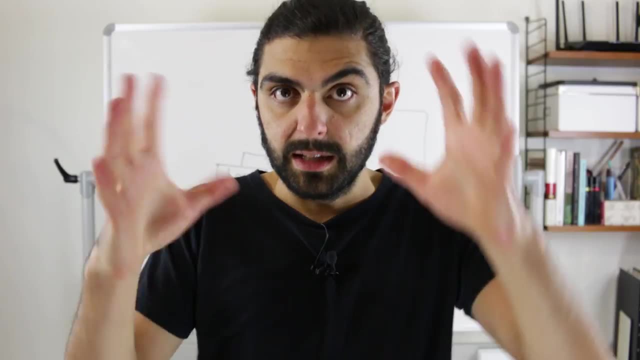 in the application is sliced off and passed down into sub components so that every component gets its its tiny piece of the state tree that it needs in order to display whatever it needs to display. But those are some real world examples and real world analogies. 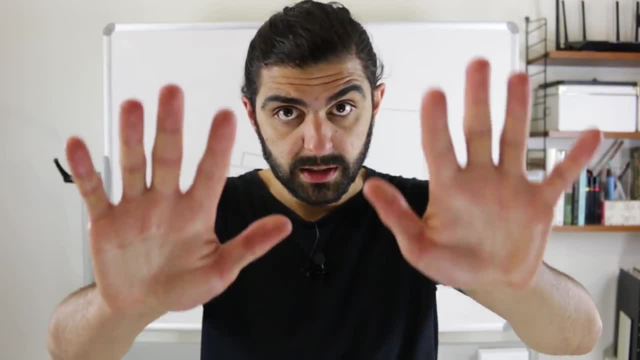 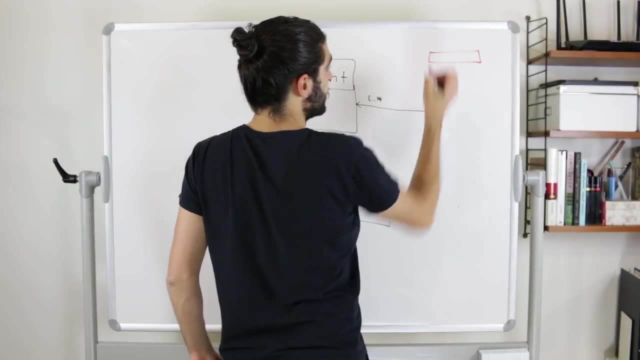 But anyway, let's talk about a simpler example. So imagine, imagine that you are building a to do application And this to do application is super simple. You just have, let me draw some to do text and then you have a checkbox next to it. 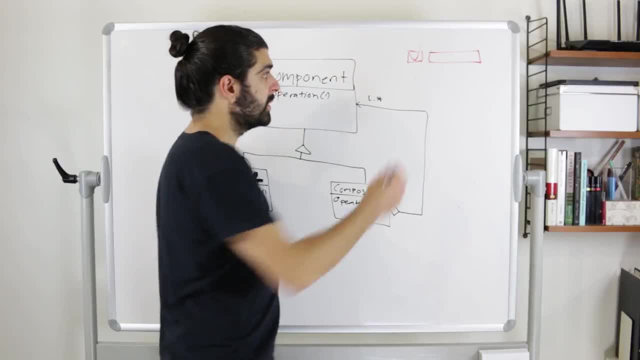 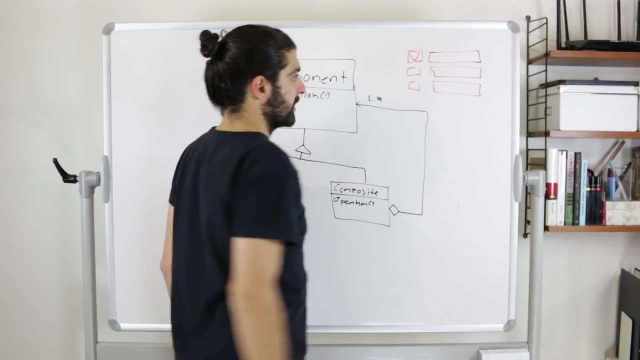 Then you can check as to indicate whether it's done or not. And then a to do list is simply a collection of these to do's, or I should say a list, more specifically, a list of these to do's where they can be checked or not. 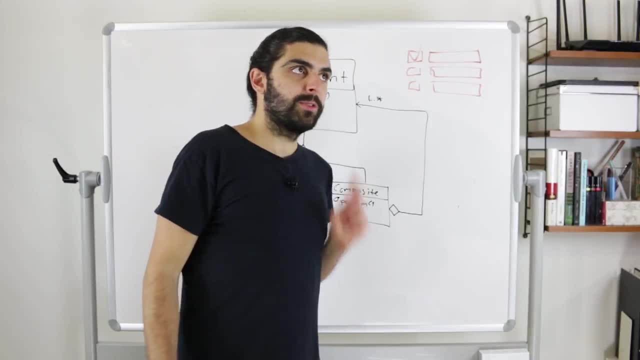 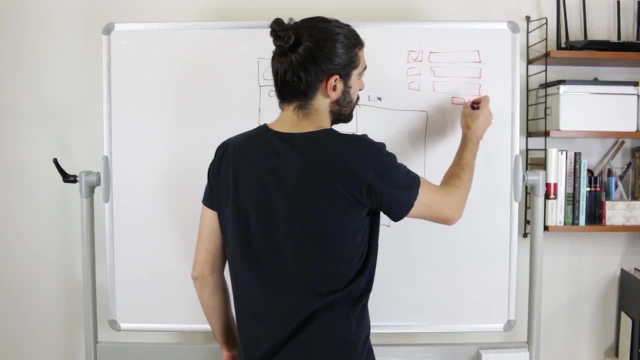 But then this is how we get into composite pattern. Then we say: what if you can have sub tasks of tasks? What if you can have sub to do's of to do's? So maybe this to do is compressed, All these to do's, and then we have another main to do out here, and then clearly, of course, 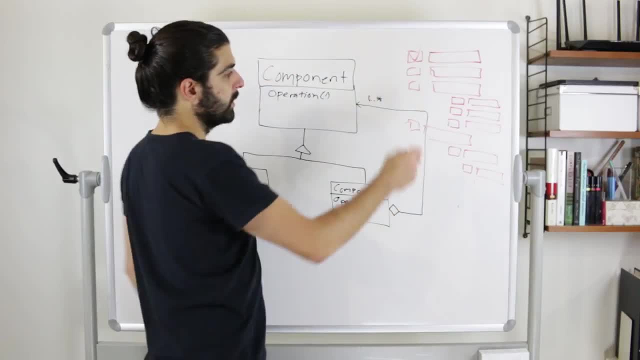 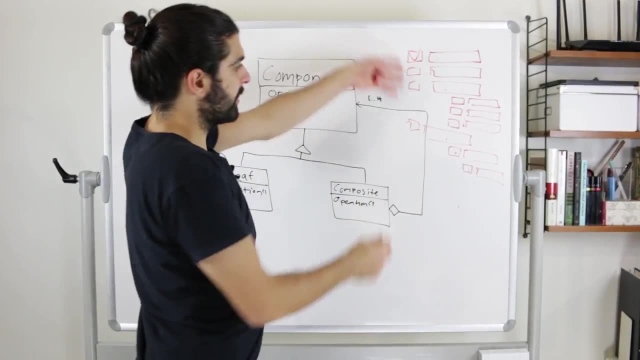 we could go further down into this hierarchy indefinitely. So this to do has three sub to do's, This to do has one sub to do, and this sub to do has another sub to do, And again. then, if you think about this, it's the same thing as saying that: OK, you have a. 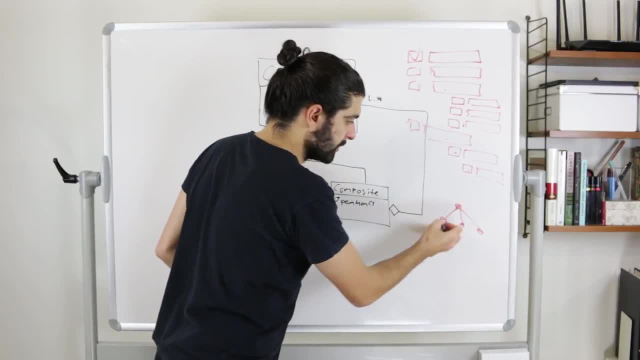 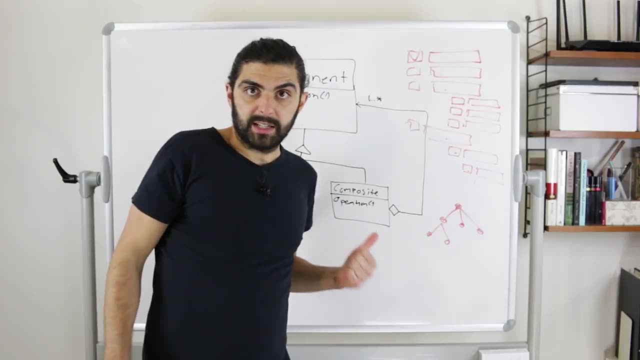 bunch of to do's and each of these to do's can either just be a to do or they can have sub to do's and so forth. So it's so. it's a tree in some sense, And the reason we want to use composite pattern here. 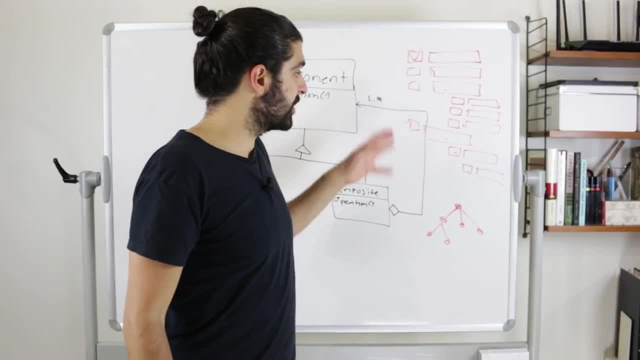 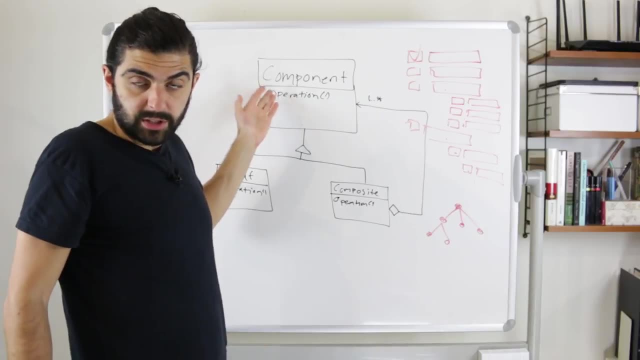 Is that we have the following requirement: What we want to do is that we want to be able to generate HTML for this. So let's say that we have objects in memory that describe this, but we want to be able to. our operation, Essentially, the function that we want to run, is that we want to say: give me the HTML that 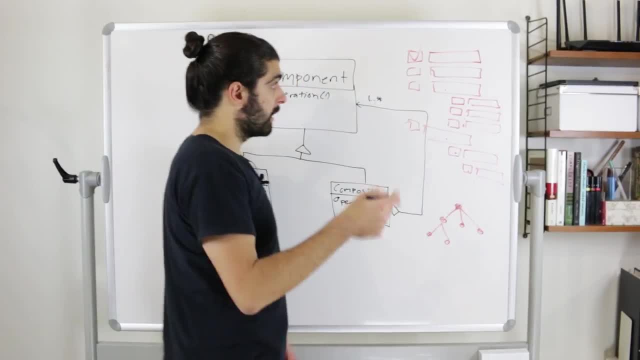 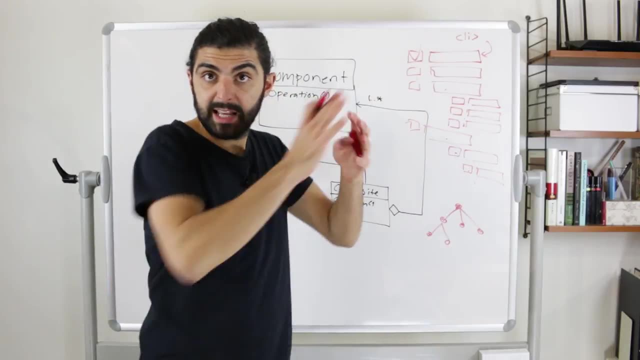 represents this to do list And we're just going to do it super simply. I mean, hopefully you're familiar with this, this level of HTML, but let's just say that we use LI elements to represent these. So it's an LI element with some text. 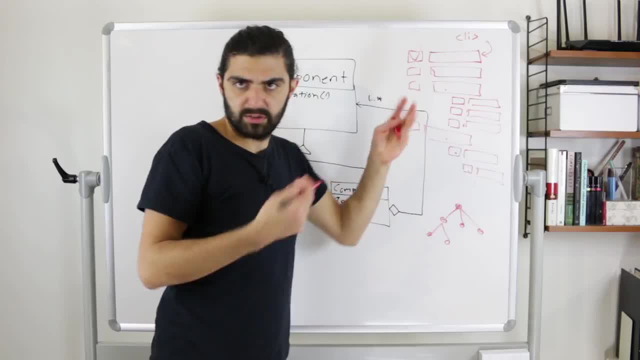 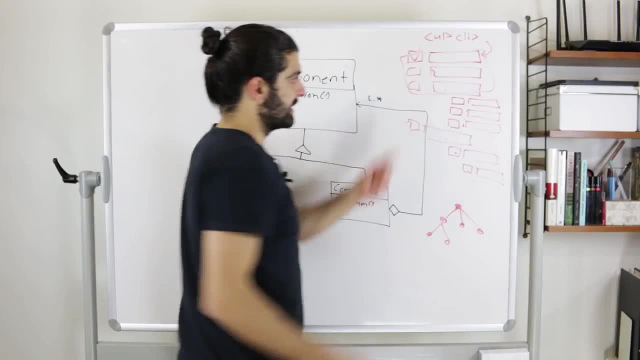 That's the to do right. And then maybe this is a checkbox, But maybe we'll skip it just to make it simpler. And then, clearly, when you have LI elements, you need to put them inside of a UL right. 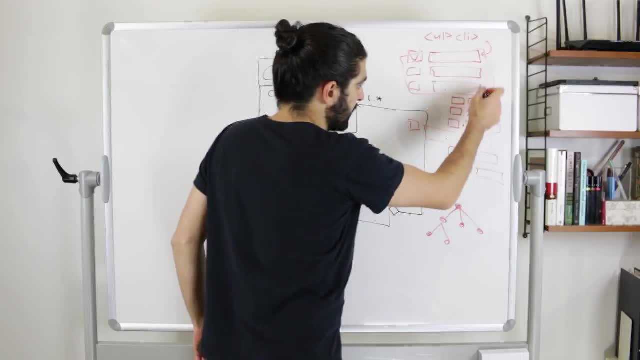 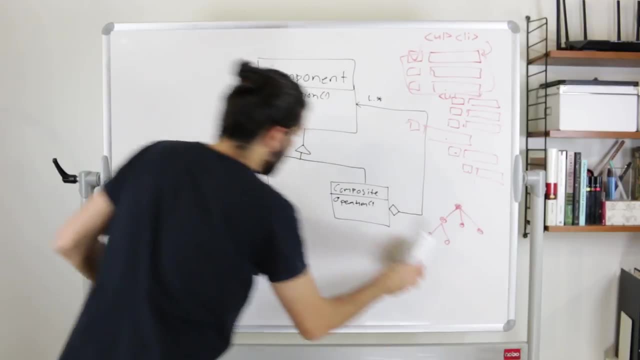 That's. that's how lists work in HTML, which also then means that when we have a to do that has sub to do's, we need to have a new UL. So actually let me remove this stuff because it's getting a bit crammed. 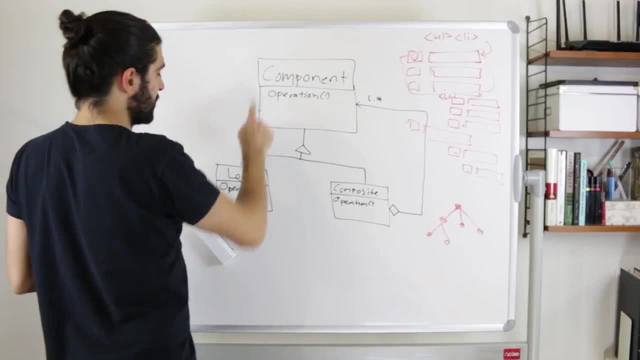 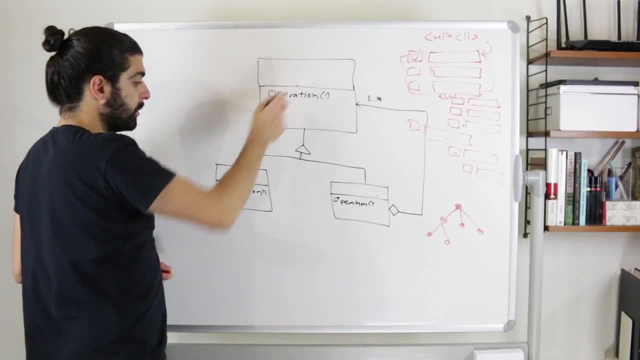 Actually, before I remove this, I want to get into the UL stuff. But let me just let's establish some terms for our example here, instead of these sort of generic names. So in this diagram we had the component, The leaf and the composite. 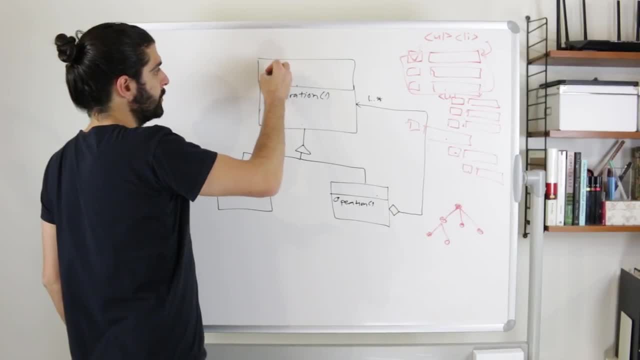 And in our case, what would we have? Well, let's say that this is maybe a to do collection. Let's say OK, let's say to do list. We have a to do list. That's sort of the main type. 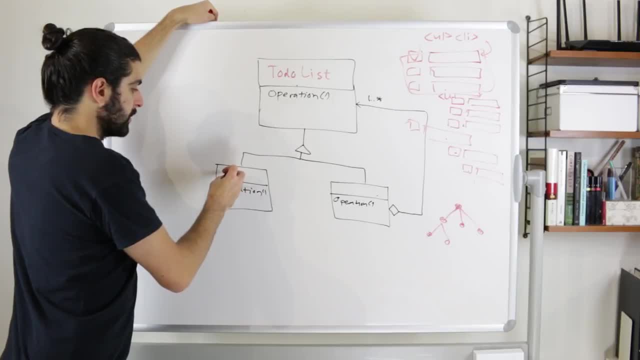 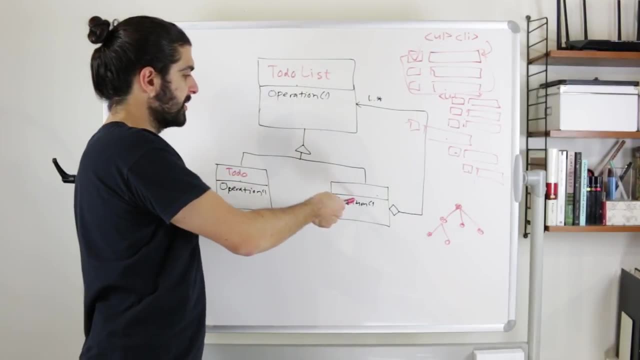 Let's call that to do list. And then, what do we call a leaf? Well, we should call that, maybe, a to do. And then, and then I realized the naming got a bit tricky because I mean, if this is a to do list, what will this be? 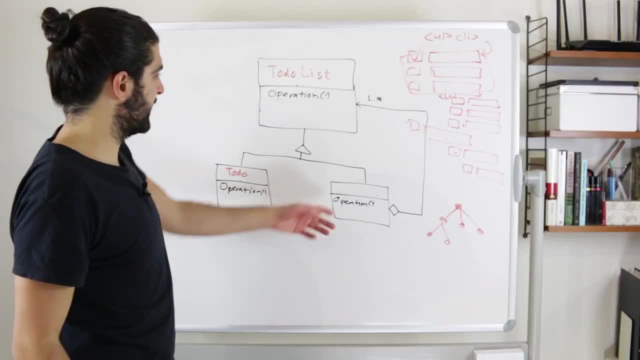 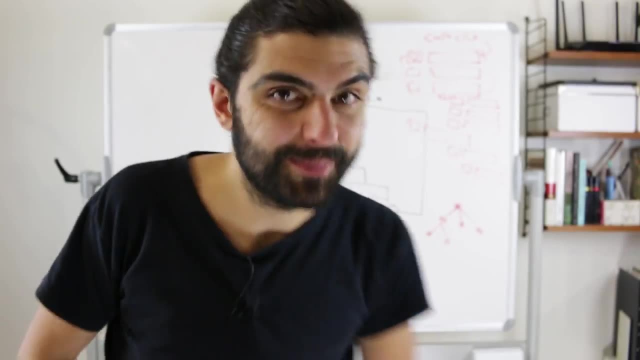 I mean, previously we had component and composite, So I mean, I guess maybe this would be to do's, or to do collection, or parent to do. We could call it multi do. Actually, let's think of it this way. Let's call this a project. 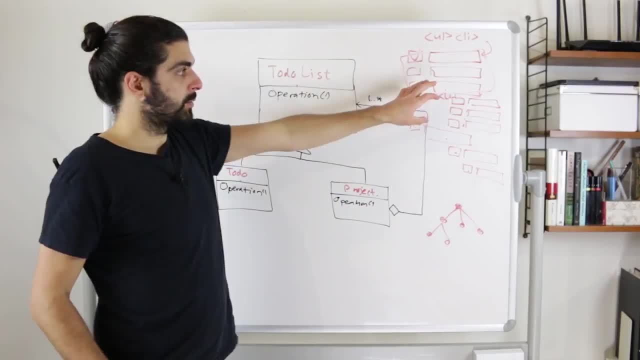 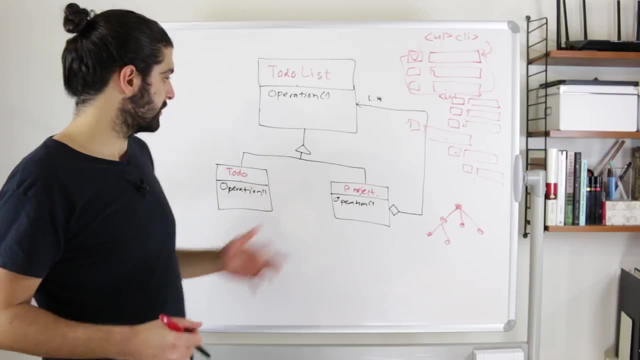 So that actually makes a bit of sense, right. Like, if you have a to do that has multiple sub to do's but it still has a name and it can be completed or uncompleted, then maybe that's a project. So a project is in some sense a to do list, and a to do list is comprised of either a: 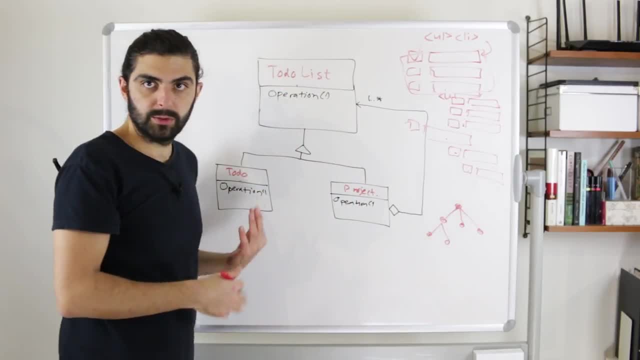 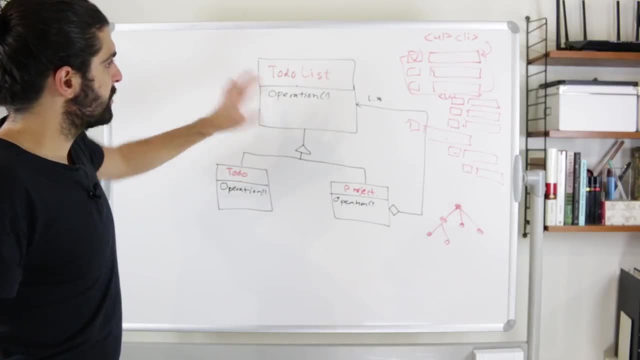 project and a to do list is either a project or a to do. I mean is sounds kind of funny in this sense, but hopefully I think actually this will play out quite nice, But let's see. So anyways, I was about to delete that. 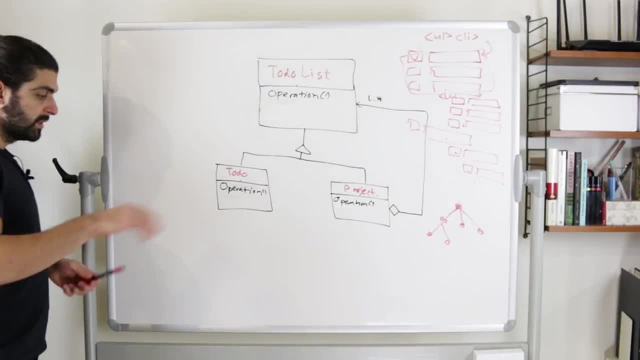 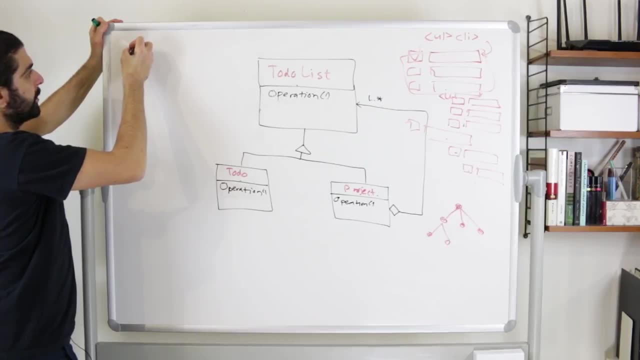 Do we want to do that? No, actually, let me use this space here. So what I wanted to do is just super quickly say something about how lists in HTML work, just so that everyone's on the same page. I mean, so if we want to have an unordered list in HTML, we say UL and then we put ally. 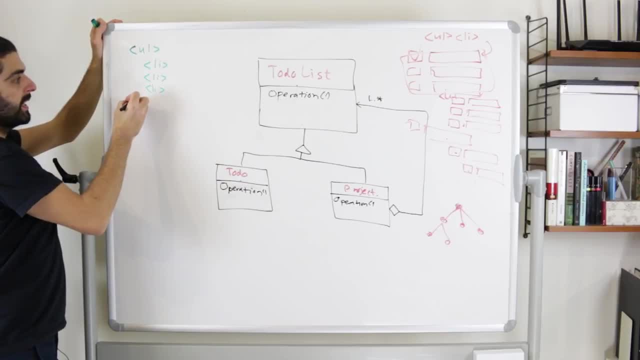 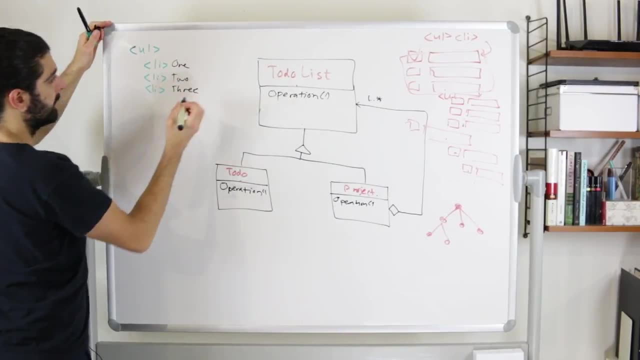 elements. that will contain all of the items and then we close the UL element whenever we are done, But let me put these items first. So just say one, two, three, That's it, And then we close. So this is an unordered list of individual ally elements. 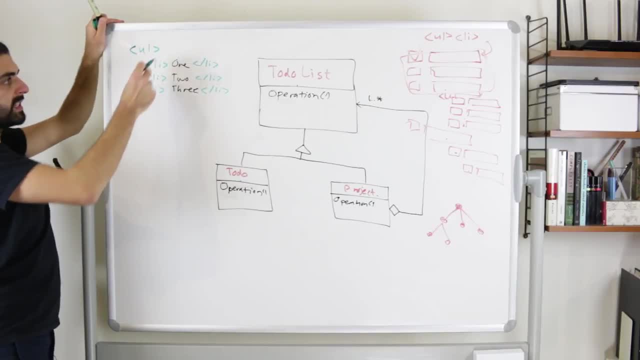 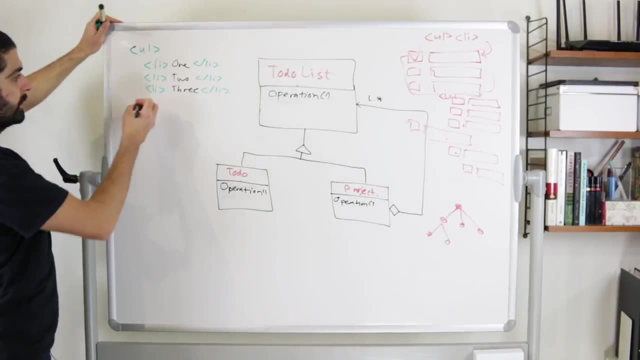 And, by the way, ally stands for list item. So UL stands for unordered list and ally stands for list item. So this is an unordered list of three list items and we need to close the unordered list. But what I want to do is also show that the fourth element here let's say that we have. 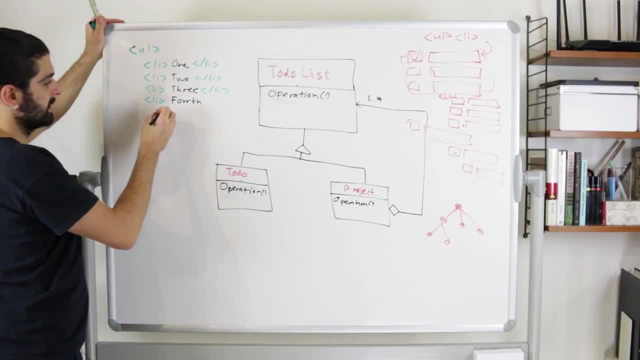 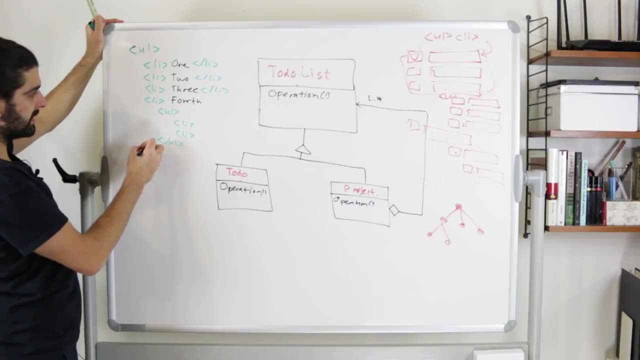 a fourth element here We could also say that this one also contains a UL, which in its turn, contains a bunch of ally elements. So, and here we close this UL, we close this ally and we close the outermost UL. We need to close these as well. 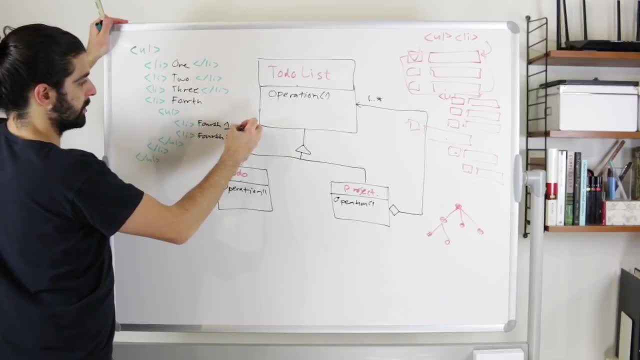 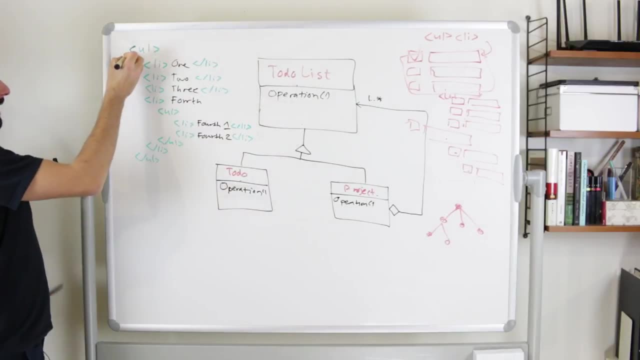 So let's say fourth one and fourth two, And then we close these sub ally elements. So HTML isn't necessarily a bit messy, right, But just think about which tag closes this tag. This UL closes this UL. These allies are all closed on one row. 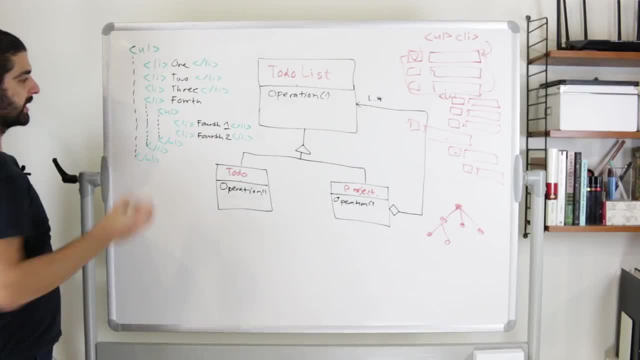 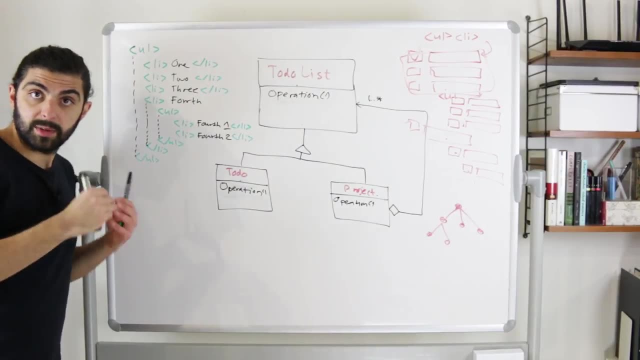 But then this ally is closed here and this UL is closed here, And then these allies are closed individually. So whenever you have a list of items, we need to have each item wrapped in allies, But that collection or that list of ally items 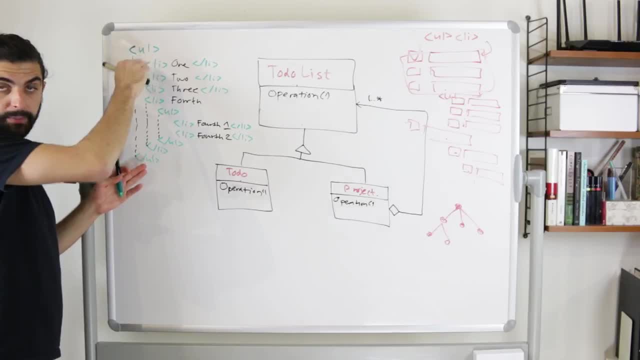 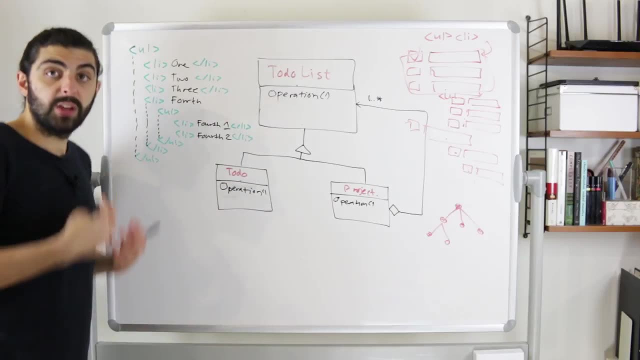 Need to be wrapped inside a set of UL tags And then, whenever we have sub lists, whenever we have projects, using our terminology, we need to introduce another UL within an ally, But we also use the name here which is then supposed to be the name of that project. 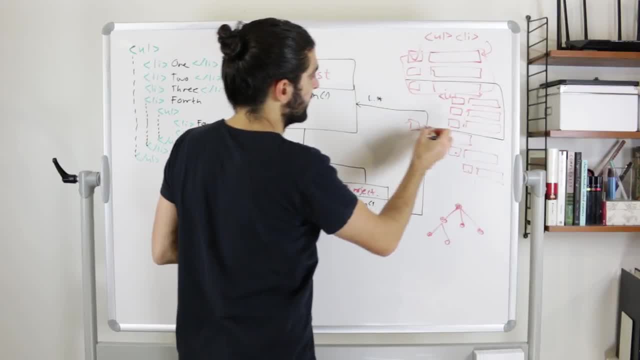 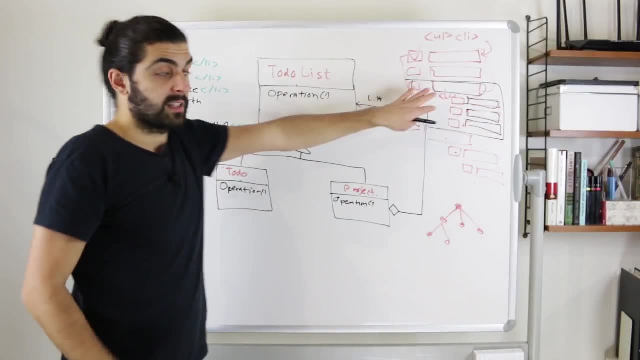 So if you think about this, if you look at only, let's say, this subset here, then this is the name of the project And these are the sub to do's of that project, meaning that this is a composite, where this is actually the composite. 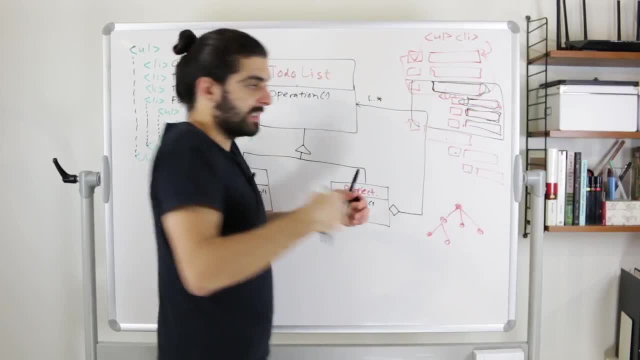 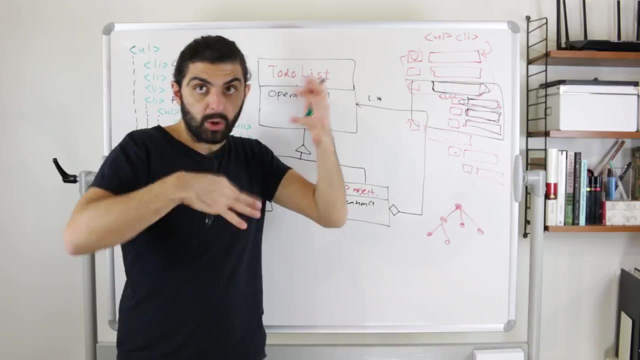 And these are the leaves that the composite is pointing to, These are the children of that, of that composite. And again, if you think of the first example, we took it way back in the beginning. I used children in the opposite sense because then, which was maybe a bit confusing- 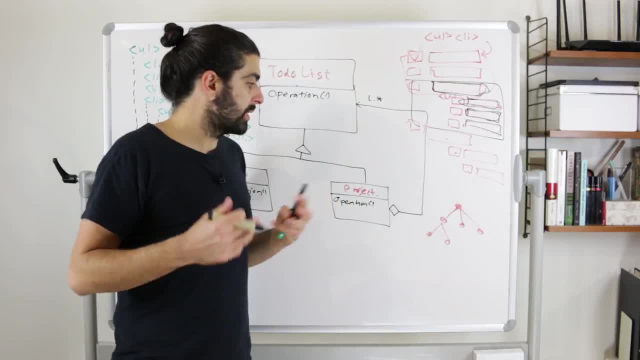 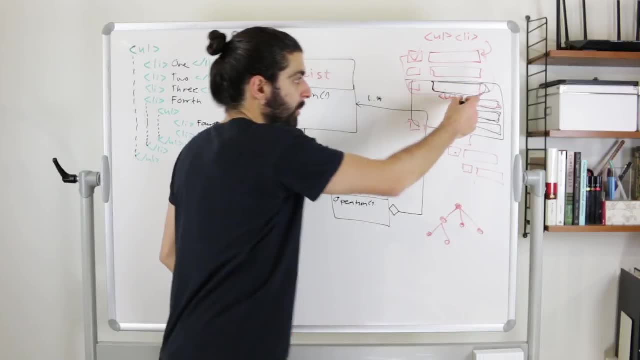 But again, when I say children here now, I mean what's in the collection of that composite? The composite is a collection of object, The composite is a composite of objects, And this composite is a composite of these children, of these objects. 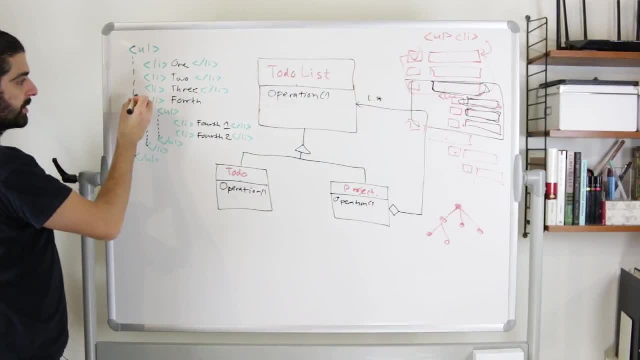 So again, if you think about only that, That subset, then that subset corresponds- let me choose a different color- is, let's see, equivalent to this subset here. So that looks a bit counterintuitive because I'm including the text. 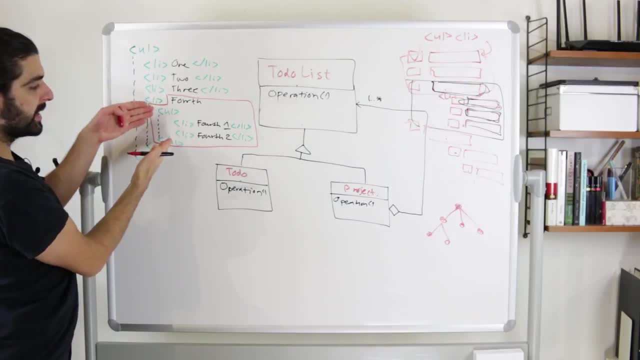 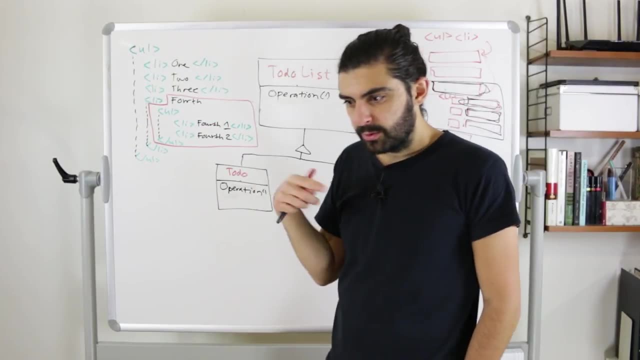 I'm including the text but not the li element, And then I am including the sub list, the whole ul element, And the reason for this is I gave this a bit of thought just in my head before I started making this video And I thought actually there are two interesting paths that you can take when modeling this. 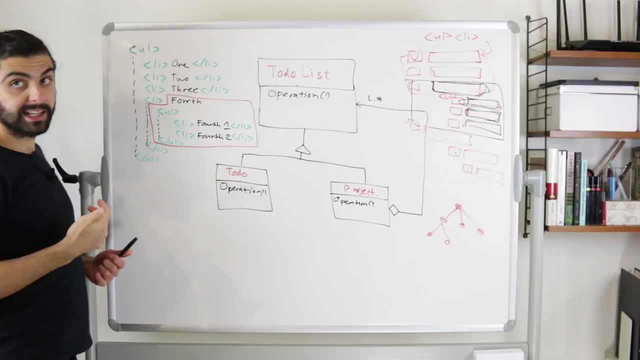 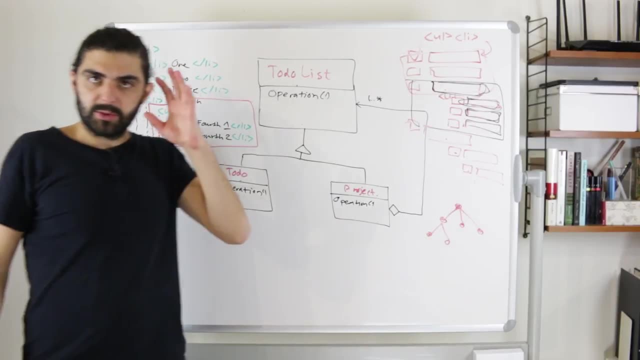 Either you say that a composite element includes an li tag Or it simply includes only the text, Or, if you think about it from another perspective, the leaf. That makes more sense. If you think about the leaf, does the leaf include the li tags? 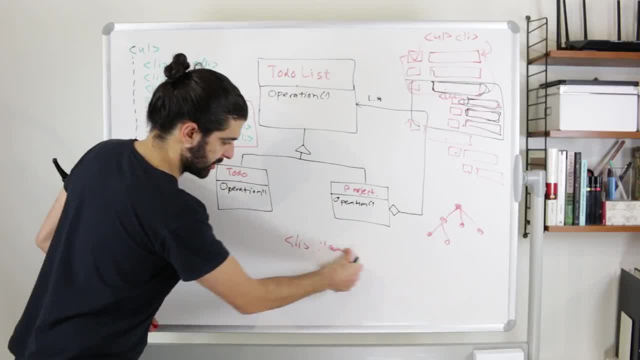 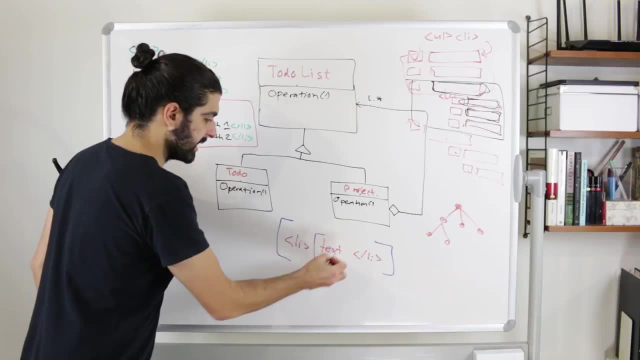 So you have the li tags and then you have an item, item text where I should actually say text here, And then you close the li. So either this whole thing is a leaf or only this thing is a leaf. And what I decided is that if you would have the check mark, I would put the check mark. 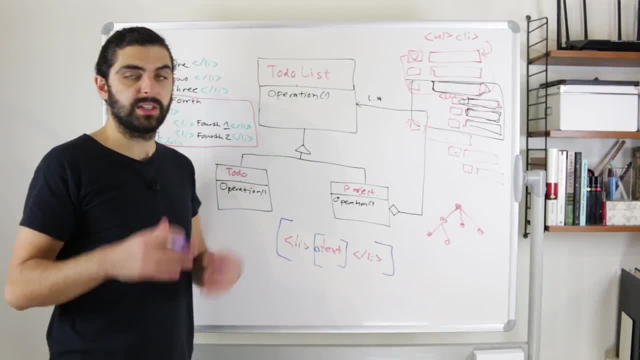 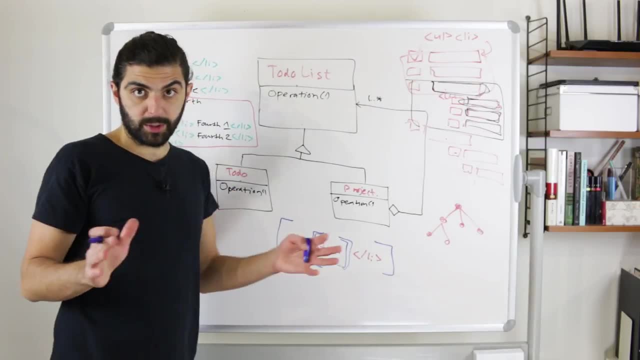 inside here. So the text and the check mark or not the check mark, Sorry, The check box. The check box and the text, I would say, is part of the leaf, but the li needs to be part of a component And hopefully this will play out when we think a bit more about this scenario and when we 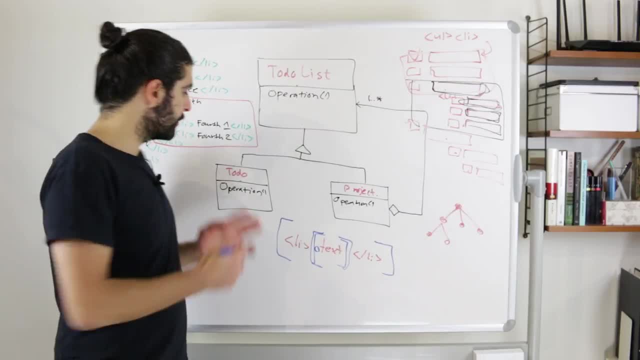 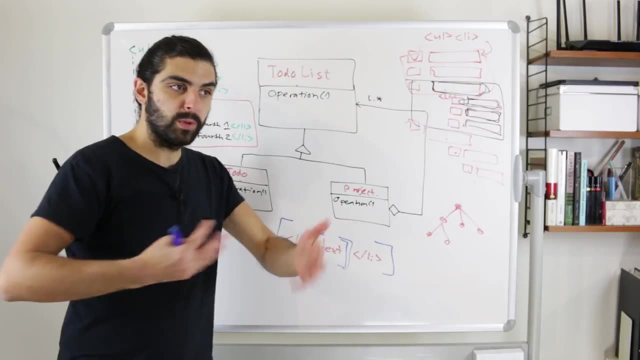 look at the code. So the reason I'm raising that question is that what code you put in leaves versus what code you put in components depends on your scenario. But it's also possible that you have multiple solutions for your scenario, but with different benefits and with different drawbacks. 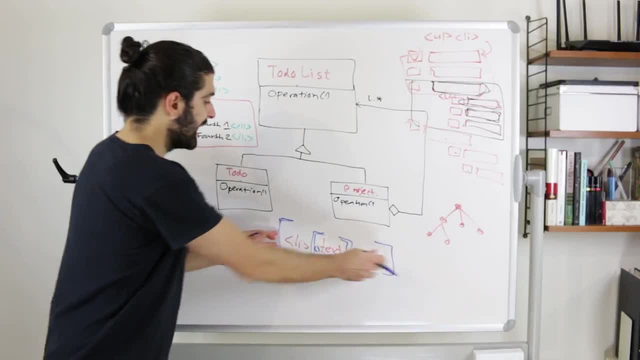 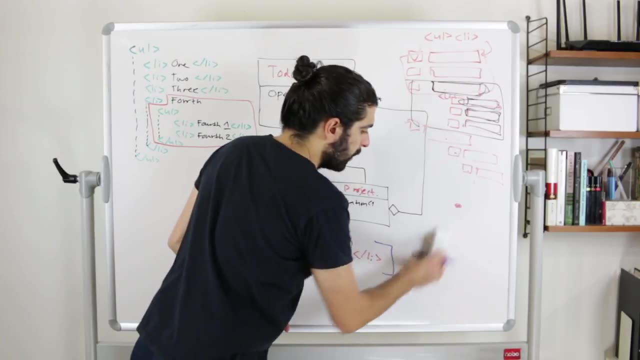 So one drawback of doing this, for example, Like making the li's included in the leaf, is that, since leaves are to do lists, it would then be possible for the user of the code to say that what I have is not a tree. What I have is simply a single leaf. 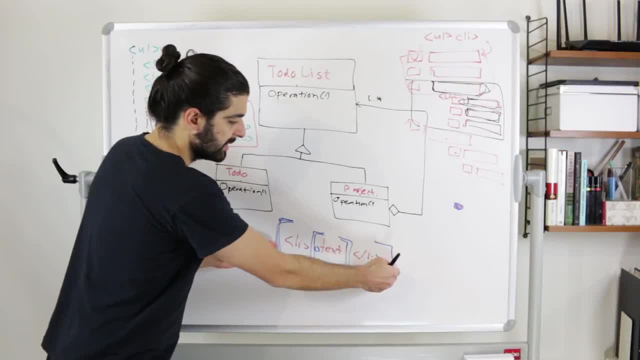 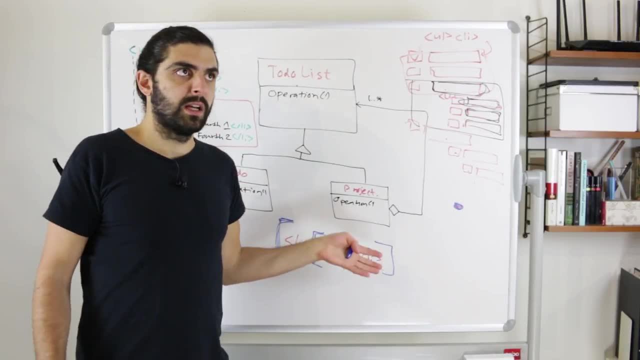 And then that single leaf would render as an li element without a wrapping ul element, And that's sort of the killing blow for me. That's when I thought, OK, wait, in this scenario I think that's an unacceptable drawback. So I would think that you definitely always need a ul. 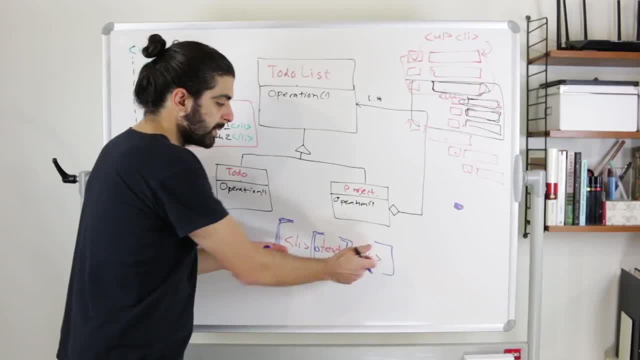 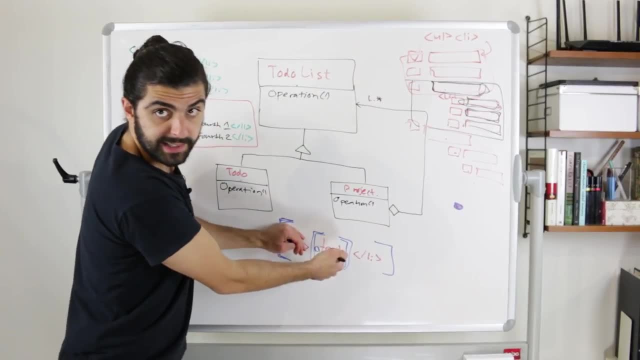 But at least If you put only a single to do, we can't render only li elements, because that's probably not even valid HTML. Instead, let's only then render the check, the checkbox and the text. Maybe that would make sense, right. 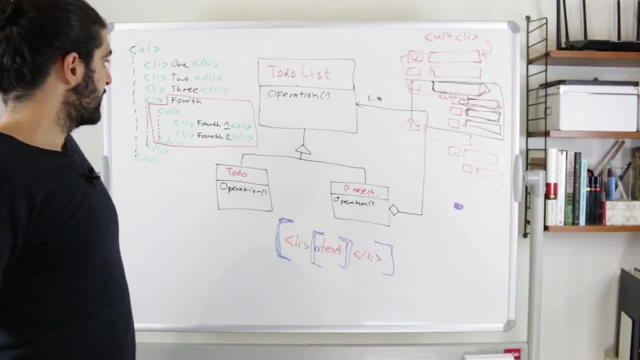 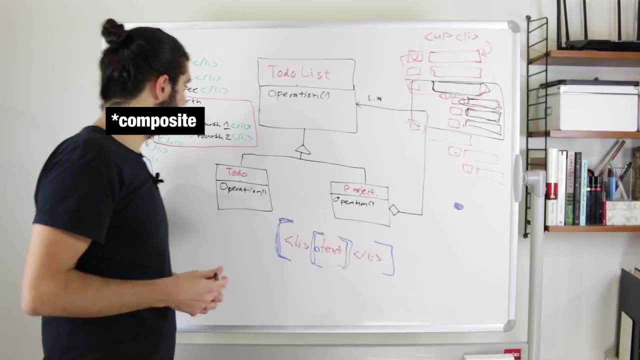 Like maybe you could reuse that component in a different context, But anyways, now we're getting ahead of ourselves. The general point is that in composite pattern you can think a lot about what should be part of the leaf and what should be part of the component. 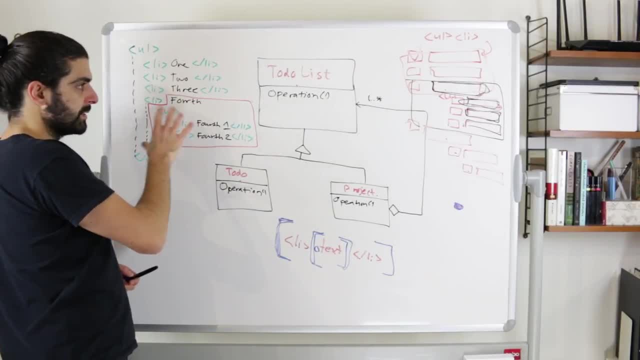 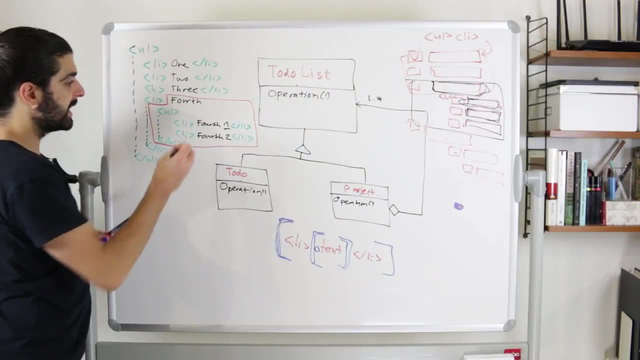 Anyways, this is what I decided. So this means we drew this red area here to to specify that this is part of a composite. Let's draw the same thing For a leaf, So, as I drew down here, then the leaf would then simply be this thing, the text. 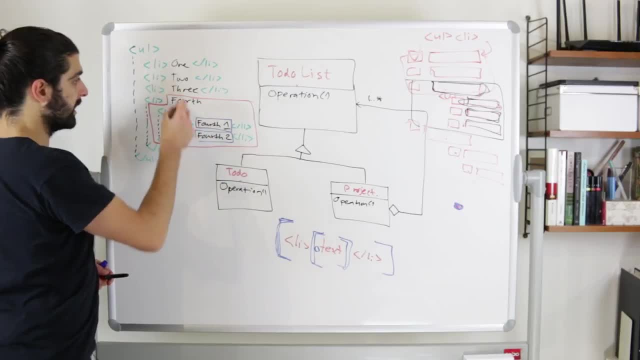 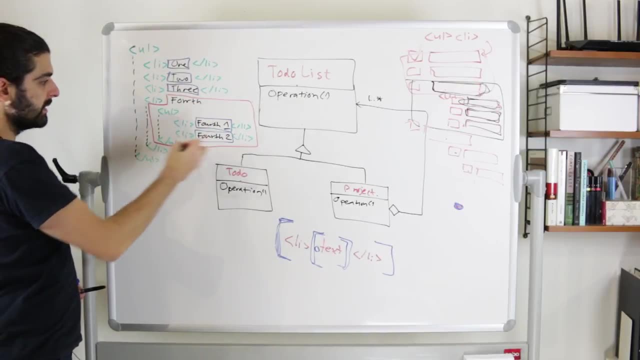 And again, if we had a checkbox, it would also include the checkbox. So these are all leaves And actually here these are leaves as well. These are leaves. Fourth is not a leaf because it's composite And if you think about the whole structure, this whole structure is actually a composite. 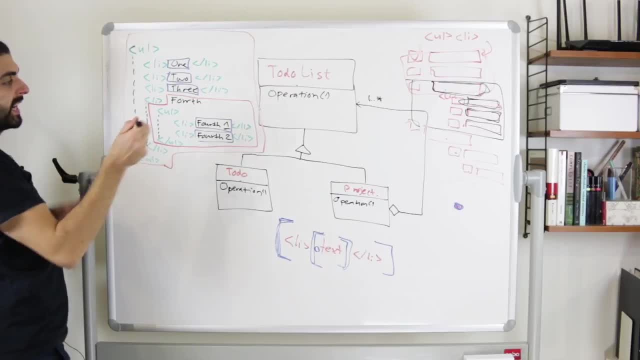 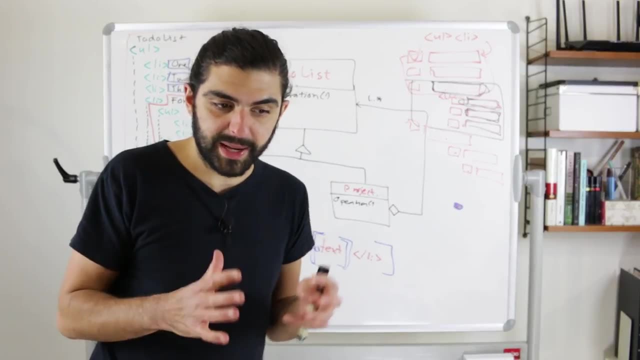 as well, which probably means that it needs to have some kind of title here If this is the structure of our composite, So maybe we will call this our to do list. So hopefully you can start to see now how this pattern could be useful in contexts where 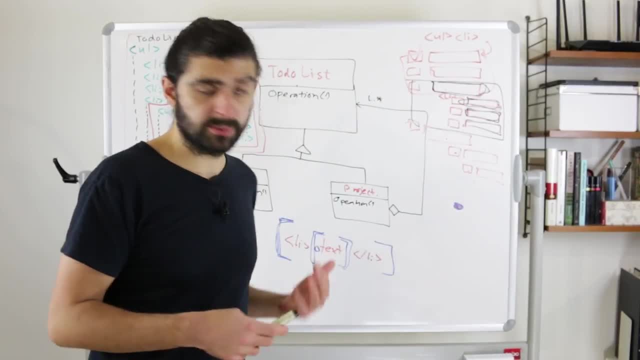 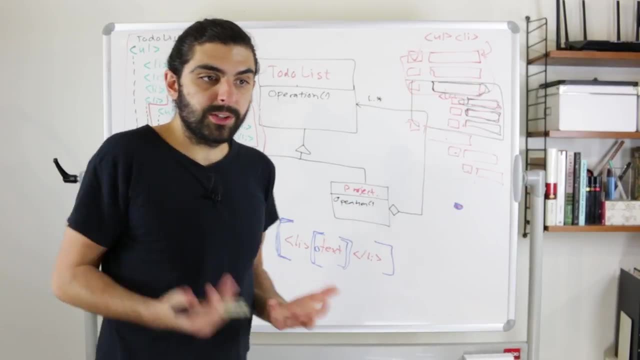 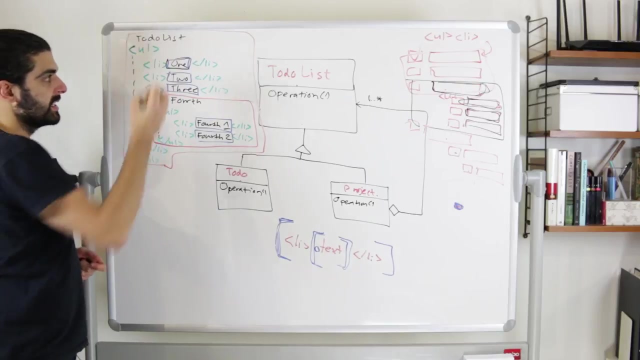 you have sort of a data that's hierarchical by nature, such as, for example, HTML. I mean in some sense, then it's kind of trivial to construct your, your object hierarchy and then render HTML from that object hierarchy. So this operation here in the to do essentially only has to specify how to render this, which. 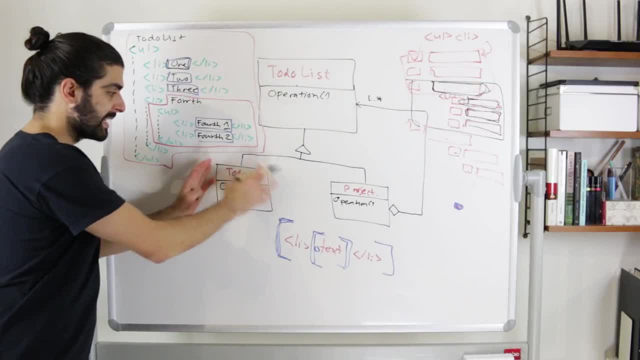 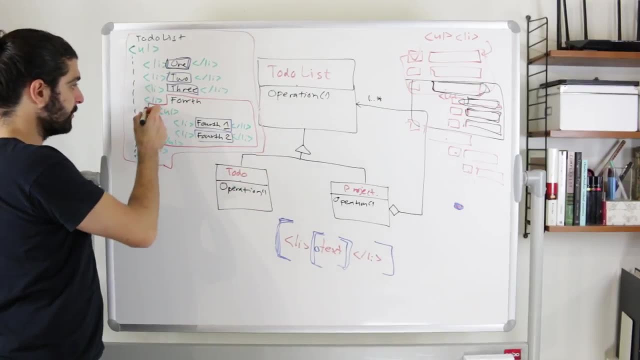 is essentially just to return the string that represents the text that is contained within this. to do So, the project- in this case, or in the general sense, the composite simply has to has to figure out, or the algorithm that we have to write simply has to be, how to render this. 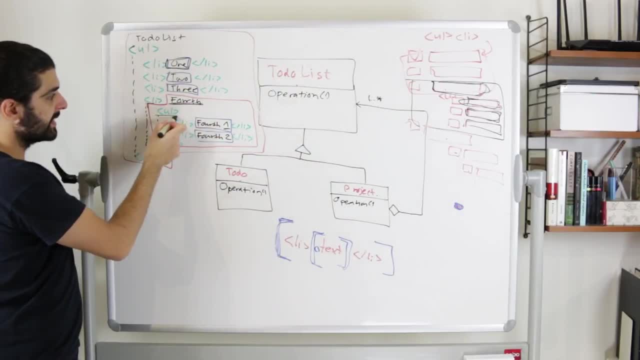 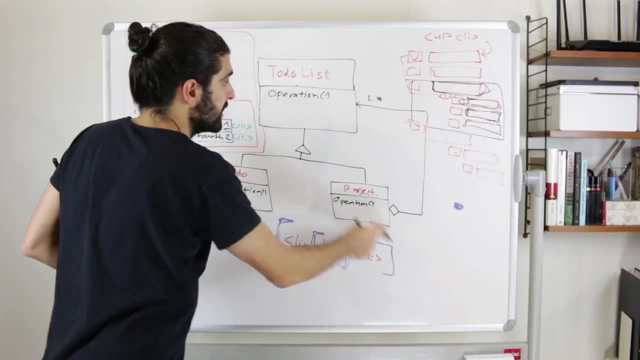 stuff which is essentially just a string comprised of the title concatenated with an opening UL element, And then we iterate through all of our children, We iterate through all of the components that we have, That's, that's part of this composite, And then we call the operation on them. 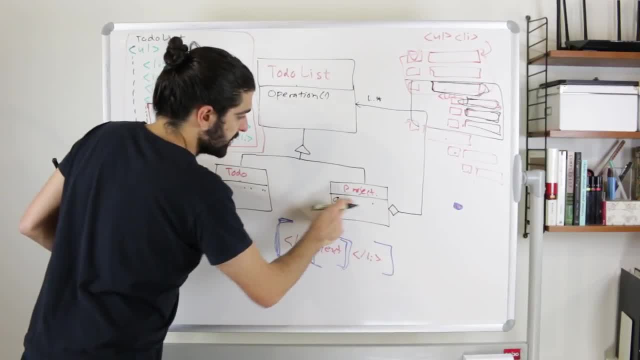 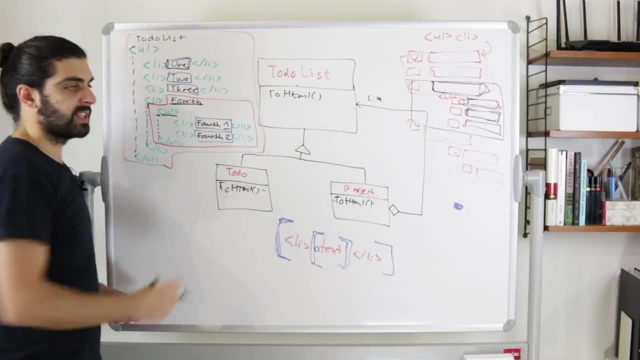 Sorry, I didn't change the name of the operation here. Perhaps the name of the operation here in our to do Example should be to HTML or something along those lines. Right, And I'm saying to HTML rather than render, because I'm trying to imply that it would. 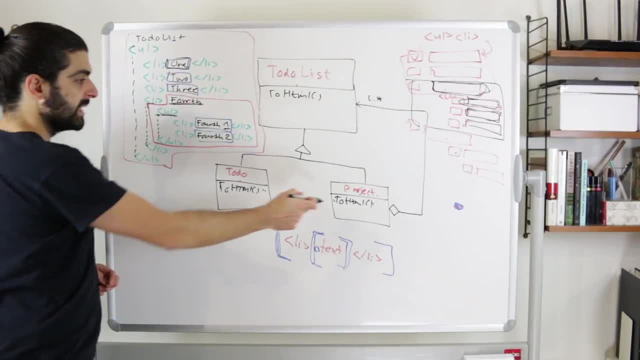 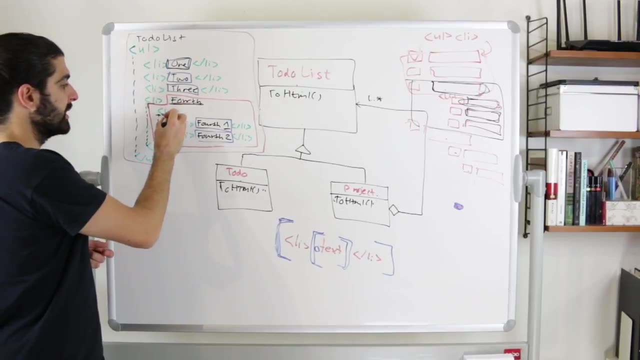 return a string rather than sort of printed to screen or whatever, But then this to HTML method of the project, essentially of the composite would then have to figure out how to print that. So again, so how to render this area depends on the number of components that it has. 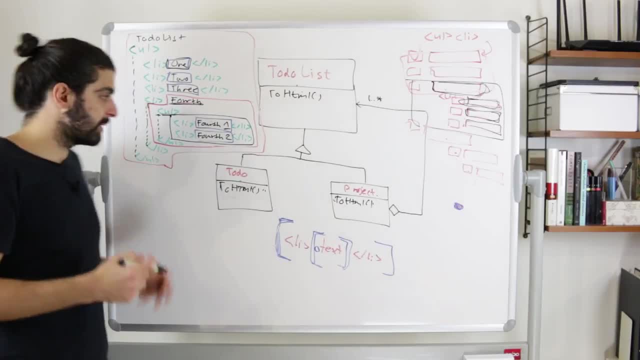 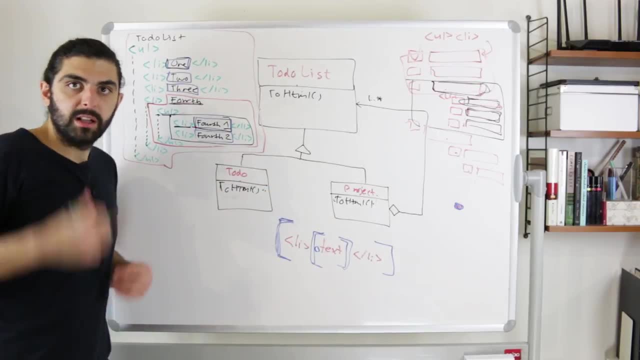 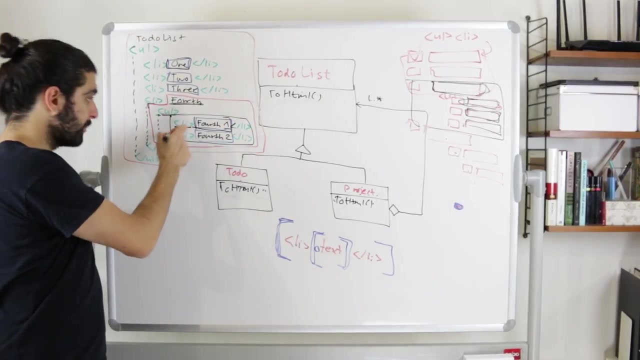 So it has a list of sub components and it iterates through this list of sub components and puts: So it's an ally, an opening ally tag, and then calls get HTML or to HTML for that sub component And then, whenever it has that HTML, closes the ally tag. next step of the iteration: prints. 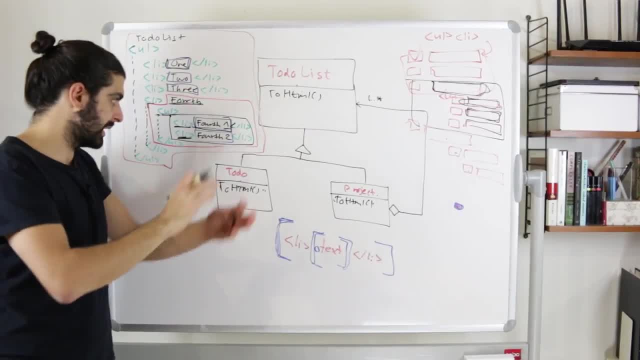 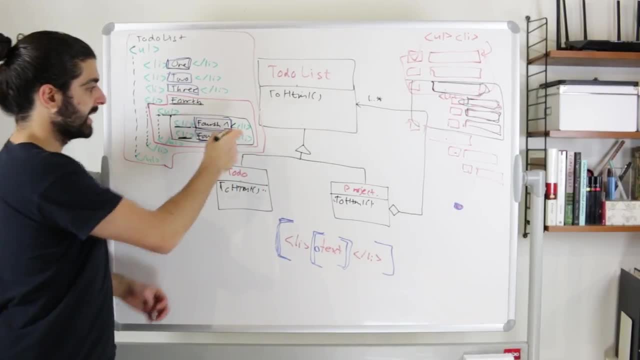 an ally tag again, or adds an ally element to the string, then calls to HTML on that next child of the iteration, on that next sub component, gets this text back and then closes again. So here's where the recursion gets in. But I think it's probably easiest now if we start to look at the code but just think. 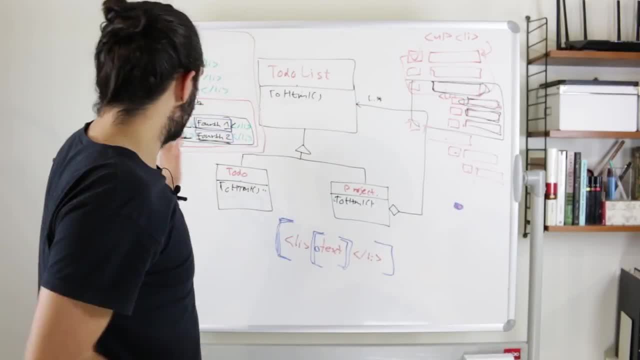 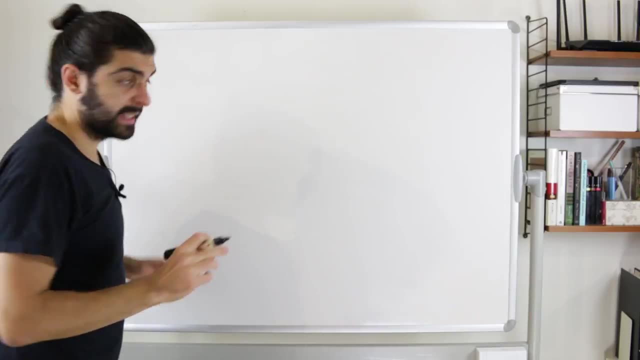 about this example. Just remember that this is sort of where we are going. but let's, let's now try to model exactly this scenario in some sort of pseudo code. Let me remove this stuff, Okay. So let's define the stuff that we have. 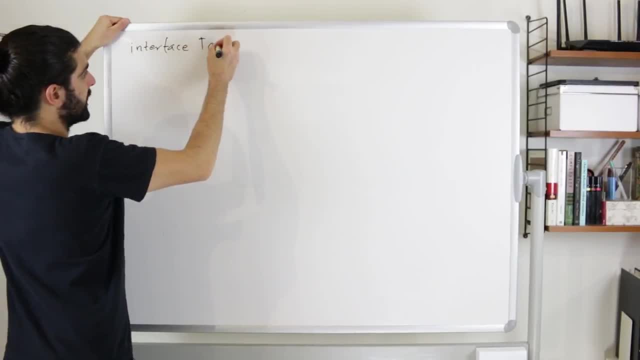 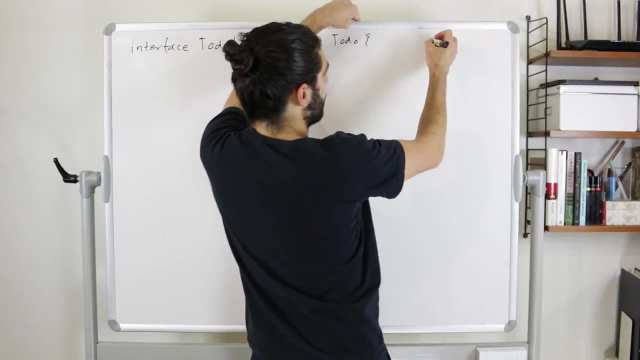 Let's start with. we have an interface that's called to do list. Open that up. Then we have a class that's called to do and that's the leaf. And then we have a class that's called project, which is a composite of to do's project. 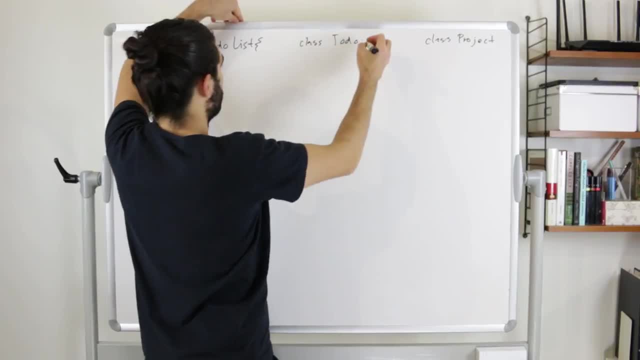 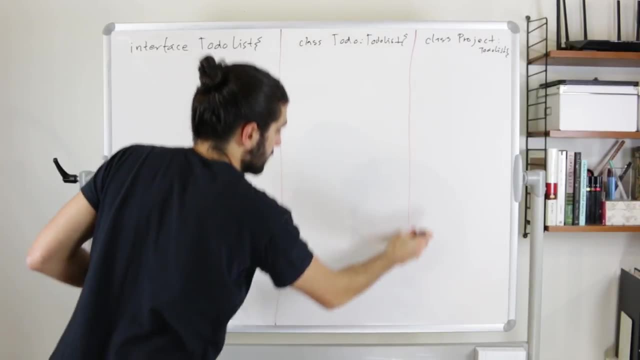 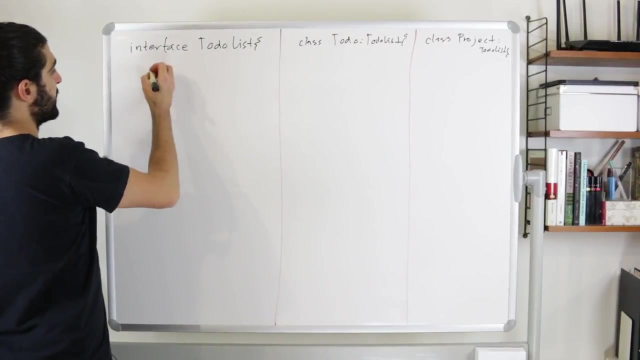 And immediately. We know that to do's should implement the interface to do list and projects should implement the interface to do list. Okay, To do list, to do and project. So the to do list interface simply specifies a single thing. It specifies that in order to be a to do list, you need to have a method that returns a string. 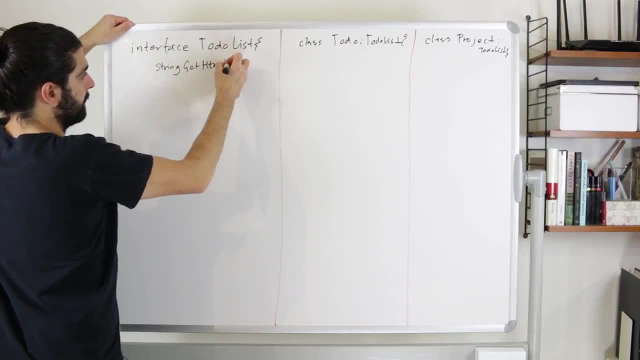 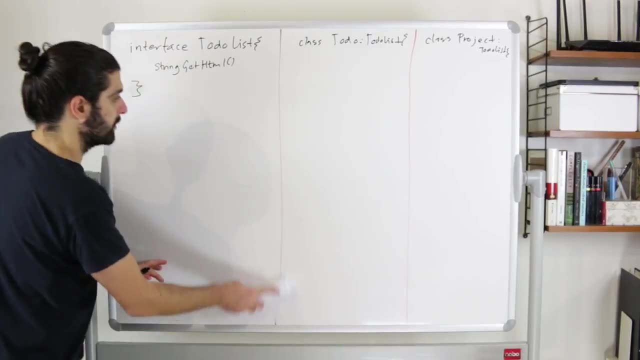 and it needs to be called get HTML And that's it for the interface. And actually this division is pretty stupid, Because if that's it for the D interface, there's no need to allocate all the space to that. So let me remove this divider here and then let's just draw it here instead. 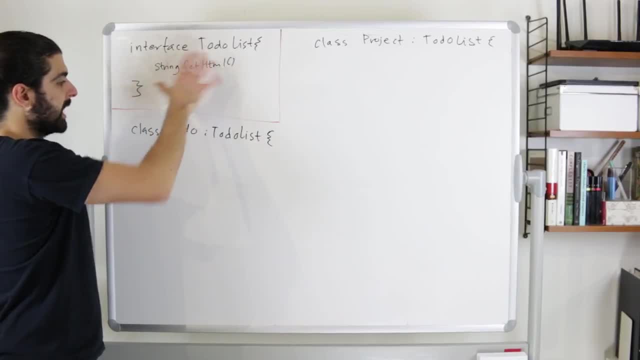 Yeah, sorry, So let's just redo this. So we have the interface to do list and then we have two classes. We have a project that implements the interface to do list and we have to do that. implements the interface to do list. 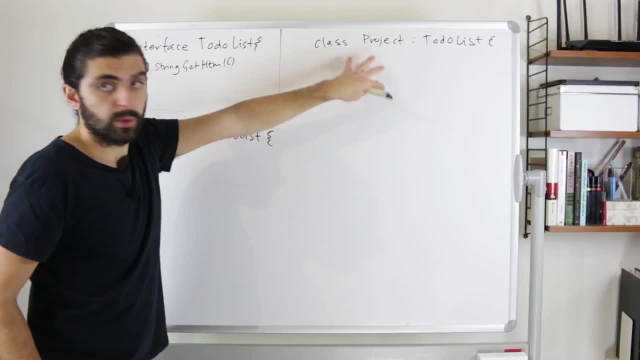 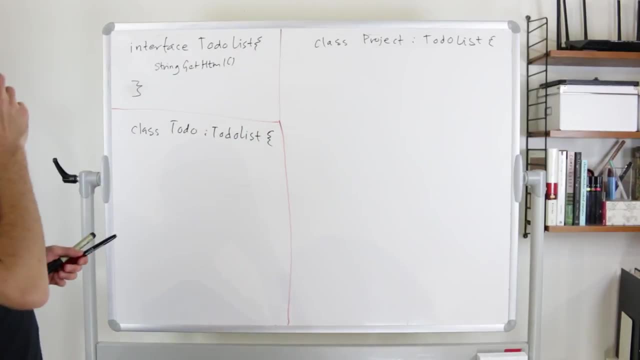 And, on the general plane, this to do is the leaf and the project is the composite And, of course, the to do list is the component. Let me extend this divider Now. what about implementations? So the to-do needs to maintain a property which is a string, and let's call it text. 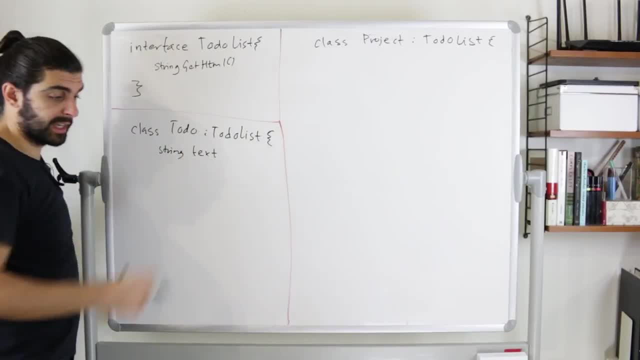 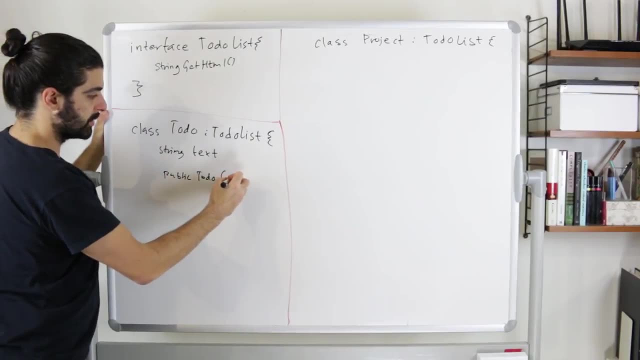 So that text is the text of the to-do. I mean it's the actual to-do, like buy milk. So then, in the constructor of the to-do, let's say public to-do, we accept what, We accept a string which is the text. 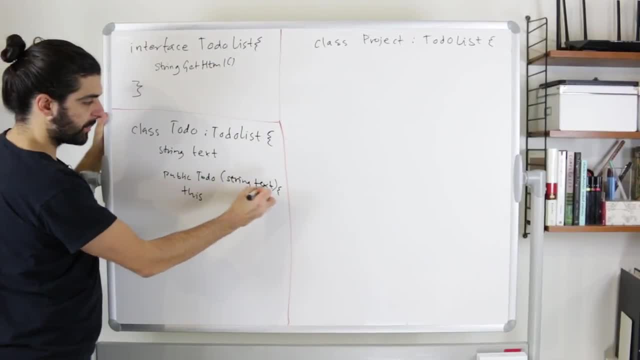 We open up the constructor And then in the constructor we assign this passed-in text to this property text of the instance to-do or of this instance variable text. So we say thistext equals the text that we were passed in And that's it for the constructor. 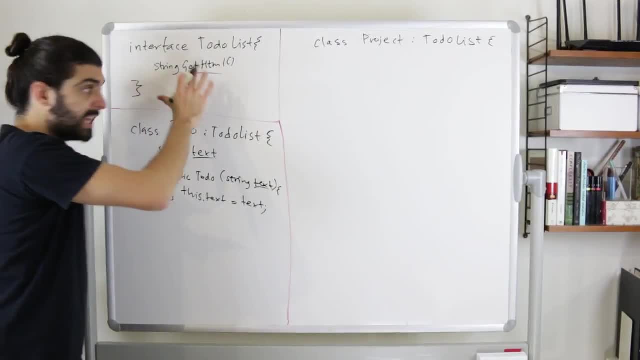 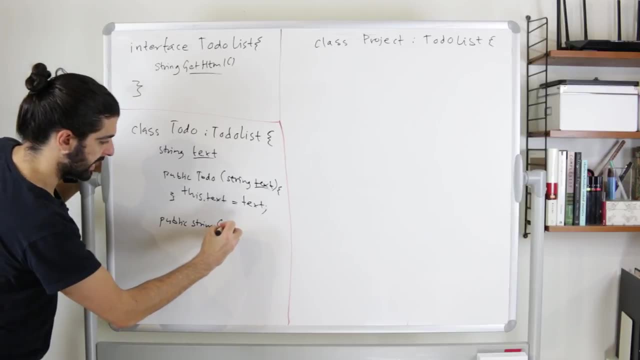 Then the crucial part: we need to implement, or we need to supply an implementation for the getHTML method. So we have a public method that returns a string and it's called getHTML. Now it doesn't take any arguments, but what's the implementation? 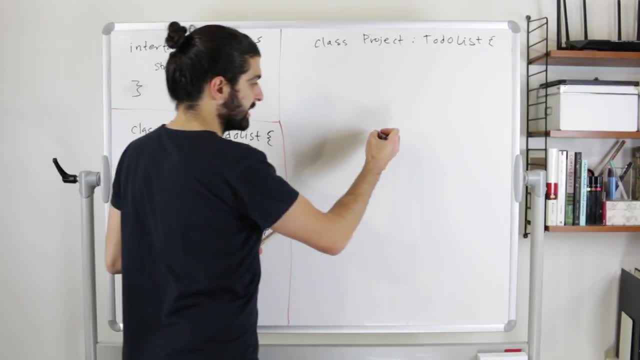 Well, according to what we talked about before, what we specified, what we said, is that it should not have to return li and then the text and then li. It should not have to return li and then the text and then li. It should not have to return li and then the text and then li. 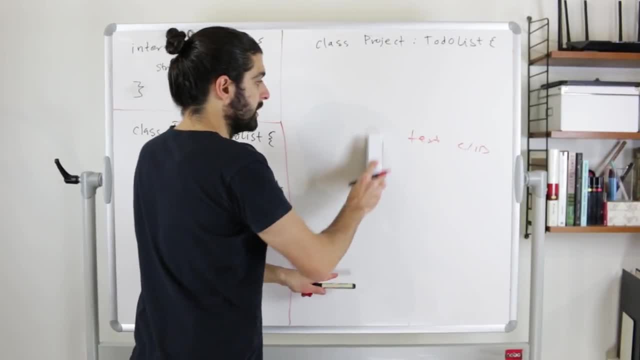 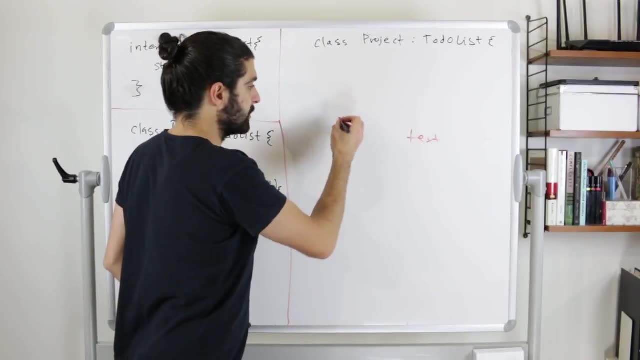 It should not have to return these elements. Instead, it should only return the text simply, And then you can imagine that what we would also do is that we would add a checkbox. So instead of just a text, we would probably have- like I can't remember what- the syntax. 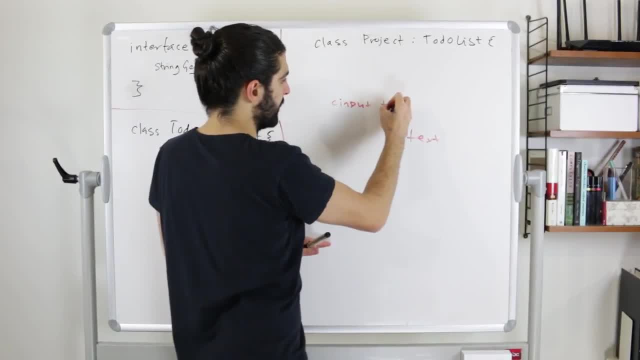 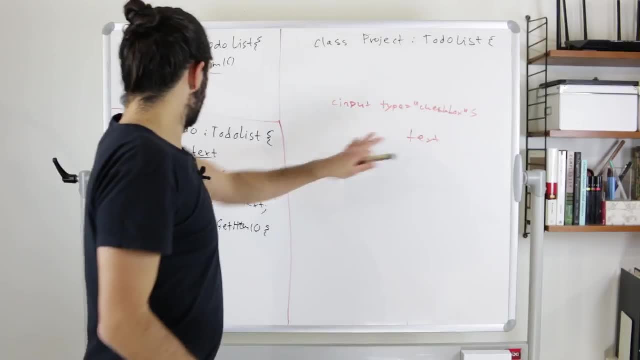 is in HTML, but it's probably something like an input tag where the type is equal to a checkbox, And maybe that's self-closing or I can't remember- and then we put the text So. but I'll skip the checkbox. 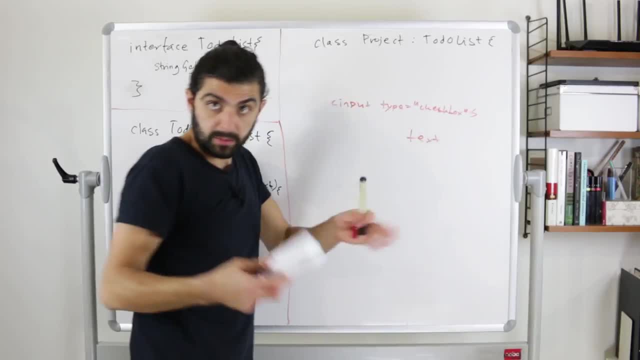 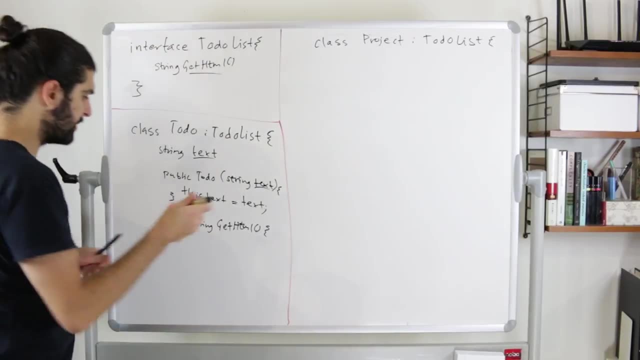 And you can just imagine that whenever we say text, we mean that Maybe we should probably have a checkbox in front of that. But if the job of the getHTML method is simply to return the text for the leaf, then that's super simple. 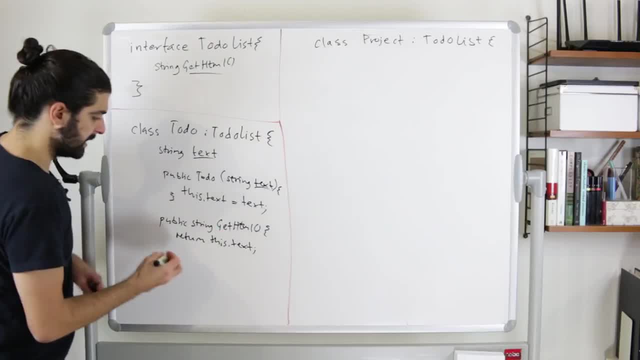 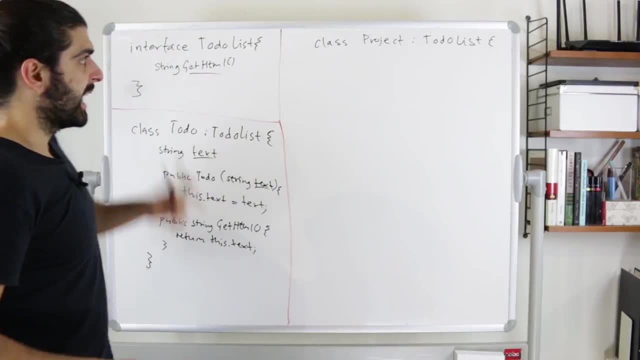 Then we just say: return thistext. That's it. Then we close this, We close the getHTML method And then we close the class, And then we're done with the to-do class. That's it for the leaf. Now to the more trickier part. 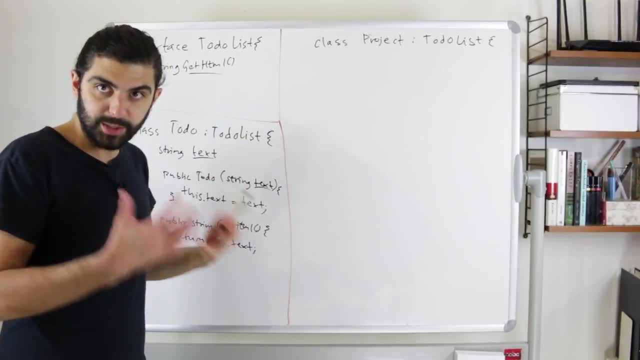 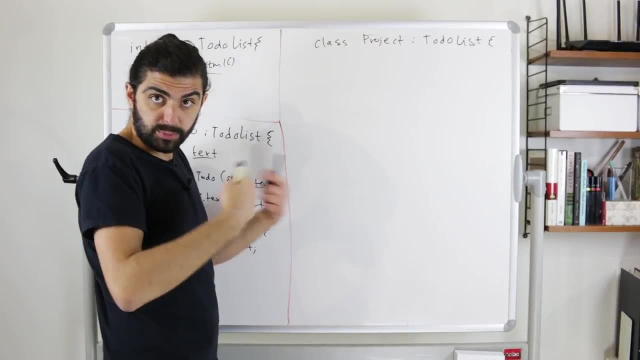 Let's talk about the project, Let's talk about the composite to-do, So in other words, a to-do that has sub-to-dos. It, too, needs to have not a text, but a title Right. A project has a title. 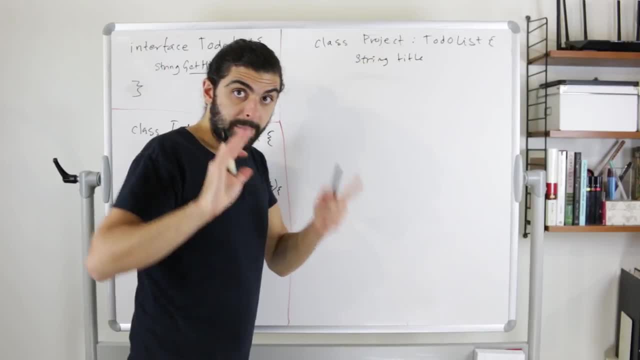 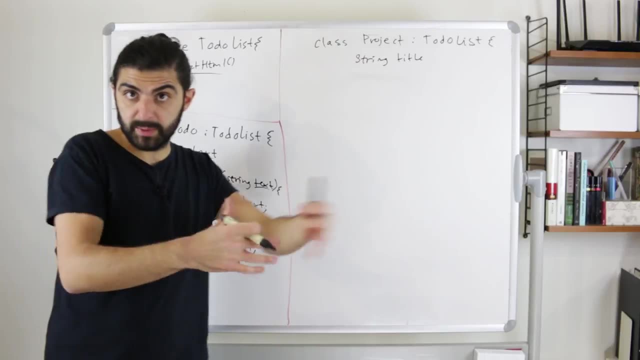 So it has a string and let's call it title. But because it's composite, it also needs another thing. What it needs is that it needs some kind of ordered collection- In our case ordered because we care about order- Ordered collection of components. 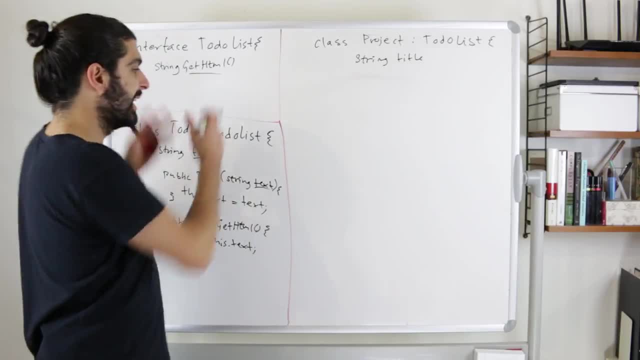 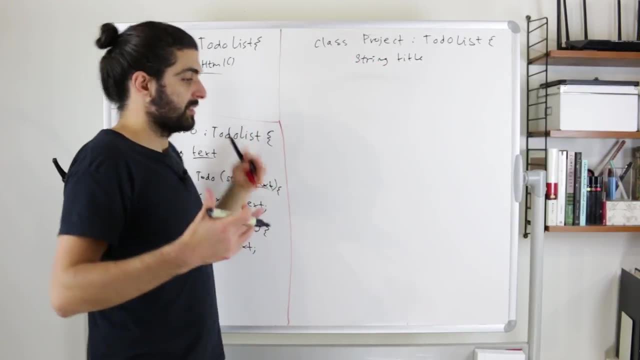 In other words of to-do lists, which by extension that means that it needs a collection of either to-dos or of projects, because both of those can behave as components or as to-do lists. So let's just say I'll use sort of C-sharp. 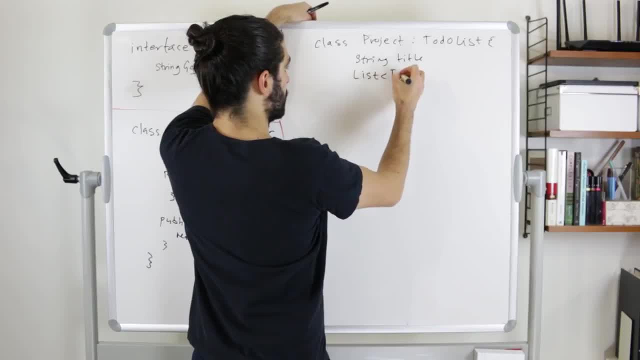 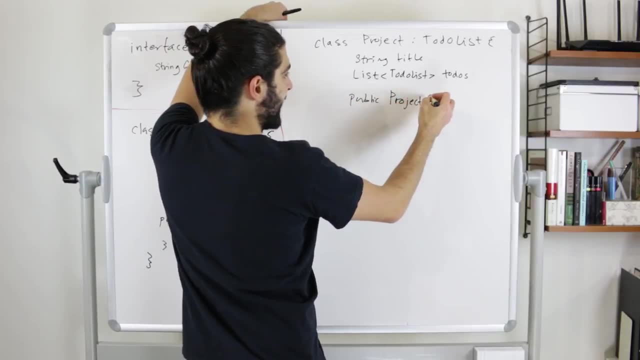 Like syntax, So we'll just say we have a list of to-do lists and let's call it to-dos. But then on to the constructor. So let's say public project and it will take what arguments? So firstly, clearly it needs to take. 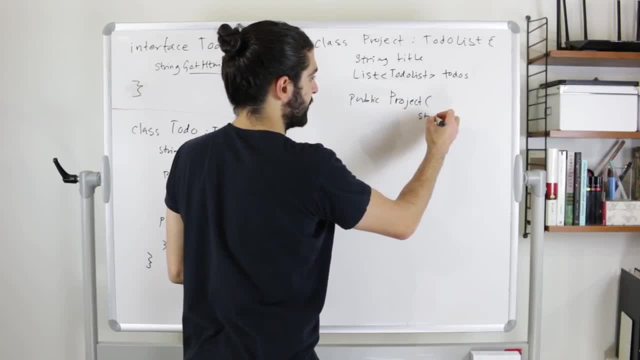 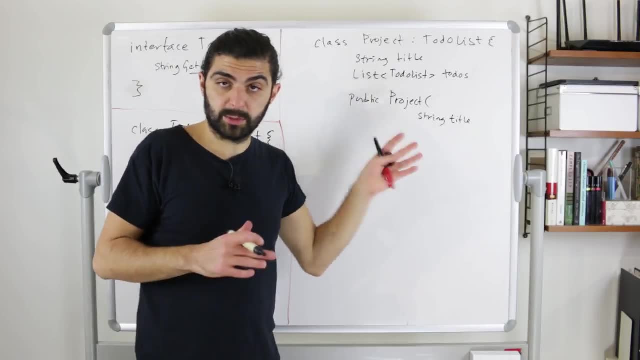 Let me do a line break here, Sorry about that. It needs to take a string that will represent the title, which is the title that we will set to this instance: variable, clearly. But now is where we get the repercussions of what we were talking about before about immutability. 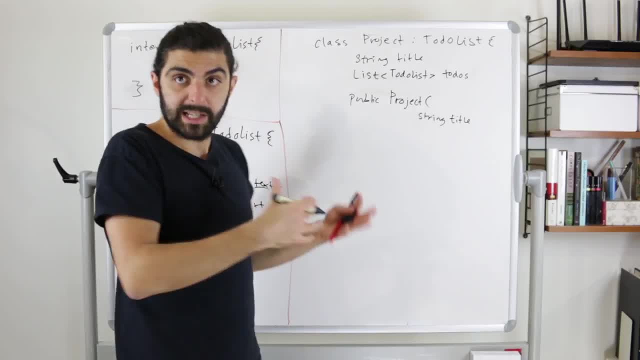 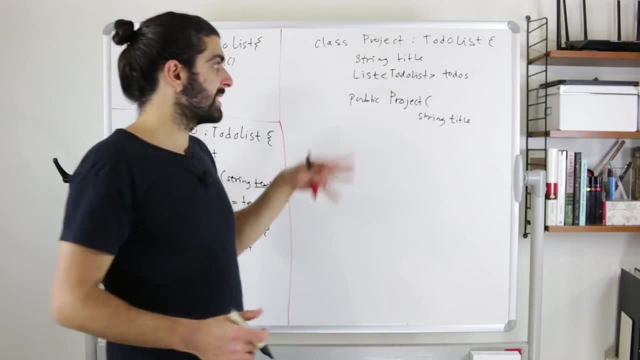 If we don't want to be able to add in Components, or rather to-do lists, after we've created this project, but rather we want them to be added from the start, That means we need to accept this list of to-do lists in the constructor. 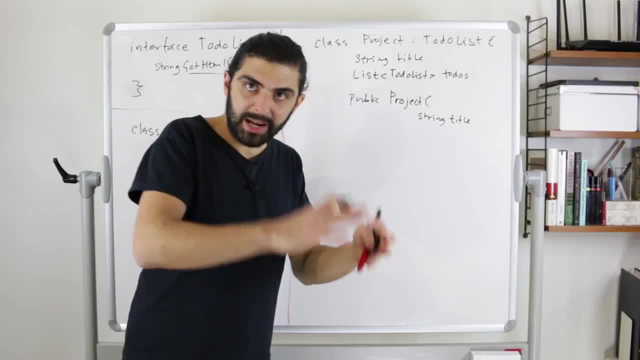 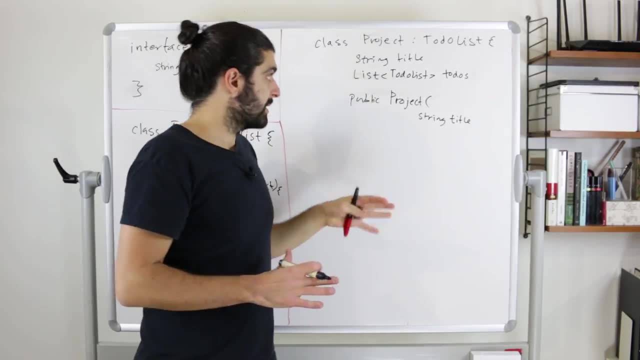 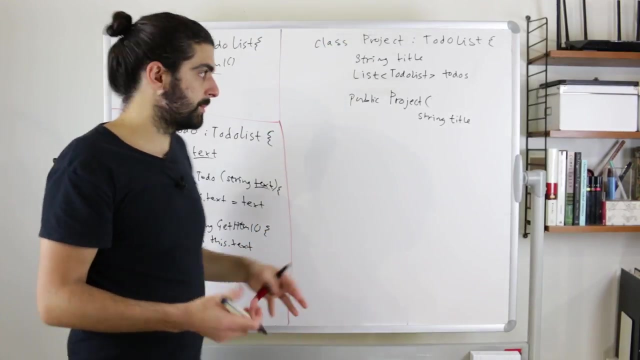 So upon construction of a project, you need to supply it with all of the to-do lists that it will contain. So we do this because then we can avoid exposing methods that you can use to mutate the contents of this list, which means that it sort of behaves as an immutable data structure. 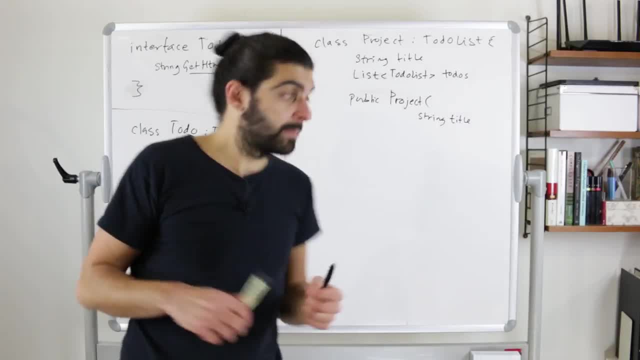 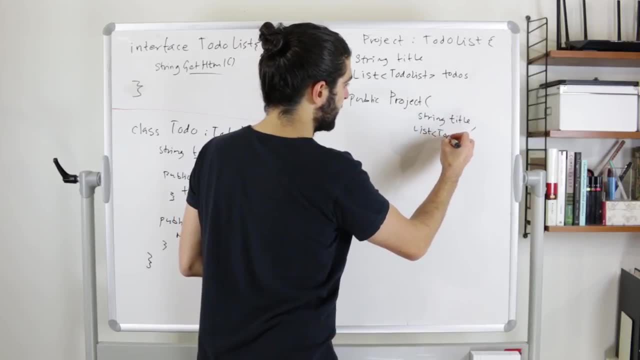 Which, again, in my opinion, is good but clearly can be discussed. So, anyways, that means that we have a second argument, not just the title, but we also need to take an argument, which is a list that will contain to-do lists. 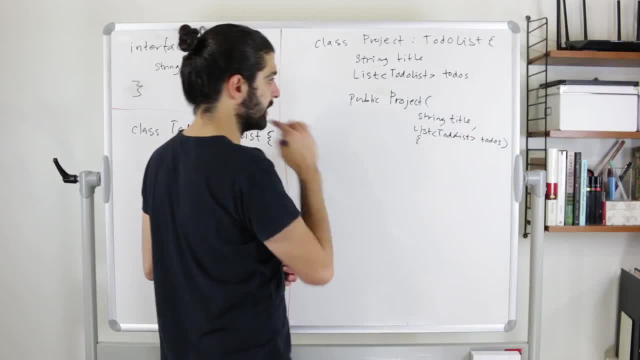 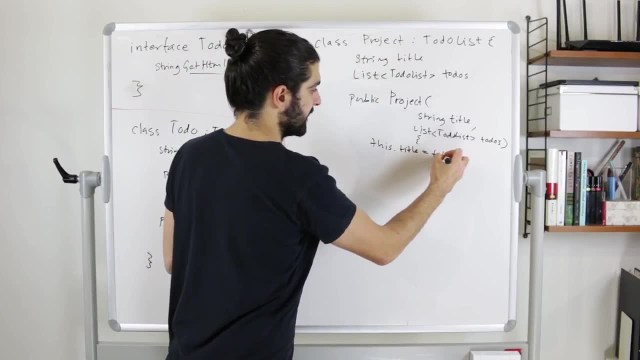 And let's call it to-dos: Close the parenthesis, open up the constructor. And then what we do in this constructor is simply that we say: OK, thistitle equals the title I was passed in, and then thisto-dos equals the to-dos that I was passed in. 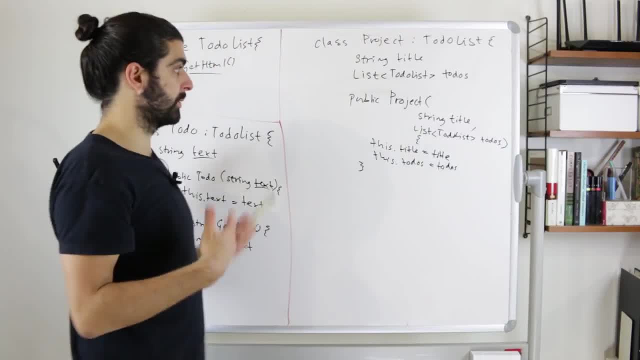 And then we close that, And then we close the constructor. And I mean, in essence, we're doing the same thing here as we're doing here: We're just assigning the values that were passed in through the constructor to the instance variables. 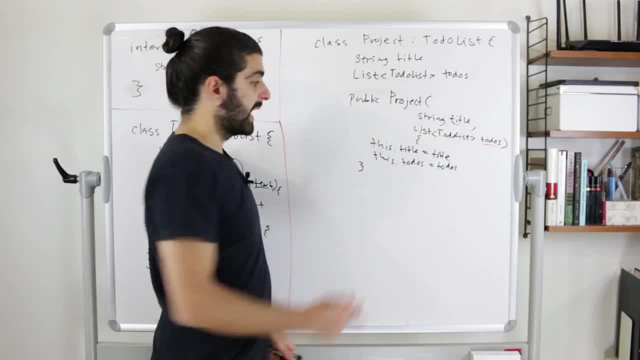 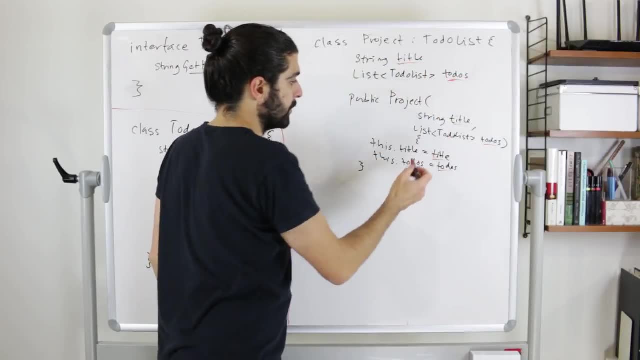 So we're passed a title and we're passed a list of to-dos And we're taking this title and we're taking this list of to-dos and we're assigning it to the instance variable title and to-dos, thistitle and thisto-dos, so that we can have access to it across this instance. 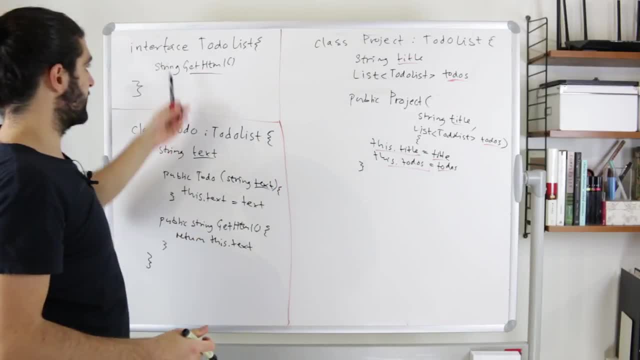 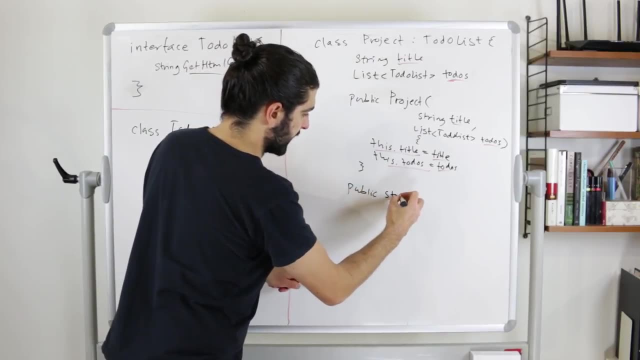 Now, that's the easy portion of the project. The more difficult portion of the project is now that we need to implement this getHTML. So let's start. So we need to have a public method that returns a string and is called getHTML. 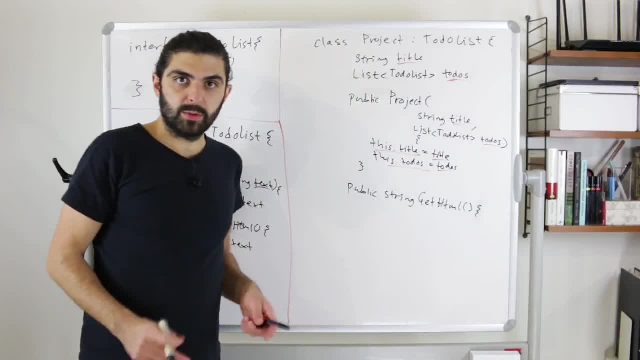 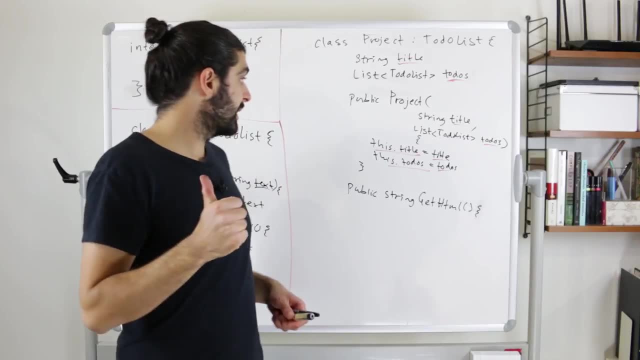 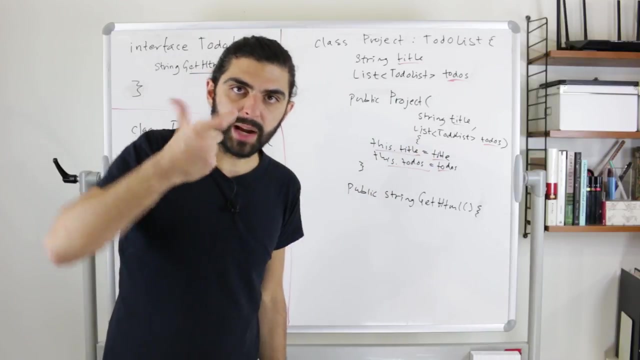 Takes no arguments and let's open it up. So what will this implementation do? Well, what we said that it will do is that it's responsible for printing the UL and then printing the HTML of every item, every to-do list that it has in its list of to-dos, but wrapping all of those within LIs. 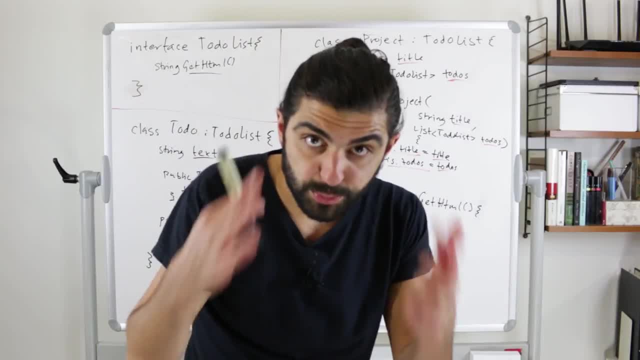 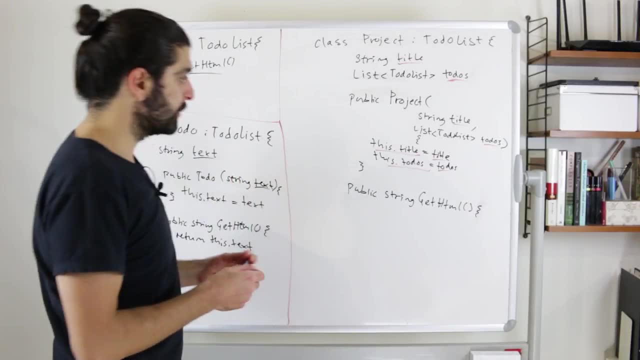 Because, remember, the to-dos didn't print their own LIs, So the project must be responsible for printing not just the UL, but also the LI. So how do we do this? There are clearly more elegant ways of doing it, but I'm just going to do it in the most simple fashion. 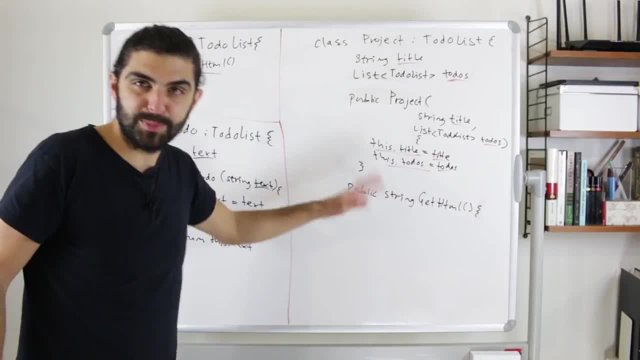 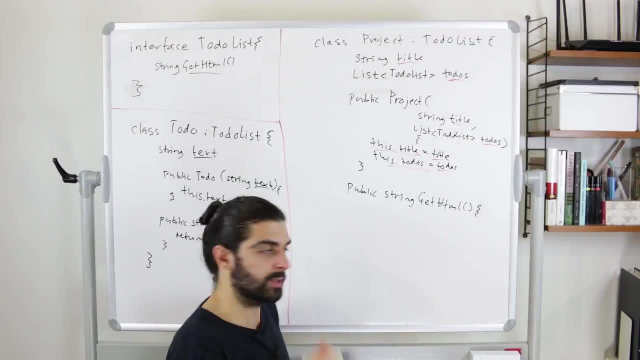 And again, I just talked about immutability, but I will use immutability in order for this just to be as simple as possible. What I'm trying to say is that you would probably use a map here rather than a forEach, but we're just going to use a forEach. 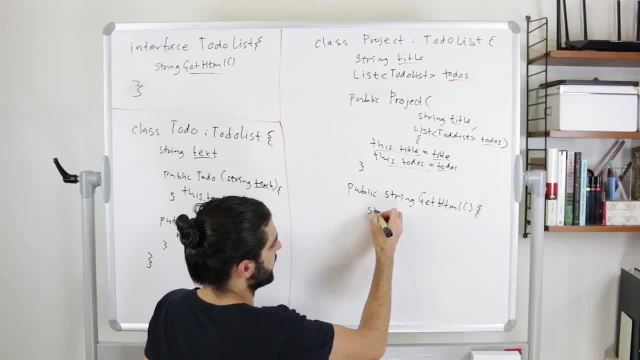 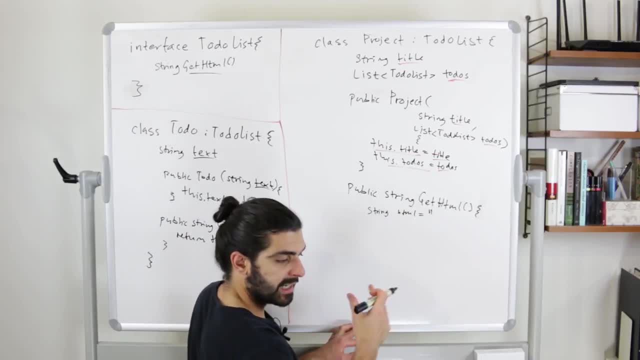 So we know that it will contain some things. What we know that it will contain is that we know it's a list, so we know that we need the UL element. Then we know that it has a title, so that means that we need the LI element. 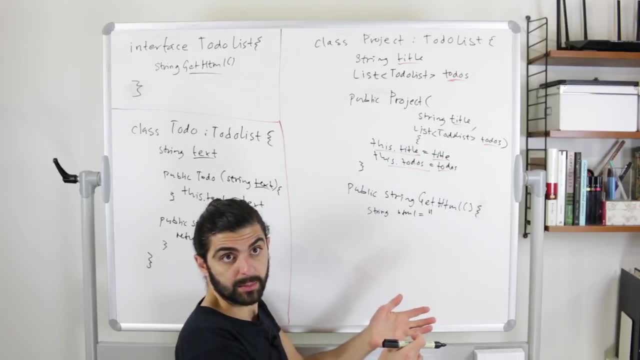 And then we know that we have a title, so we need to add that to the LI element. But then within this LI element we need to add a sublist containing all of the LI elements. So actually I'm getting a bit confused now about whether I drew it incorrectly before. 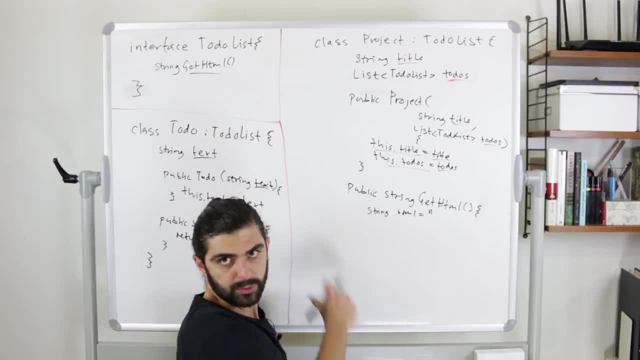 Let me write the correct implementation as I'm thinking about it now, and then let's draw up the LI UL example again when we see this output, in case I drew it incorrectly before. So if you have a list, it necessarily has to be a project. 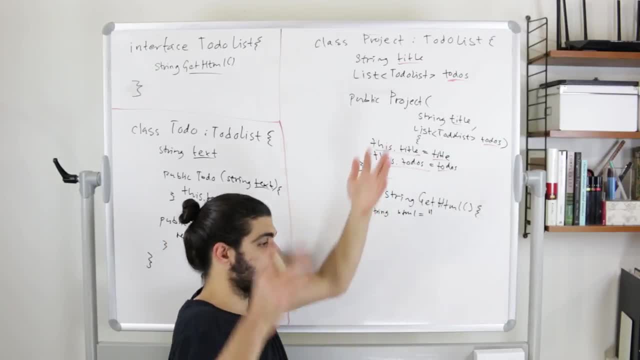 So, like the full to-do list, if you have only a flat to-do list, it will be a project. It would be like the project of my life or whatever, like all my to-dos, that project. So that means that we start with UL. 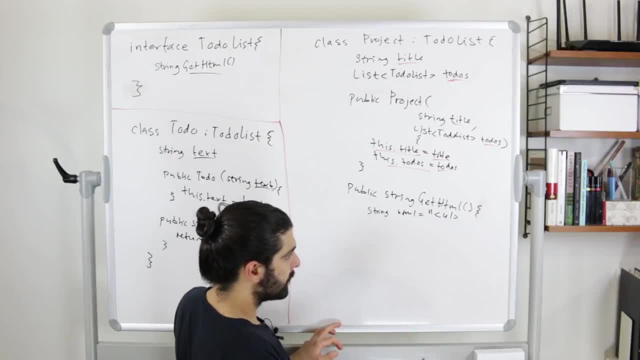 So we start with the UL tag and then we want to add the title. But in order to add the title we need to have the LI tag, because that's the first element. So we add the LI tag, then we close this string and then we want to add the title. 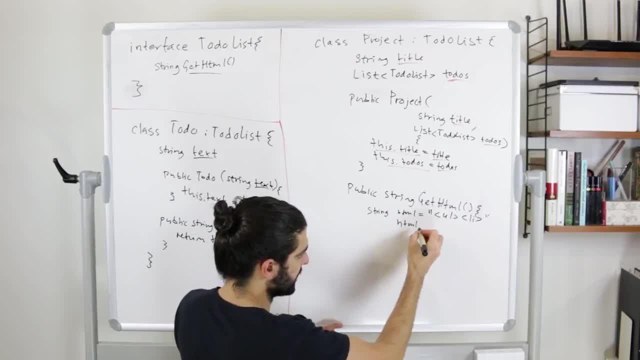 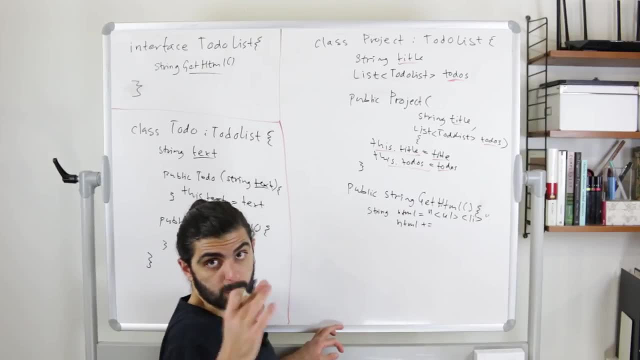 So then let's concatenate into the HTML. So we add the HTML variable into the HTML string. so I'll say plus equals to denote concatenation. So HTML after this line will be equal to whatever it was before, plus this new thing that we're adding in. 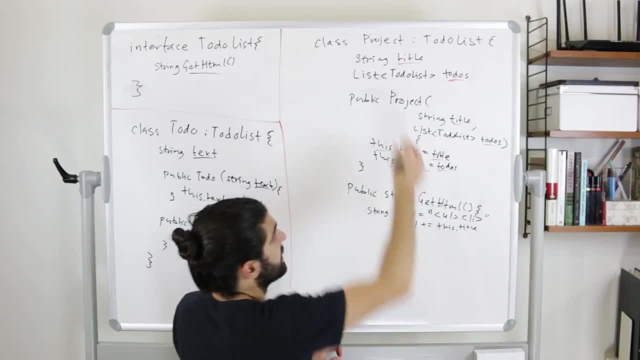 And what we're adding in is this dot title. So the title that we've gotten, that we've been passed in through the constructor and now saved to the instance variable, we're adding that into this locally scoped HTML variable that contains the UL and the LI opening tags, but nothing else. 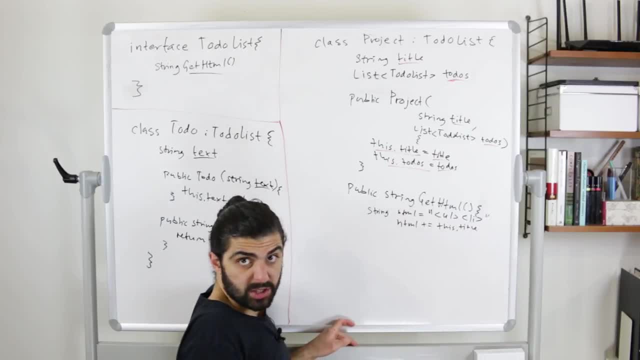 It's a project, so it might contain to-do. So what do we need to do? Well, essentially we need to iterate through them. So let's say forEach. now we can't say to-do, because that's a specific type. 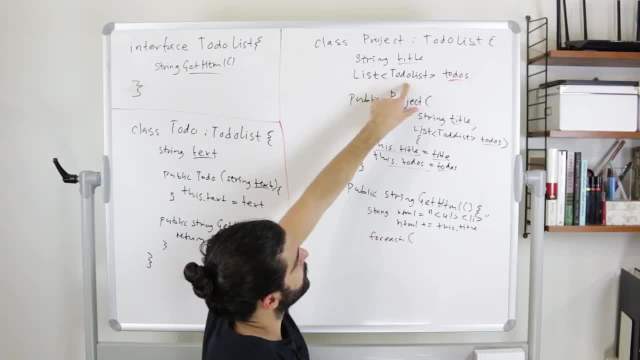 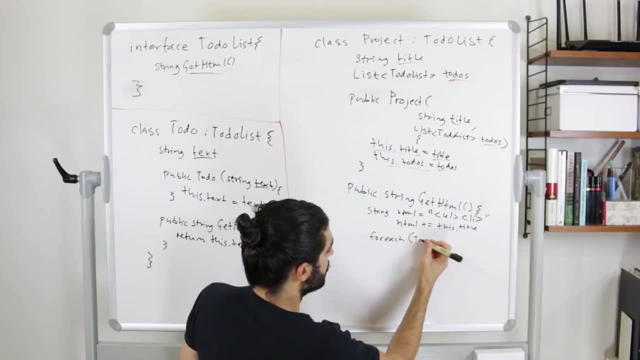 and we can't say project, because that's a specific type, because what we know is: we know to-do list, We know the general type that both of them can have or that both of them behave as. So we say for each to-do list, let me just call it TL in thistodos. 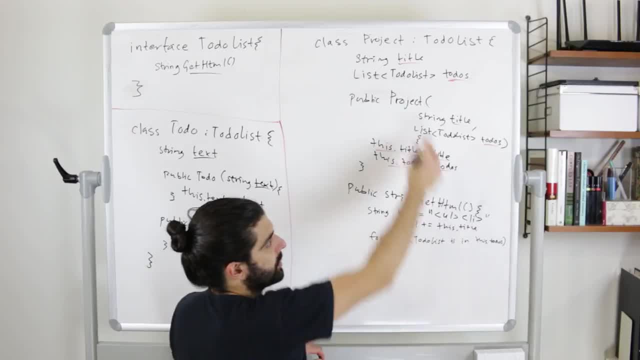 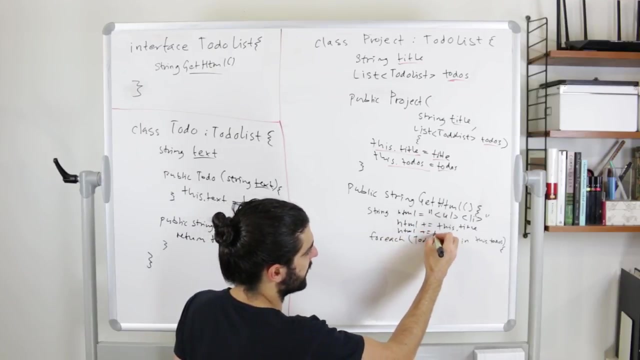 Thistodos. It's a bit of funny naming here. I should have called that to-do lists, but sorry about that. So for each to-do list TL that we call TL in thistodos and then we open this up. Ah, sorry, what I forgot is before this we need to add, we need to further concatenate into the HTML: 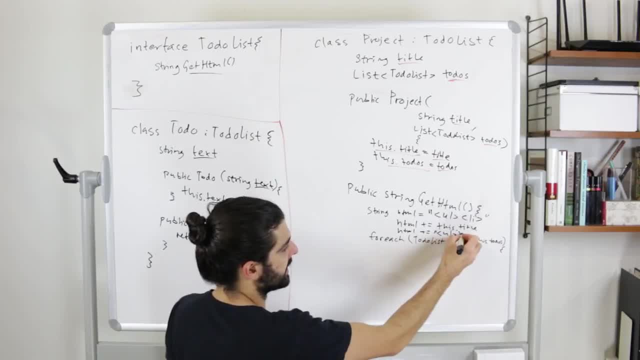 another UL element. right, because now we're opening up for adding in more list items. So we add UL LI, the title, and then another opening UL tag, Then we start to iterate, and then for each of the things that we find in this list. 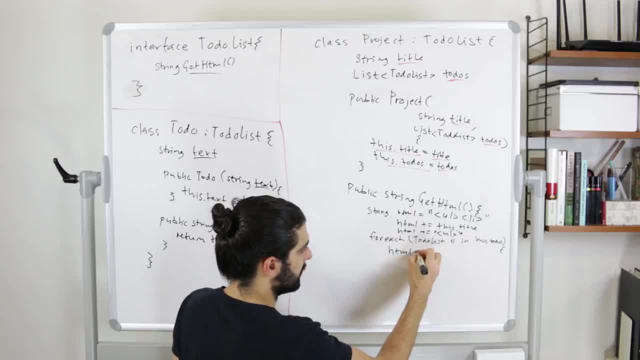 what we do is that we further add to the HTML string HTML plus equals, and then we add first an opening LI tag. Let me do this on separate lines to make it super clear: HTML plus equals. here's the super crucial part. 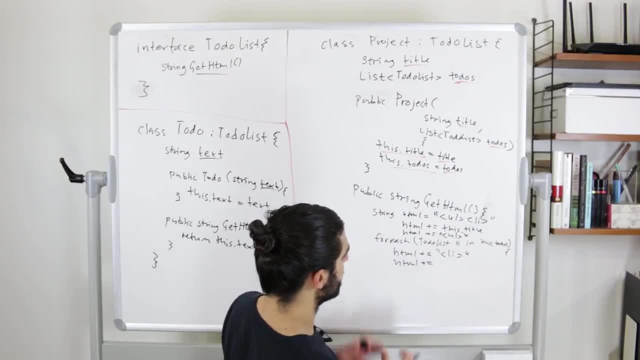 Here's the recursion. This is where we to this HTML string add: we concatenate whatever we had in the string before, In other words, HTML with TL dot get HTML. In other words, we concatenate To whatever we had in the HTML string before, into that we add the result of calling getHTML. 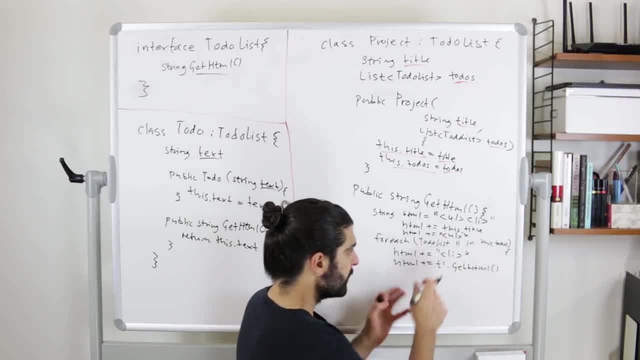 on this particular TL, and this particular TL, of course, is the variable name that we chose for this variable of type to-do list. that is the one we are currently at in our for each iteration over this dot to-dos, In other words, think about it. 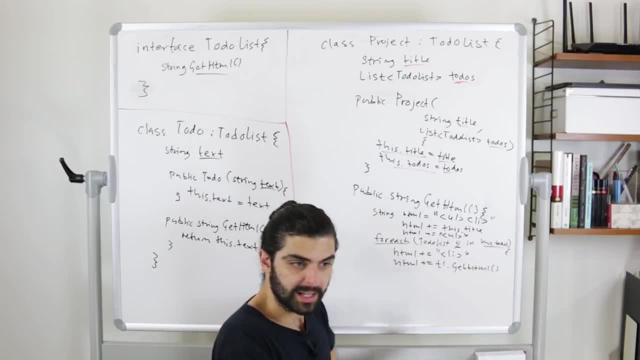 The project is a composite of to-do lists. It's not just a single to-do, It is. It is a composite of to-do lists, which means that it may contain projects or it may contain a single to-do. So when we say for each to-do list, TL in this to-dos we will step by step get a hold of, or I should say 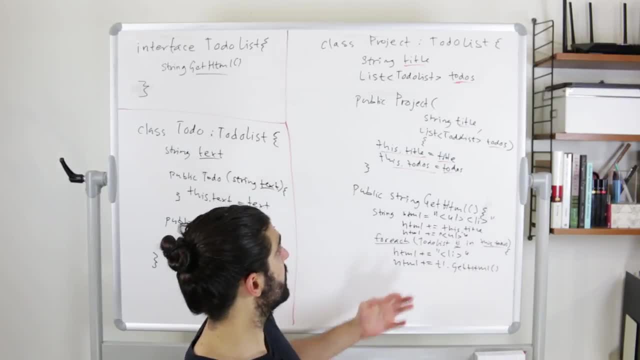 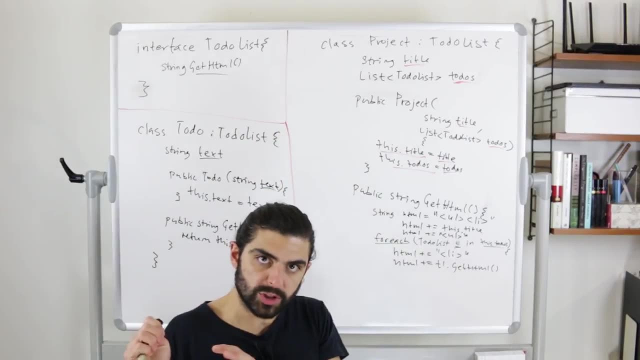 one by one get a hold of through this iteration, get a hold of individual to-do lists, And these to-do lists are either individual to-do items or they are projects. So this project may either contain a series of to-dos or a series of projects that have to-dos. 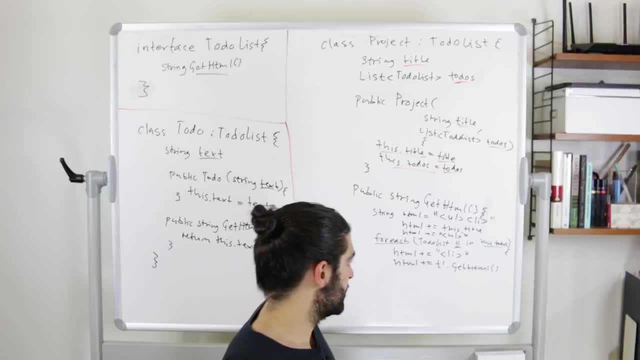 or any mix of those. And again this is where the recursion comes into play. So when we call getHTML on this particular to-do list, then that to-do list, if it is a to-do, then it will simply print the text of that to-do. 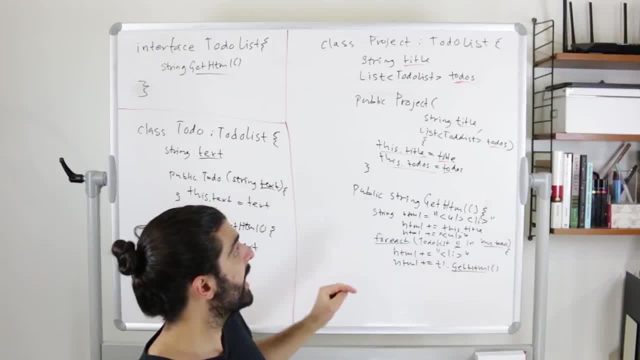 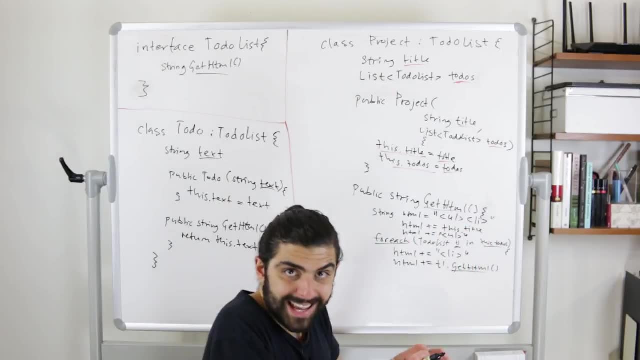 But if it happens to not be a to-do, but rather if it happens to be another project, then we will end up in the getHTML method of project again. this is what we talked about before when we talked about recursion. We will end up in the same function, in the same getHTML method. 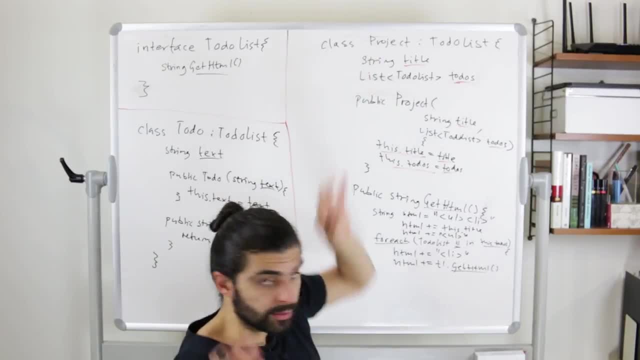 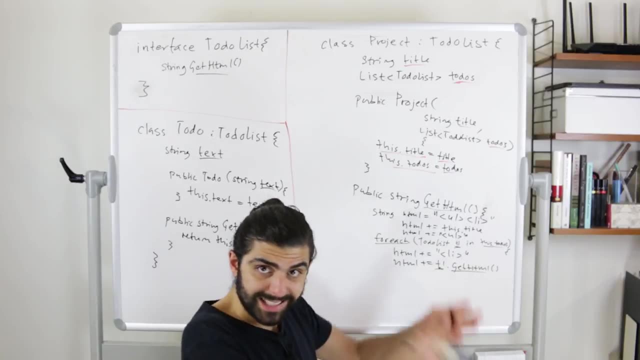 but in another instance, which is this other project instance, which is this TL, And that instance in turn can have a bunch of to-do lists in itself, And so when we call getHTML on that, that might cause us to call getHTML on all of its children. 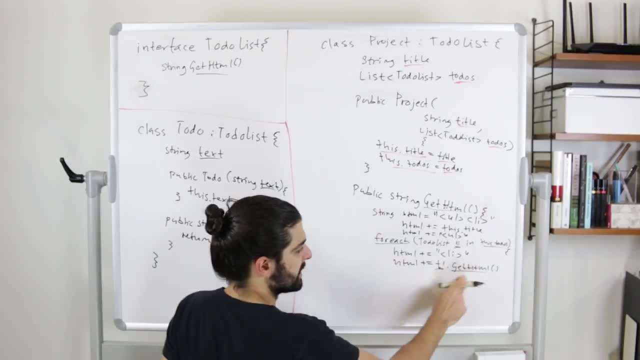 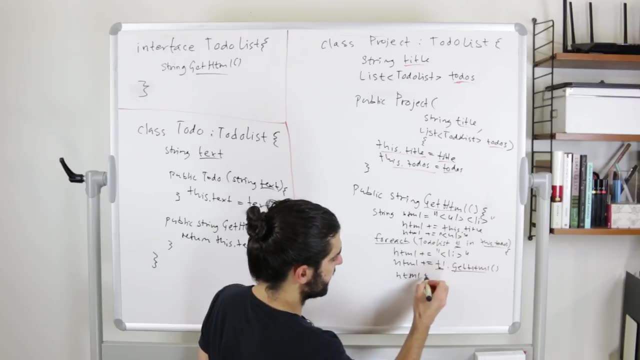 and so forth, and so forth and so forth. We're digging our way down. So, essentially, we call this getHTML here and concatenate it into the HTML string. What else do we need to do? Well, we need to sort out the HTML here. 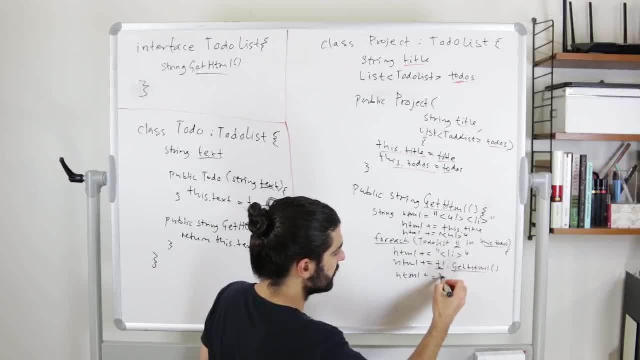 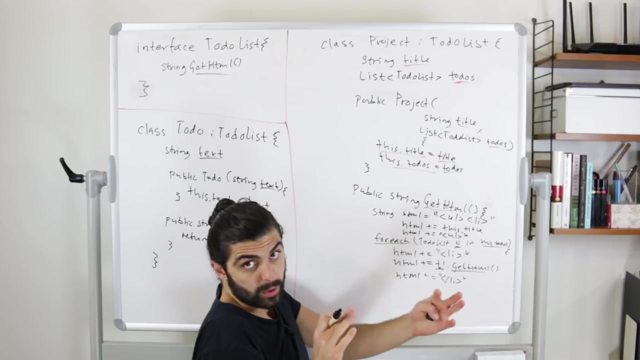 We need to do some closing tags. So after we've gotten that HTML, we need to close this li tag. So now we're closing this tag, right? We're closing the list item tag that encapsulates this particular item in the to-do lists that we're iterating over within this project. 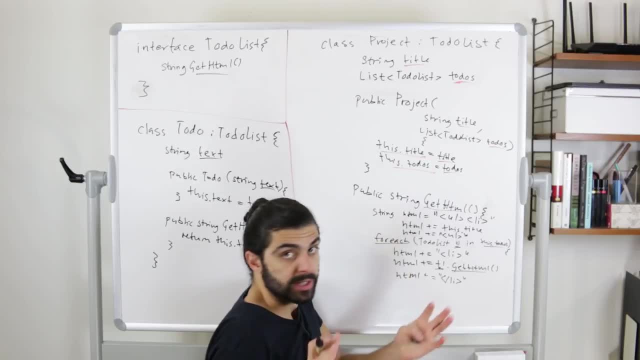 And again, this to-do list might be so in the simple case, these to-do lists would all be to-dos. So we are in the project and we are iterating over all of the to-dos that we have and we wrap them in li's because they are to-dos. 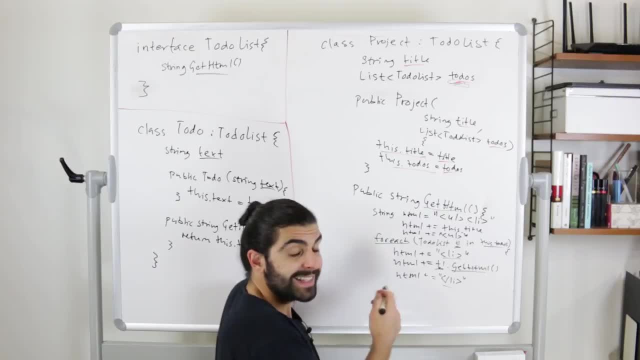 They are items that need to be displayed separately. But again these might turn out to be projects rather than just to-dos, and then we will recurse again, because then we will call getHTML and run this method again, but within the context of that project rather than this project. 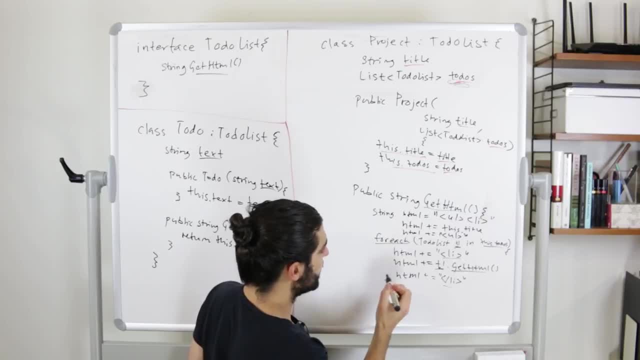 But anyways, we close the li tag here And then we close the forEach, because then we need to stop circling around all of these to-do lists, because we're done with what we want to do to each to-do list And then some more concatenation into the HTML string. 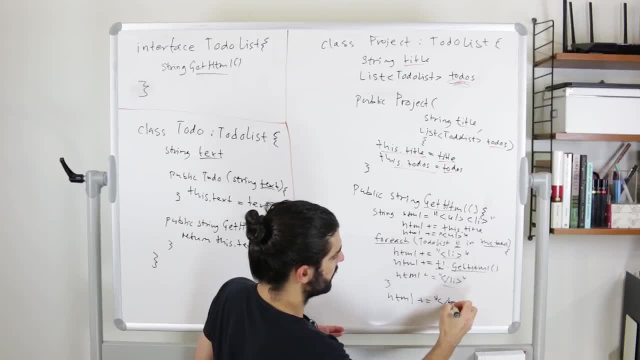 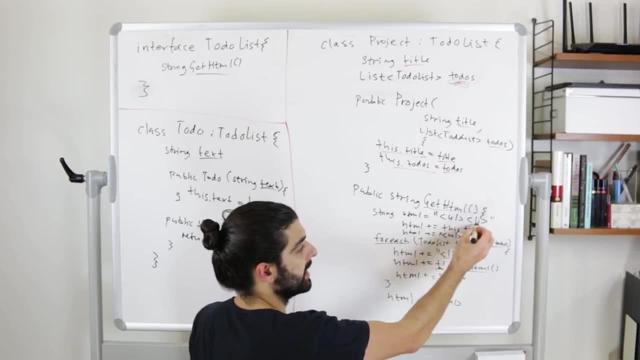 So we concatenate another string that closes the ul tag. Now we're closing this tag And then we need to- I'll do this on the same line- we need to also close this li tag that contained the title, essentially, And then we need to close the outer ul tag, the first ul tag. 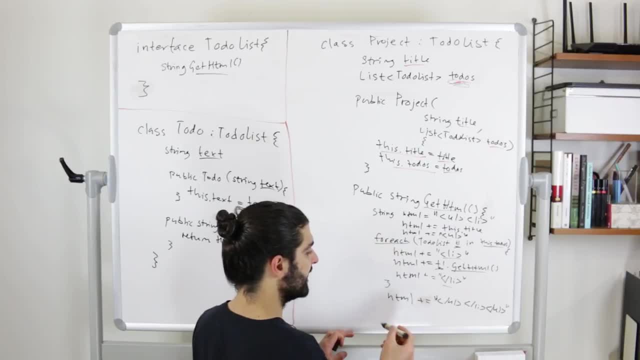 That we had here, And then we're done with the HTML, And then we can simply say: return HTML. So we will return this massive string that we've constructed and we'll close the getHTML method and we will close the whole class because the class is done. 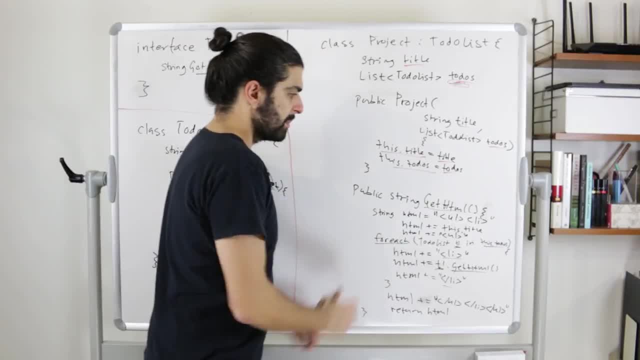 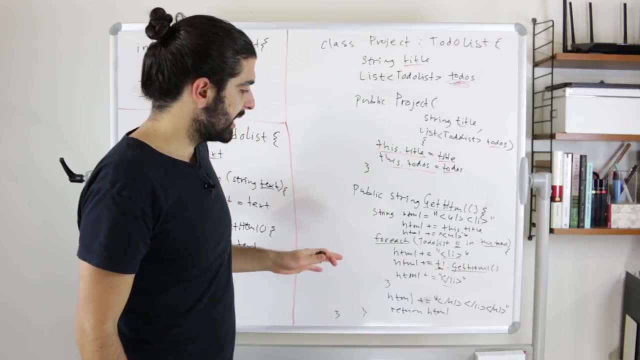 And now actually I'm realizing back to this point where I said that maybe I did it differently with the ul's and the li's than what I explained over here before when I drew up the HTML. Actually, it's completely unnecessary to say that the title- let me emphasize this- the title here. 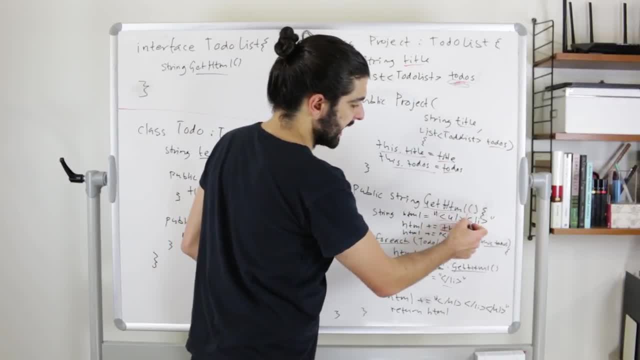 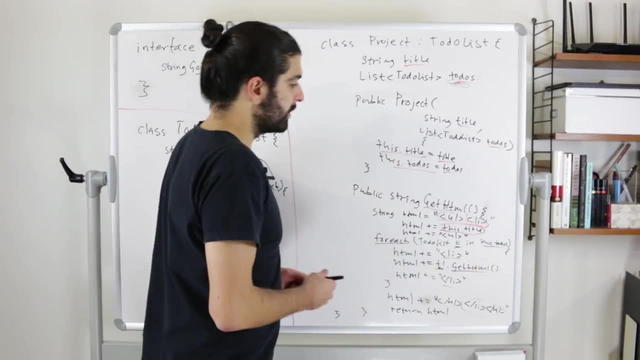 that I wrapped this within a list that had a single element that I then have to close here and here. I mean that's actually completely unnecessary. Probably what we should do is we should just skip this right. There's no outer ul element. 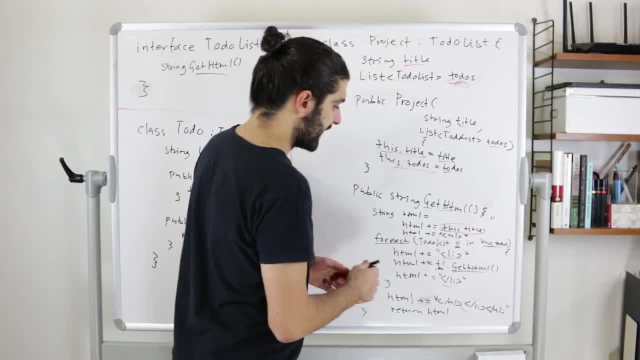 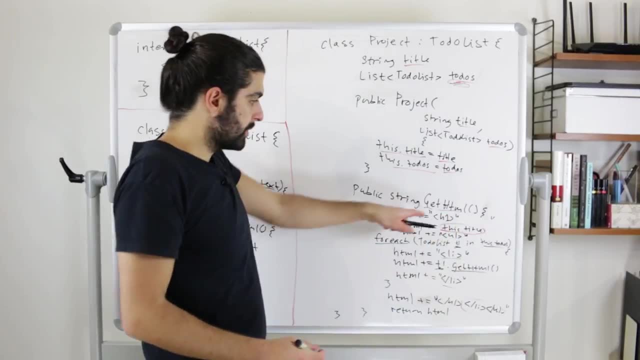 Sometimes it's really tricky to think about recursion. So what I would do instead, I guess, is just we would maybe put an h1, let's say right, So we make it a header like a proper title, So it's an h1, then we add the title. 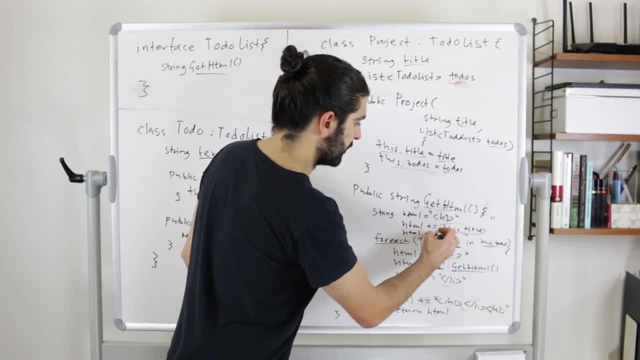 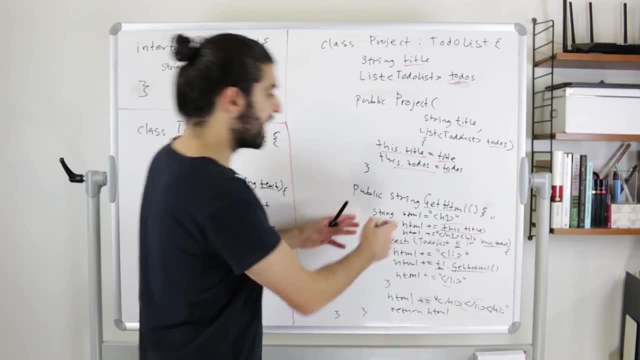 and then, instead of just opening the ul, let's think about it- then we immediately close the title, we close the h1, and then we open the ul. so we open the unordered list and then we're into this foreach thing where we're printing li's. 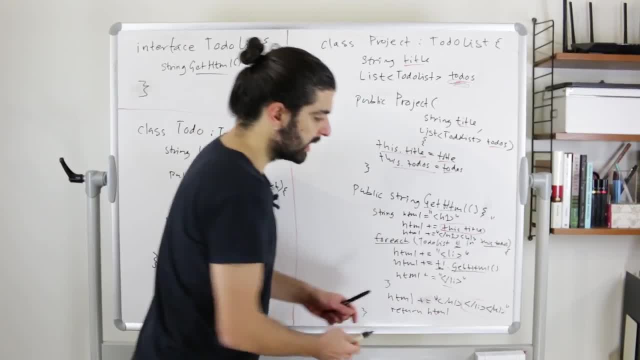 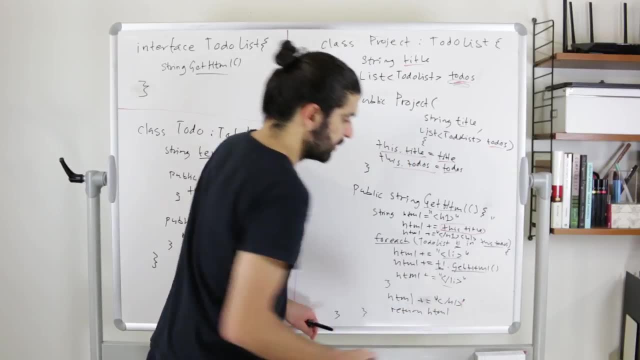 and then we are here when we're out of the foreach, we are closing the ul, but then there is no need to, as we were saying, close this li and close this ul. This actually makes a lot more sense. So we just close this ul of todos. 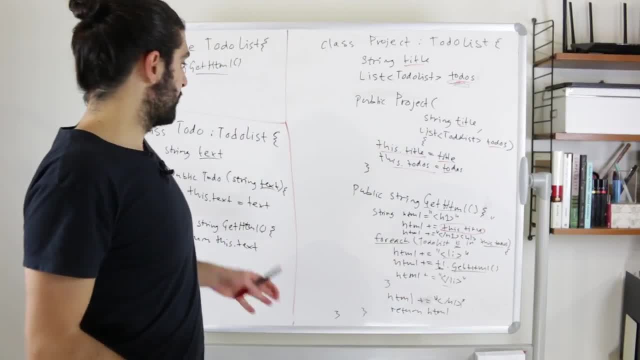 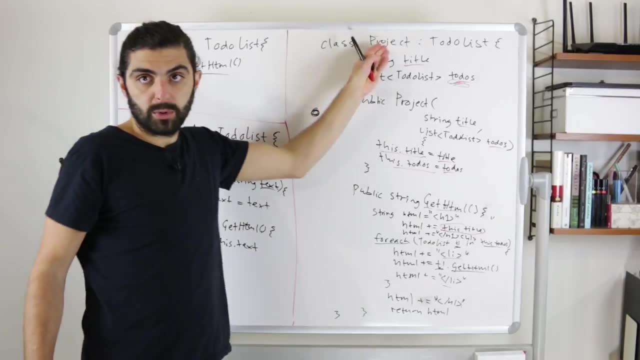 And, if you think about it, I mean that kind of makes a lot more sense, because what we were saying before is that if you have any particular instance of something that is of type todo list, it can either be a todo or it could be a project. 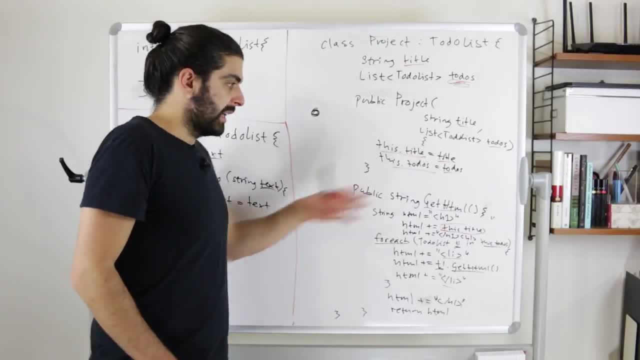 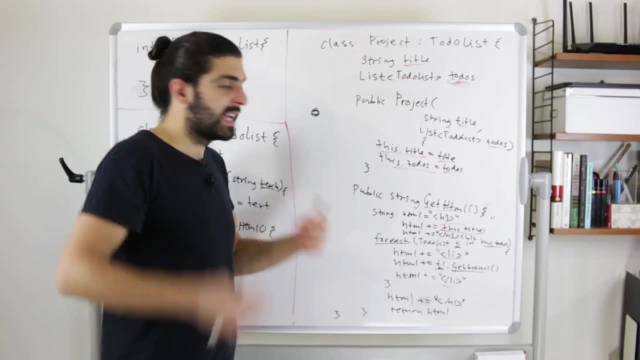 And if it's a todo, it just has a text. But if you have a project and you ask it for its HTML, it will begin by printing the title wrapped within an h1, which, I mean, kind of makes a lot of sense. 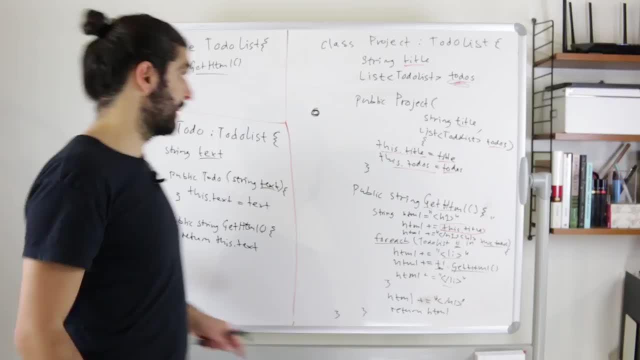 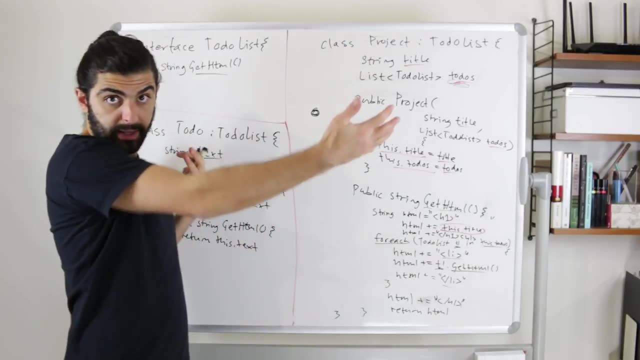 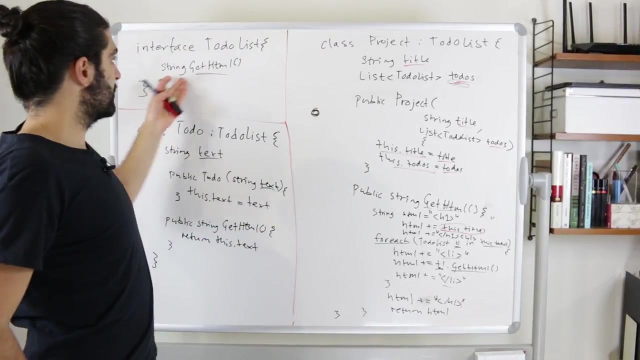 and then it will print the list. So that's it, Super quick recap. There's an interface called todo list that both todos and projects implement, So todos and projects can be used interchangeably. Adhering to the notion of a todo list simply requires that you implement a method. 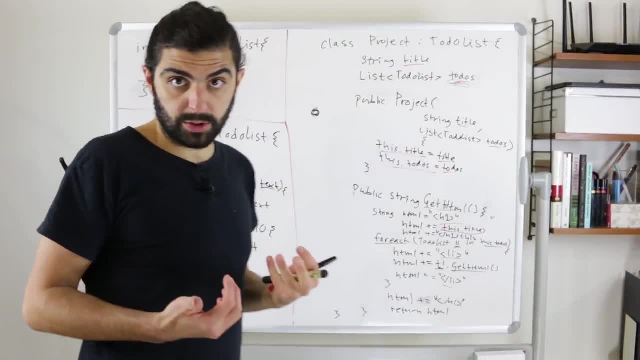 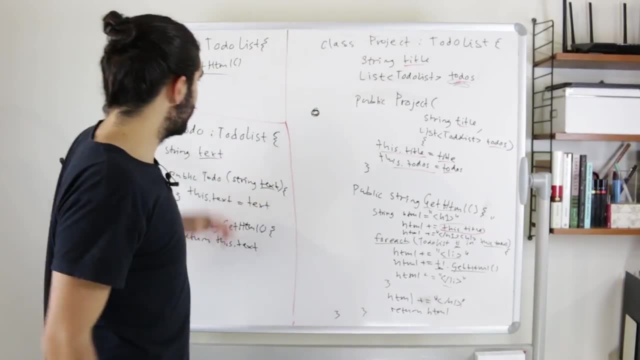 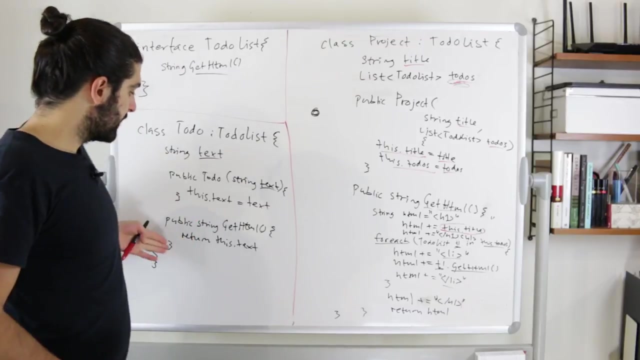 that returns a string and is called getHTML. It takes no arguments. And then, of course, these two classes, the todo class and the project class. both of these have implementations for the getHTML method, And the implementation in the todo is simply that it just prints the text. 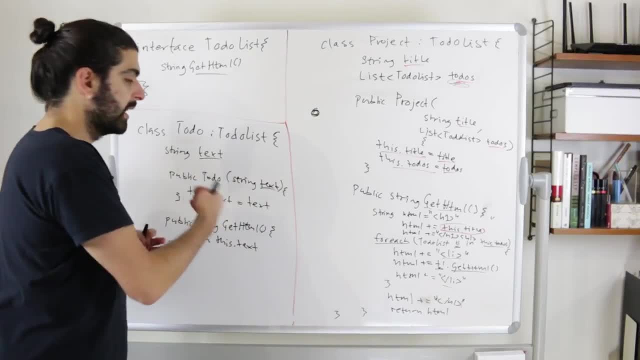 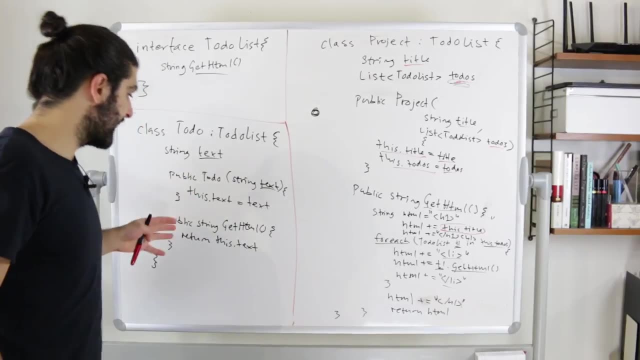 of this particular todo. So in the constructor of the todo we take a parameter, which is a string, which is called text, which represents the text of the todo. We take that into the instance of the class And then, when we call getHTML, we simply print that text. 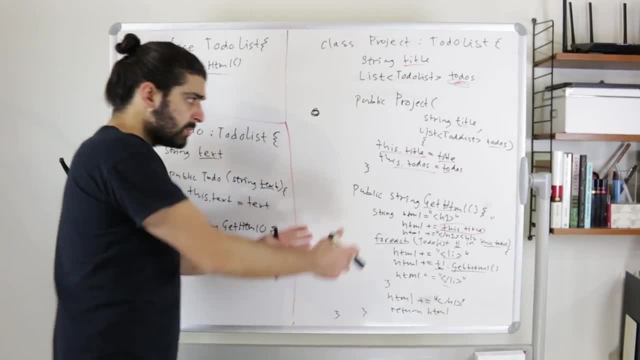 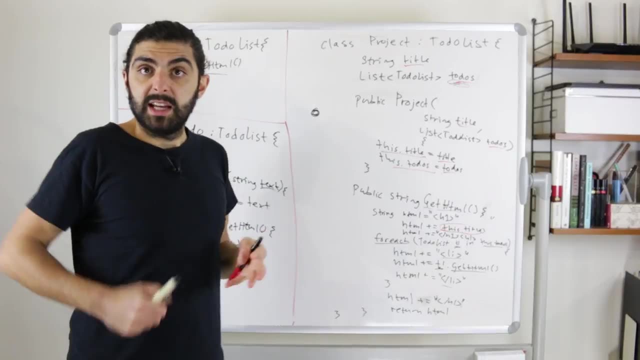 Or sorry, I shouldn't say print. We return that text- As opposed to the project, which is a little bit more complex, because the idea of the project is that the project is a composite todo list, In other words, it contains not only a single todo, but it contains multiple todos. 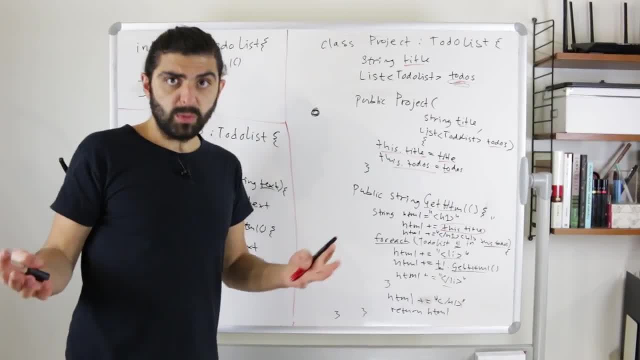 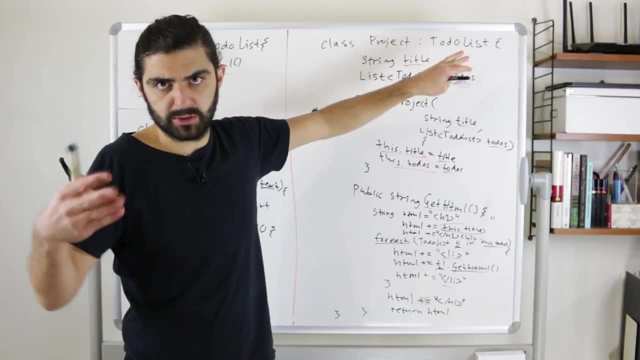 And actually, by extension, multiple projects, if you want to. To be more specific, the project is a todo list, behaves as a todo list. Sorry, not is a, because of interfaceness. I mean it behaves as a todo list. 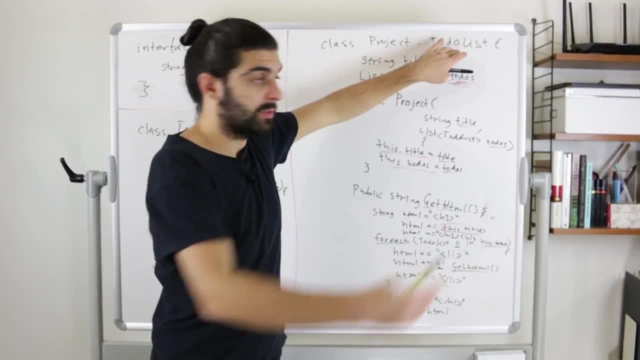 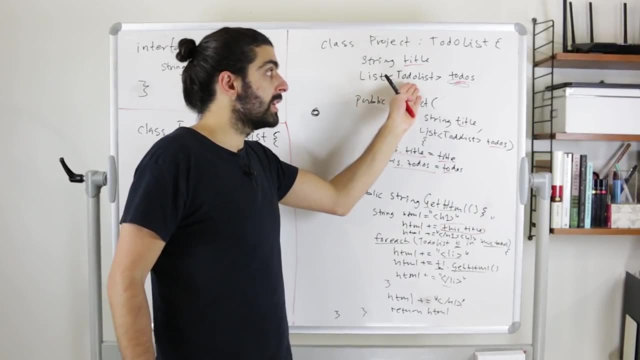 It responds to the interface todo list, So you can think of it as is a todo list. But it also has todo lists And in this case we implemented that by saying that it has a list of todo lists And we call it todos here. 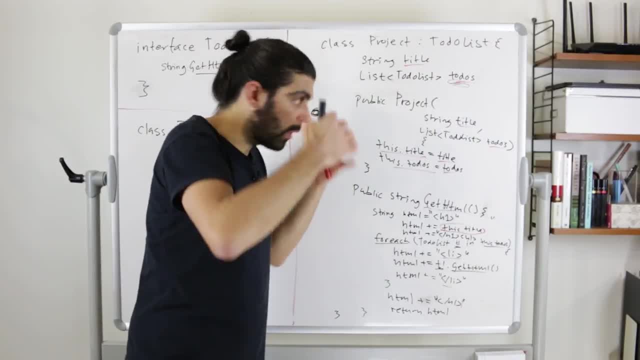 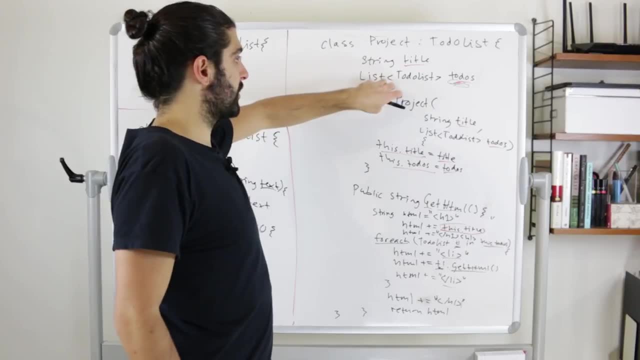 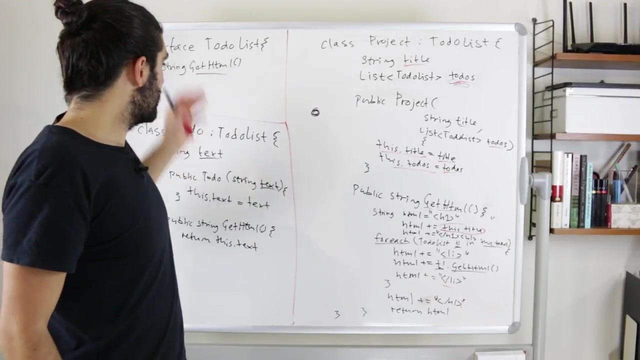 Either way, this project class, then again, is a composite todo list, So it contains multiple todo lists. So we said that it behaves as and it contains multiple todo lists, And because it contains multiple todo lists, that means that, since every todo list can either be a single todo or another project, 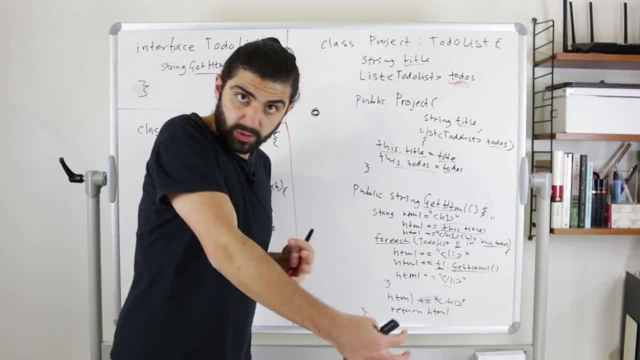 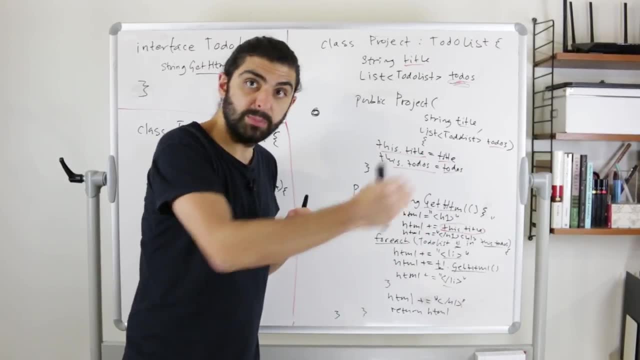 that means that we can infinitely nest projects within projects, Because if projects behave like todo lists and if projects can contain todo lists, that means that projects can contain projects. So somehow then, when we ask a project for its HTML, it's not as simple as with a to-do. 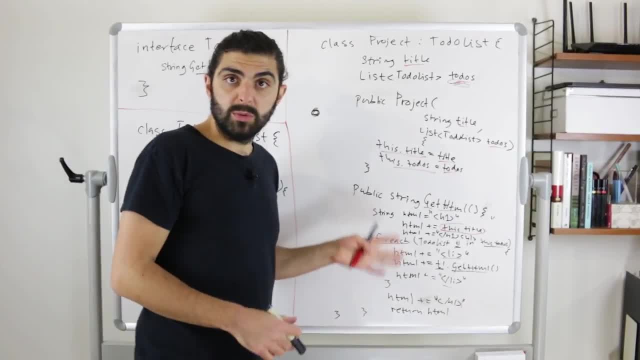 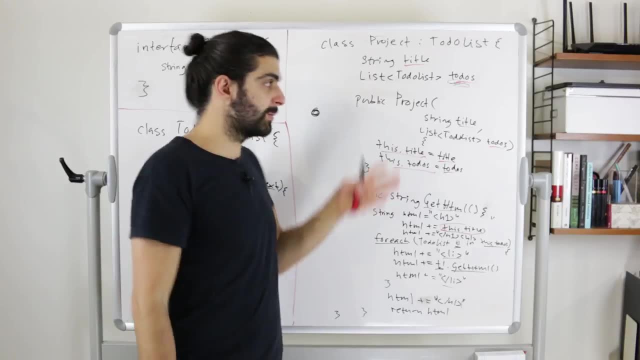 where we can simply print the text of that to-do. What we have to do is we print the title. so it's the text of this project, but we call it the title. Sorry, now, I said printing again, but again I mean returning. 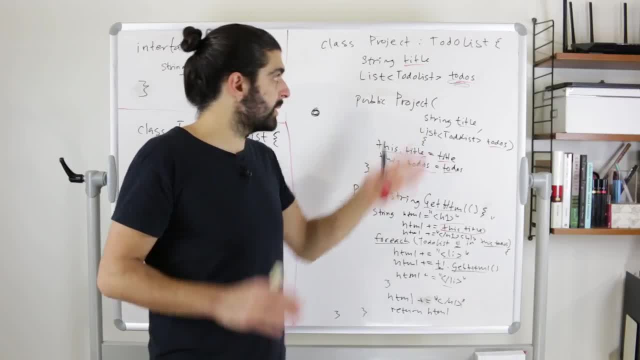 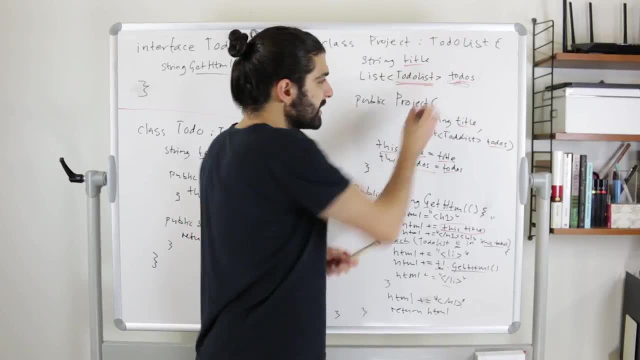 We start by constructing a string that we will return and in the string we will put the title. but we need to put more stuff, and that stuff is dependent on what's in this to-do list, what's in the actual composite, what it actually contains. 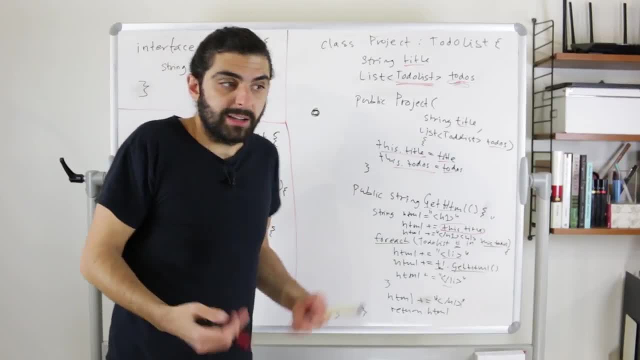 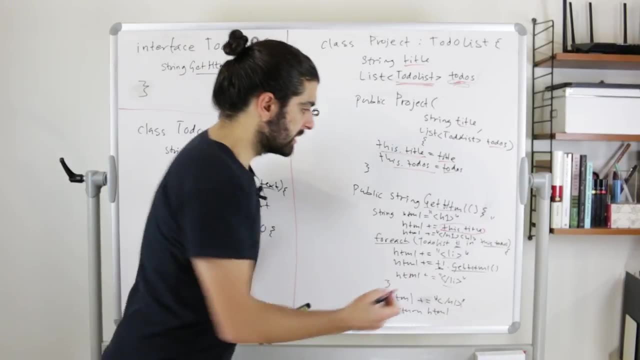 So somehow we have to iterate over that collection that we have, in this case an ordered collection, so a list and simply this is the recursion. ask each of those things for its answer to the method getHTML. So when we call getHTML, 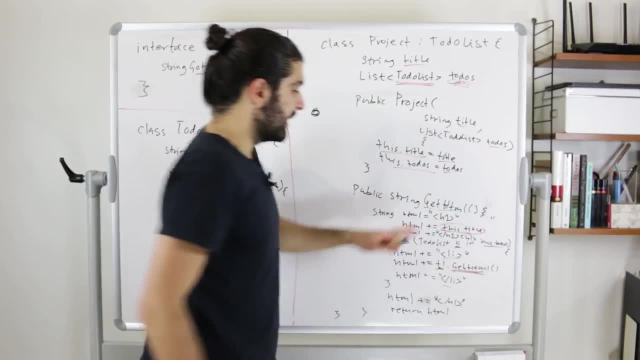 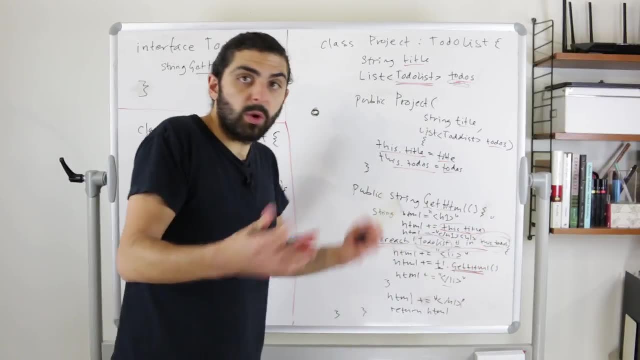 yes, we print the title of this particular project, but that's not enough. We need to also print every to-do list that we have in the instance variable thistodos, In other words, in all of the contents of this composite. So we iterate over the contents of this composite. 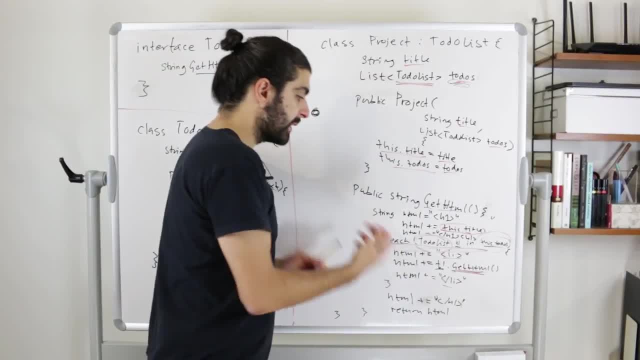 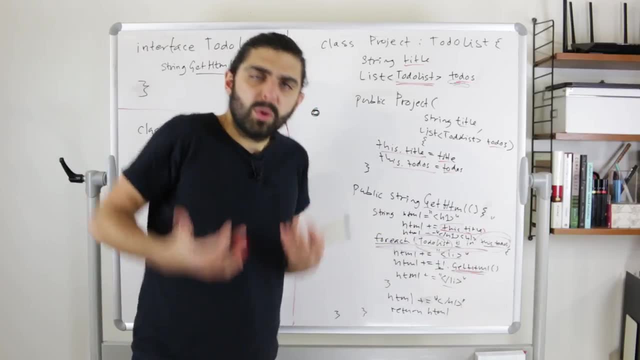 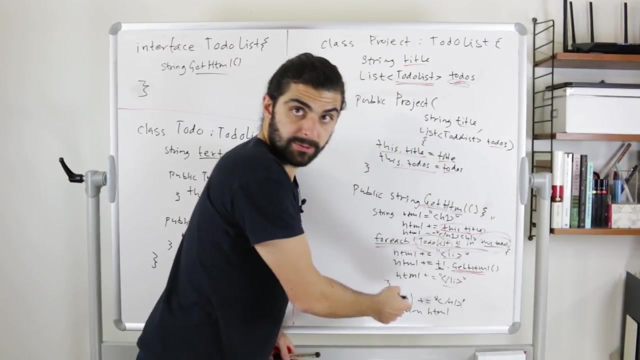 we iterate over the objects that it has, and for each of those objects we do some particular computation. but most importantly, we call getHTML, and since those objects might also be of type project, that means they will also do all of this stuff. 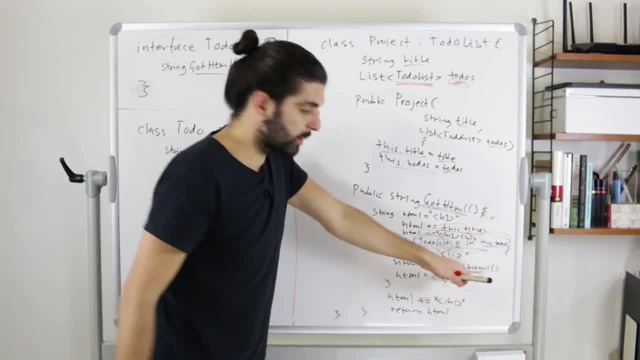 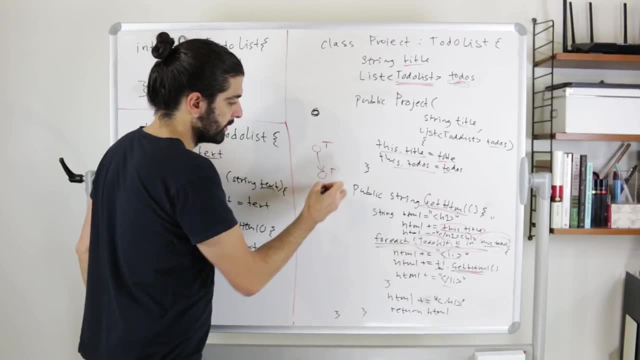 because they also have the getHTML method and that's the method that we're calling upon them and this is the recursion. So you have something of type T and it has another thing that's also of type T and it has another thing that's also of type T. 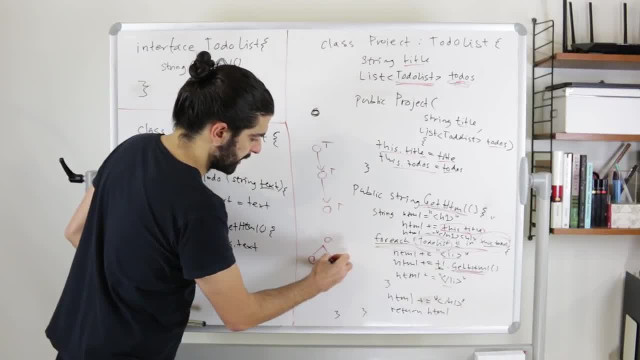 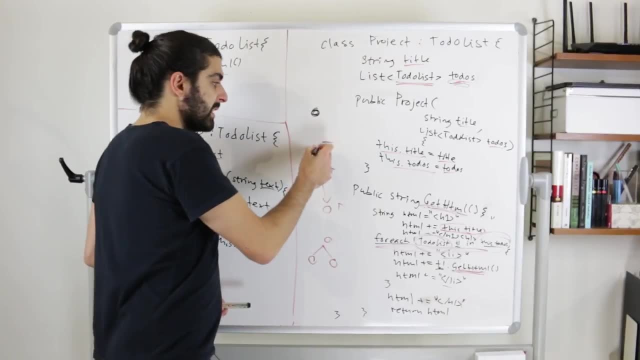 and so forth, but it's actually- I mean, it's more again, because we have a hierarchy like this, so it's more like this thing can have multiple things, but if we just think about it simply, you can think about it as a decorator pattern, right? 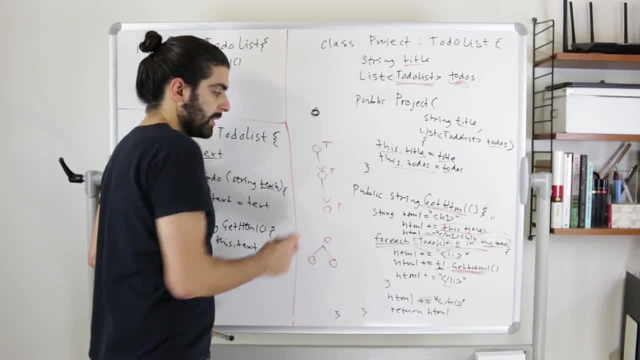 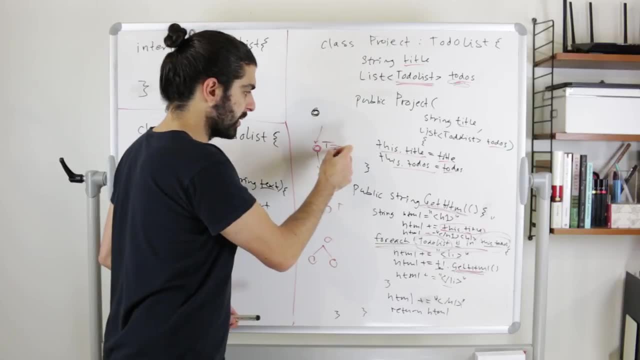 This first thing has a reference to the second thing and the second thing has a reference to the third thing, but they're all of the same type. So when the first one is asked for getHTML, it can't answer. It has to do some computation by itself. 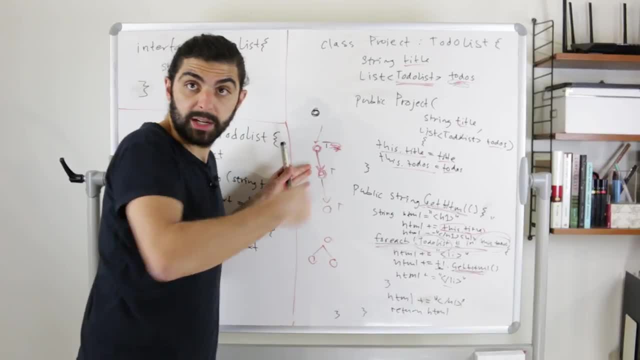 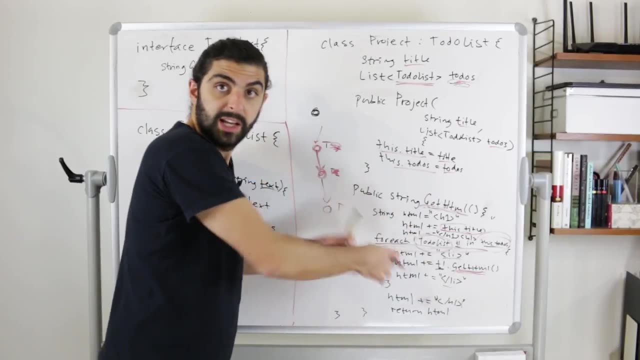 but also merge its own computation with whatsoever in the one it has a reference to, and that one does some computation by itself, actually in the same computation, because it's of the same type. So it's the same method but it's in another instance. 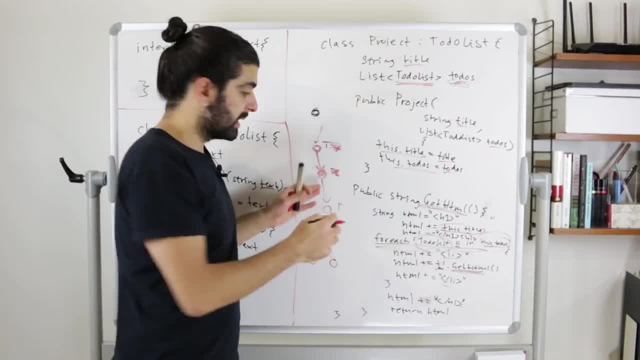 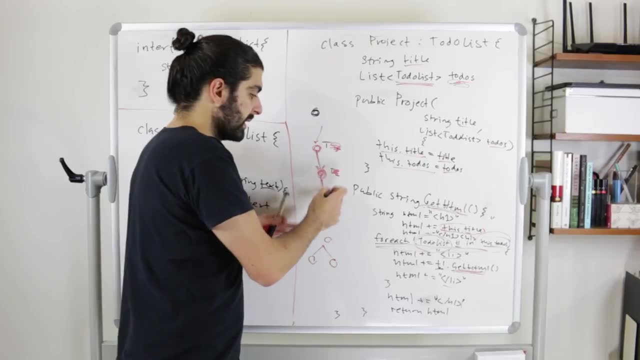 but then again it can't just return immediately because it needs to know what the object that it refers to, what it will respond to in its computation. So it delegates to the next one, to its children, in this case just to its child. 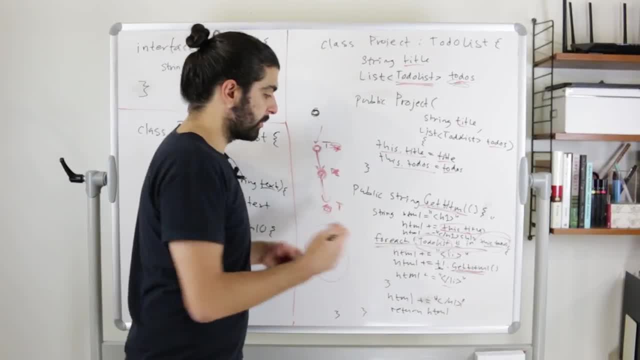 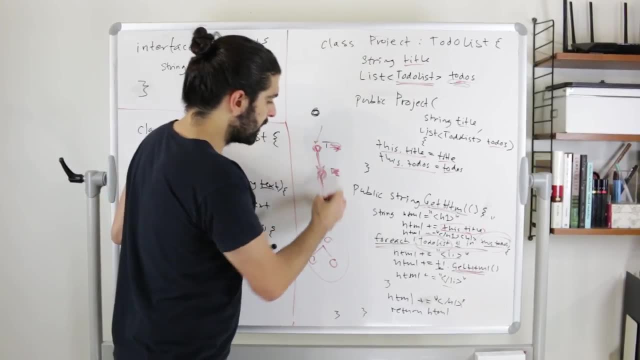 but in a case like this, to its children and asks them to perform their getHTML computation and merges it back with what it has, and so forth. right, So we drill all the way down and then the value propagates all the way up. 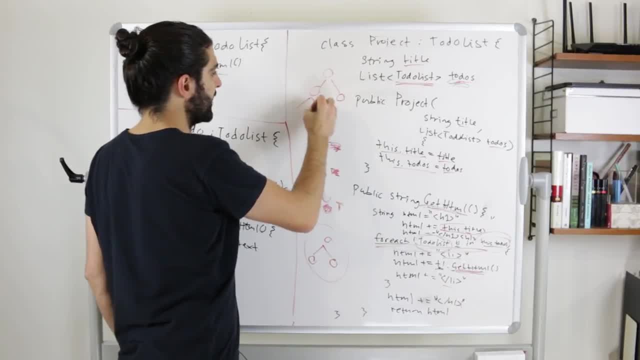 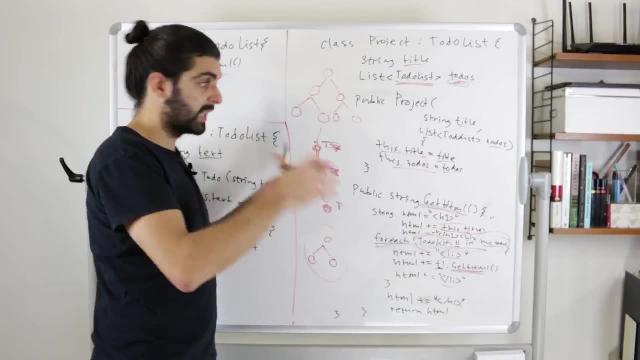 So if you're in an algorithm course and they talk about in-order and pre-order and post-order and all that stuff, this is a way of implementing these orders in which you traverse a hierarchy, because now you can have an algorithm that traverses this whole hierarchy in a particular order. 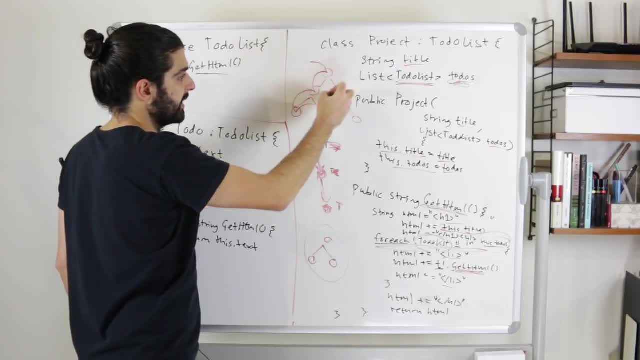 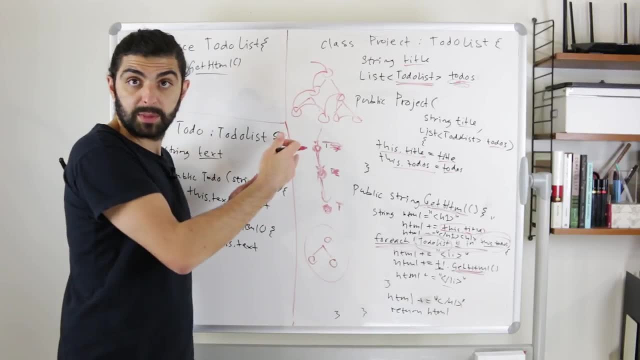 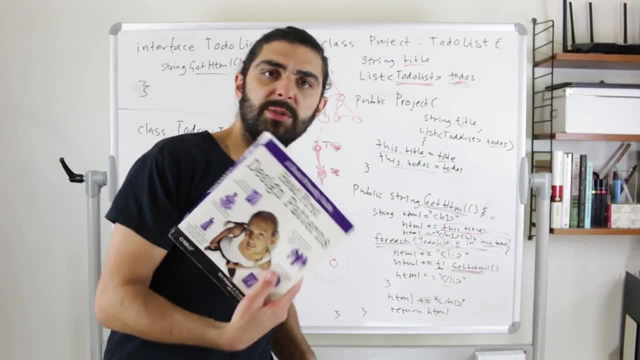 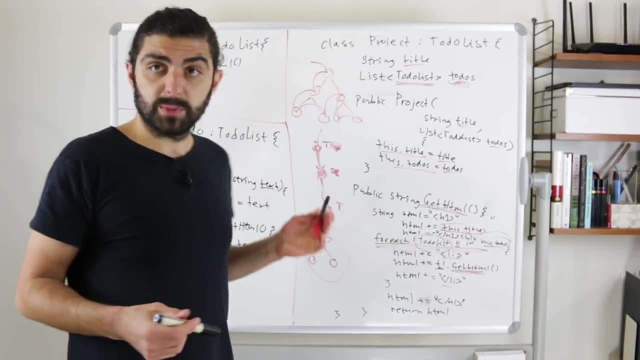 The potential criticism here would be that- and I think that's actually raised by the headfirst book. so if you want to know more about that, check this out. but the potential criticism that could be raised is single responsibility principle because, if you think about it, 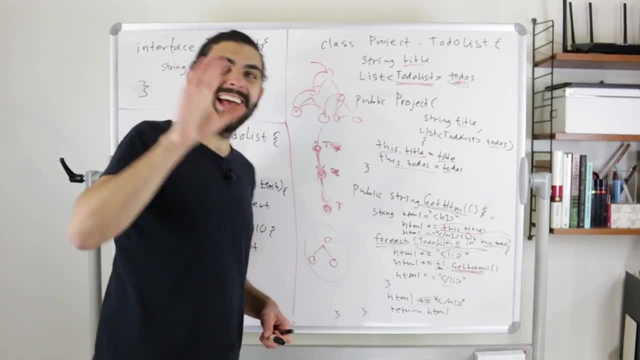 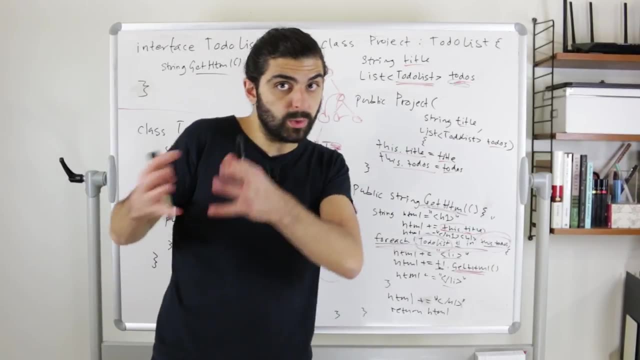 what we want to do is that we want to traverse in a particular order and we want to perform some kind of computation. So I mean, in this case, the computation here is that we want to build up the HTML, and that's one thing. 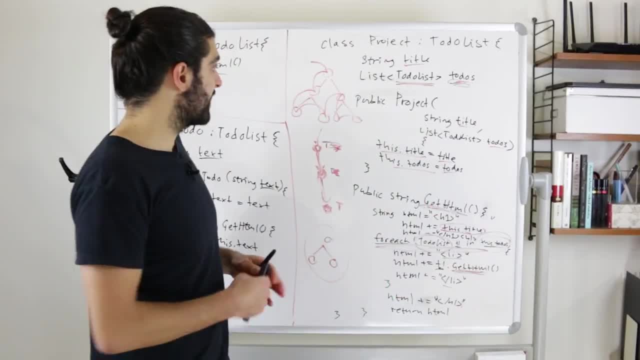 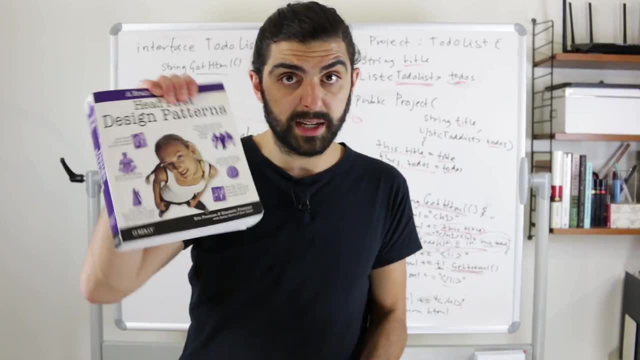 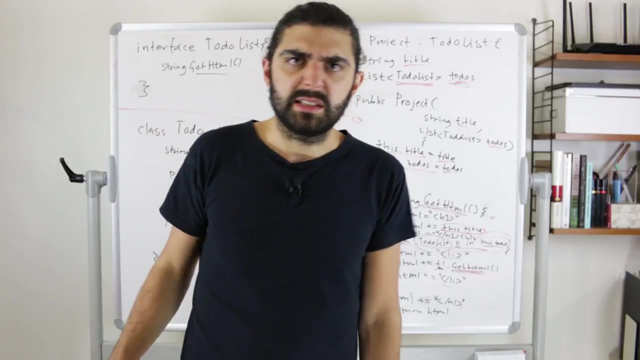 but the traversing is actually another thing. So you could think of a scenario where we would separate the traversion from the actual HTML building, and this is why the headfirst book actually talks about composite pattern and iterator pattern in the same chapter. I separated into two videos because it was super long, man. 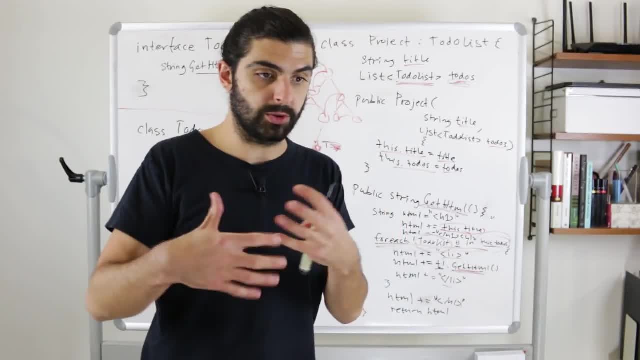 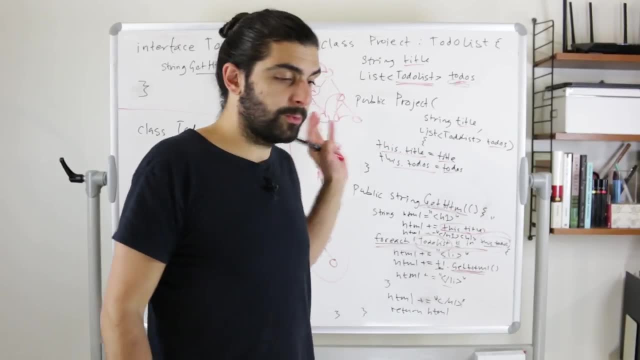 but you could actually do that. You could actually separate the notion of the traversal from the actual algorithm. In one of the upcoming videos we will look at iterator pattern. We probably won't look at code for traversing something like a composite structure or something like a hierarchical structure. 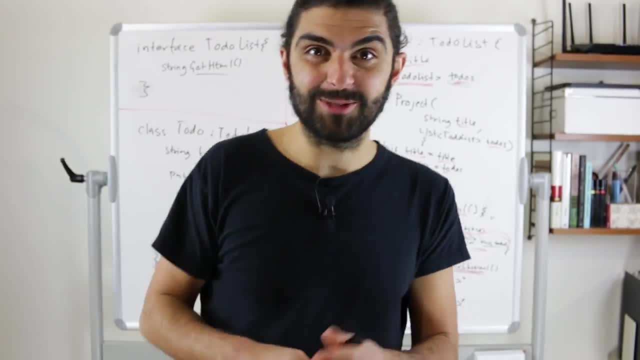 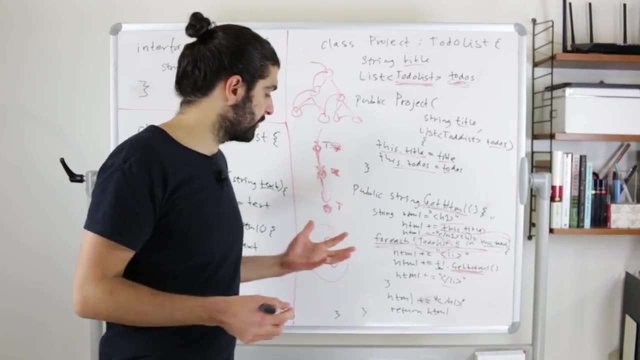 but we'll talk about it. Before we wrap this up, let me mention one final thing. Hopefully you can start to see how this can be very powerful in particular scenarios, especially if you want to do sort of computation over the whole hierarchy without writing really complex algorithms. 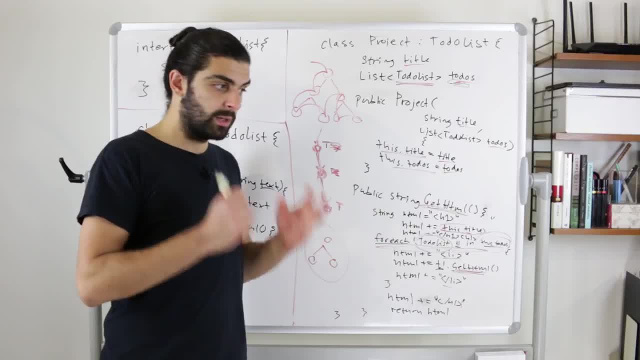 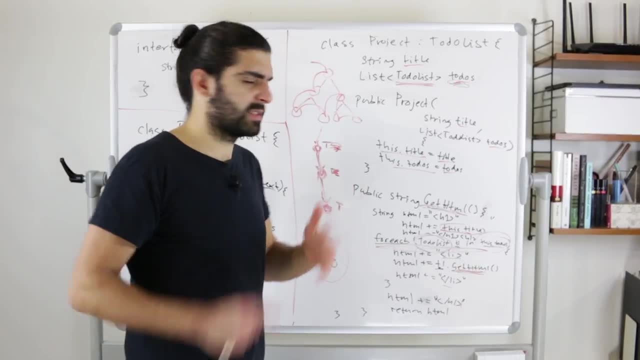 and really I mean generally. this is the power of recursion. Like you can identify very simple algorithms that actually give you very complex answers, That sounds like overly unnecessary complex answers. That's not what I mean. I think you see what I mean. 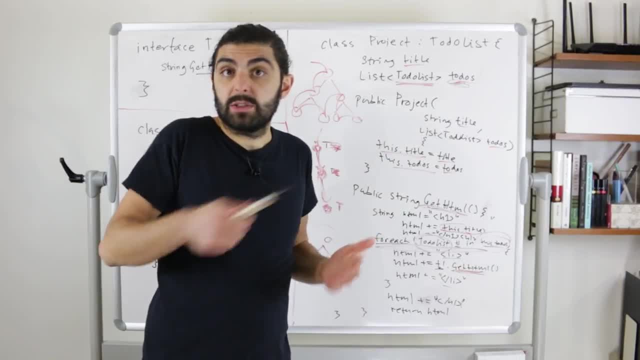 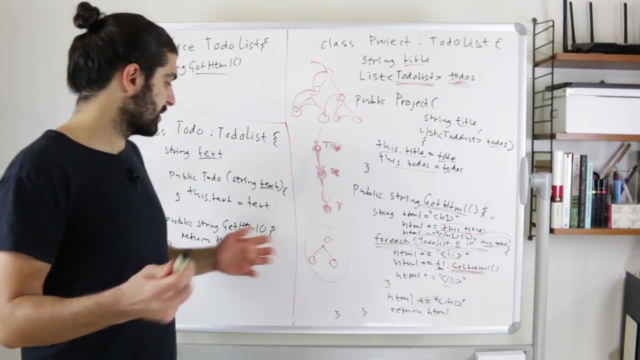 So one example here would, for example, be if we had the check marks, if we had the notion of a to-do being done or not done. I mean there are multiple ways of implementing this and actually I should say there are multiple ways of stating the requirements. 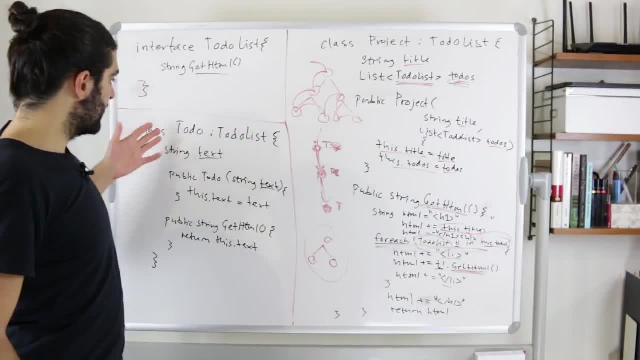 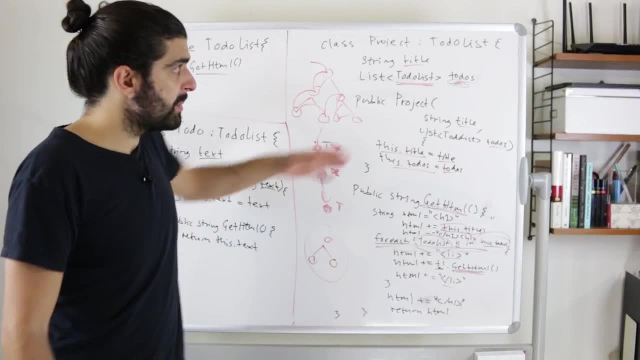 I mean we might have different requirements depending on what application we're building. but let's say, I mean one thing would be that maybe to-dos could be marked as done or not done, and we could also envision that maybe projects could be marked as done and not done. 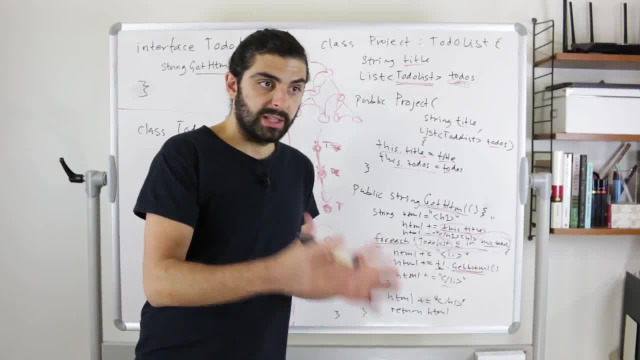 Like. I guess the sort of burning question is: can a project be done even if a sub-to-do of a project is not done? I mean, it's not an insane idea, right? It could be like: well, you just 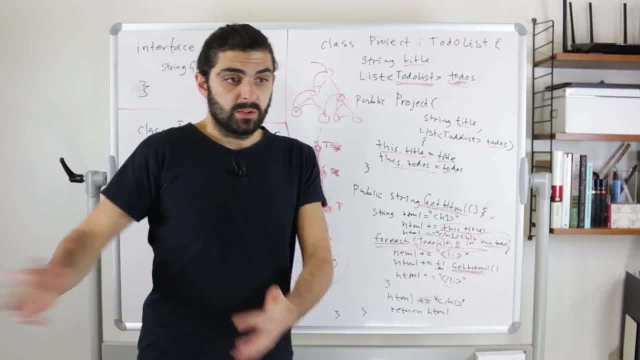 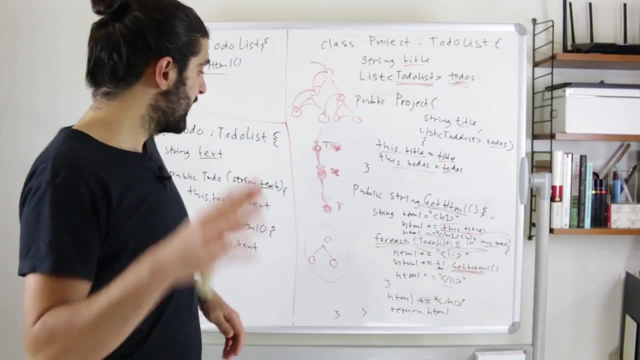 we ran out of time so we closed this project, or we figured out that this to-do was unnecessary so we just said, nevermind, let's just mark the project as done and move forward. This is good enough. I mean, it might be a multitude of different reasons. 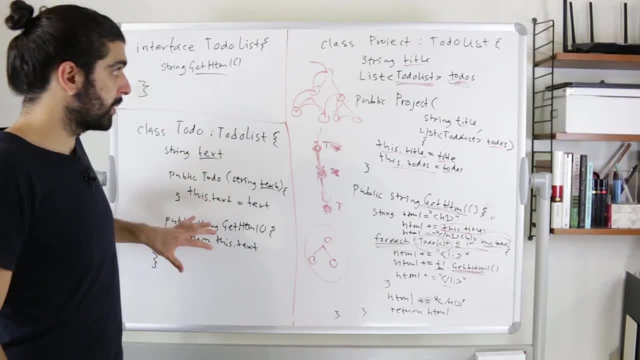 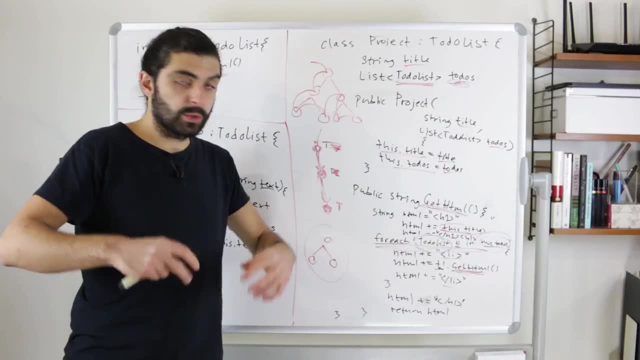 Either way. if we think about the scenario where only a to-do can be marked as done and a project cannot be marked as done and a project cannot be individually marked as done, maybe then the notion of a project being done is a sort of computed property. 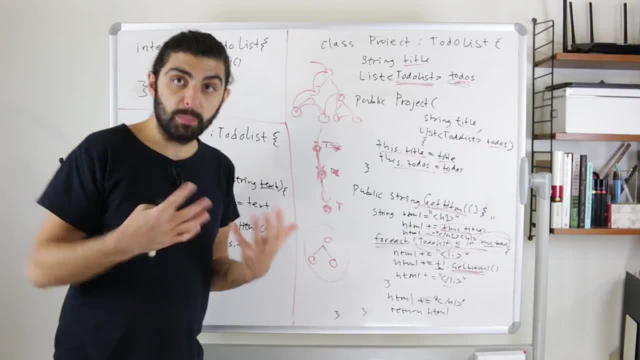 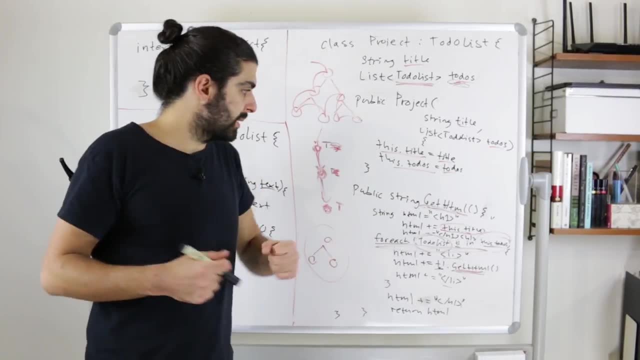 is an aggregate of its to-dos. So if a project is a composite of to-do lists, if a project is composed of multiple to-do lists, and those to-do lists can be projects or individual to-dos. let me express this in simpler terms. 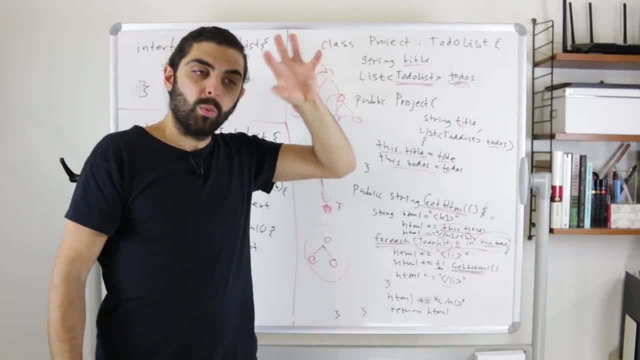 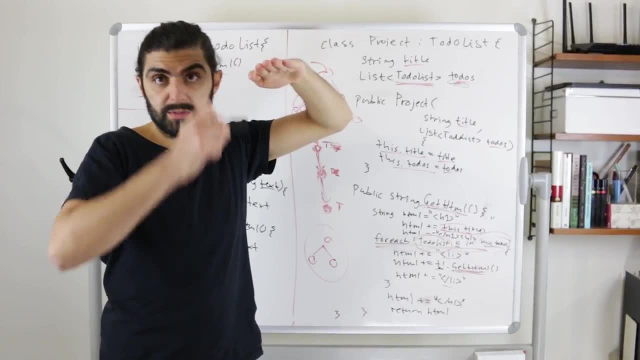 If you have a to-do that has a number of sub-to-dos, what if the notion of that initial to-do being done depends on whether all of the sub-to-dos are done? So if all of the sub-to-dos are done, 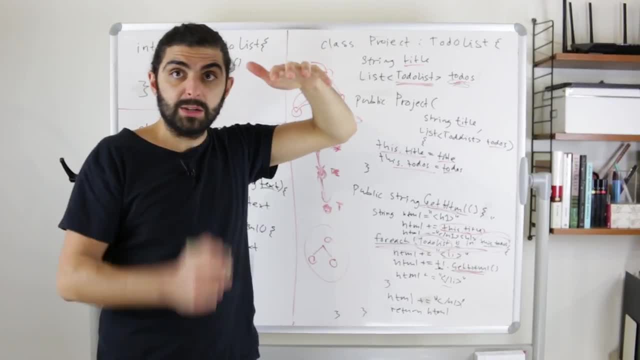 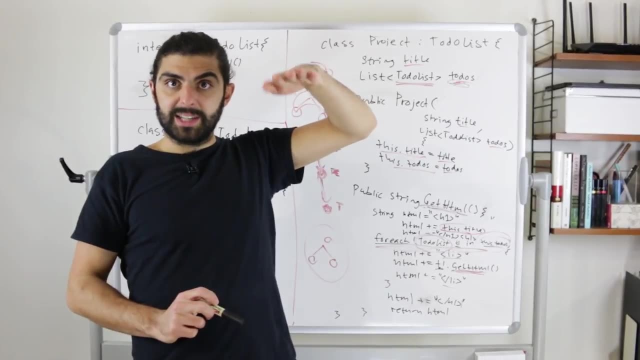 that means that the parent to-do is done. If any of the sub-to-dos are not done, that means that the parent to-do is not done. So essentially it's an AND operation right. We have the parent to-do and we join the doneness of all of the sub-to-dos. 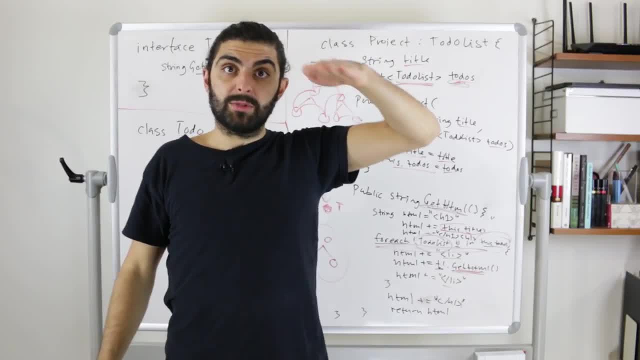 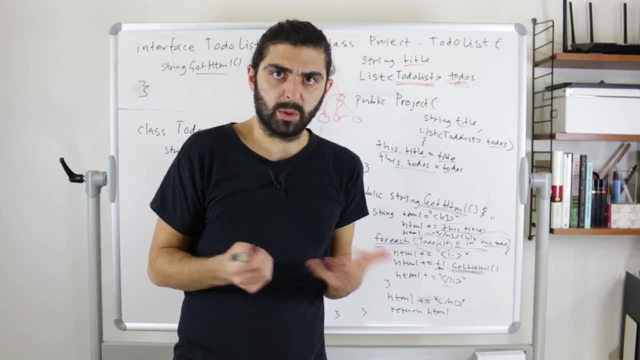 using the logical AND operators. So the doneness of the parent is the doneness of the first child, and of the second child, and of the third child, and so forth, which means that using the operator AND if any of them turn out to be false, 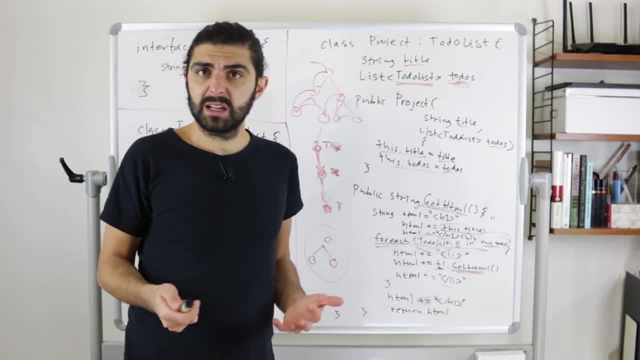 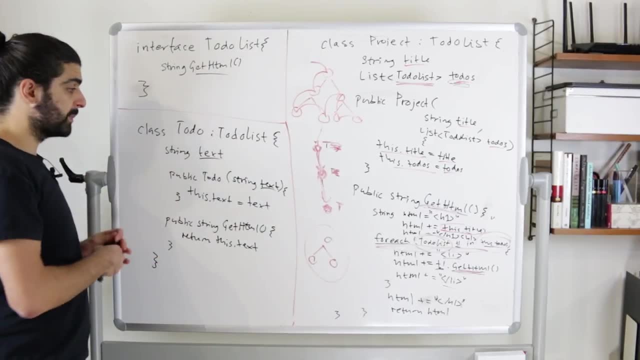 that means that the aggregated answer is false, And this would be extremely trivial to implement in this scenario. So the isDone method in the to-do would be super simple, right? Because that's just a property that is changeable by the user, right? 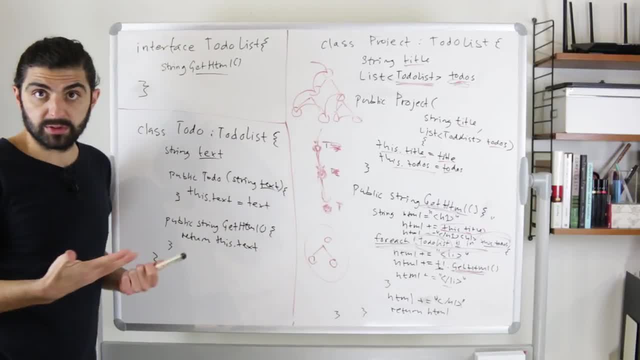 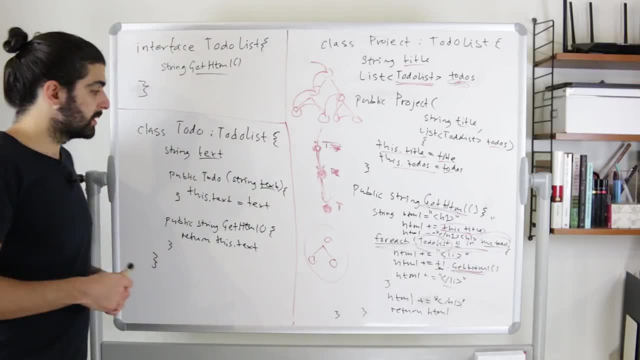 Either the to-do. it's like we have the property's text, but then we would also have the property isDone and that says whether it's true or not. So you have a Boolean here which says that it's either done or not. 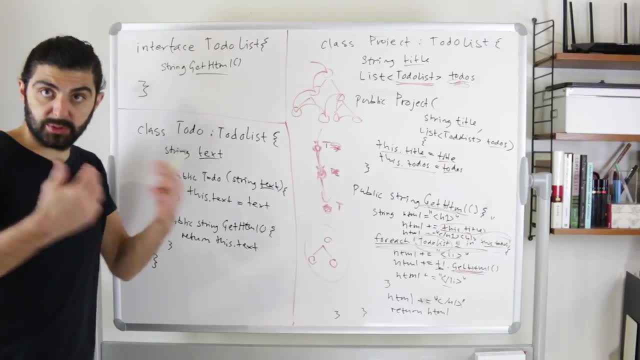 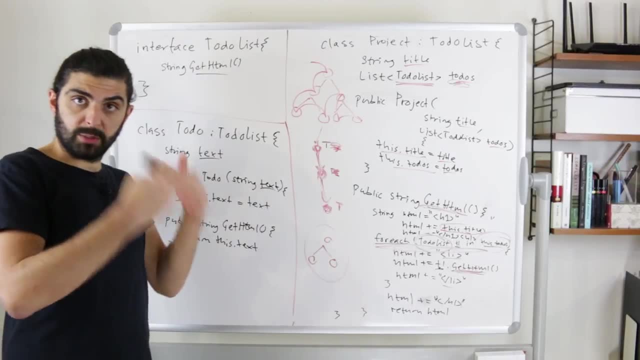 Or if this was built as an immutable data structure, maybe we actually have a done to-do and an undone to-do or a not done to-do, Or maybe then it would make more sense to say that we have a to-do and we have a completed to-do. 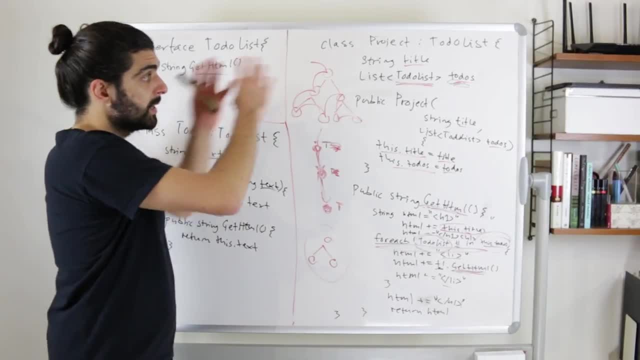 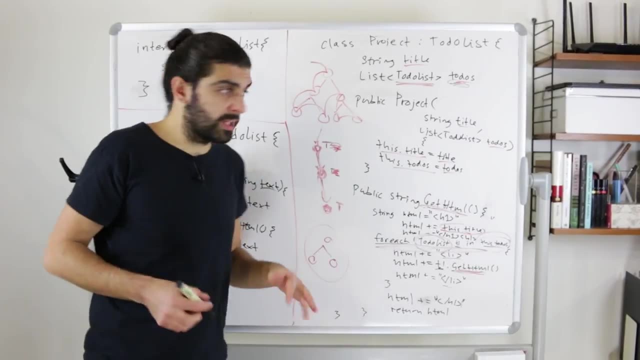 or something like this. Either way, that implementation would be really simple. However, the project implementation, the project implementation for the isDone method, would not be as simple, but it would be fairly trivial In functional programming jargon. what we would do is that we would simply: 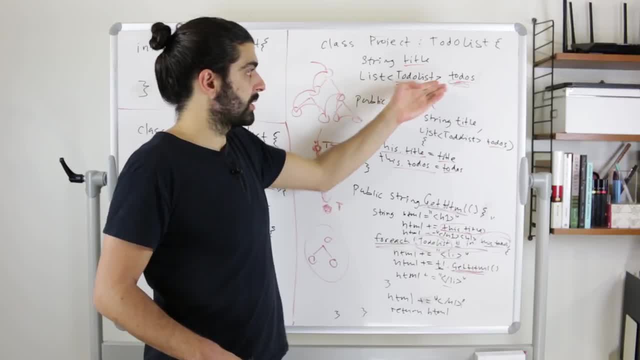 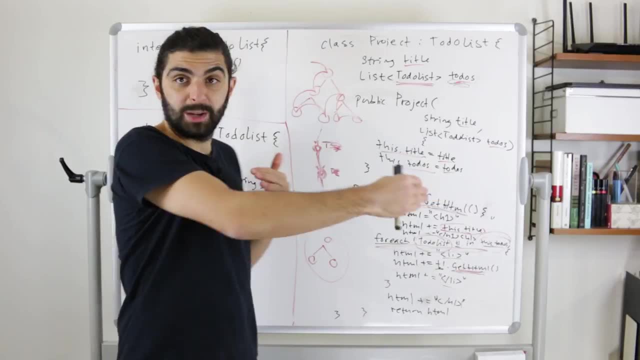 map the function getHTML over the collection of to-do lists, and then we would reduce using the logical operator and right, That's like one line. I mean super simple, But in non-functional programming jargon, what we would simply do is that we would: 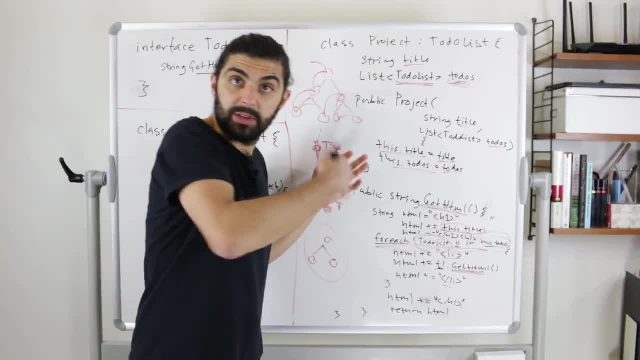 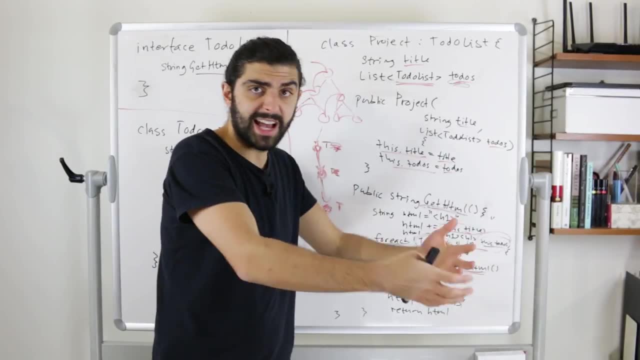 forEach through all of the to-dos in the to-do list and then we would ask them for their isDone. And remember, when we ask them for their isDone they recurse downward, So they ask any objects that they have in case they are composites. 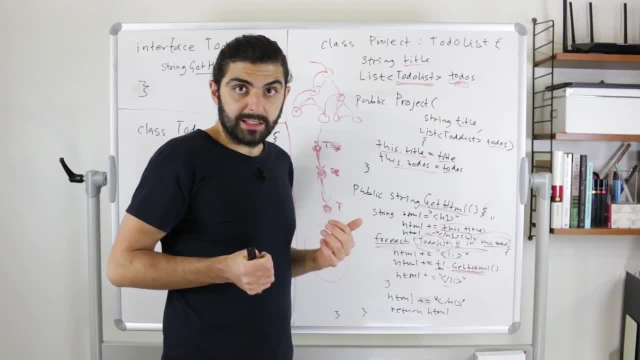 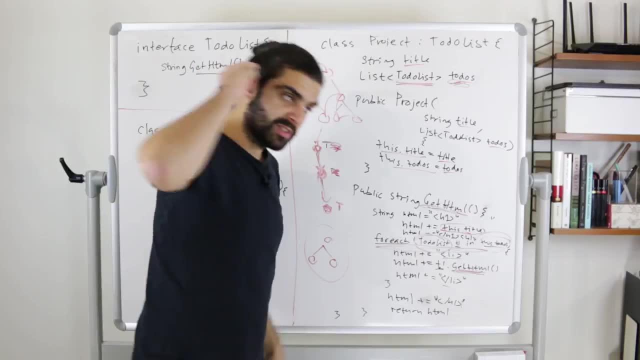 And then if any of them report back that they are not done, then we simply eagerly return false. We eagerly return that well, this project is apparently not done because there's something down the chain that's not done. Somebody returned back false. 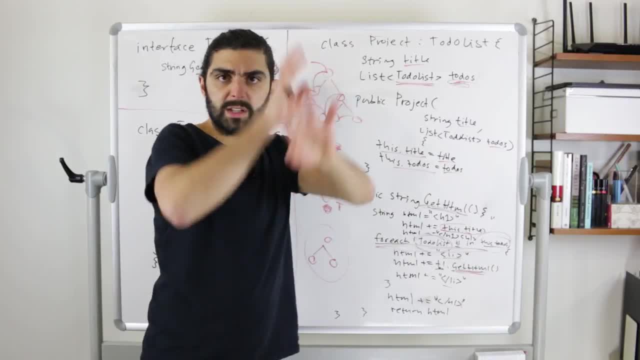 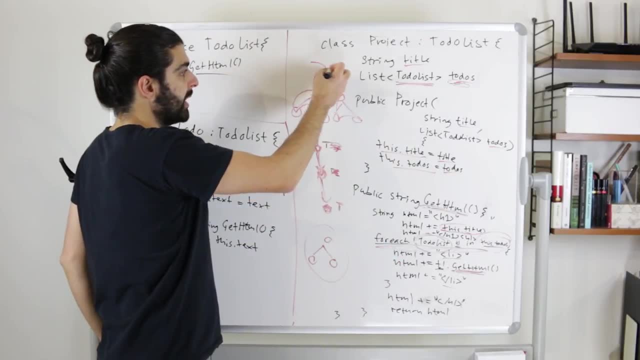 so we immediately return and we say false, This is not done. And if none of them do that, then we just return true as a default, because then apparently this has to be done. So that means again that if you have this outer project, 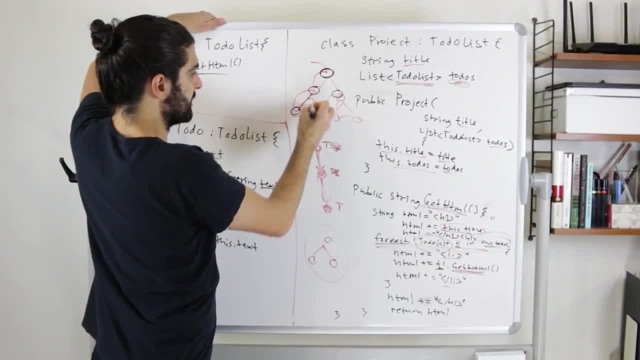 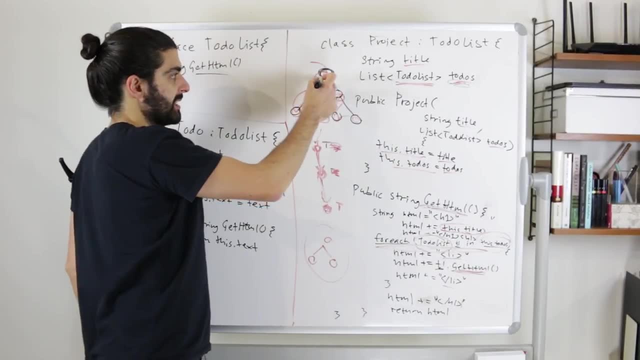 that has two sub-projects and these two sub-projects each have two to-dos. then, and these two sub-projects each have two to-dos, then when we ask this outer project if it's done, it will ask: well, are you done? sub-project number one: 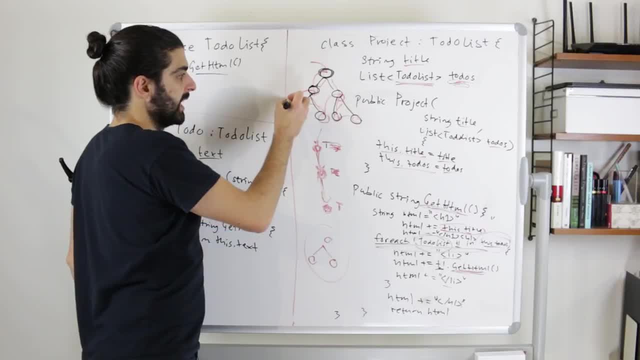 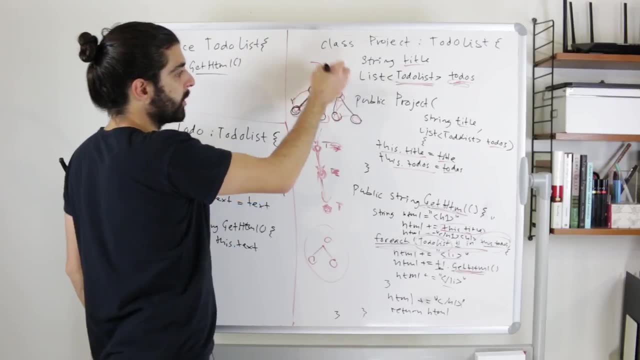 And sub-project number one will ask its to-do number one: are you done? It will say maybe yes, and this one will say maybe yes. so then sub-project number one will report yes, But that's only one part of the problem. 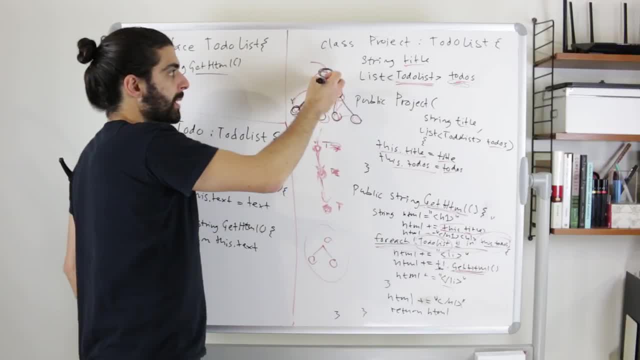 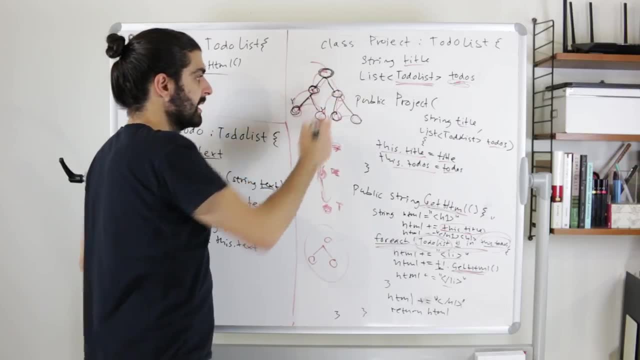 Then this outer one, within its forEach or within its map, will ask the next one sub-project number two: are you done? And it can't answer right Because it's a composite, so it asks its to-do number one. 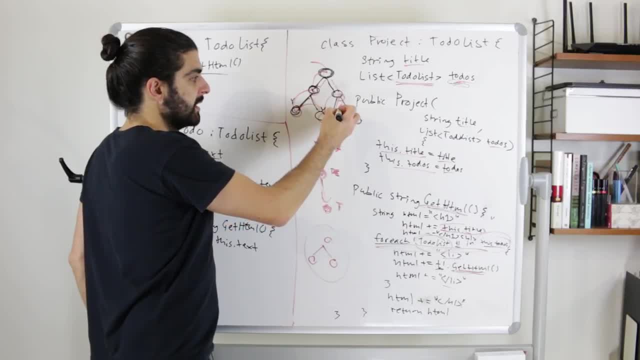 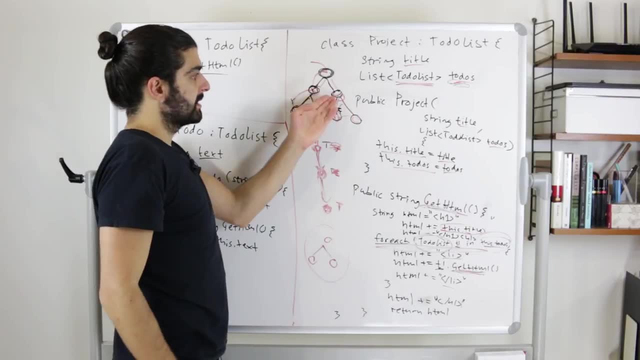 it's to-do number one: are you done? And maybe that says false, no, it's not. no, I'm not done. Then we don't even bother to check this one, because that's why I said eagerly return. So then this sub-project one says: 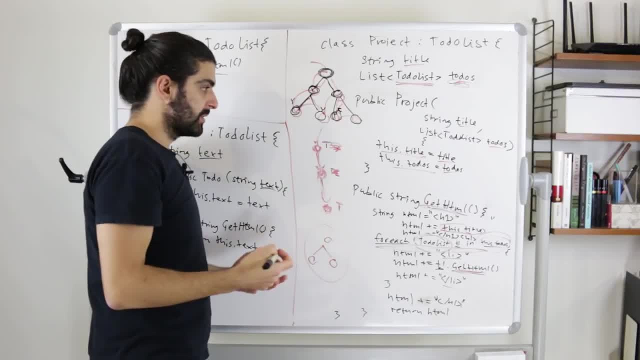 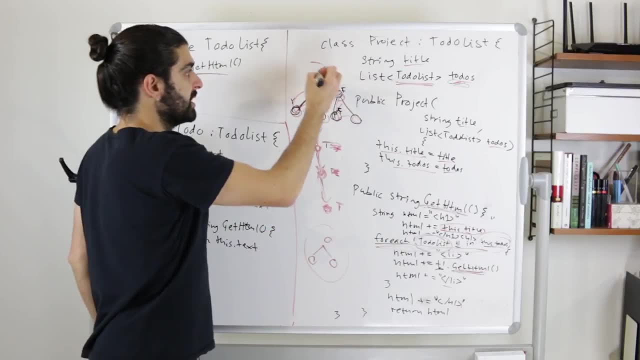 actually in my forEach I noticed that one of my to-dos answered: false, that I'm not done. Then I'll just immediately report back up: false, I'm not done. And then we know that this project then is false. 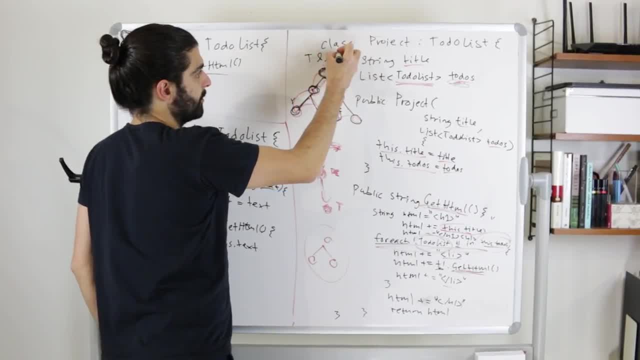 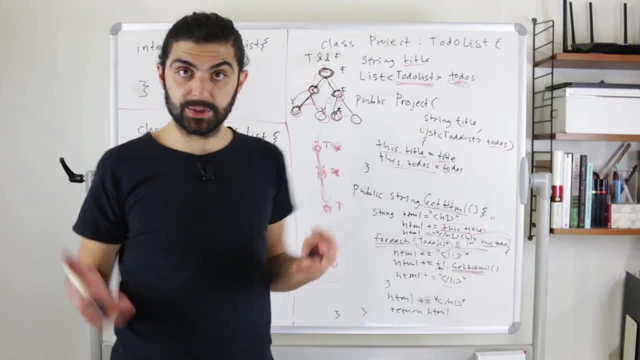 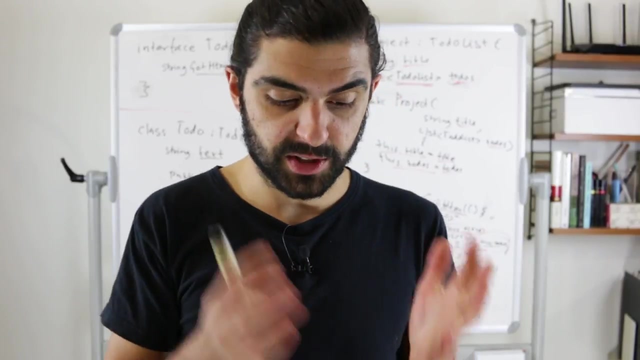 because we're doing a logical comparison between true and and false, which is clearly false. So again, hopefully, you see how somewhat complex problems suddenly become very trivial because we have an appropriate data structure, Anyways. so I mentioned in the beginning that I would shortly talk about the differences. 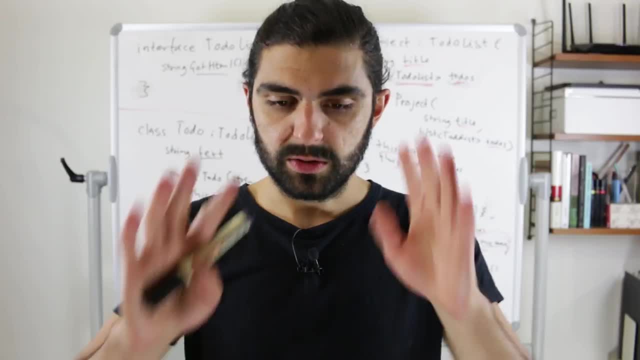 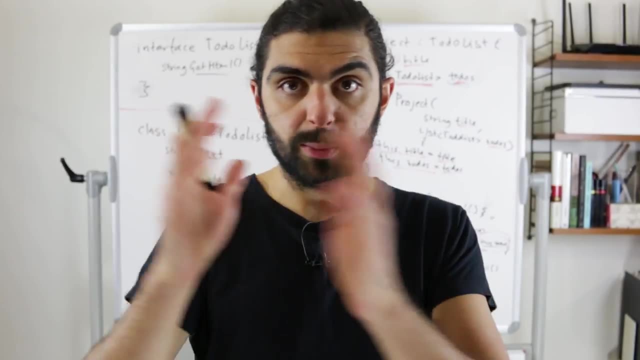 between composite pattern and decorator pattern, but this video turned out so long, so I think it's best for everyone if we don't do it now. Instead, I will make the next video about exactly that: the differences between decorator pattern and composite pattern.